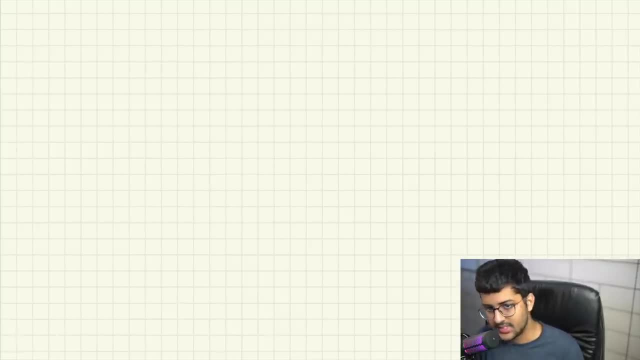 into like classes and like objects and stuff, so it's easier to you know, like break your code down into chunks, Chunks of code So it's easier for you to like debug it and change stuff and things like that. All the things were covered in the introduction to programming video And 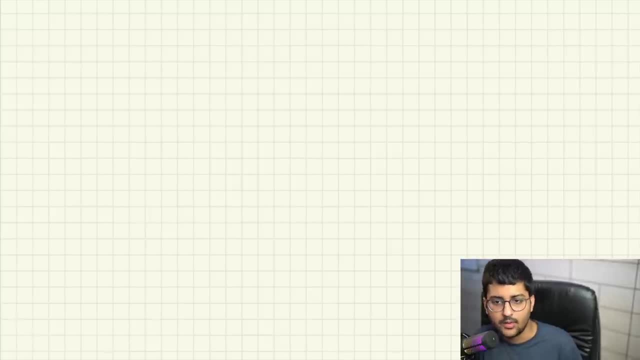 in the previous object-oriented programming videos as well, we gave it a very more hands on approach. Now in this section we are talking about: okay, object-oriented programming is fine, Kunal, it does this, it does that. You know you are saying it has so many benefits. 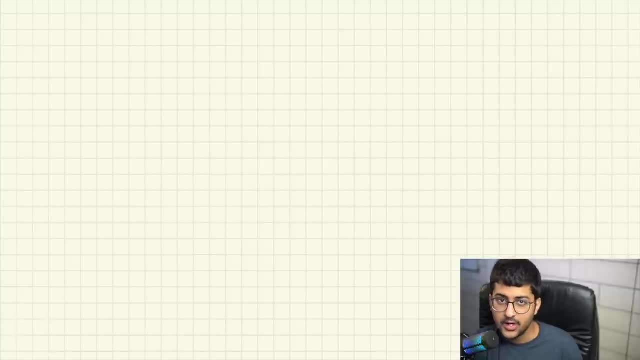 You divide your code, you provide some security to your code and some access and stuff and you provide some rules to your code sample make it more secure and things like that. But how? How can we do it? We know object-oriented programming does this. We know OOP does this. 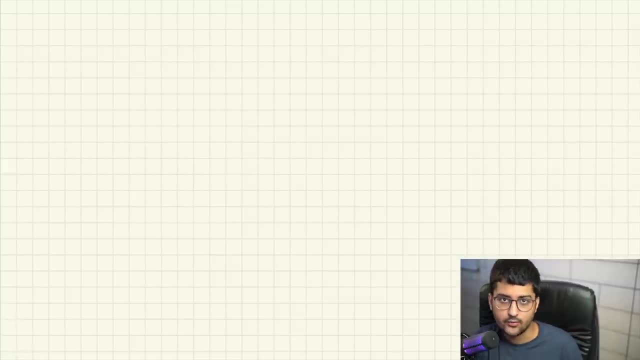 But how does it do it? For that we have to look at the properties of OOPs. So there are like four fundamental properties, like four important properties, the main properties of object-oriented programming, and that is something we will discuss in this lecture. 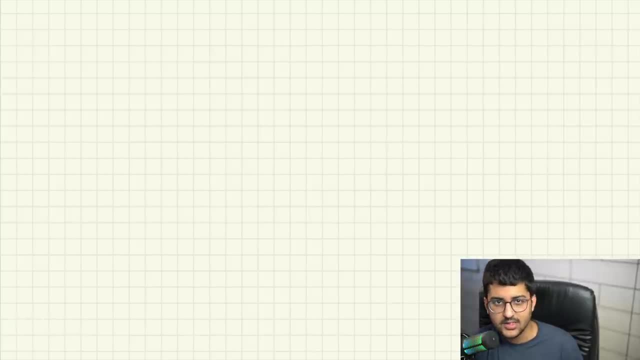 So this is the most important lecture for object-oriented programming. In interviews, mostly these questions asked about properties. cool. one more thing about properties is that many people have difficulty distinguishing between the properties, so i teach you everything about it, okay, literally. first, property is like four properties we're learning: inheritance, polymorphism, encapsulation. 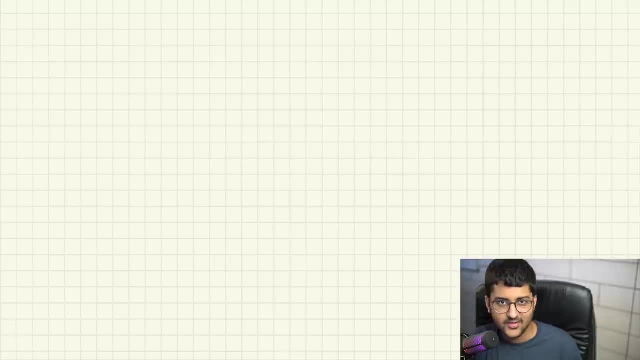 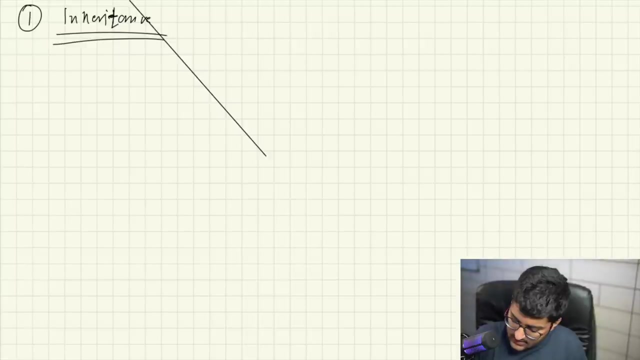 and abstraction, even if you think you know about it, trust me, we'll learn something definitely amazing over here. let's get started. so first one is inheritance. what is inheritance? um, the first property of objective programming we'll look into is inheritance. okay, so what do we mean by inheritance? inheritance is same as- uh, you know your. 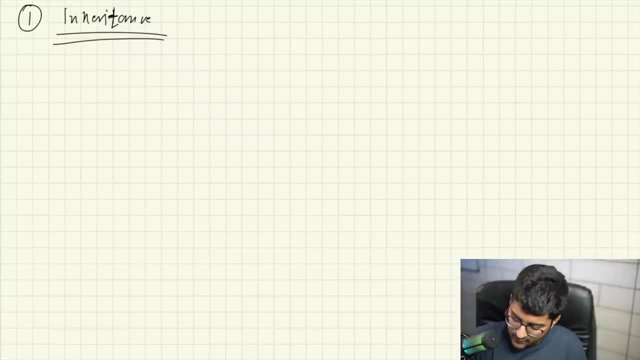 inheritance in your like, uh, in the real life you have your parents, okay, so you have your parents. they have some properties and stuff like that, like literally properties or money or something, and uh, the they pass it on to their children, okay, so not just, not just that they pass on things like 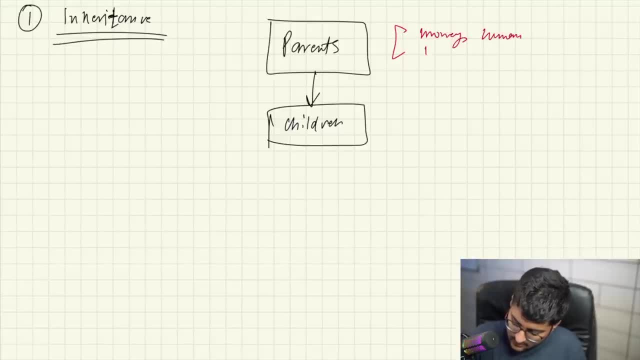 money, human traits- right. so people say you look like your mom or dad or whatever. human traits, values- okay, all these other things they pass on. so they have all of these things and the children can use those things- okay, children can use those things, all right, that's it. that is inheritance. in terms of classes, we can say that a particular class 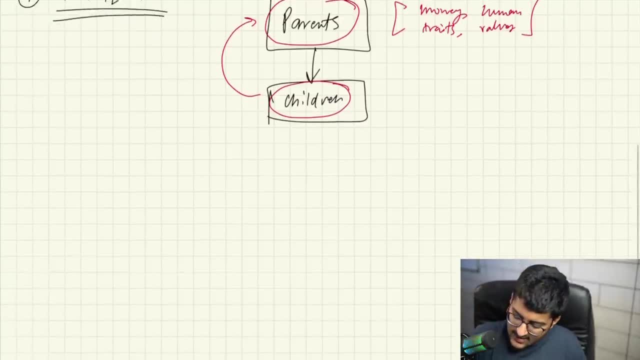 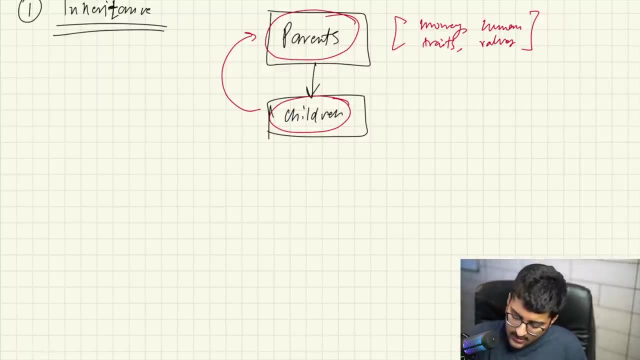 what is class? name, group of properties and functions. a class has, like, some variables or functions or whatever. so we can say that if there's a class that is able to use the particular properties and functions- i mean you see basically the, the links here- exactly properties and stuff of the other class from which it is basically what it means is that 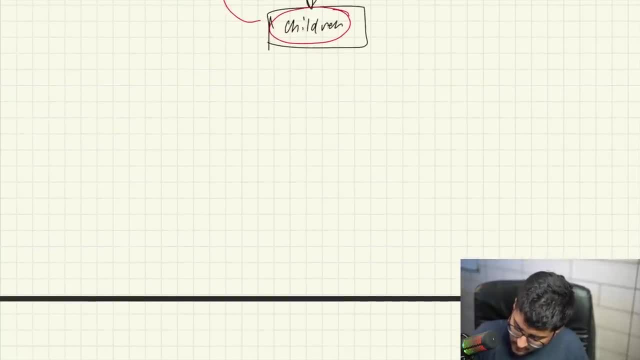 in object oriented programming sense. in object oriented programming this is known as, like the base class, normal class. any class is base class and any class that it derived from it. this is known as child class. child class is going to have access to the members of base class if base class has, let's say, something like some variables like length, width and 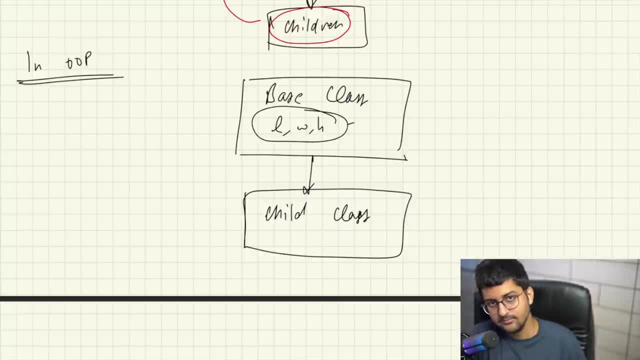 height and child class will have access to length, width and height: okay. child class may also have some additional arguments, like weight. let's say, if we are talking about a box, okay, weight. for example, for obvious reasons, is the base class going to have a variable known as. 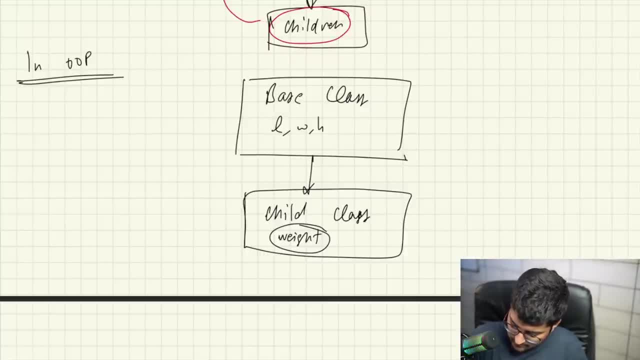 weight. no, because it's specific to child class only. okay, that is it. so this is known as inheritance. this child class is inheriting properties from base class. okay, the child class is inheriting properties from base class. this is known as inheritance. okay, so you can say that these are sort of like interlinked with each other, or 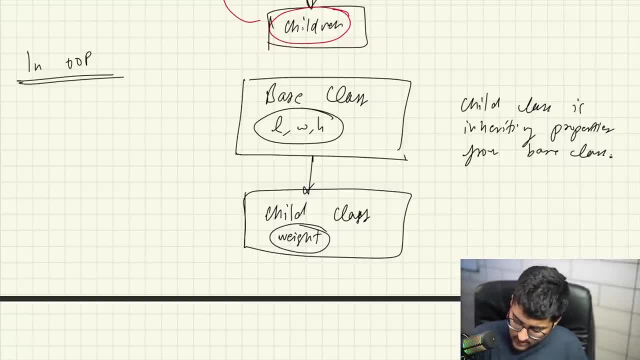 something. if you want to use that like this child class, you can definitely use the the base class as well. the properties are the base class as well. as simple as that. that, is it okay? so just to simply like to incorporate, to like inherit a class if you want to inherit. 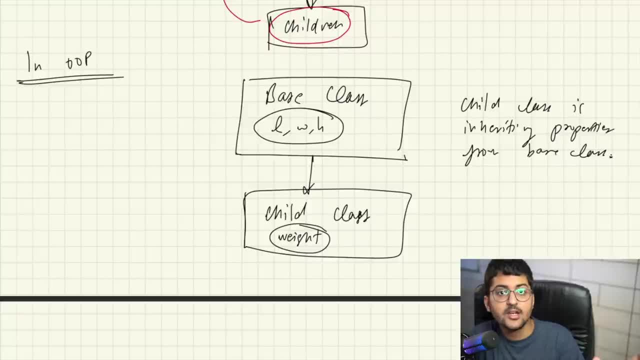 this base class. you simply just incorporate the definition of one class in another class. basically, class is what it's: just a definition, it's a template. so how do you incorporate the definition of this? let's say, the definition of this contains length, width and height. how do you? 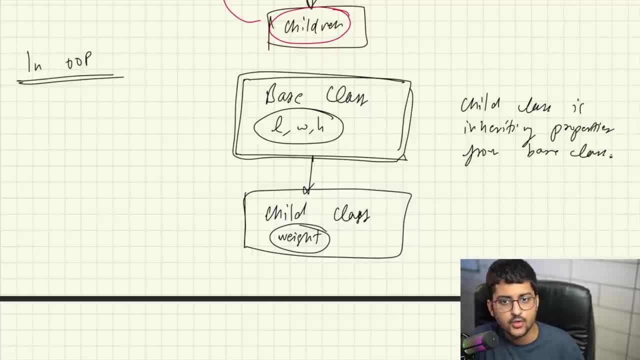 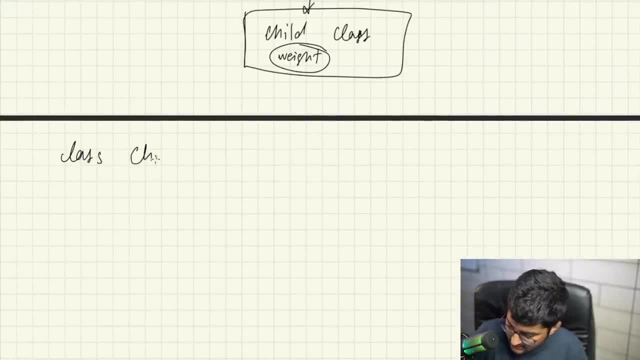 incorporate this in this in the child class, using the extends keyword. so you can say a class, child class, extends keyword, base class. now what will happen is child class will have whatever you can say int weight, but it will also have access to all the properties in the base class. 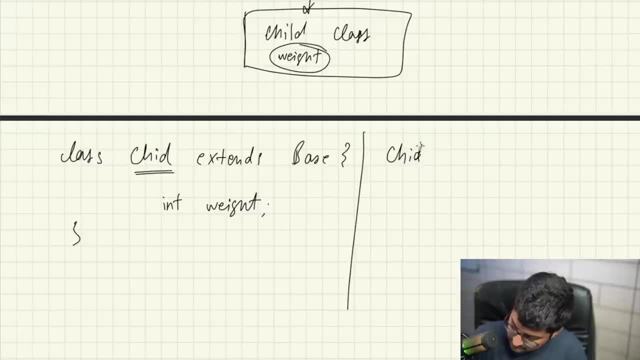 okay. so if you do something like this, if you say child, child is equal to new child and then we'll say child dot length or child dot width or whatever should be able to give it. we'll talk more about how constructors work in inheritance, but that is like i'll cover it in this video. only, obviously, child. 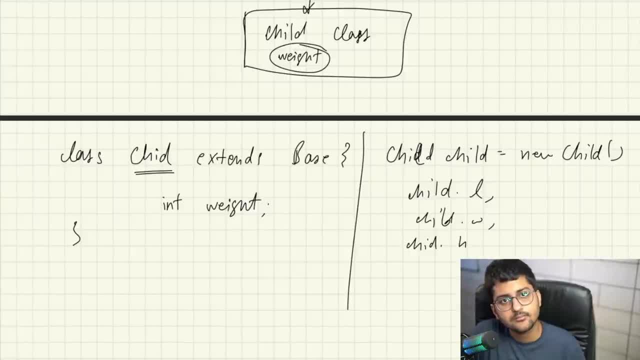 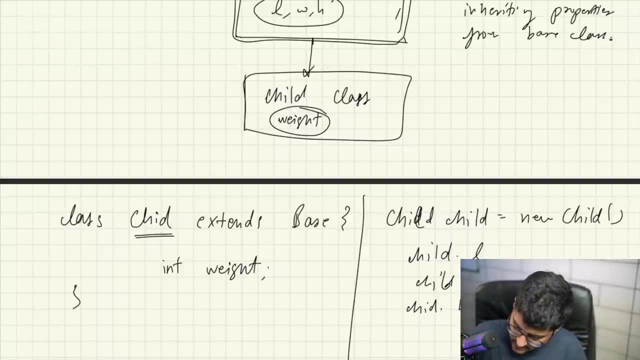 dot length, width and height. okay, that is it. so it's going to be like hey, does. when you take for, when you call, like, when you try to access child dot length, it'll be like: hey, does the child class contain length? it's going to be like: 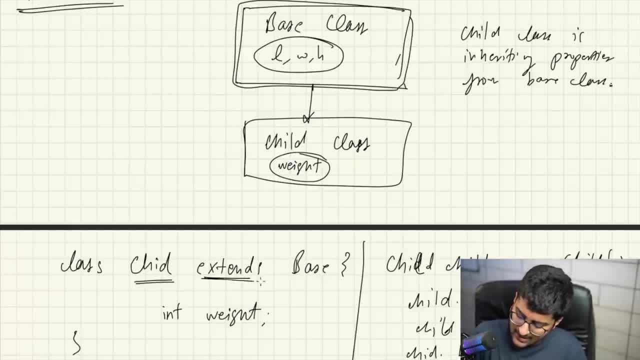 no, it doesn't. then it's going to be like: okay, well, i also know that child class actually extends the base class. so does base class contain length? it's going to be like, yes, it does, and it's just going to print it. what does it mean? it means that if you're extending a base class to a child class, 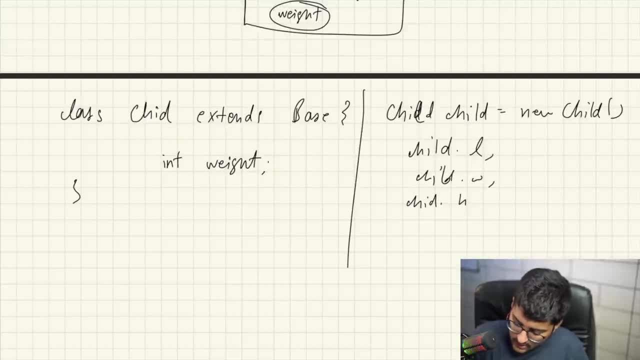 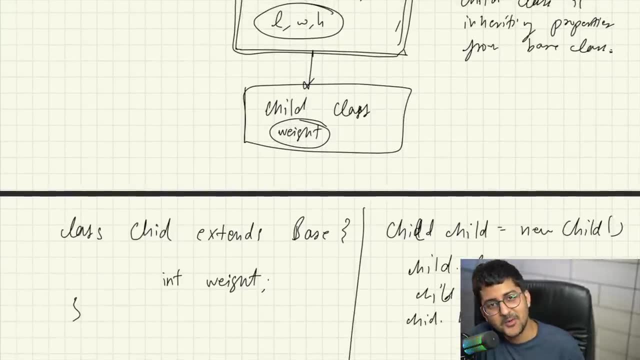 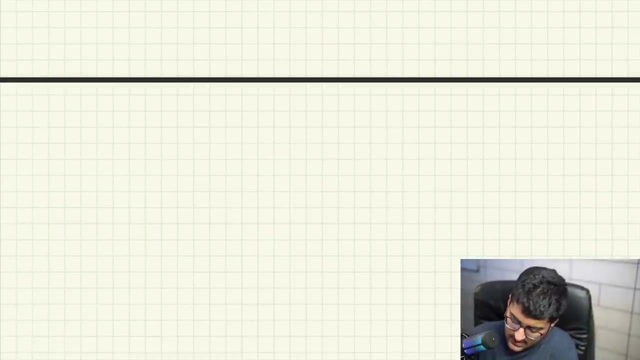 like this: if you're inheriting one class in another class, so when you're calling the constructor, you should also define the properties that are in the base class make sense, because if you want to access the properties, so, for example, why does it make sense? let's see. so let's say there's a human, there's a species class- okay, species. 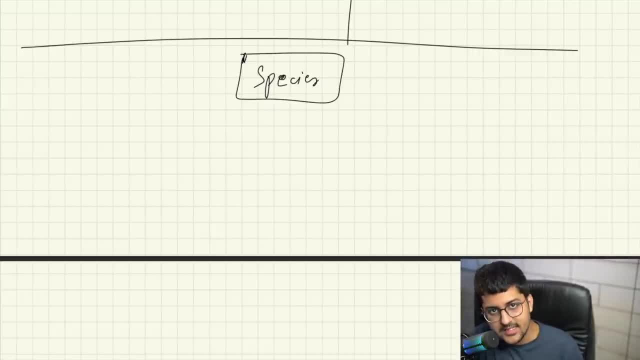 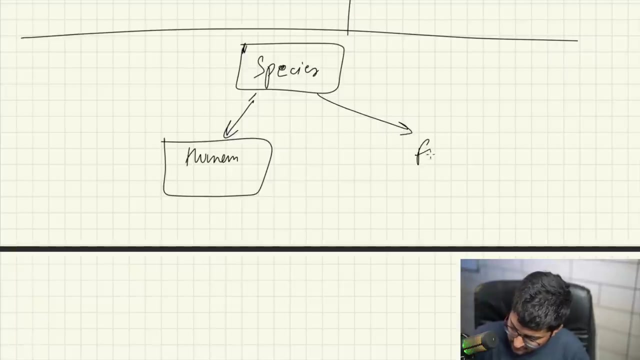 okay, some properties of species will be available in the classes that come into species. what all classes come into species- human fish, okay, so what is the meaning of this? obviously this is a child class, right? because it's very simple, let me explain it to you. child class basically means it will have the properties. 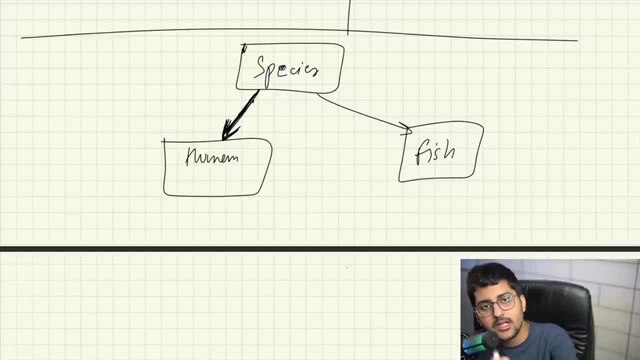 of the base class. plus, it will have some additional properties of its own. that is what child classes. it will have the properties of the base class. let's say this only has property of. let's say it has a property of species, has a property of something like this: 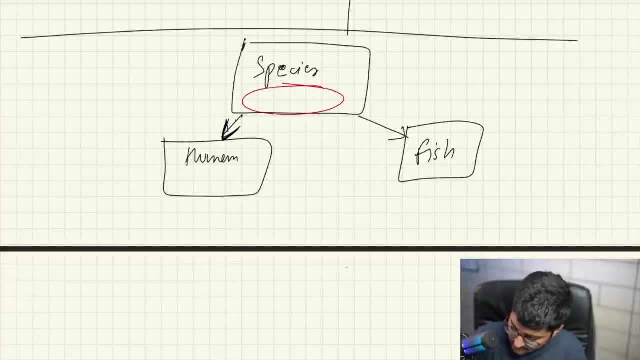 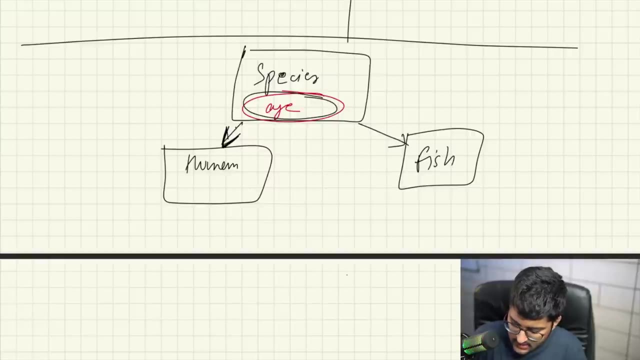 species has some property, something like, let's say, age, age or something. okay, so human being is sharing the age parameter with with this, with the main class, obviously species, because it comes under that class, obviously fish will also have a variable age. so whenever you call some like human, kunal is equal to new human, okay, and then you say kunal dot age. 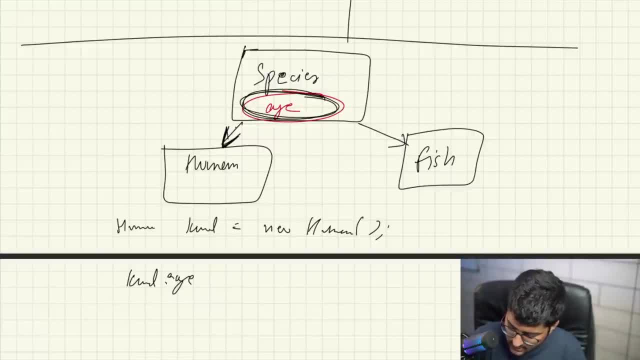 then it will actually try to get the age from here, because it does not exist over here. to like. okay, species has an age parameter. i will take this. but if you're trying to access some variables that are available in the parent class of a child class, they also need to be. 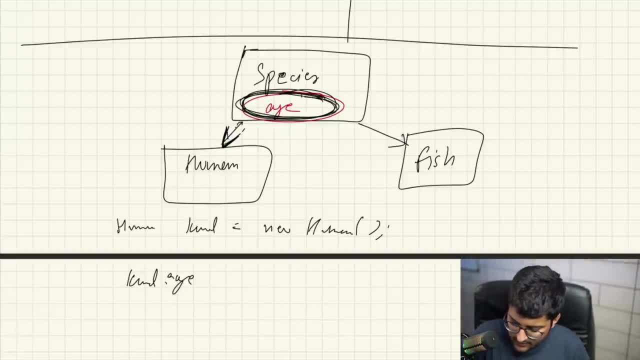 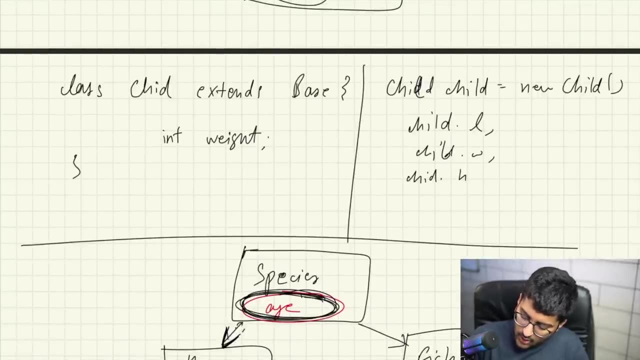 initialized. this age is obviously specific to this human. for every single human, their will be different, different age. so, similarly, for every single human, we have to specify the age. okay, what I wanted to talk to you about. so whenever you call a constructor like this, you have to. 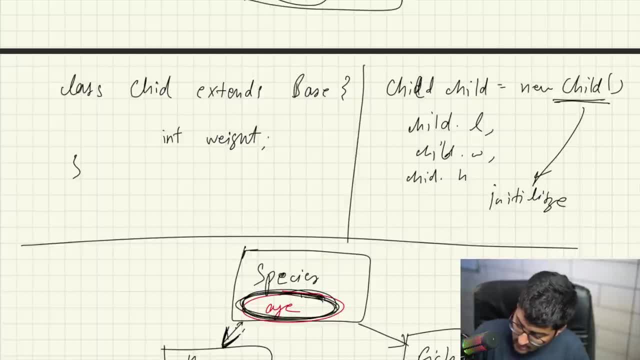 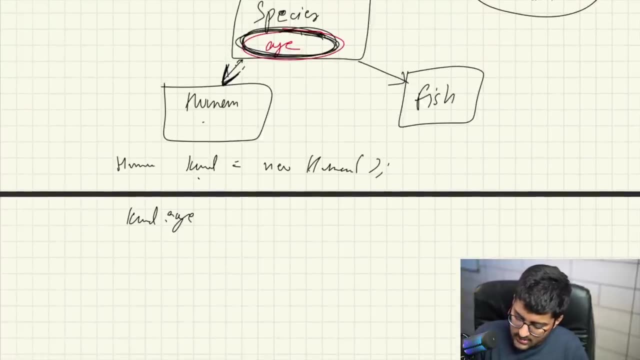 initialize parent class variables also for obvious reasons, like this species example. okay, it's gonna be. what is an age of Kunal? age of Kunal actually lies over here, because just an age parameter that I'm reusing, so I can reuse it, no problem. what do you mean by reusing? reusing? 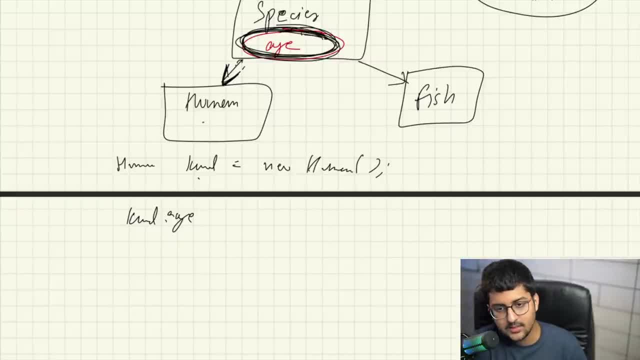 it does not mean that this reuse basically means that you don't have to put like an additional variable age over. it's just a bit more organized, if you will, because if every single child class of species contains age, then just put it over here in the main one. they can all use it, you. 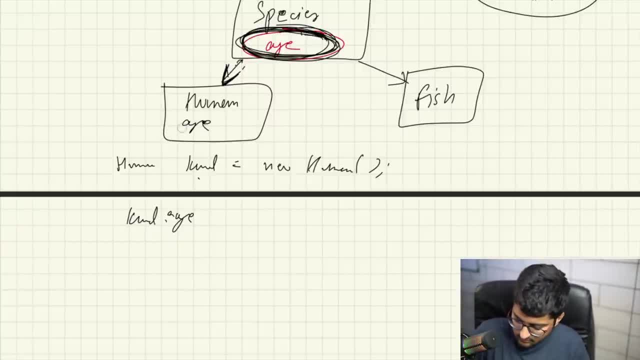 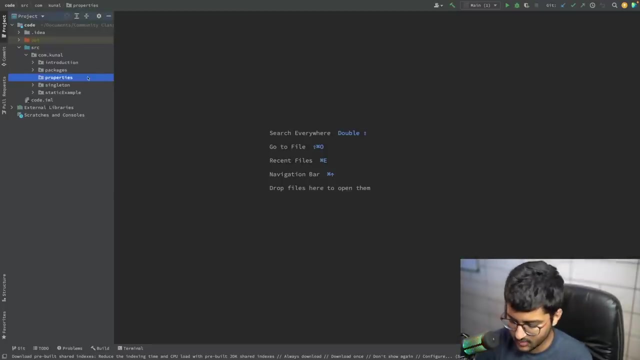 can imagine it lies over here. you can imagine it lies over here. you can imagine it lies over here. okay, so you use it. you do that by other extends keyword. that's it. okay, let's try to. let's try to code this thing. it's very, actually, very simple. okay, for now, let's say, I just create a normal. 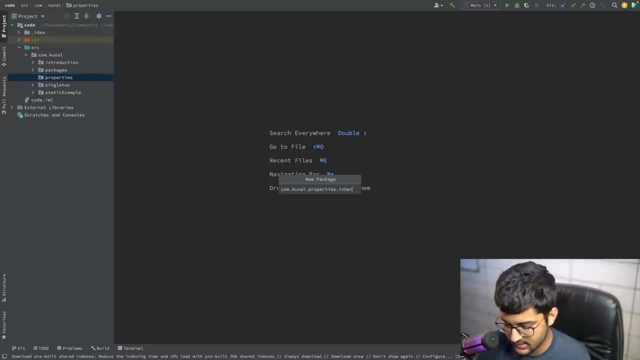 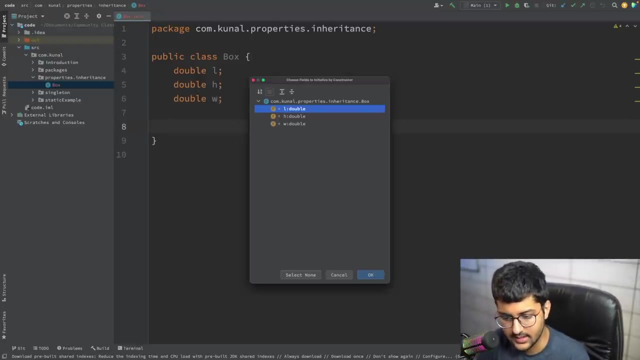 base class. so I'm teaching you inheritance, inheritance and in that I'll just create a class called box. okay, it's going to have some properties, no problem. so let's say, I put a property called double length, double height and double width. okay, something like that. I create a constructor. I let's say, 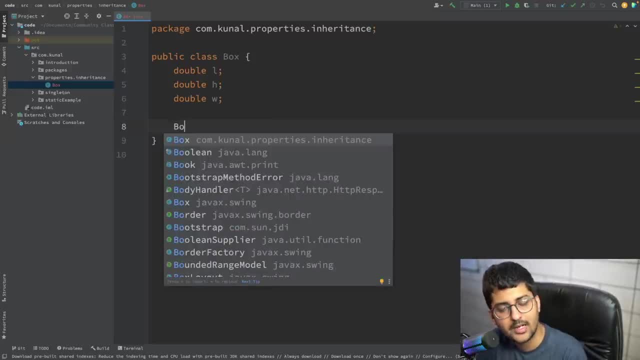 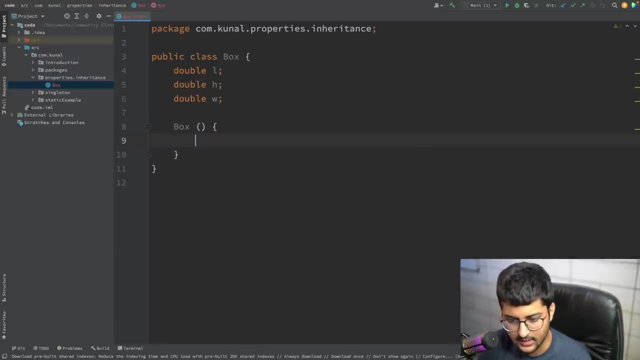 just create a normal constructor like: uh, we already talked about multiple constructors, right? one constructor like this, so initial constructor. I can just say that, um, this dot height is equal to initially. let's say this: this dot length is also minus 1 and this dot width is also minus 1.. that. 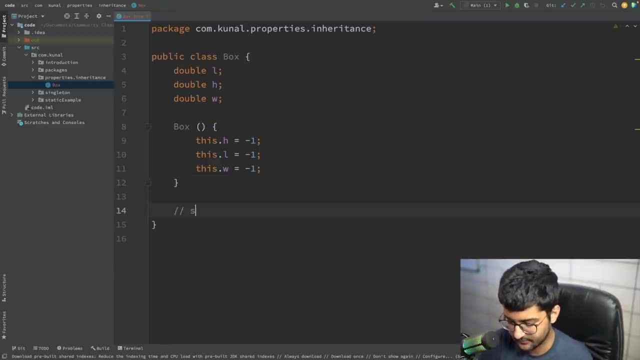 is one way we can create a constructor. let's say you want to create a square, okay, so if you want to create a square, then or cube, so you're not a square, a cube. if you want to create a cube, then someone will call this constructor. and how these constructors and things get called, like I'll. 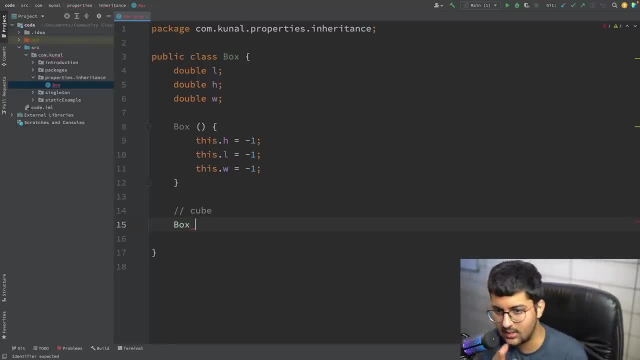 teach. I have already taught you right, I have already taught you this how this actually gets called, but um in over overloading and stuff. I'll actually teach you the internal implementation of this as well, obviously in this video only okay. so let's say, you just give it one side, so in. 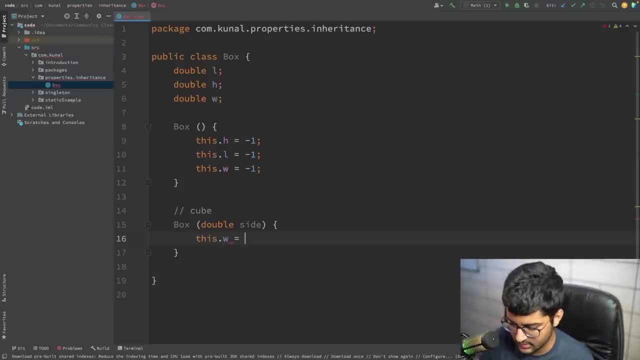 that case, all these three, this dot width is equal to side, this dot length is equal to side. like how these? i know how we know how we can like make multiple constructors right: if i pass one side, it will call this. if i pass nothing, it will cause. call this. if i pass some two, it will give. 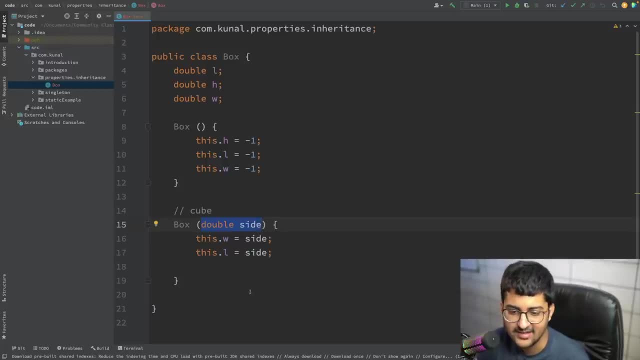 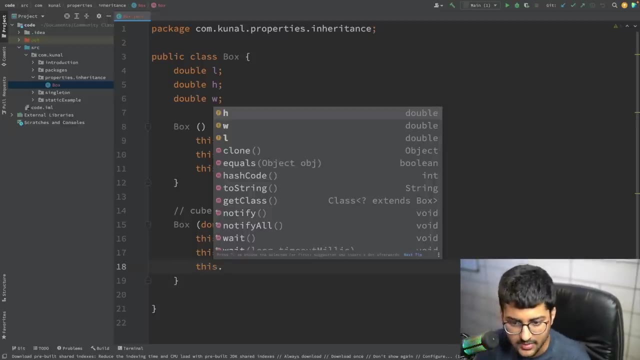 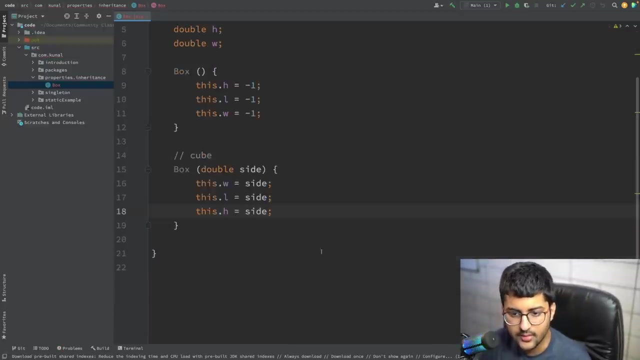 an error until unless a parameter two exists. so how that happens internally, i'll teach you right now. uh, when we do like polymorphism after inheritance, so bear with me. for a second, height is equal to also a site. now, this is a cube. okay, this is a cube one more we can make. 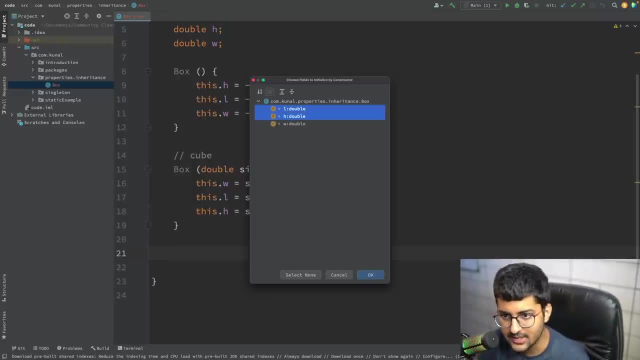 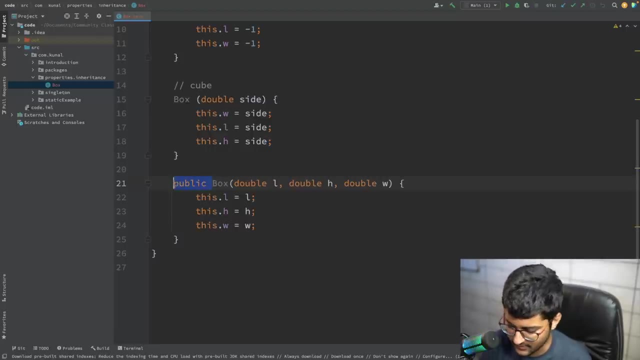 is normal, like if you pass three arguments, for example, if you pass three arguments, it will call this. okay, it will call this you. you may or may not write public, it's fine, we'll talk more about that in access modifier. okay, um, i don't have to print something like that. all right, that looks. 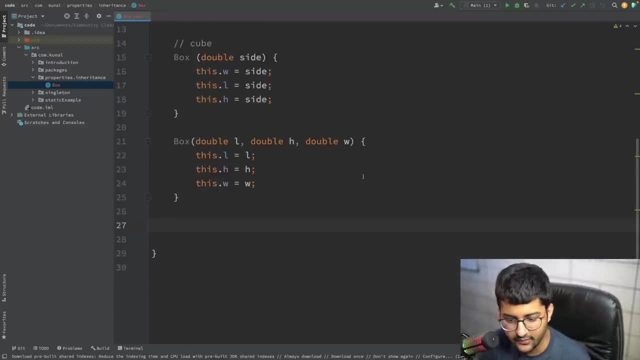 good. and one more thing can happen is if you pass a box in it. if you pass a box in it, so copy constructor. we talked about this previously. if you pass an old box or something, so you can say this dot height is equal to, or dot height. 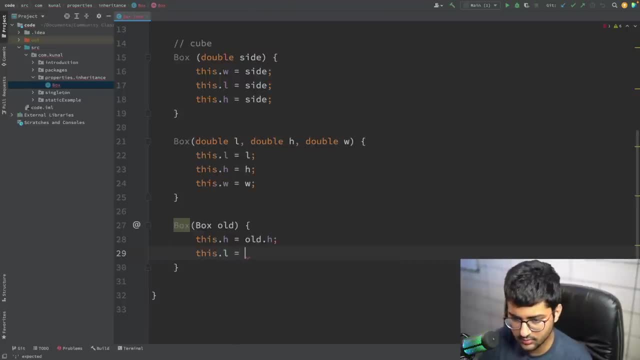 this dot length is equal to or dot length. this dot width is equal to or dot width. that's it. i can create some functions like this. i can say public, not protected, public, just void. i can say display info. or i can just say in for information like this, and i can say print: 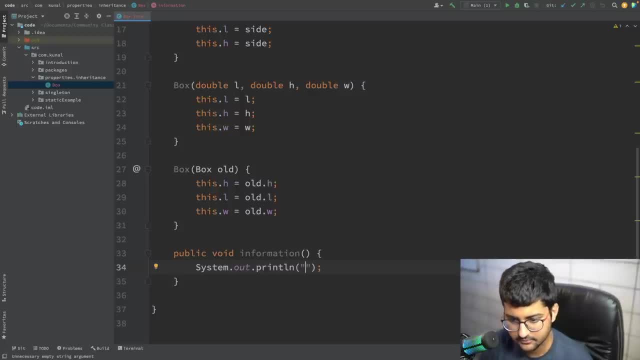 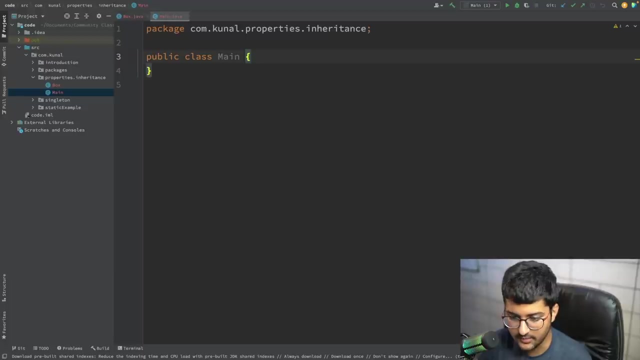 something like this: um, i can say running the box or something, okay, doesn't really matter that much, cool, so that's it normal box. i can create a main function for this. okay, uh, not me, not main function, main class. so here i can just say public static void, main. i can say box. 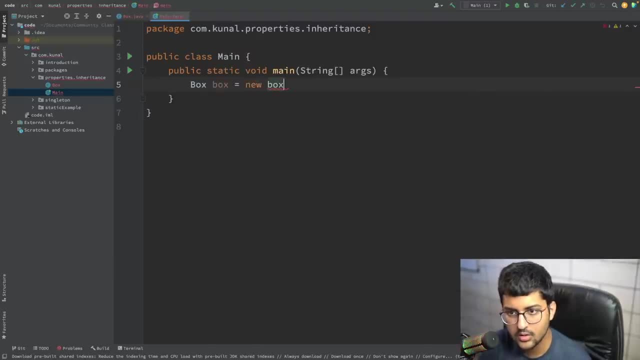 box is equal to new box, something like this. and if i just try to print box dot length, box dot width, box dot height, so it will be like, okay, which constructor is there? that takes no argument. it will be like, uh, this one. so it will just set it to. 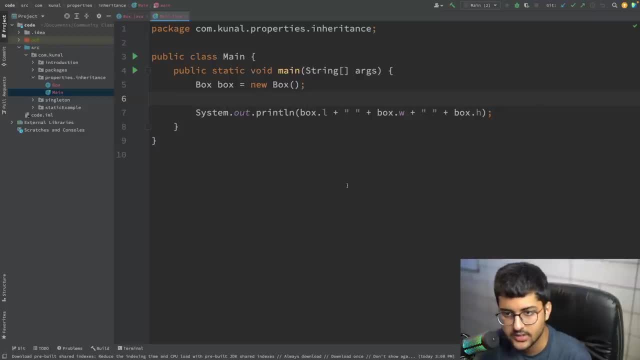 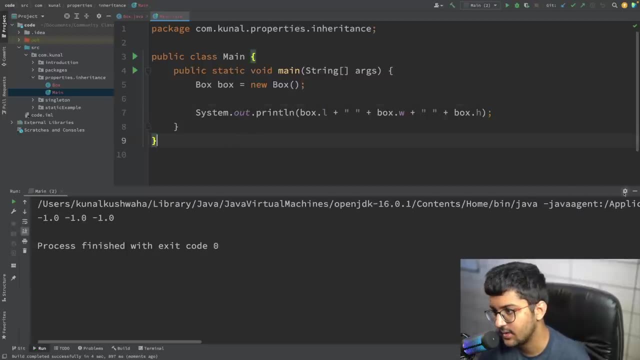 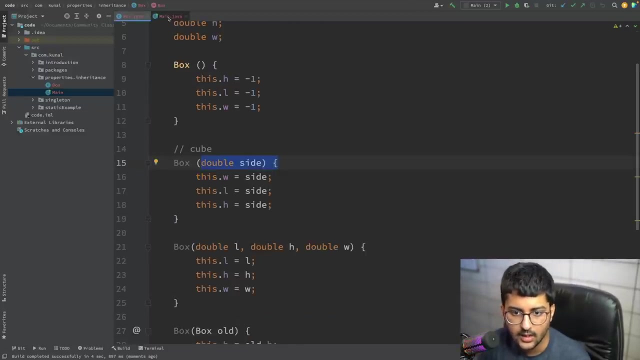 minus one, no problem, we have done this in previous lectures. nothing new over here. okay, everything is minus one. if you try to pass something here like four, we like: which box is there that takes only one argument. it will be like, uh, the this one, this one takes only one argument and we're like, okay, run it. 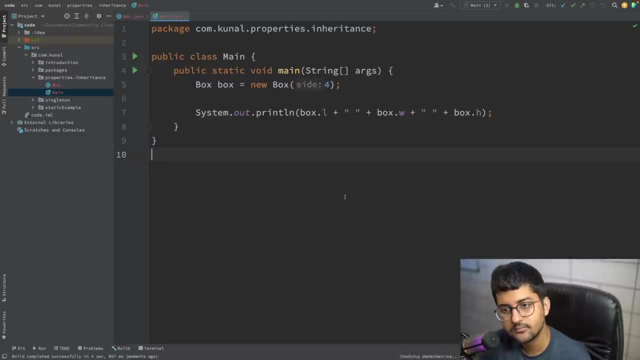 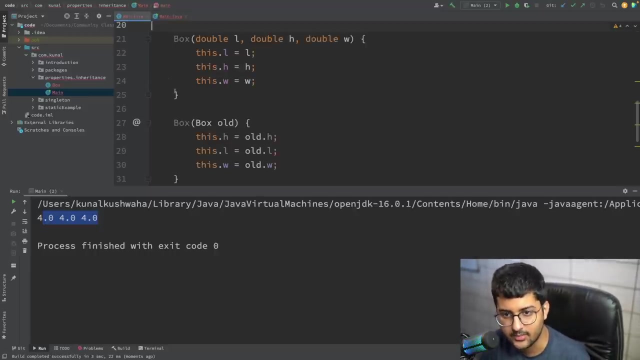 okay, square, oh sorry, cube, cube. that's right which one takes three arguments. but what if we try to put like 4.6, like two arguments, let's say 7.9? which constructor is there that takes two arguments? uh, no constructor is there, hence it's giving error. okay, which constructor is there that takes? 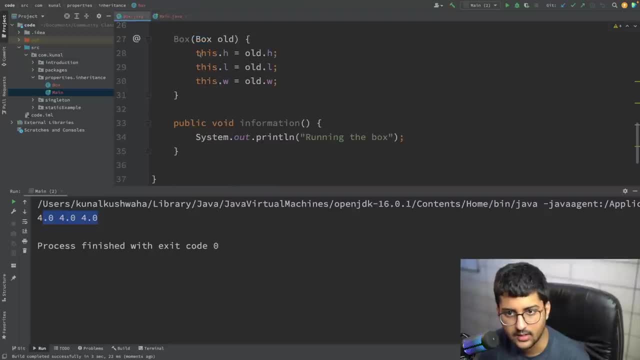 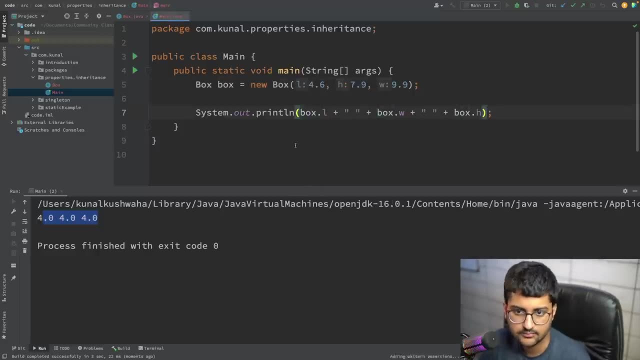 nine, uh, three arguments. it's going to be like: uh, this one takes three arguments. okay, let's call this. so. it's like setting the values like that. okay, box one. you can say, and if we say box two is equal to what new box? if i pass another box over here, another object of type box? 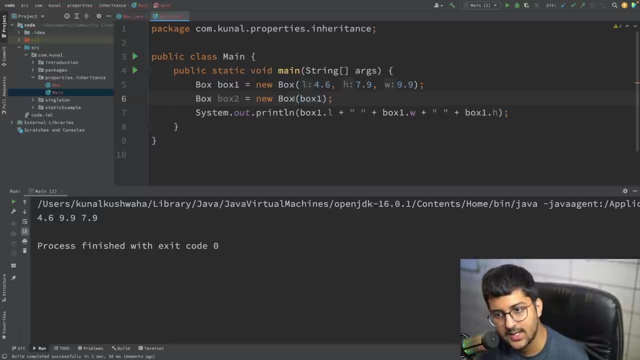 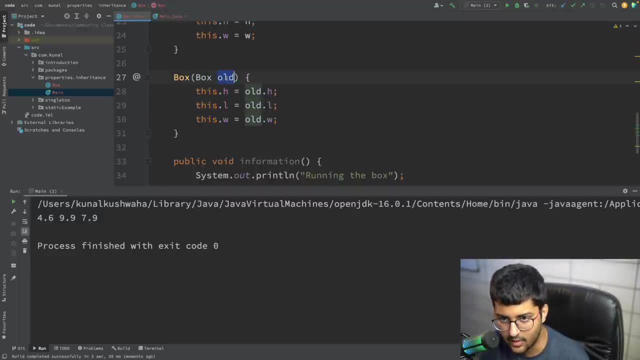 okay, that's going to be like: which constructor is there that takes another type of box? it's going to be like: yeah, there is an actually a constructor that takes a type of box. just copy the type of the past one into the new one. that's it same thing. that is what is. 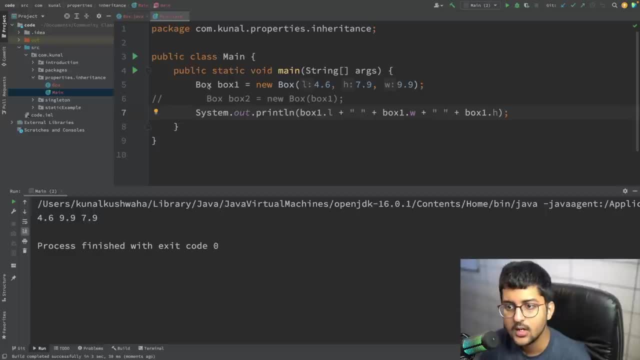 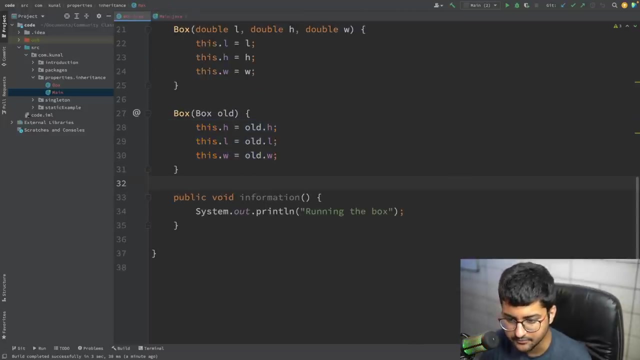 happening okay. so how this thing works internally, i'll tell you when we do like um, you know um what- when we do polymorphism, like right now. but let's first, uh, talk about the inheritance part, um how that thing works. so, in inheritance, what is happening over here is, let's say, so, we have this file, okay, we. 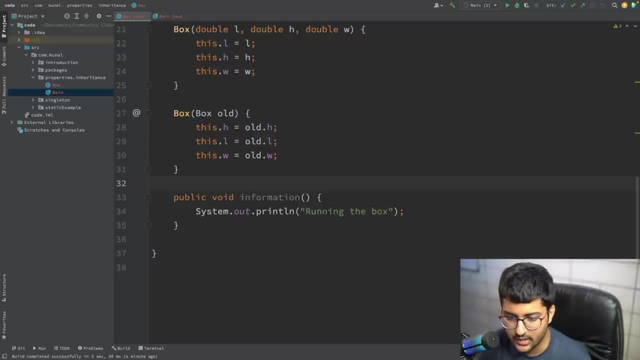 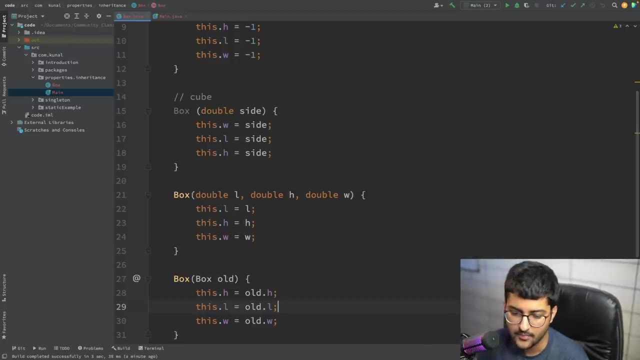 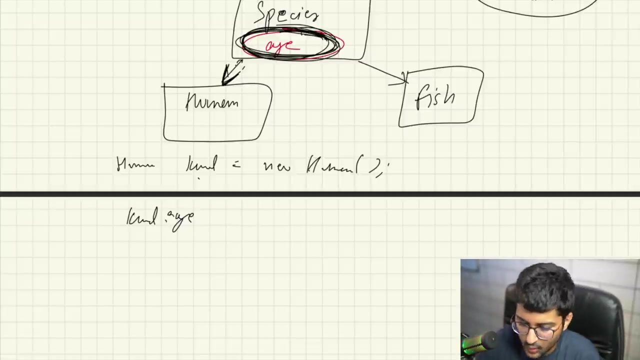 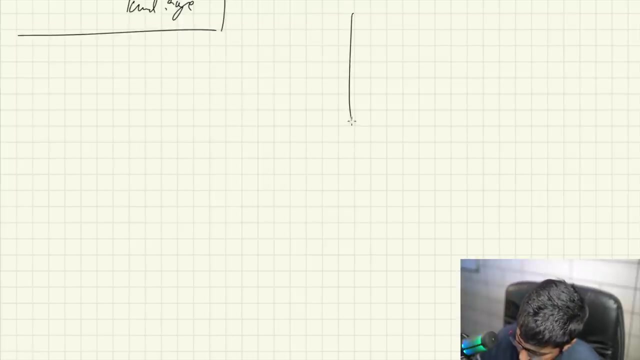 have this, uh, particular one. and now let's say, i try to create, um, i try to create a box weight. okay, so this is what we're trying to do. let me bring up my whiteboard. okay, so you have your box, something like this: this is what we're trying to do. you have a box like: 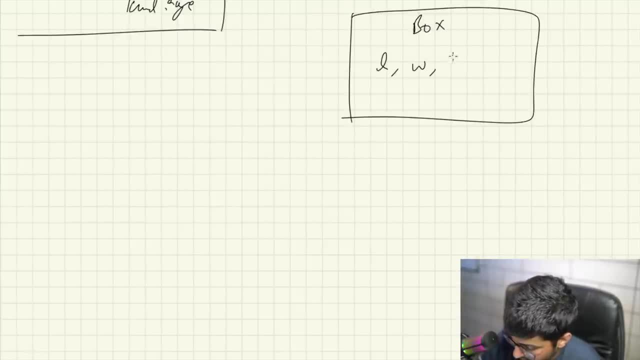 this. it has a length, width and height. you're trying to create another prop, another type of box that has a weight also. okay, so this is a box that has a weight also. now, this box is obviously going to have three properties as well: length, width and height. so, instead of creating again, 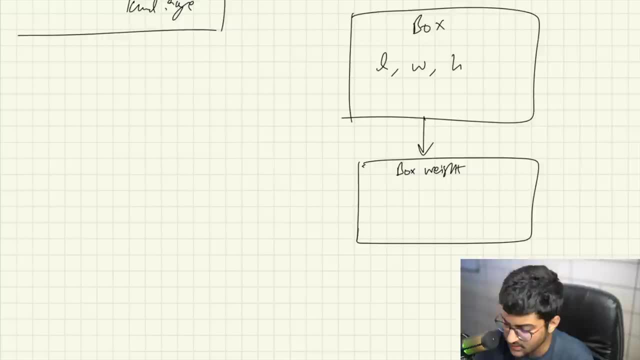 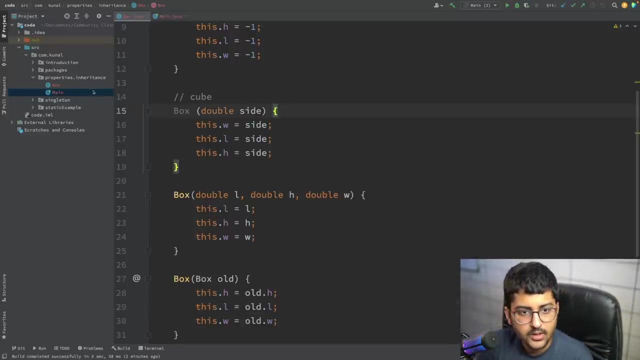 over here. i'm just going to say, i'm just going to inherit the property of length, width and height properties from the main parent, and this one is going to have weight in it. and how do we do that? via the extends keyword. let's see. so here i'm going to create a box of weight. 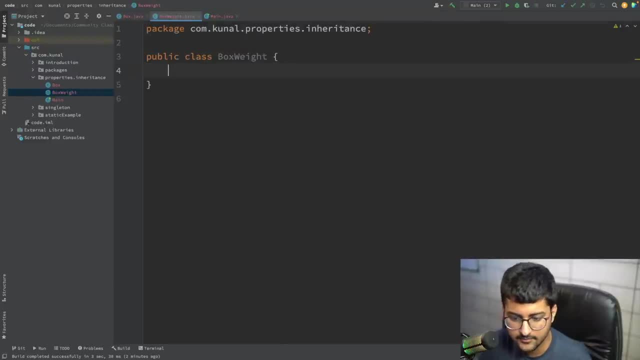 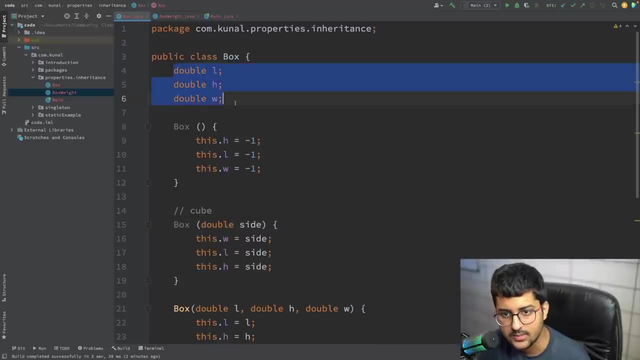 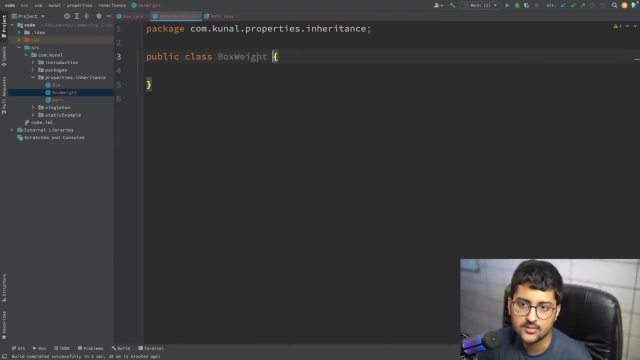 something like this: so this is a class box weight. it basically wants all the properties that are here in this box. class these properties, everything like this. okay, all of these information, everything it wants. how can we do that? extends box. that's it. extends box, that's it, it's going to have. 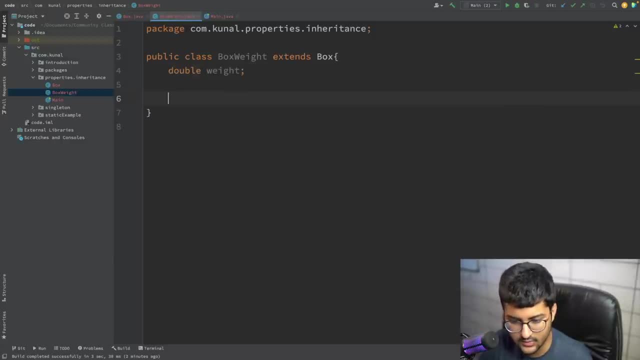 weight. now when i create a constructor, notice what will happen. i just create, let's say, a normal constructor like this. okay, i create a normal constructor and here i just say, let's say, this dot weight is equal to minus one. for example, now when i go into 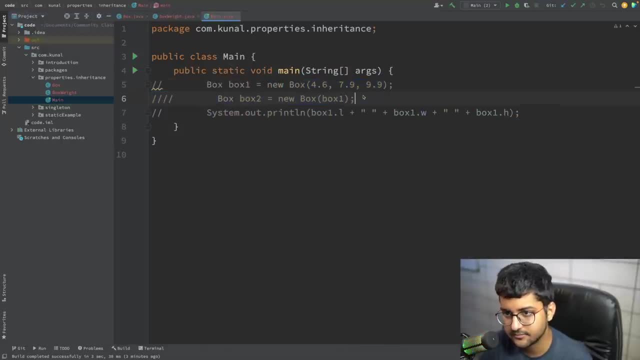 my main and i actually, let's say, create a box weight one, okay, i say box weight box three is equal to new box weight, okay, something like this. and then i say: box three, dot weight. print box three dot height. box three dot weight weight, not width. wait, let's see what it will print for height. 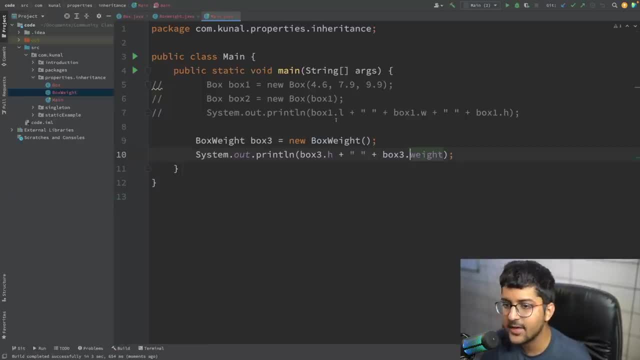 so it's saying minus one and minus one. what is happening over here internally? let's see what if i try to make another box weight. so, for example, i do something like this. let's say you say something like you want to use the properties of this class, right? so you? 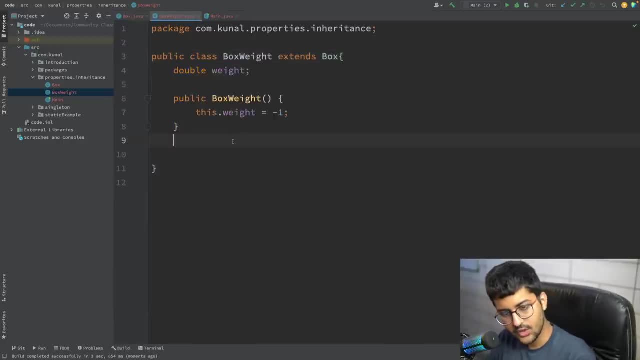 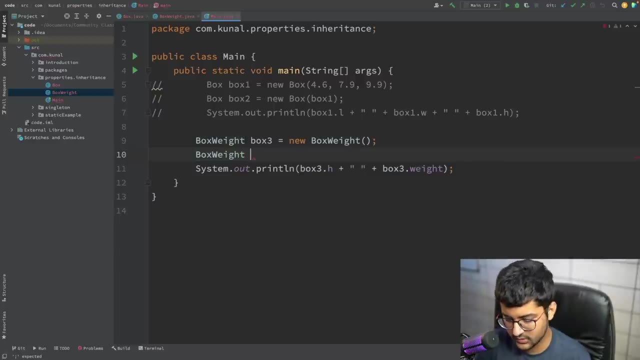 want to use these things, so you should be able to use those in the constructors as well. so what we want is something like this. we want to create it. something like this: box weight box for new box weight, length, width, height, weight. you want to do it something like this. you want to pass all these. 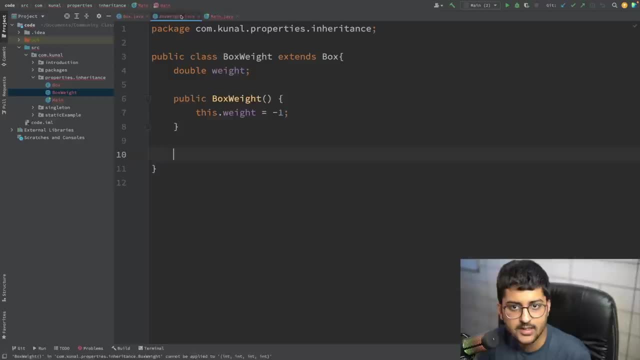 four things. so i know the first three things are actually being used in its parent class. it will. it will get it from here, but how is it going to use it inside the constructor? what happened in this case was that you are giving minus one and minus one for this, because this is how it works. 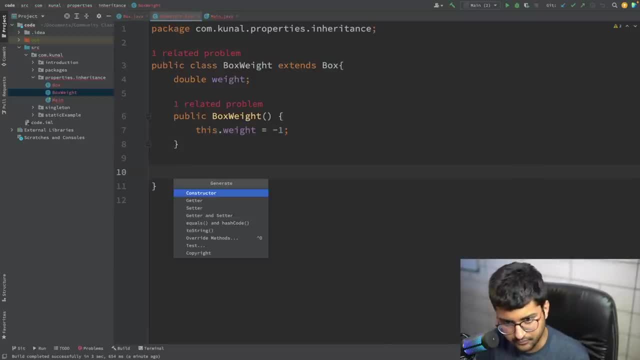 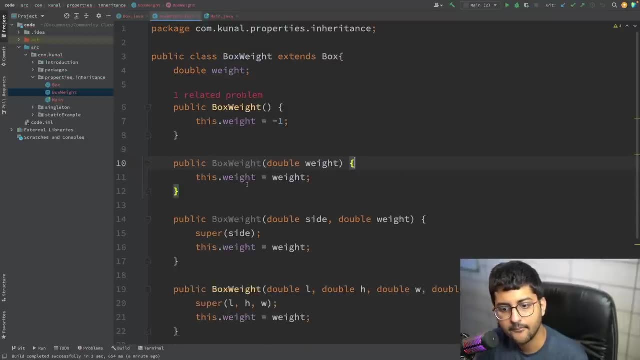 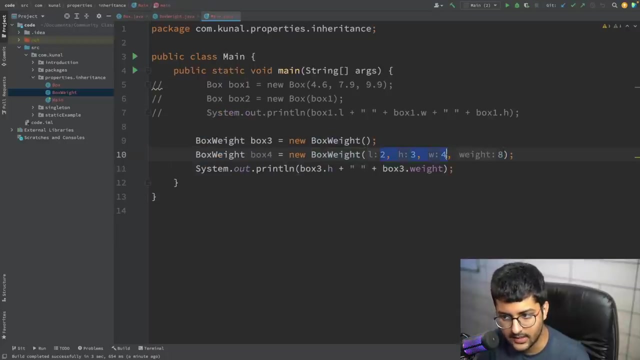 let me show you. so, constructor, all of these things i want, let's say like this- oops, sorry, constructor, like this, like this, so this is what i want. okay, this is what i want, this is what we're getting over here, okay. so we said that, uh, pass the length, width and height. 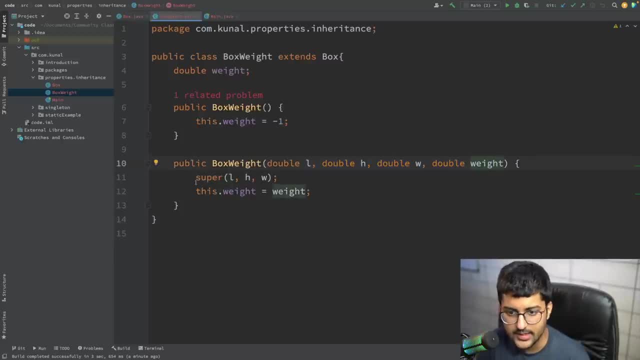 and also the weight. so it's passing the length, width and height and also the weight it's setting normally. but what is this thing? what is this? so this is what is happening: in order to set length, height and width, it obviously has to set it over here in the box, but it has to get these values from the parent class, because these 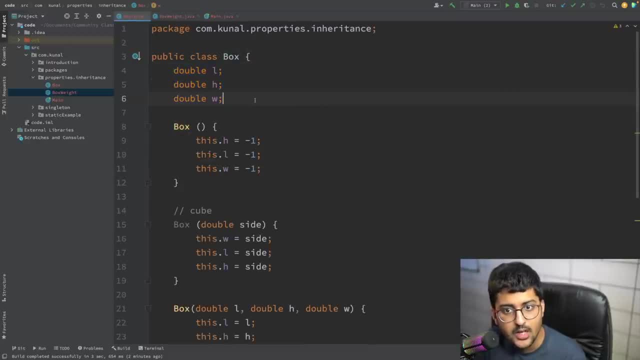 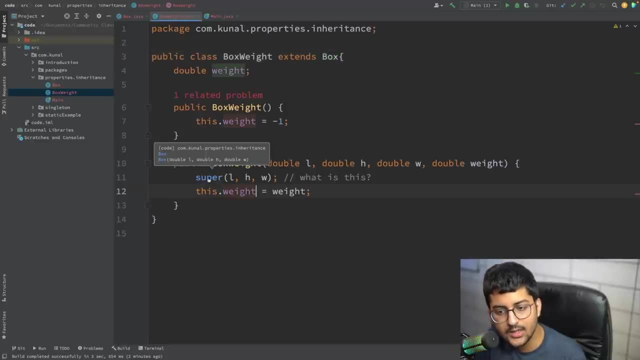 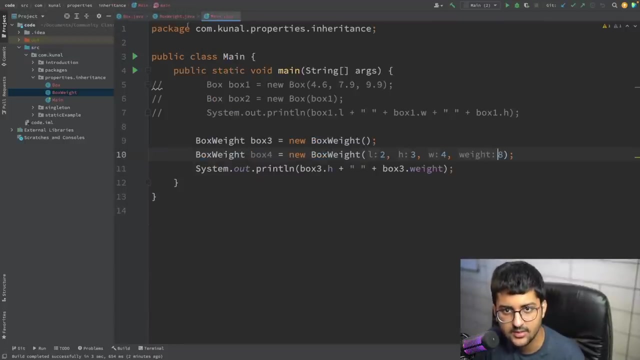 value exists over there, so it has to initialize these values. and where are these values getting initialized here? so it's basically saying: call the parent class constructor. that's it. it's saying call the parent class constructor. so if you double click on this or not, double click control, click on this, you will see it's actually calling this one. 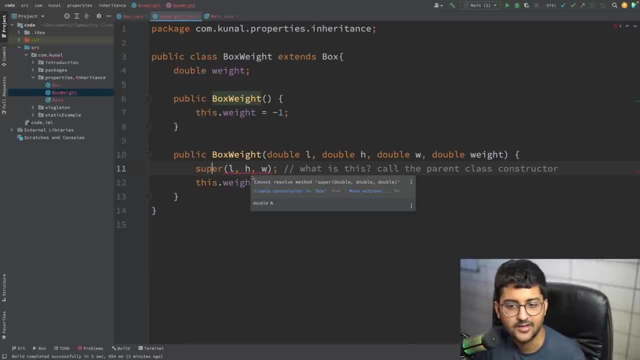 what if i hide it? then it's giving an error. it does not exist, okay. so when you want to call, when you want to initialize- so i'll just write it over there- use to initialize values present in parent class. so this is actually calling the parent class constructor. 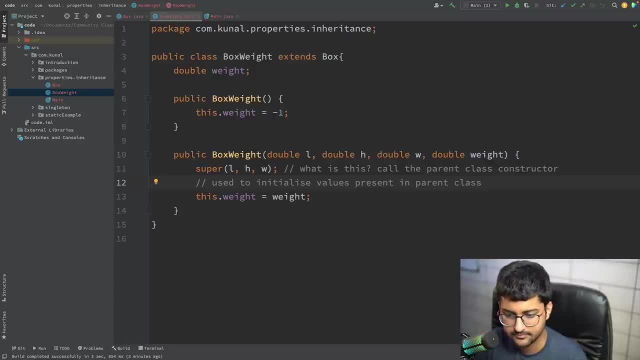 okay, that is what it's doing. okay, and although the subclass includes all the members of its subclass, okay, and although the subclass includes all the members of its- like- parent class, or super class that we like to call it, it will not be able to access those members of the parent class that have been declared as private, okay, so if you do it like this, 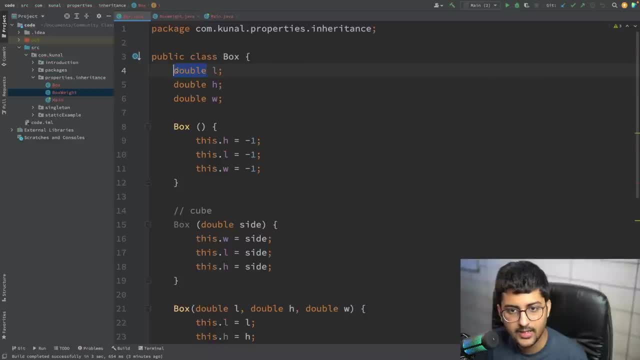 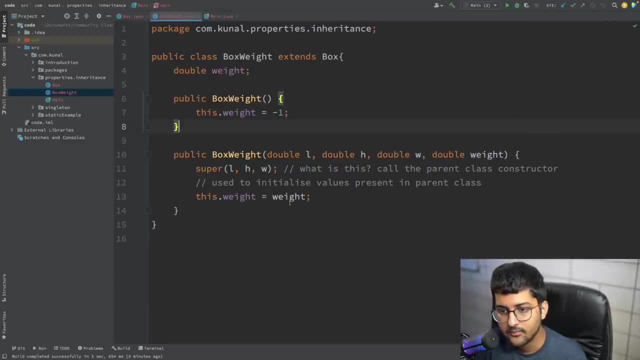 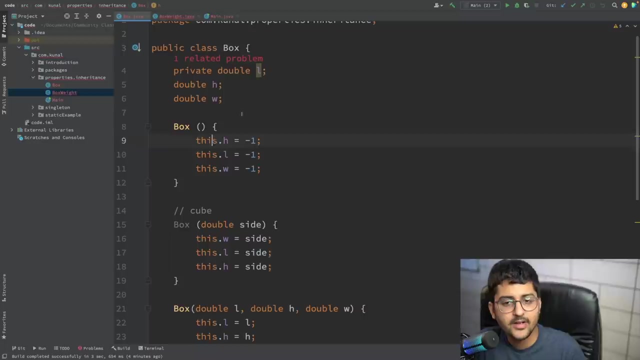 private l sorry private double l, something like this. okay, and here, if you want to do it like uh, somewhat like this, you can say: this dot w is fine, but this dot? l you cannot access because it's private. private is very simple, even though i will cover it in access modifiers, but right now i'm telling you: 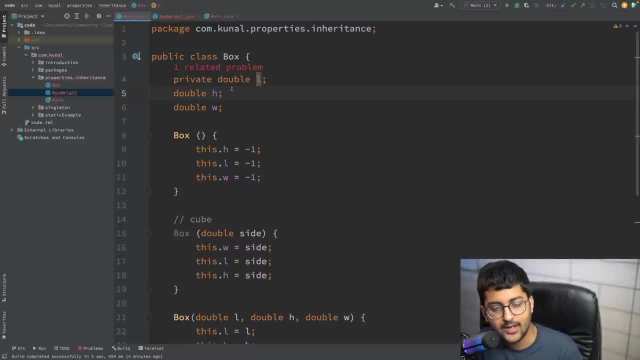 why am i telling you? you're saying, kunal, you will cover it in access modifiers. we don't want to miss anything. why are you telling it right now? you will not understand. no only reason why i'm telling you: it's because it's very simple: anything that is private, you can only use it in that file. 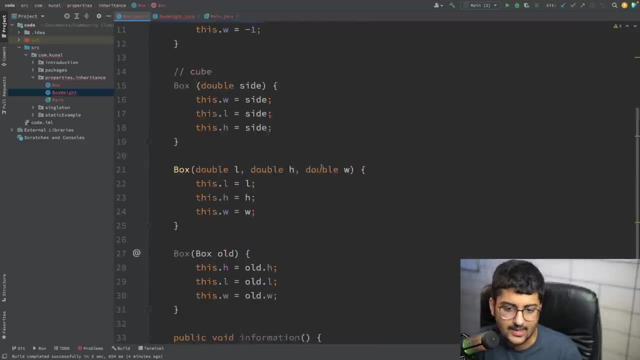 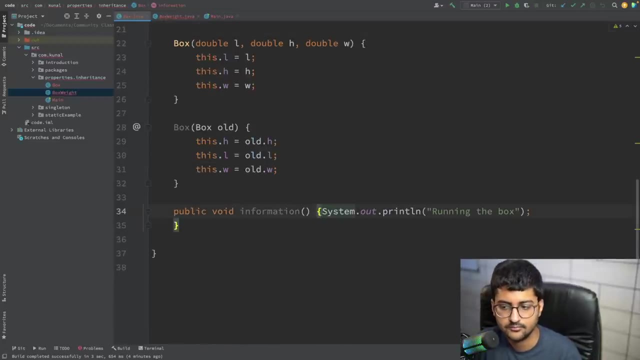 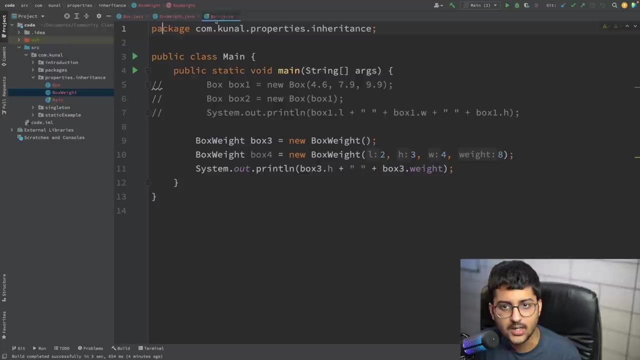 you can do whatever you want with l over here. you can access it, set it like this, you know, print it or whatever you want to do, you can do, but only in this file, only in this file. you cannot use it outside like this. another question: can i use it over here? 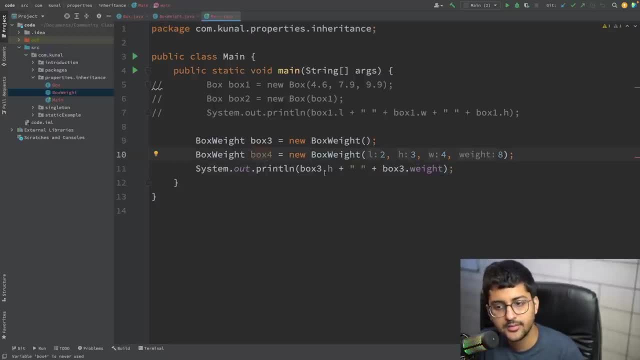 box4.l. don't even have to try it. you can't use it, you can't. it's private, private, can't okay. so this is another important point. i will mention it in my notes. although a subclass includes, like, the members of its super class, it will not be able to access the ones that 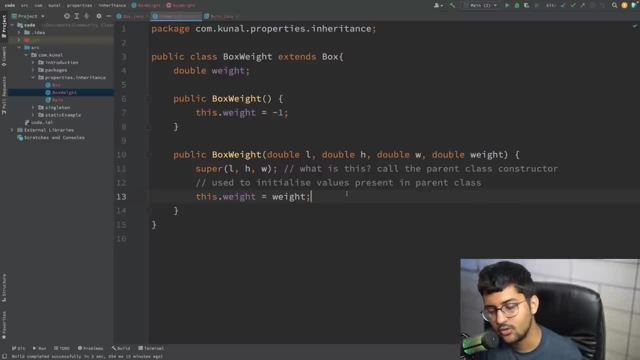 are private. okay, you now. you might be wondering then, how is it initializing this l over here if it's private? because this class is not initializing it. this box class is initializing it. see box class. constructor is being called. okay, sound good, cool. now one more thing i want to mention to you is, please, every single word. 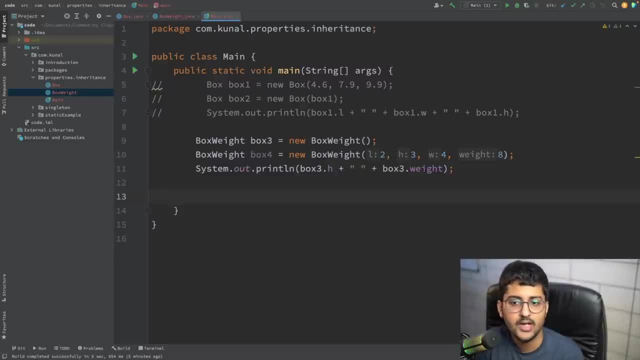 every single line that i'm mentioning in this video right is very important. every single line itself contains what concepts. that is why please listen very carefully. i have devised it very nicely- the entire path for this playlist, okay. another question can be: kunal, you made this box playlist for me, or you made this box playlist for me, or you made this box playlist for me? 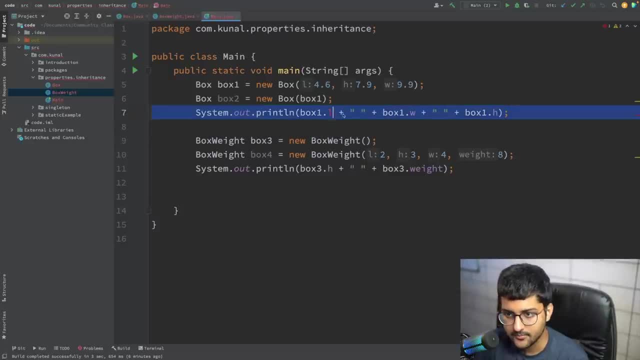 like this: okay, no problem, you made it something like this, okay, uh, let me just hide this thing right now. you're gonna be like: hey, kunal, you made it like this, okay, so you made a box of type box. this is an object of type box, no problem. can you access the elements that are in the child class? 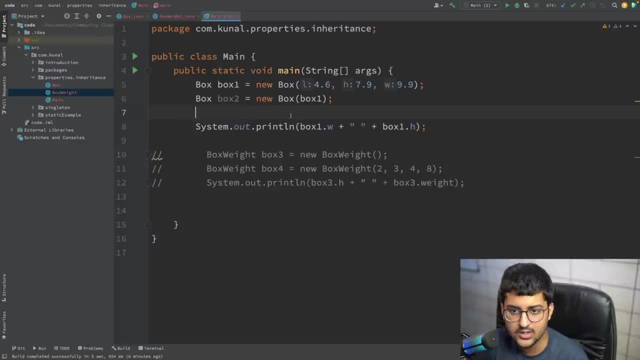 for this? for obvious reasons, you can't. logical, logical reason: okay, if you try to access the weight, it will be like weight does not exist. so you can only access extra variables that are above until, unless they are not private. okay, so child can access extra variables that are in the parent, but if the object is directly created of parent class. 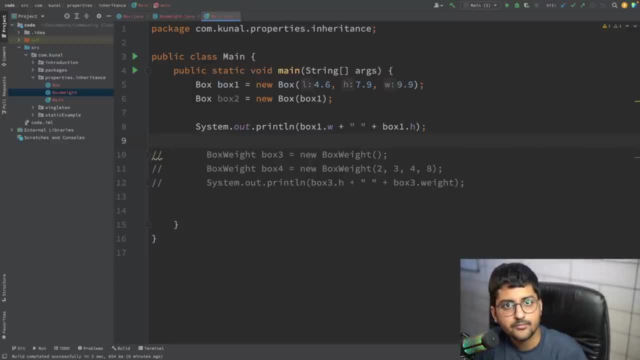 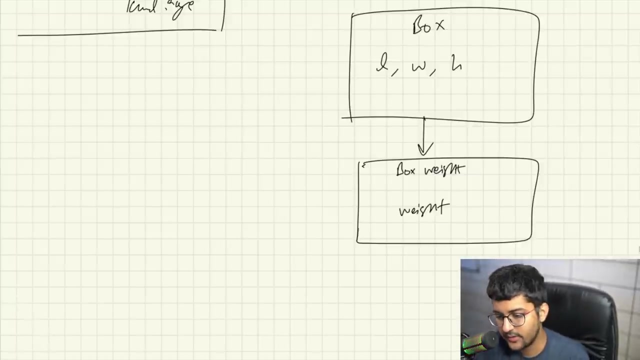 it will not be able to access the child properties. okay, obvious reason: sound good, cool, that is basically about it. okay, so, yeah, cool, let's move forward here. for example: right, so if you create an object of this class, so these are just classes, right? the only difference is this is a child class, is a parent class, the 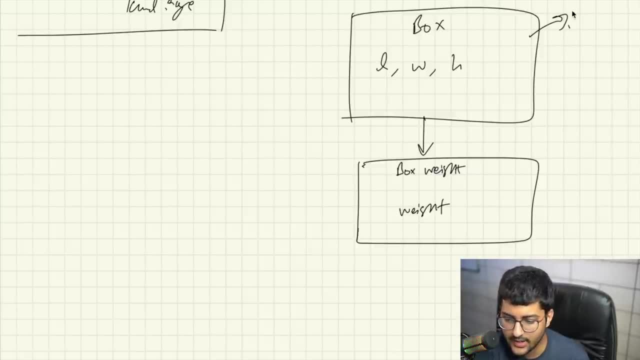 only difference is: child class can access the properties of parent class, but if you create an object of this class itself, it will not be able to access the properties of all the classes that lie below it. okay, let me show you one more cool thing. so this thing about 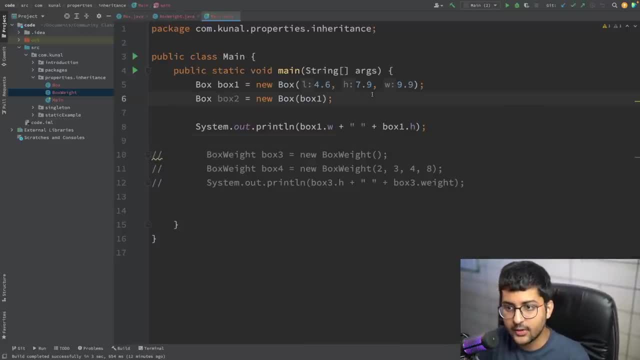 the. this is a very, very, very important concept. please listen to it very carefully. so this thing about um, the box type object not being able to use the child class parameters, or whatever, it's fine, but how? why? how is it working internally and what is actually determining this? 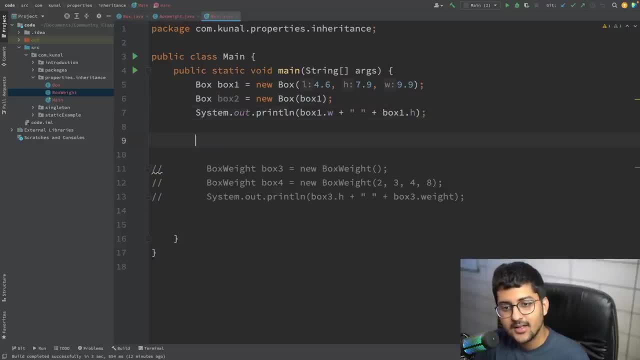 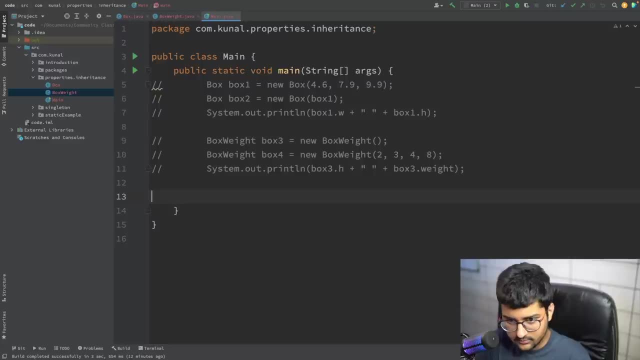 let's do something funny. let's make a box type object. the type will be boxed. the ref reference type is going to be box, no problem. by the way, I'll put it in my notes also. don't don't note anything. box type, box 5: no problem, this is a reference type of type box. 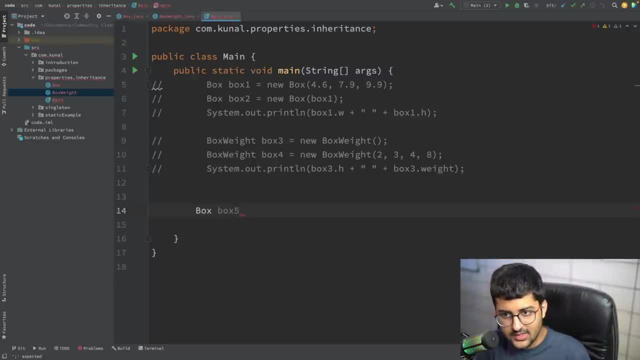 okay, no problem. but the weird thing we'll do now is we'll actually create the object of type box weight. okay, I'll copy this: two, three, two, three, four, eight, no problem. this object type is what? obviously this type is box weight, but it's referencing to something. 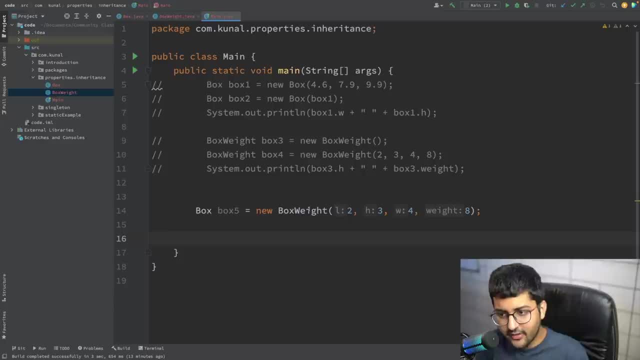 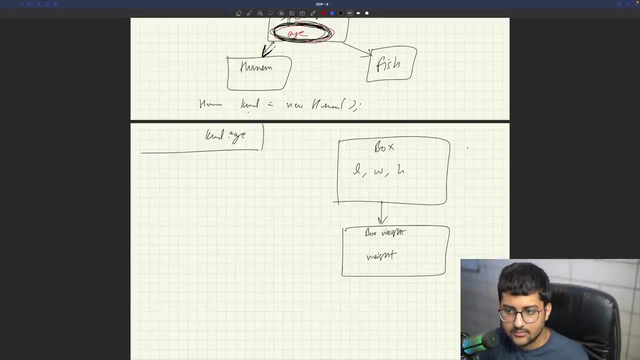 of type box it's parent. now, if I try to print, let's say if I try to access, let's say, box 5. But stuff that is in the, stuff that is in the, let's say, over here, for example, let me just put up my whiteboard- stuff that is in the box- weight class okay, or box class, let's. 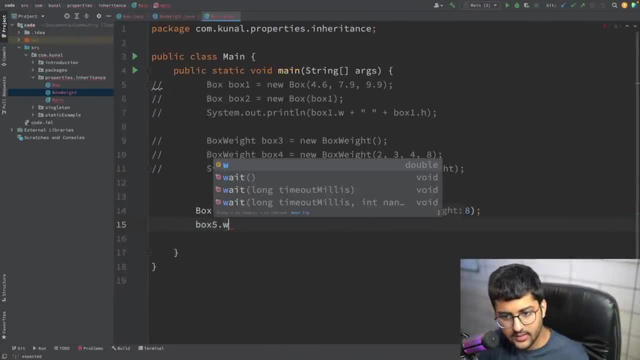 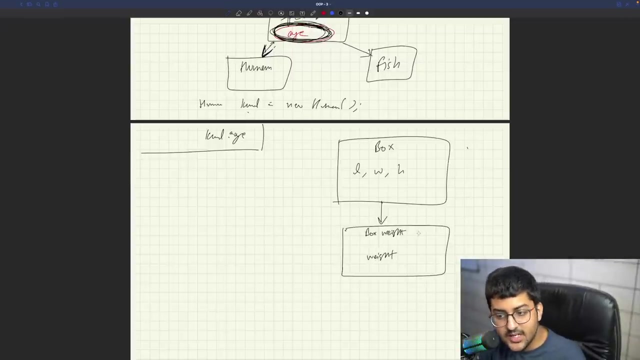 say width or height or whatever, box 5.width: yeah, it's able to access that, no problem. no problem at all. okay, so you can print box 5.width, no problem at all. But can I print it? Can it access box weight parameters? the object is of type box weight, okay, no problem in that. 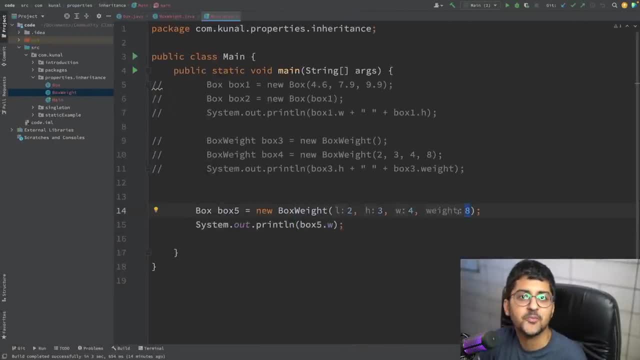 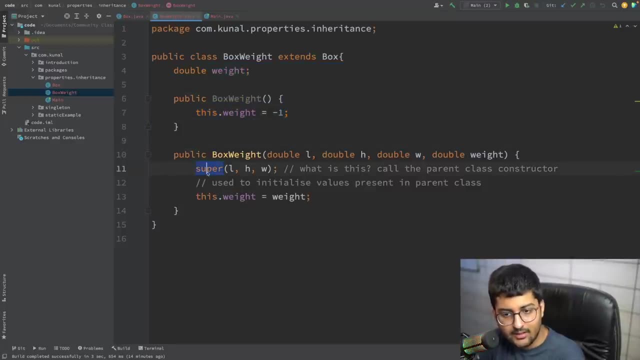 weight is also initialized also. weight is initialized also and I'll tell you in detail about the super keyword. okay, you may be having any doubts about the super thing. I'll tell you in detail after this about that. okay, but first focus on this. it is initialized also. 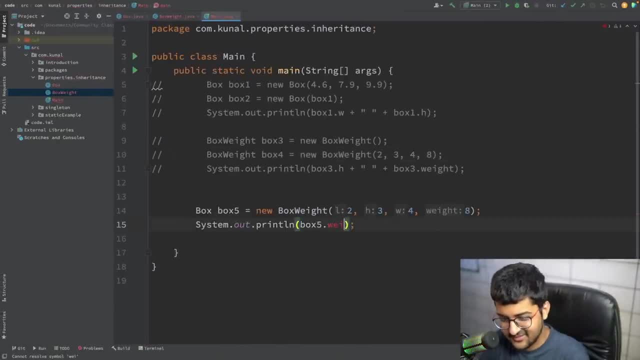 but can you access it? let's try to do it. no, not able to access it. what is happening? This is what is happening. it is important to understand that it is actually the type of the reference variable that actually determines, and not the object. it is actually the type. 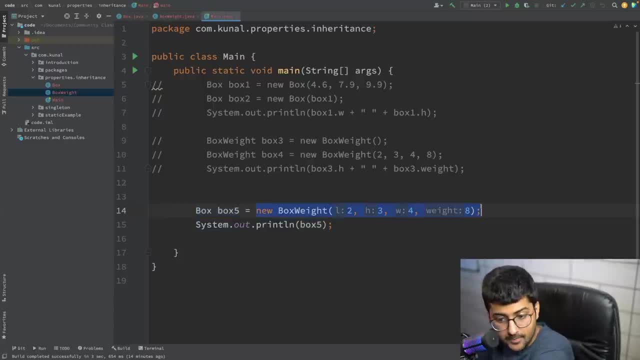 of the reference variable and not the type of the object that determines what members can be accessed. This is what happens. Okay, This is a type of reference. this is a reference type of box and it is referencing to an object of type box weight. 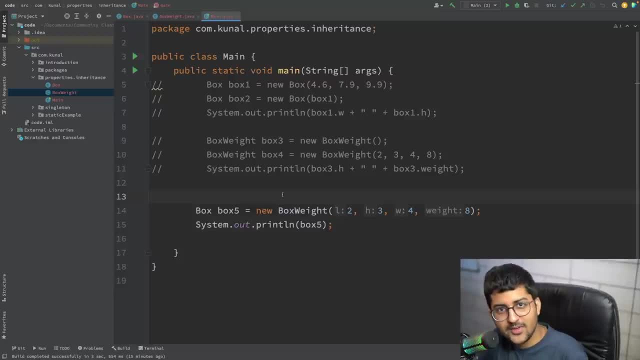 Sometimes the parent refer to you as well. right, so you are at, like you know when your parents are at parents teacher meeting, so your parent class is going to. when someone asks you who are you, the parents are going to be like: I am the father of Kunal, so parent. 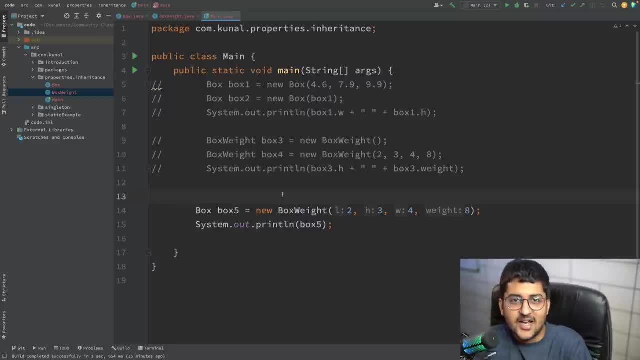 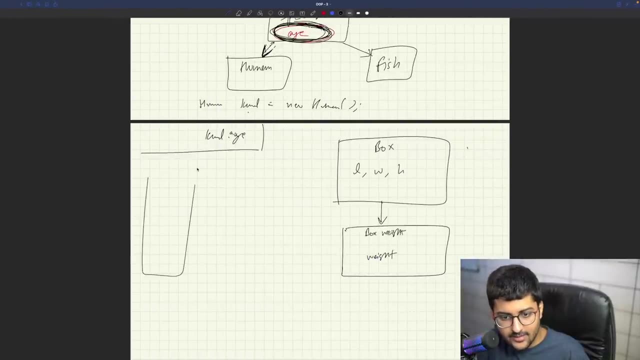 is referencing you. Parent class is referencing to child sex. so that is what is happening. this obviously is a reference variable, so it will be somewhere over here in the stack memory box 5 in the heap memory there is going to be an object of type box weight and this is going to be: 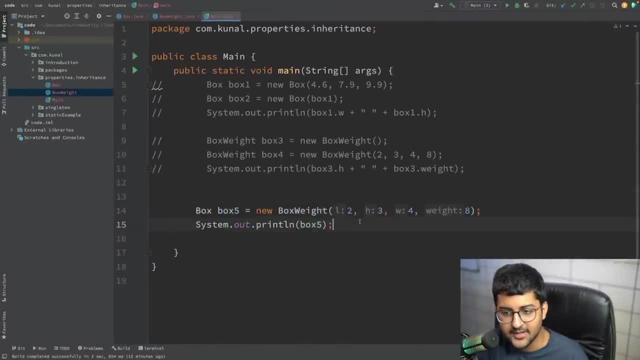 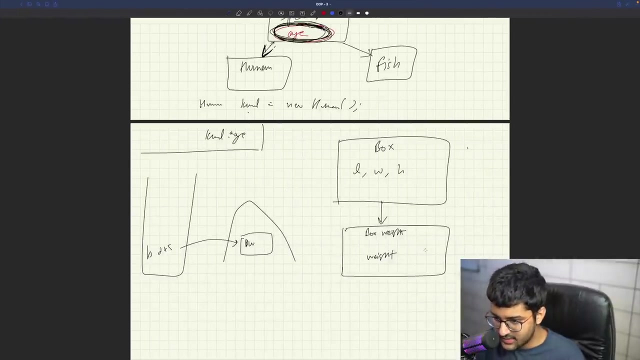 pointing to this. that is what is happening over here. so all the members that are over here in this box type- Okay, They will be able to access that. that you can access by this, similarly box weight, as have all the members. box weight has the members of itself plus of the parent class that are: 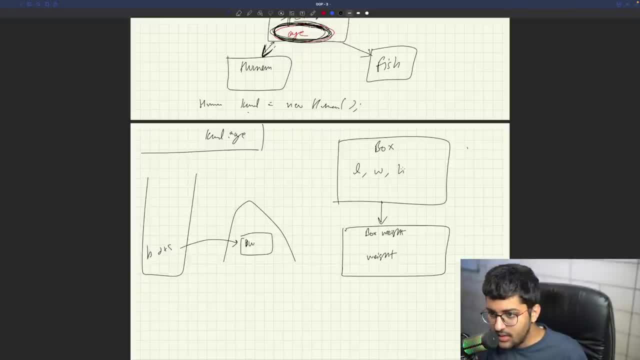 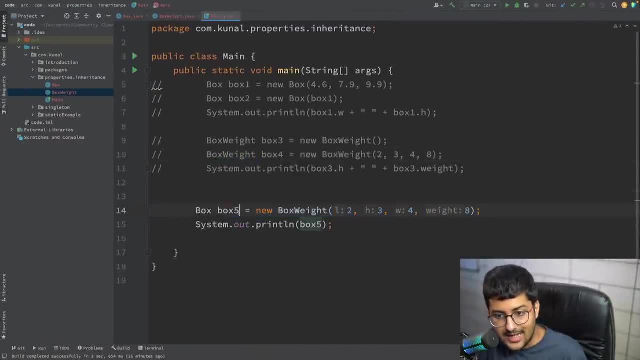 not private. hence it can access weight, W and height. so it's not actually the type of the object that determines what members can be accessed. it is a type of the reference variable. Okay, so when a reference to a subclass object is assigned to a super class reference variable, 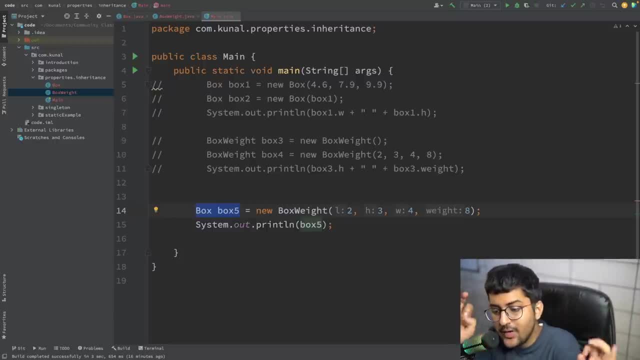 Okay, Like in this example, you will only have access to only those parts of the objects that are obviously defined in the super class, which is this. that's it. that is it? as simple as that? no problem at all. now you may ask something like Kunal: what about this? what if you want? 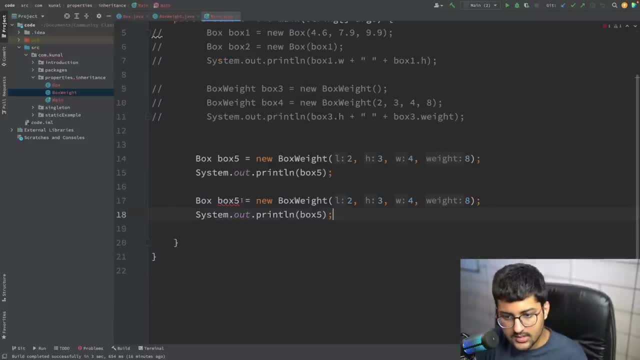 to do it opposite, like this. let's say box 6. Okay, You make it of type box, the reference type of box, weight and this of type box, and you only pass, let's say, three stuff over here. now it's giving an error, now it's giving an. 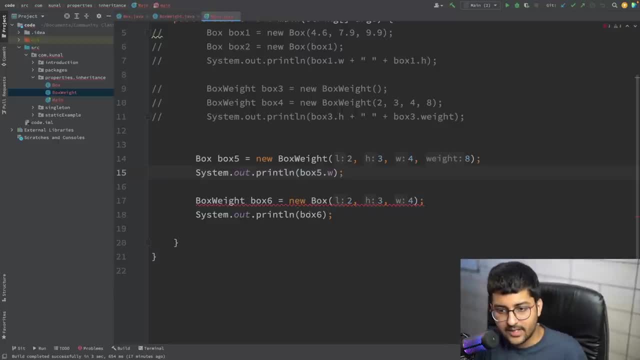 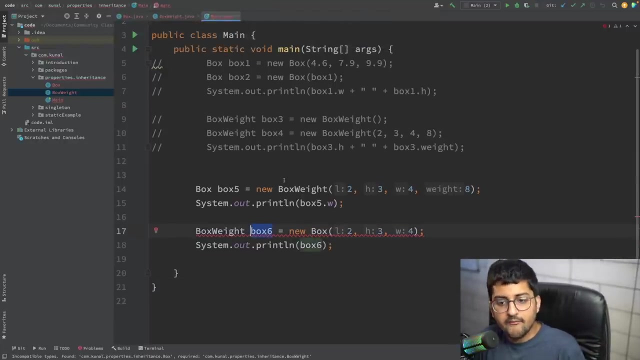 error. can anyone tell why it's giving an error? think about it. you are trying to reference a child to a parent child. you are trying to reference a child to a parent- okay, no problem. when you are trying to reference a parent to a child, when you're trying to reference 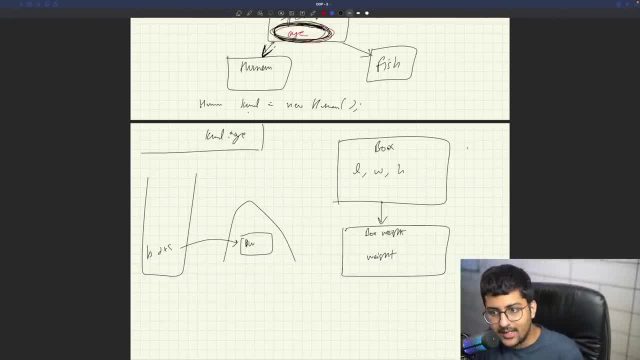 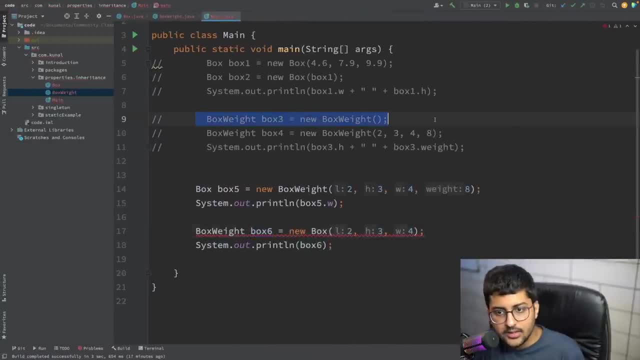 a child object to a parent? one okay, something like that. in that case, you're just able to call like you access these things when you're referencing a child with a child, for example, this one in this case also, if you just try to get weight and you try to get width and 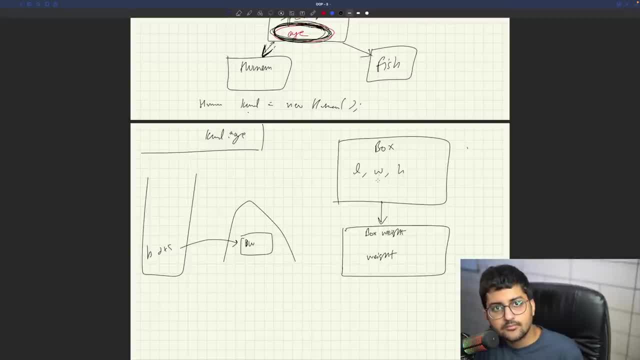 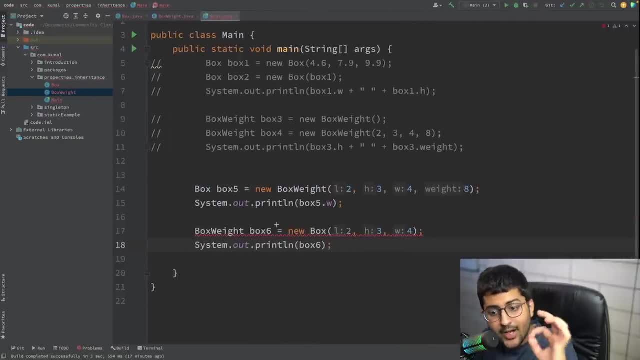 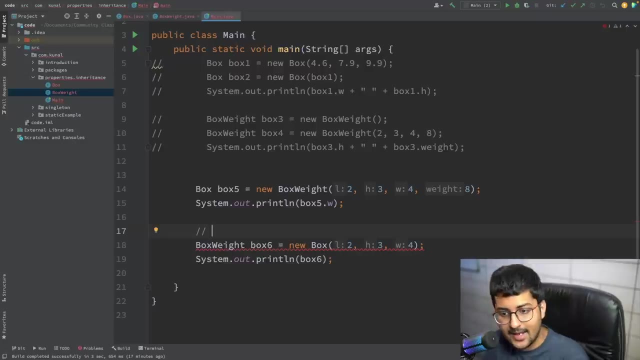 height, it will automatically call this constructor. okay, so problem arises when some values are not initialized. Okay. Okay, Let's try to think of these things. think in the logical sense. I will actually tell you how to think why this problem is arising. what are the problems that may arise? see what? 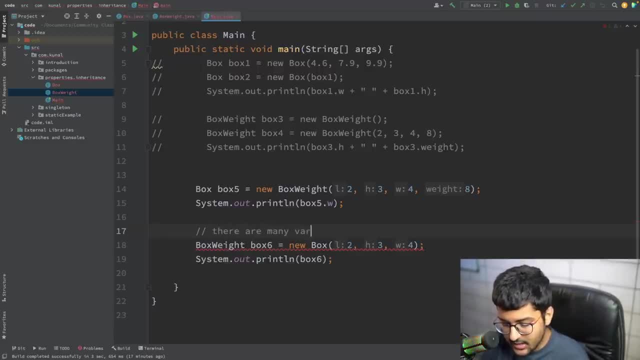 are we doing? we know in simple language, there are many variables in both parent and child classes. no problem, okay, no problem, you are given access to variables Dest Vai Dash and in the reference type, That is, in this example box with very, you should have access to weight variable. 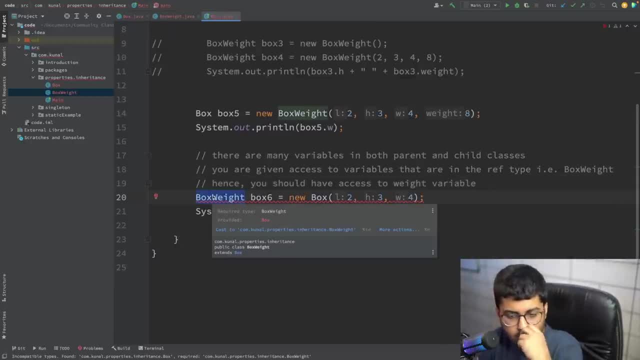 okay, this is everyone. Everyone knows that. okay, because blocks with available here in Kunal, you just said that whatever type is over here, All of this, do you mean this box, wait- is available over here and you just like whatever type is over here. This, the box, weight, and Kunal, you just said that, whatever type is over here, all of these other are access to weight variability thing, don't уng All of these, all of these things don'tales things, all plus certain things, that would be all of this, этих products, that would be present moment, very significant and important. 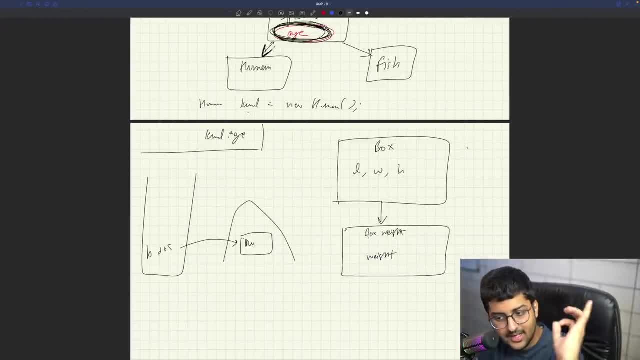 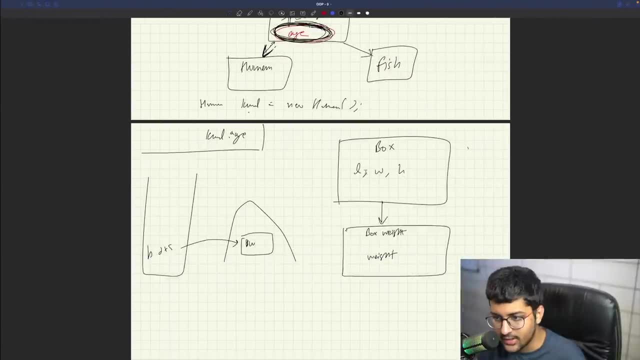 the variables and all methods or whatever that are available in that type. for example, this is a box width, so weight is available and this is available. hence you can access all those variables, so you can access- actually you can access- width, height and weight, because l is private, no problem. 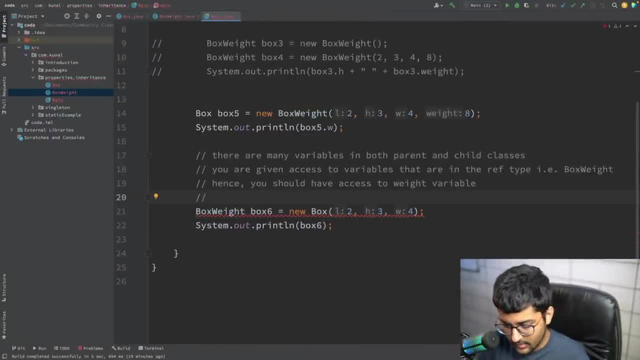 okay, so this also means that the ones you are trying to access should be initialized. no problem, so you're trying to access weight. hence, if you're, if you're able to access weight, if this is the rule, that is stating that, okay, you are able to access weight, no problem because box. 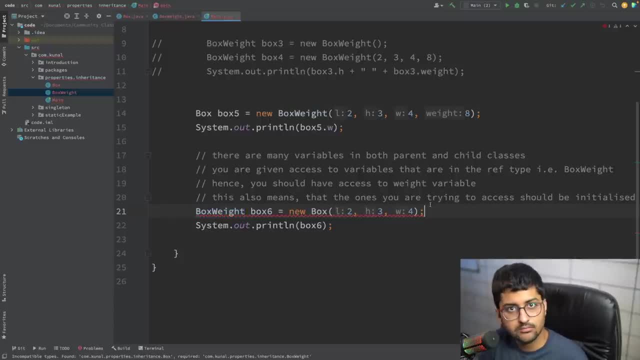 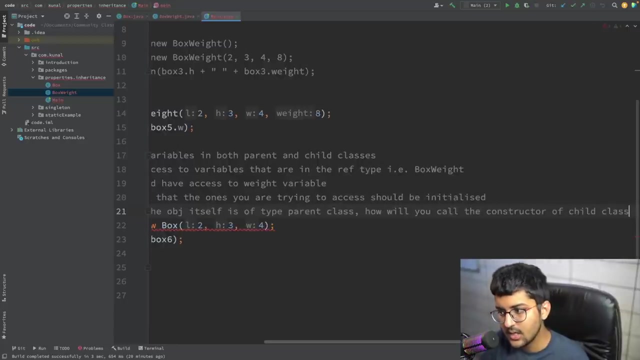 weight type is available over here, then you should be able to initialize that as well. you should be able to initialize that as well. but here, when the object itself is of type parent class, how will you call the constructor of child class? it's like: okay, kunal said that. um, if box weight is available, then i can access weight. okay, yeah, 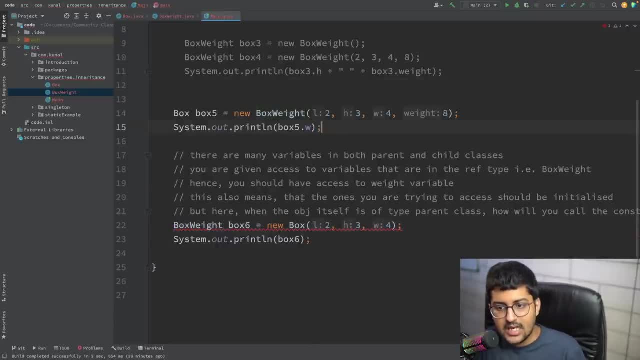 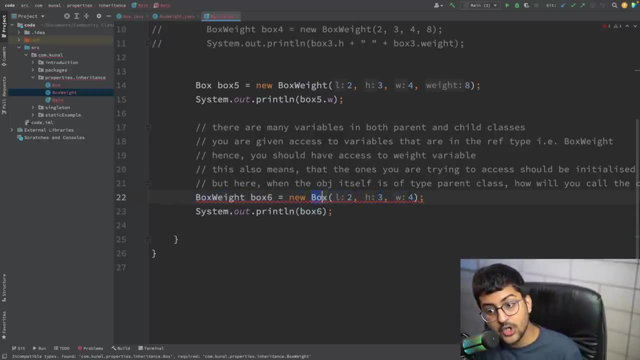 that is totally fine, you can. but now java tells us. java is saying: okay, you are able to access that, but you are not able to initialize the weight variable over here because you have called the constructor of parent class. parent class has no idea about weight. this has no idea about weight. 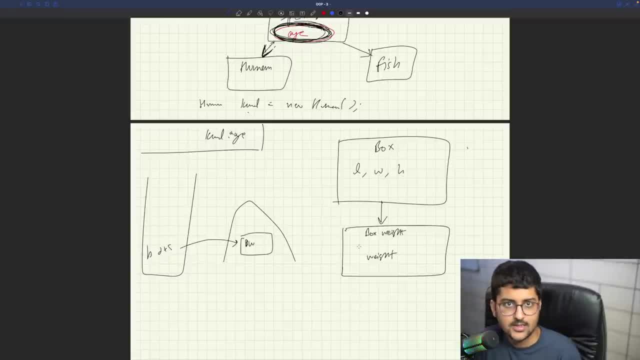 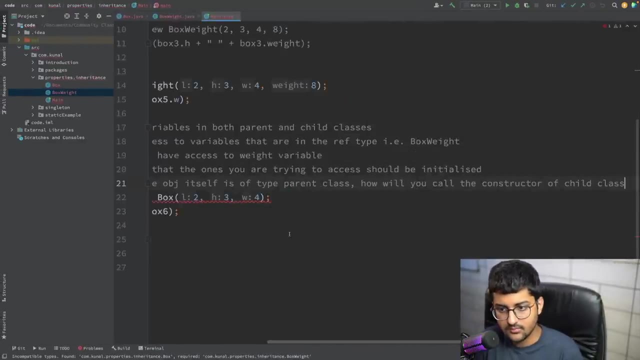 downward motion has no idea about the downward classes. this box class does not know what classes are below, but the below classes know what classes are above. hence you are not able to initialize this, because the object is of type this, hence it's giving an error. that is why error, hence it's not allowed. 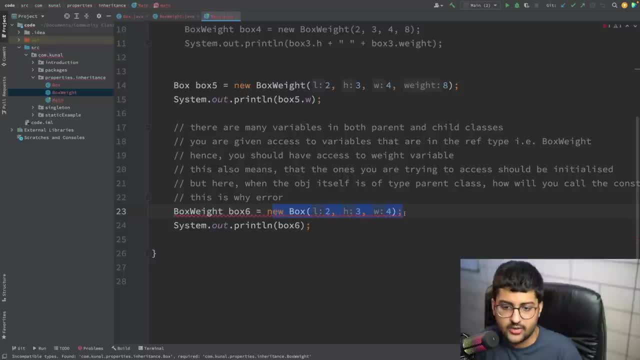 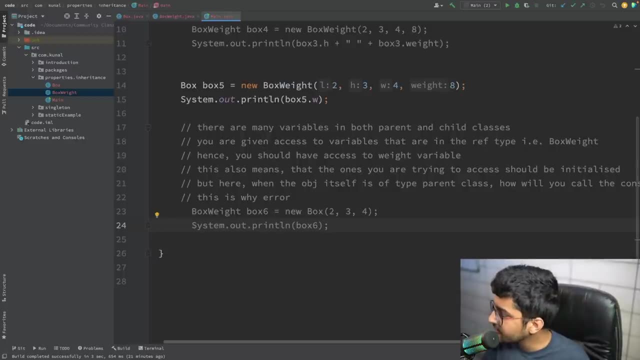 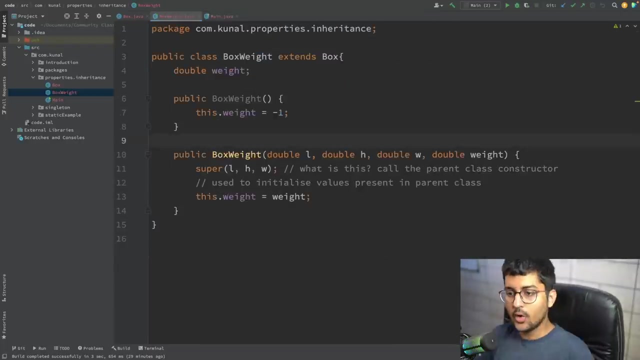 so you cannot have a child reference variable and an and a parent object. you can't do that. okay, easy stuff, all right. so that was another good, important point. let's talk a little bit more about the super keyword now. okay, so let's learn a bit more about the super keyword in detail. what does it? 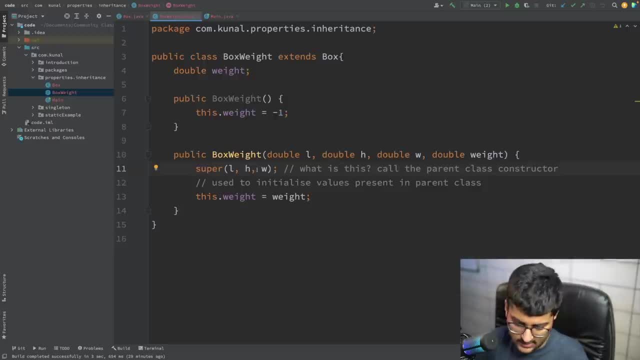 mean this thing. okay, so we know that it's calling the parent class constructor. so whenever a sub class, like the box weight, needs to refer to the super class from which it is defined, from which it is like derived, for that you can use the super key word. so let's talk a little bit more about the 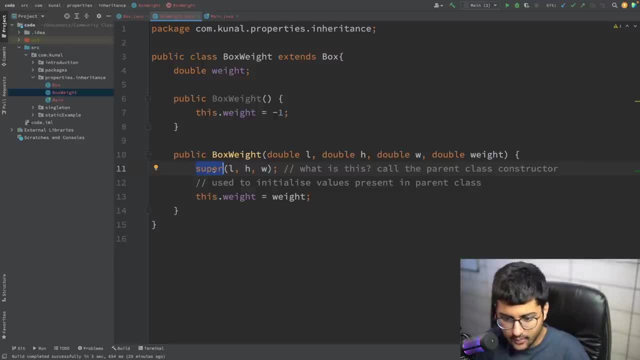 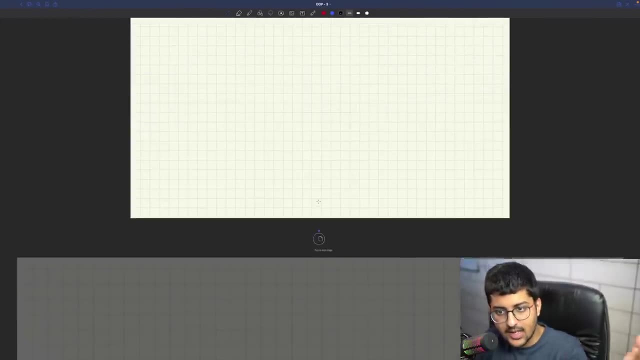 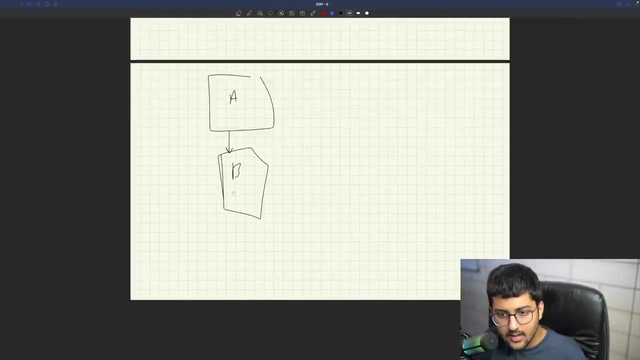 super key word. it has like two use cases. i'll go in both of those: uh like right now. but uh, it also works in like multi-level classes. so for example, if you have multi-level inheritance- one class inheriting from other class, then something like this class a, then having a derived class b, then 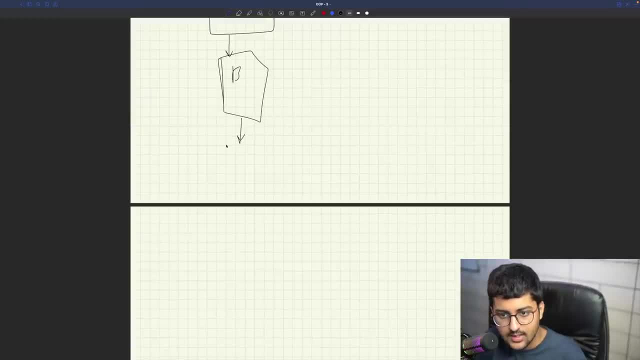 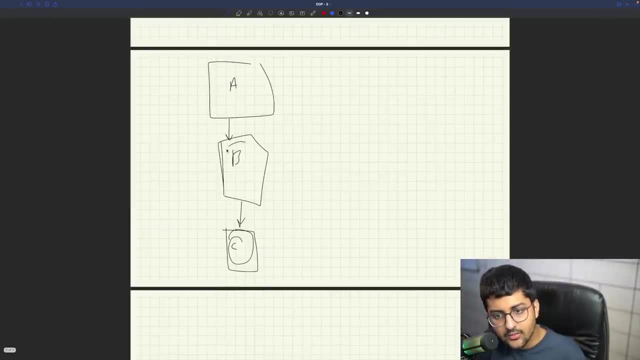 having another class. we'll talk about like types of inheritance as well. no worries, like right now, see, for example, the super keyword used in this class will be referring to b. the super keyword used in b class will be referring to a. that's it. what if you use the super keyword in a? in that case, 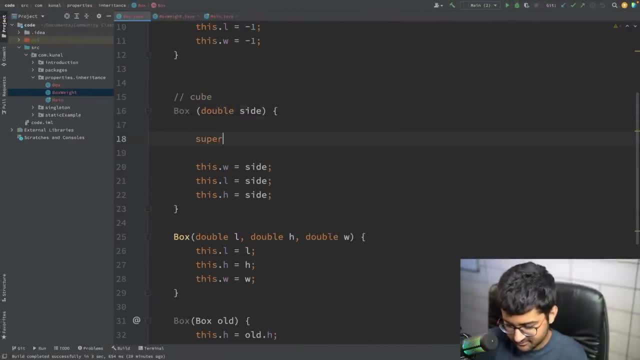 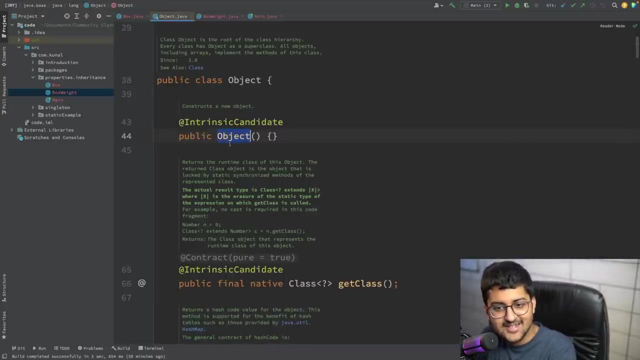 what will happen? it's not giving an error and kunal box is not derived from anything. what are you calling it then? let's see object class. so the object class is like the main class, in from which every other class is inherited, so you can see every single class that you create. 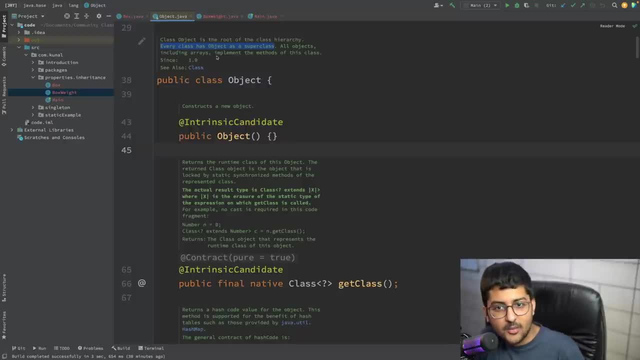 has object as a super class. all the objects like arrays and all these other things that you create, even your own classes that you create- are directly like. internal implementation of java says that they are referring to the object class. this is presented by java. okay, this is known as the object class. we 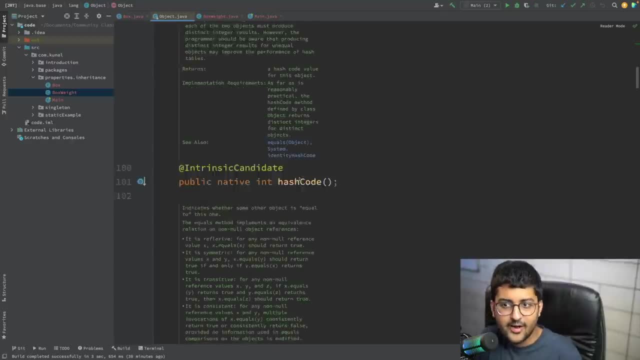 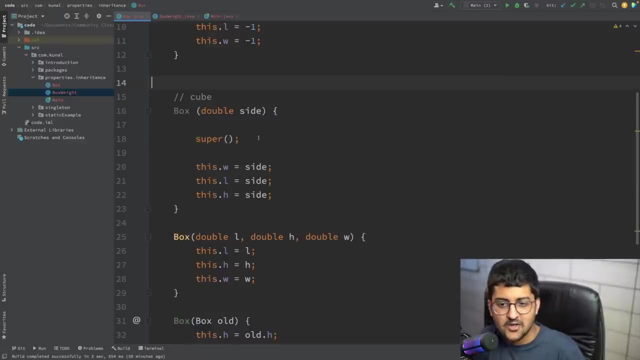 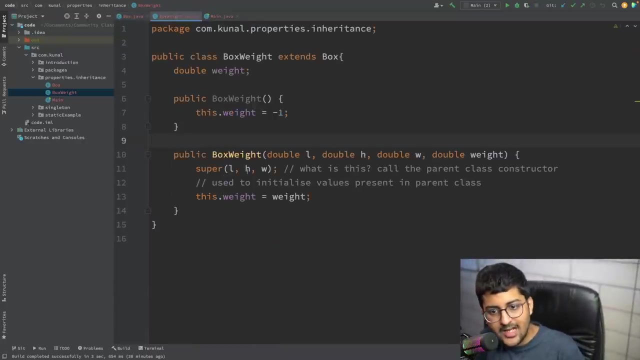 talk more about object class in a separate video, but uh, for now i believe it's a pretty cool stuff, right? so this is a simple object class and every single class inherits and inherits the object class. so super basically means directly above it. so why is box weight not inheriting object class? it is. 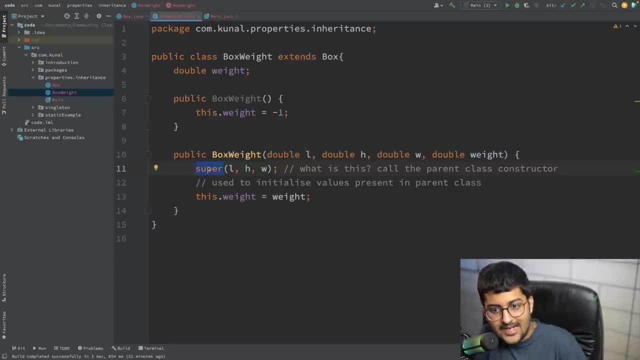 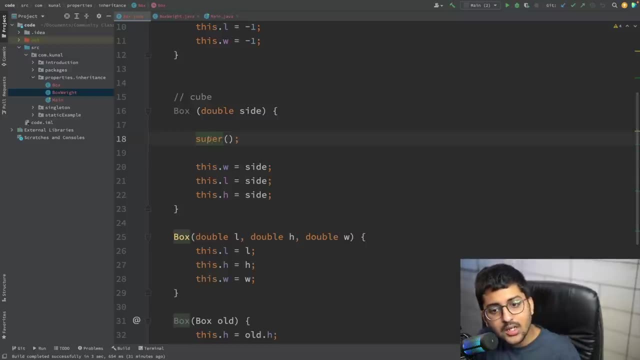 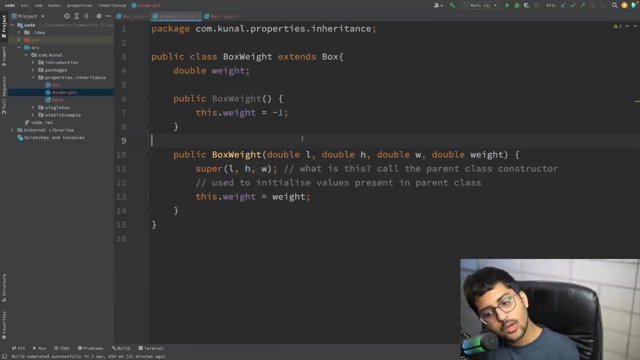 but super will actually point to the directly above it one. what is directly above box weight box? okay, so that is the first use case, which is to call the constructor. to call the constructor that is actually called by the media: construction in the internet, Andy, why I'm curios why it was calling the. 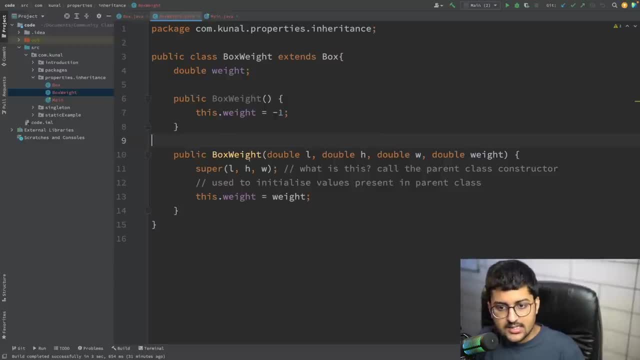 constructor, but you already know it. object class: is it recording? yeah, cool. so here what is happening: use the super keyword as the this keyword, but the only difference is that it will be used to access the super class keywords. okay, so you can say something like super dot h. 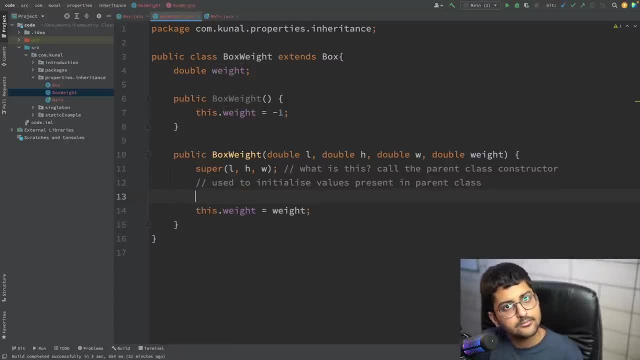 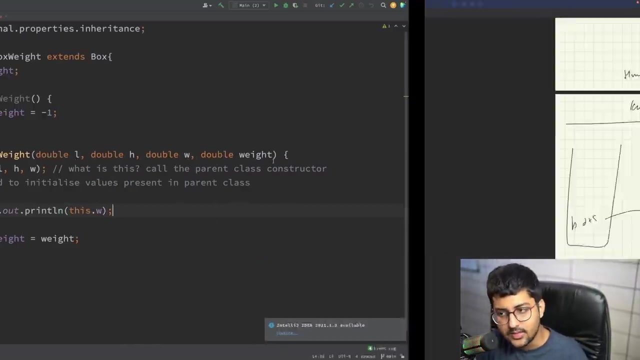 you can access it like that, okay. so here you can see it's not giving like an error. if you wanna like, print it. so, for example, what i'm trying to say is the the second use case, something like this. so i can say this dot width. so hey, does width exist over here? it's gonna be like: 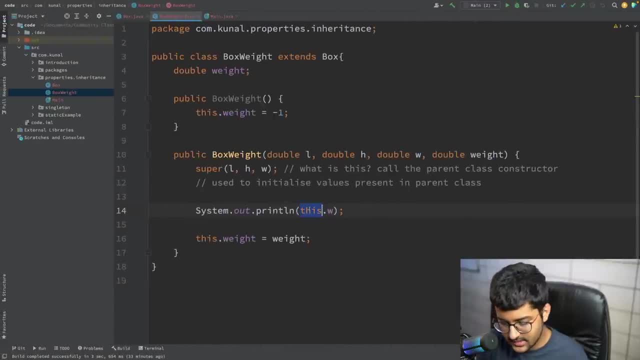 no, it does not. it exists over here. so, okay, print it. you can also access it directly using the super keyword. then it will directly access it from here. now the question might be kunal: why are you using the super keyword over here if you can just use the this keyword also? 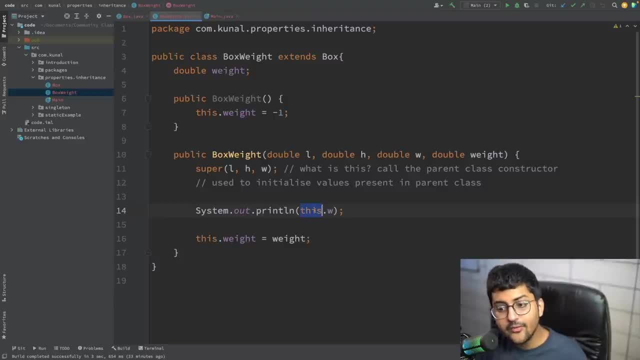 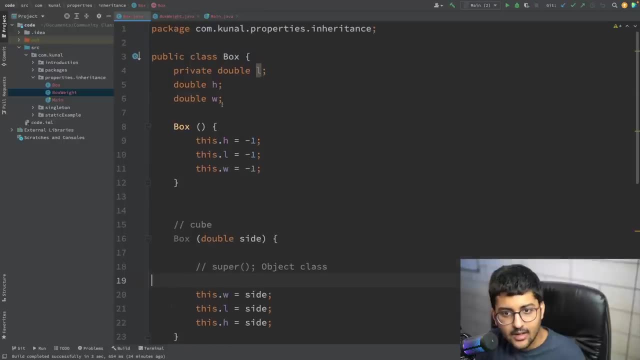 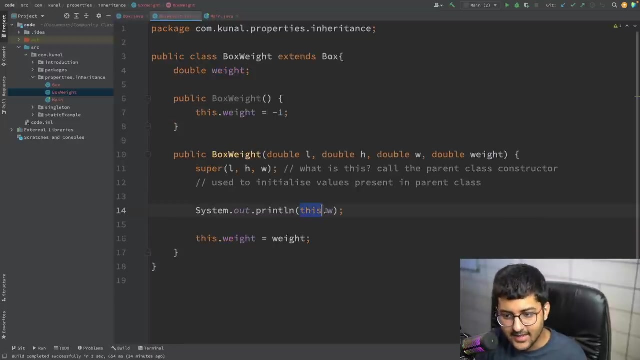 it's doing the same thing. well, the reason for this is what the reason for this is. if the super class also has a, a, a variable known as, let's say, weight, like this, in that case, if you say this dot weight and you specifically want to access this weight, then you will just say super dot weight. okay. 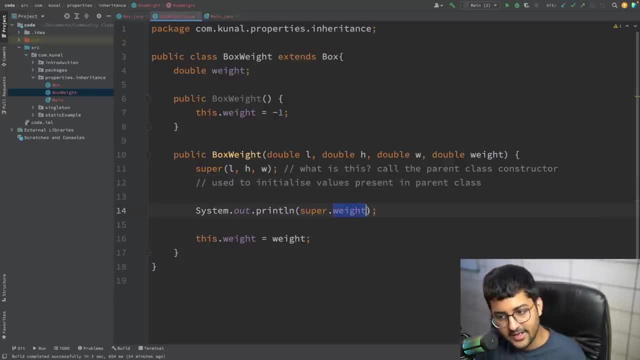 so why would you wanna use the super if you want to explicitly refer to something that is present over here? because now it has same, same type of name? right, this has a weight, this also has a weight, so this will also have a weight over here. let's say so. you'll be like this dot weight, this. 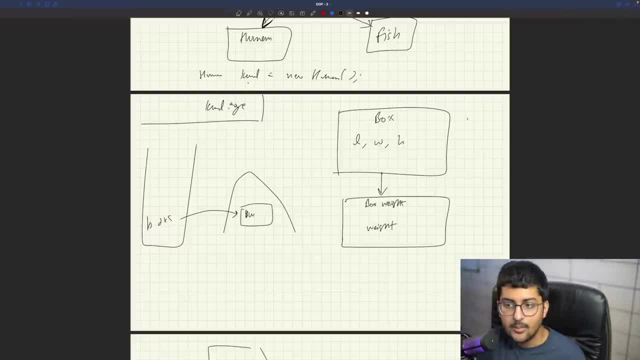 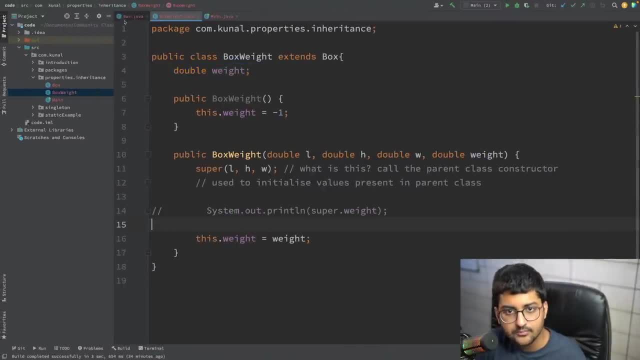 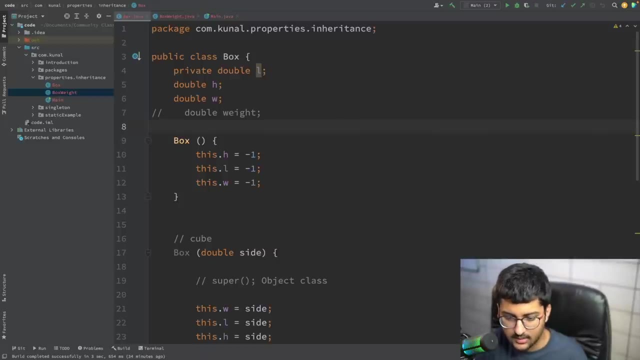 dot will be like: hey, does weight exist over here? it will be like, yes, it does, it will return this weight. what if you wanted to weight in this? in that case you can say: super dot weight. okay, that was like the second stuff, that was like just the second use case. um, so the member. 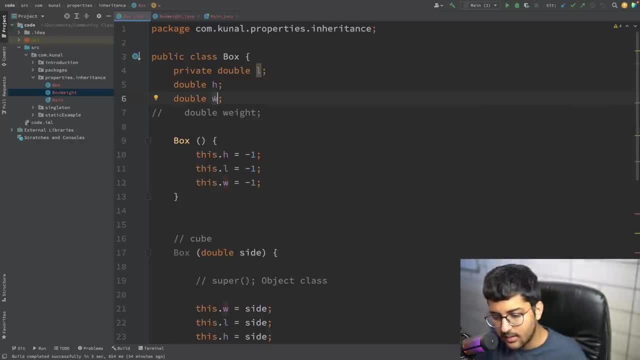 can either be like this: we have, like instance, variables, but if it can either be like a method or something, and uh, that is also why we use the input here again, when you are using an, we use it right and the super, you know, always refers to like the constructor in the closest. 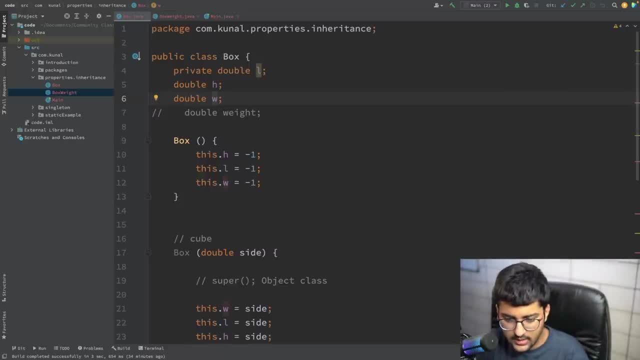 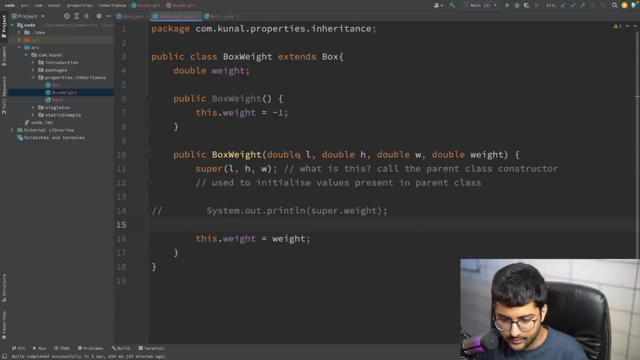 superclass. so yeah, that's uh pretty much about it. so in this box, weight one, it was calling the box one, and the super obviously requires the uh. you know the uh, the arguments. so you know, in the, in the hierarchy of our classes, if the superclass constructor requires some parameters, then all the 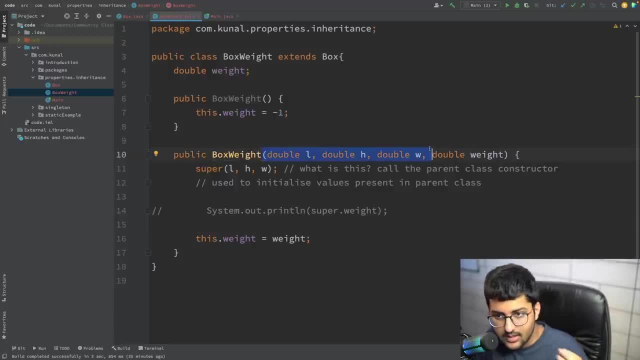 subclass, you know, must pass those parameters like this over here up the line. they're going to pass it up the line, okay, uh, so it's true, basically, whether you know whether or not a subclass needs the parameters on its own. so it does not, let's say, need l, h or w, because we are just using. 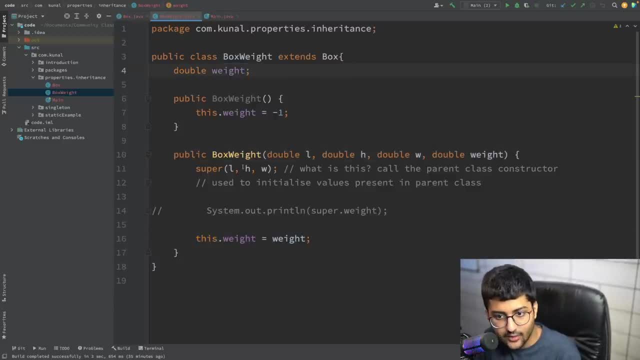 this dot. weight is equal to weight is just setting it, but it needs it for the super one, okay. so if you think about it like, it makes sense that constructors complete their execution in like the order of uh derivation. we can see the execution for this as well. so let me just uh put something over here. 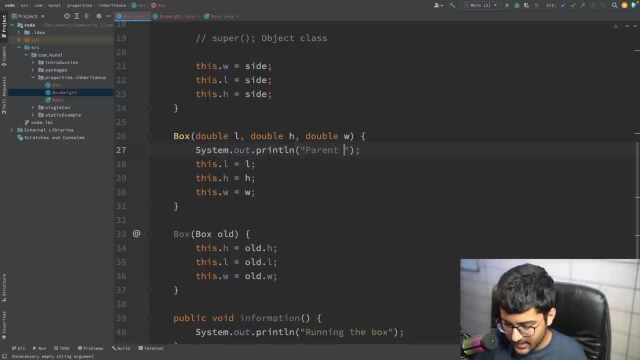 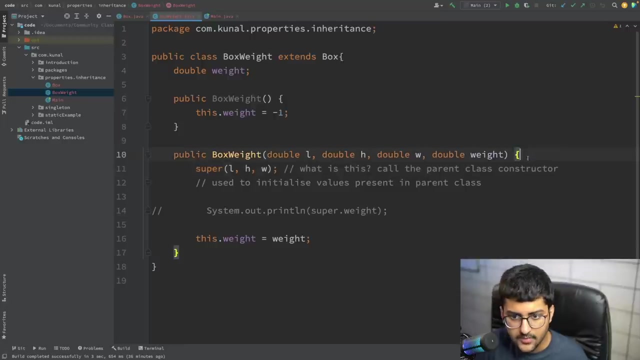 let's say print parent, or i can say box class constructor, so we'll also see the order in which this runs. okay, and here i can just say something like this: one second, yeah, because one one thing i mentioned was that the above classes will have no knowledge of the 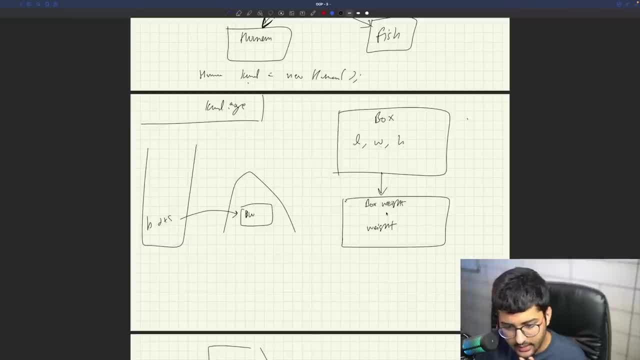 below classes. right, so that is what we mean, that, um, the superclass will have no knowledge of the subclass and any initialization it needs to perform it's going to be obviously then separate from the- uh, you know, any possible any like prerequisites to to like any initialization you? 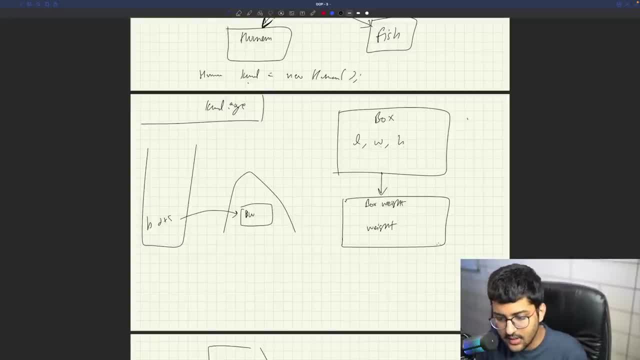 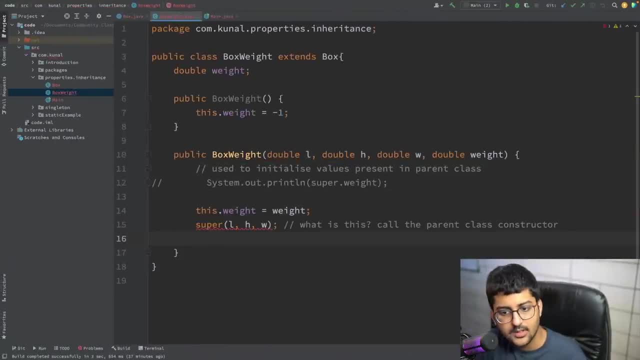 know, performed by the uh classes below it, for example. therefore, it makes complete sense to execute this thing first, okay? so if you put it somewhat like this, it's giving an error. that is what i meant. okay, because the superclass does not need, does not care about base class superclass. 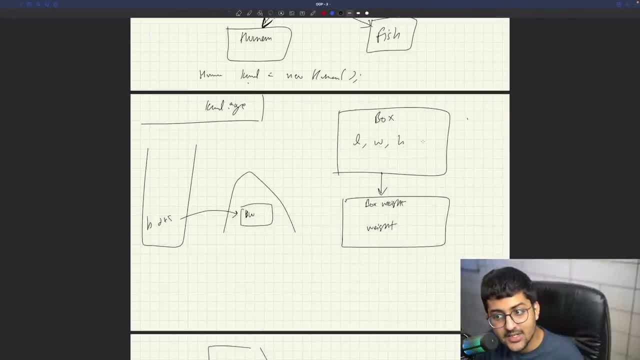 does not know what the base class contains. this class has no idea what this contains. base class contains base class. now the superclass has no idea what the child class contains. okay, box has no idea about what weight contains. so box is going to be like: okay, i don't really care what box weight class contains, so i am going to. 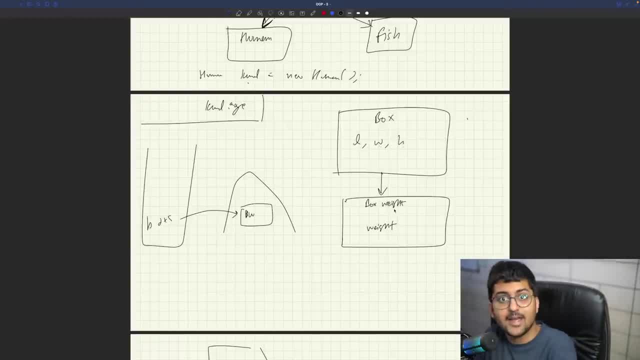 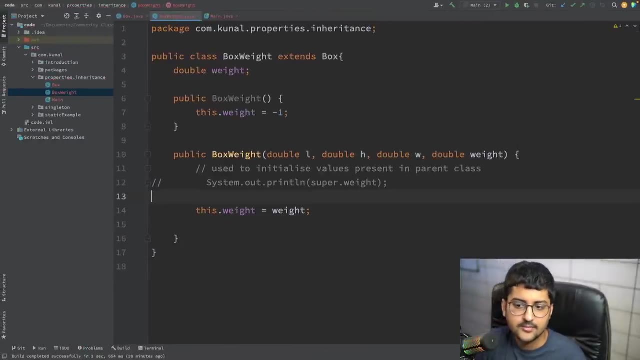 initialize myself first. but box based does care about what box contains. child class cares about what parents parent class contains. that's why child class is going to be like: hey, parent class, i really do care about you. please initialize yourself first. that is why like this, that is why it was giving an error when i was doing it before. 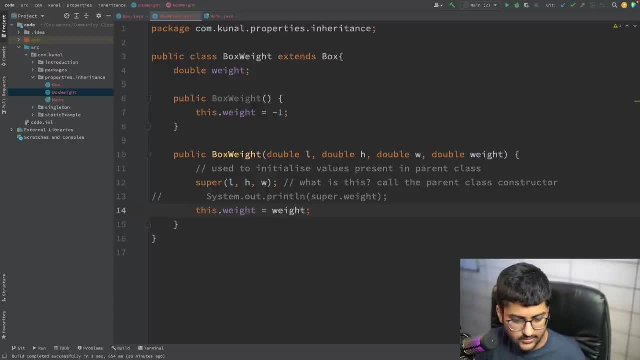 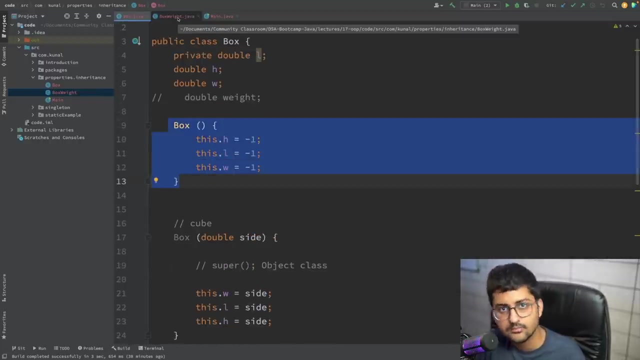 so that was also covered. and uh, yeah, and note one thing: if the super is not like used in a subclasses constructor, then the default uh, or like, the parameter constructor of of the super class will be called. so, for example, if i do it like this, the default one will be called. okay, this default one will be called. makes sense, that's it. 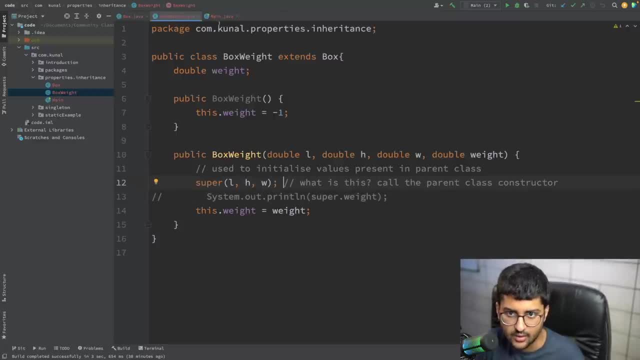 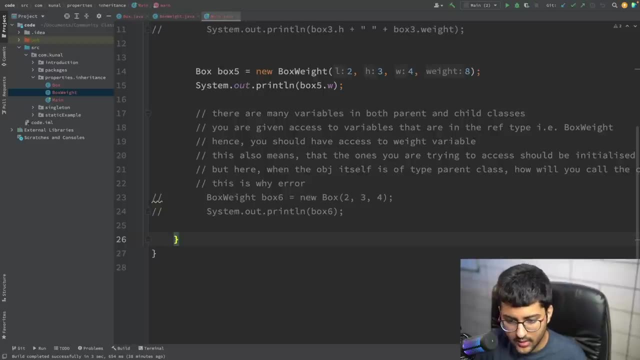 this is also something we covered previously, because when we were doing this, it was printing uh minus 1 or something. so it was covered okay. so that was like a use of super. okay, it's cool, let's move forward. okay, let me show you one more thing. let's say i create uh in the box. 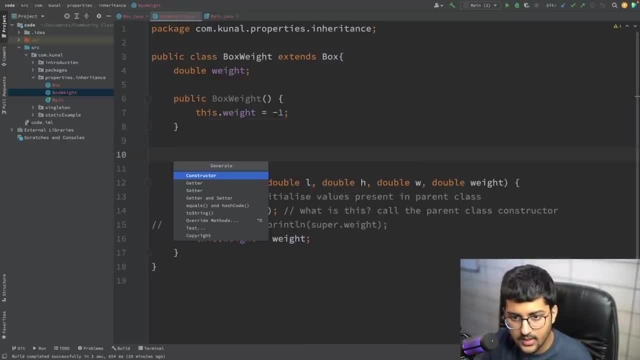 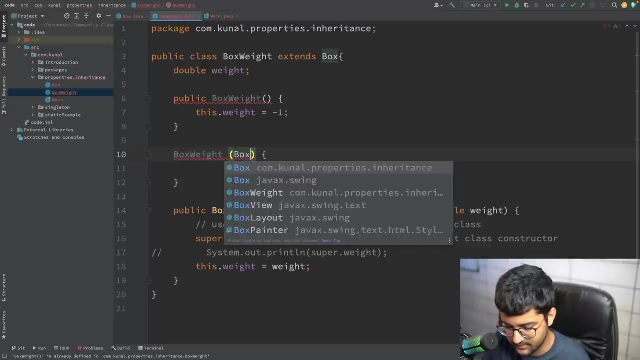 weight, I create another constructor. okay, I create another constructor, that just simple constructor. it does not take anything. I can just say: box weight, not take anything. it's actually like a copy constructor. it takes another box weight, for example, another box weight, other object, okay, something like this, so you can say: weight is equal to other dot. 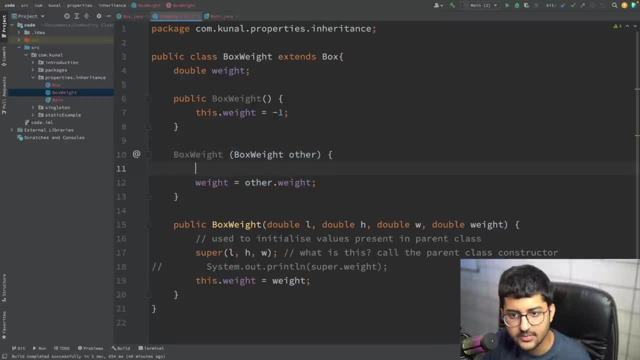 weight and you can then just say something like this super of other, it's not giving any error. what is happening over here? note that in this super, the other type that you are passing, it's actually a type. it's actually a box weight type, but here it's actually taking. 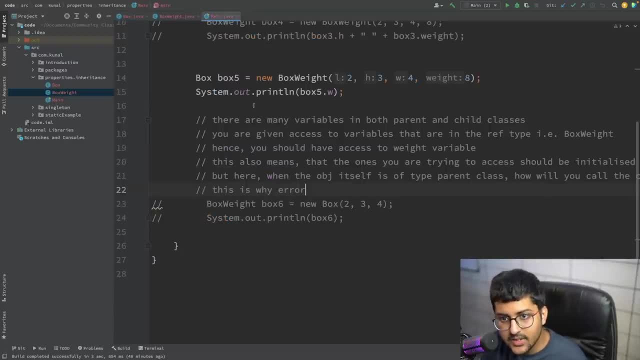 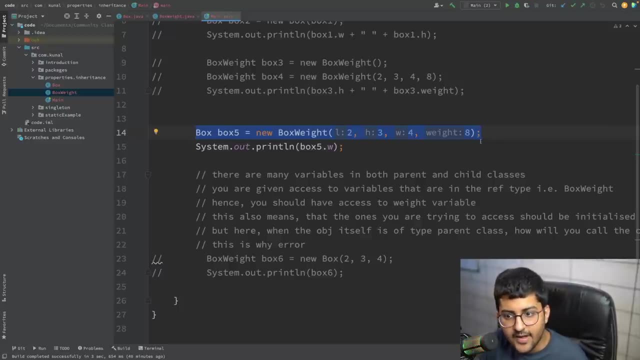 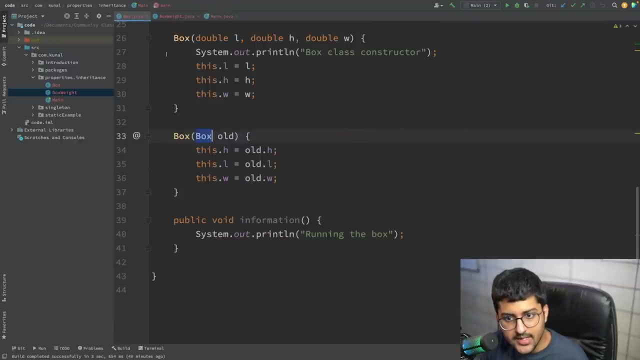 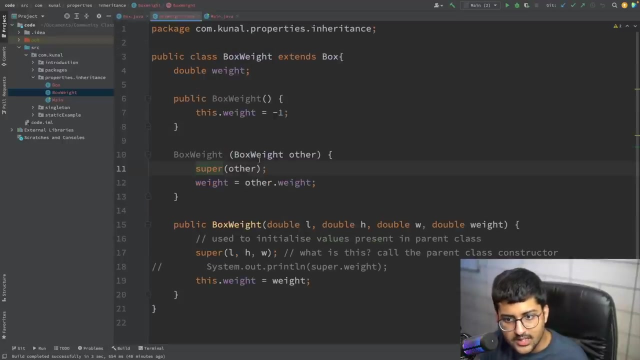 a box type. isn't this the same thing as this? okay, okay, whenever you see anything like this, check out these common sense questions. so here it's saying that, okay, the copy constructor actually is taking a box type. you are passing an object of box weight type. does box weight type have access to all the box type? yes, it does, for 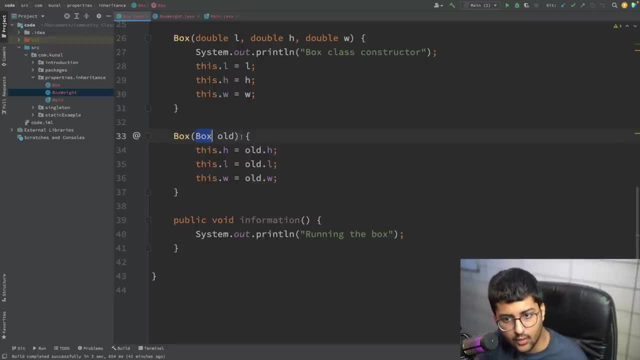 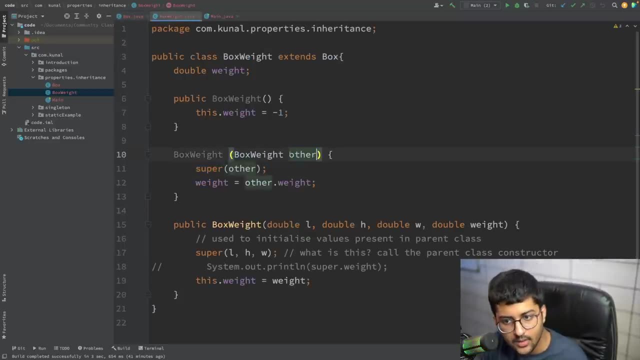 obvious reasons, because the parameter over here is box, so it will only have so. this internally says box. old is equal to other, something like that of type box weight. so it's going to be like the reference type is box, so even though this is a box weight, 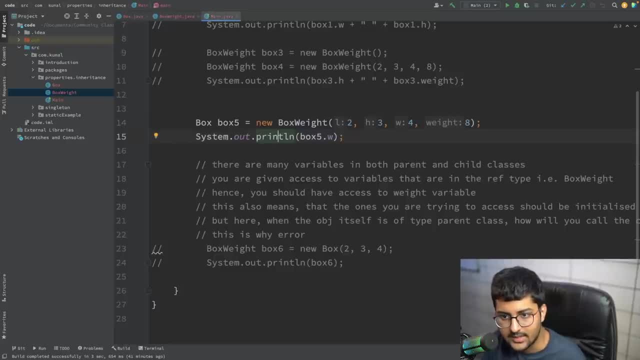 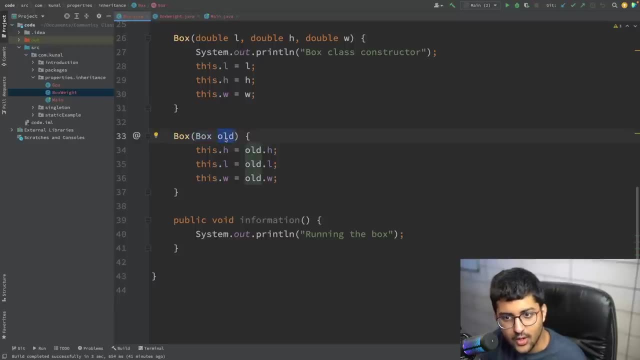 type, it's going to only have access to box type. so something like this, exactly like this, not something like this, exactly like this. so here it will not have access to old dot weight, obviously, because if it's a box, it's a box type, but if you're passing a box weight, 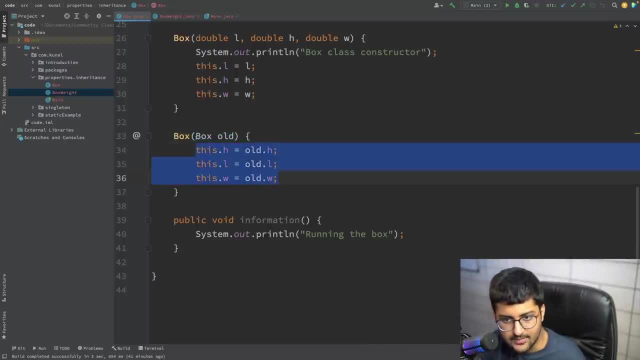 object over here, it will only have, obviously, access to the three types that are available in box only, because what is accessed is based on the type of object that you are passing over here. so this is the type of the reference variable, not the type of the object. same part. 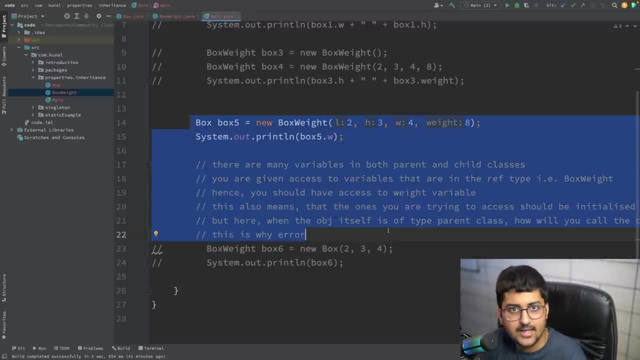 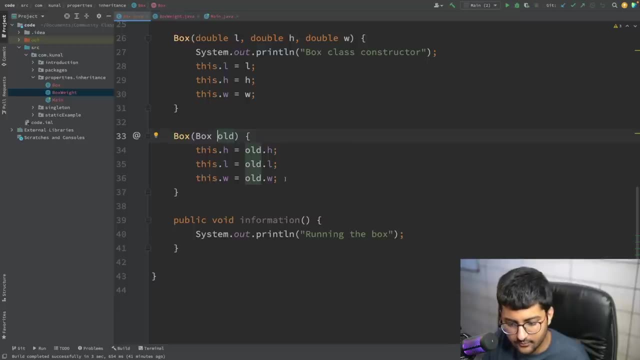 as this thing, exactly same, dicto copy paste. this thing, concept in this thing. exactly the same thing, exactly the same thing. okay, so in the super, when you pass the object of box weight- uh, box weight, you know of type that is not box, it still invokes the constructor. 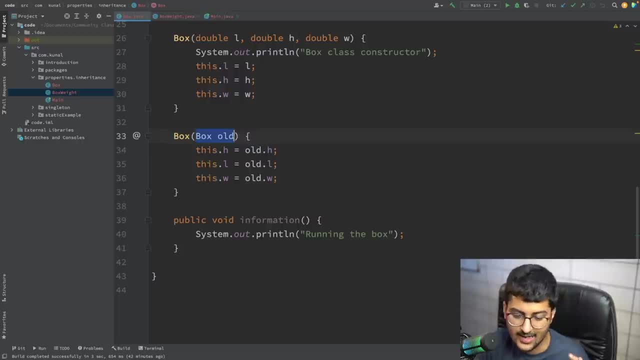 this one because, uh, you are able to put it over here, it's allowed. okay, so super class variable can be used to reference any object from that derived class. hence we are able to pass box weight object to the box constructor. obviously, the box will only have knowledge. 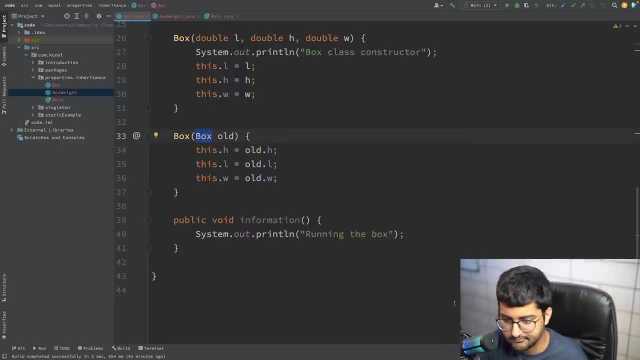 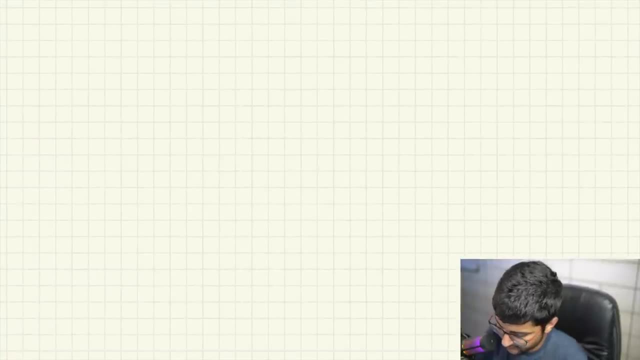 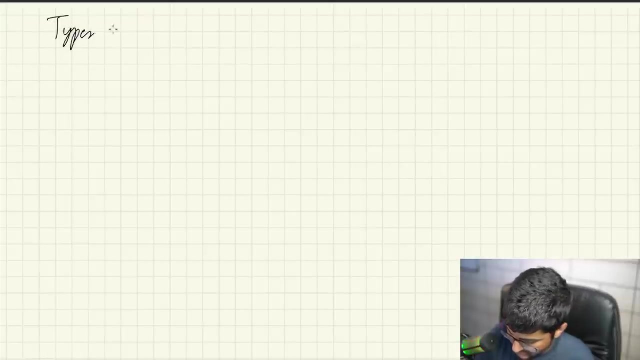 of its own variables because it's of type box over here. okay, cool, let's move forward. okay, now let's talk about, like, let's say, the type of, uh, types of inheritance. okay, so, let's talk about the types of inheritance- important concept also for your exams and stuff in BTech or your. 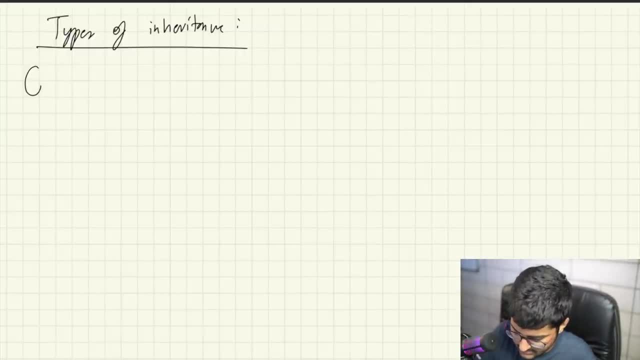 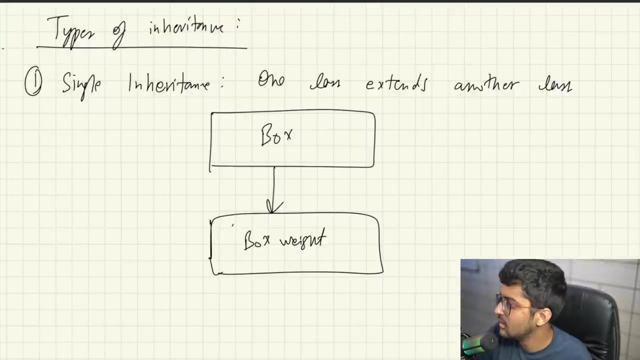 bachelor's degree or whatever. so some, the first one, the one we already like, just covered: single inheritance, single inheritance. what happens in this? one class extends another class, one class extends another class, no problem, we did it. something like this, something like box, box, wait, no problem, no problem at all. right, that's the first one we've already. 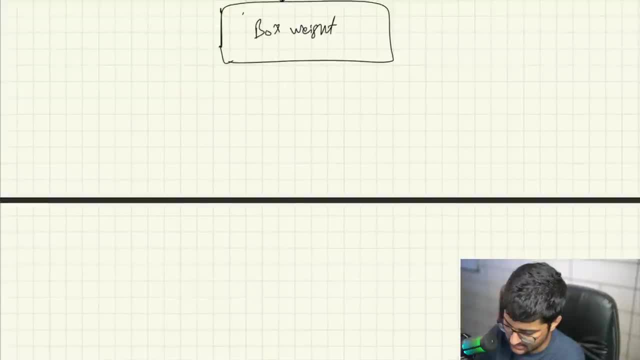 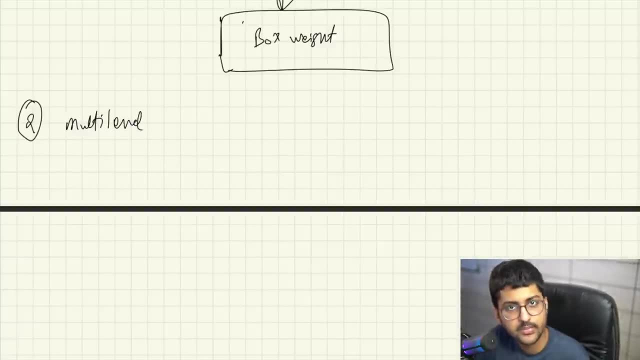 already covered it. second one can be, let's say, multi-level inheritance. so what happens in multi-level inheritance? one class can inherit from, like, a derived class and the derived class will then become a parent class for another new class. so something like this. let's say, I have a box class, so 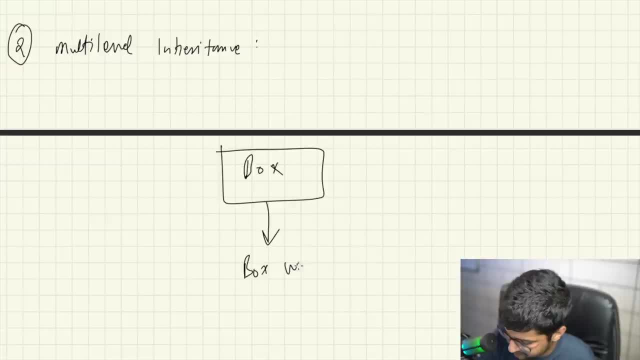 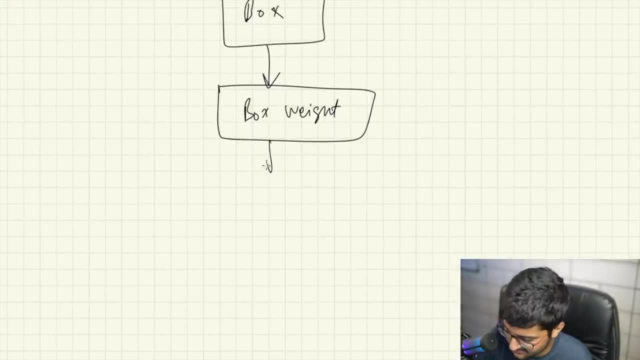 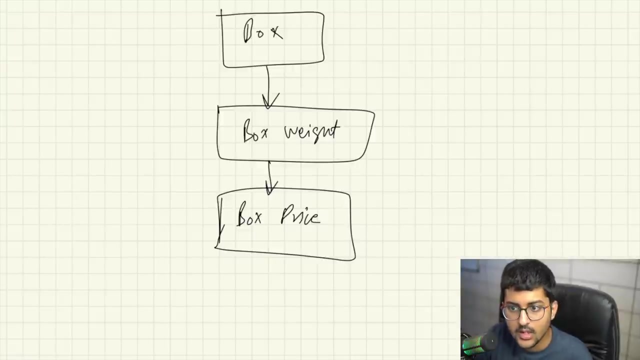 box class is actually parent for box weight class, no problem. now this box weight can itself be a parent for another class. this will be a parent for, let's say, box price price, okay, something like this. okay, so here you can see that Box Price is a subclass of Box weight. 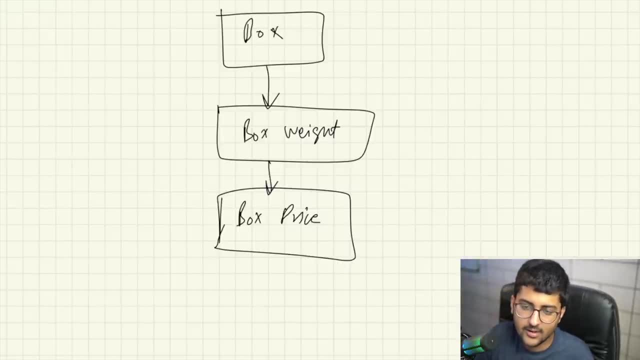 and Box Weight is a subclass of Box weight, subclass of box. now you may be having a lot of questions, kunal, can the elements in box price access box? how will you call the constructor of box weight and then constructor of box if you're making an object of this type? can you make an object of this type, okay, so so many questions. 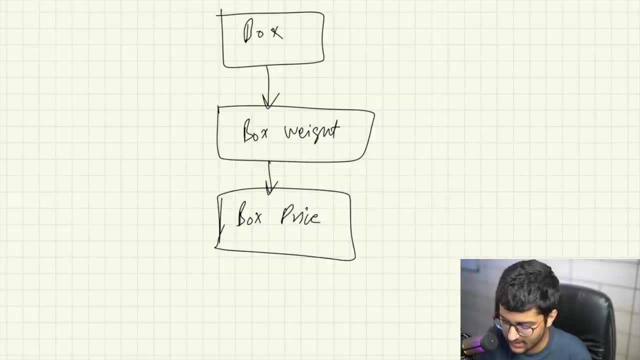 you may have in canal. if you're making a type of this thing, then will you call the super class of this or super or this or whatever. how will it access? how will it actually run? so one thing i really want to tell you bluntly right now. bluntly, i will cover all these things right now. but 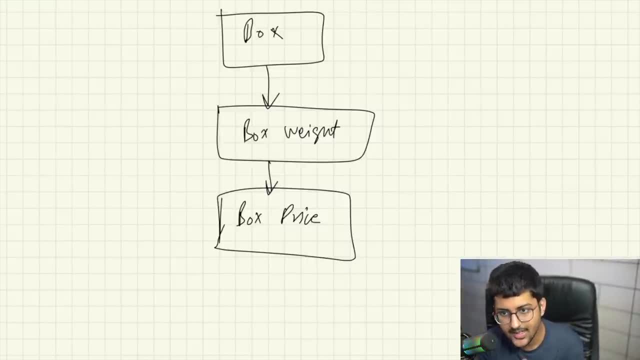 you will not understand object-oriented programming till you use the hit and trial method. what does it mean? trying out various things at random go like: do random stuff, put something over there, put something over there, make base classes, add constructor, add this, add other functions and things like that. call one constructor from another constructor, put a debug. 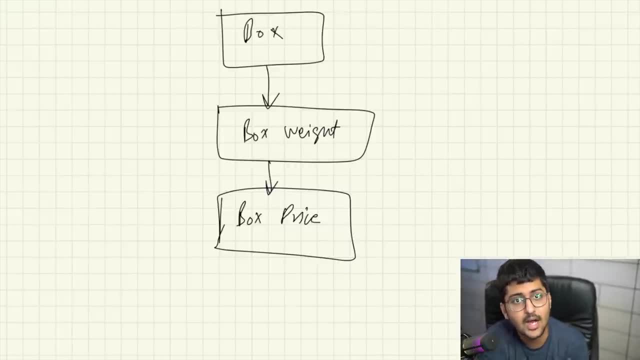 pointer, put print statement, do random things and then see how things are working internally, because oop is common sense. there's no algorithm or anything in objective programming, it's just a set of rules. hence it should be easier to understand. but you would not know what to understand until you do it. 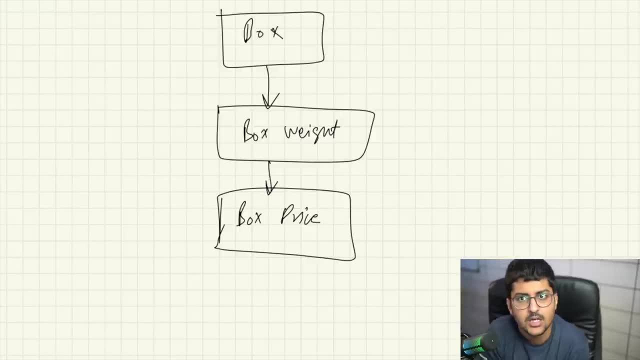 yourself. people ask me questions like this: don't be this person. if you are this person, no one can help you in this world. so some people will like what will happen if i try to put this instead of this and print it. well, what will happen? do it yourself, code it, print. see what will happen. 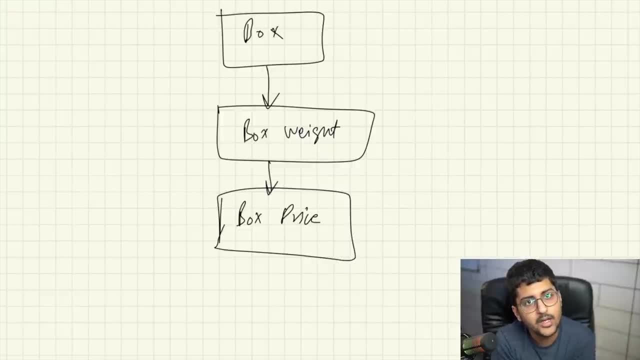 how weird is this? what will happen if i put uh protected in the? obviously i will cover protector and stuff. so what will happen if i say put this method as private? what do you mean? what will happen you? you don't have a computer, try it out, run it, please. object. 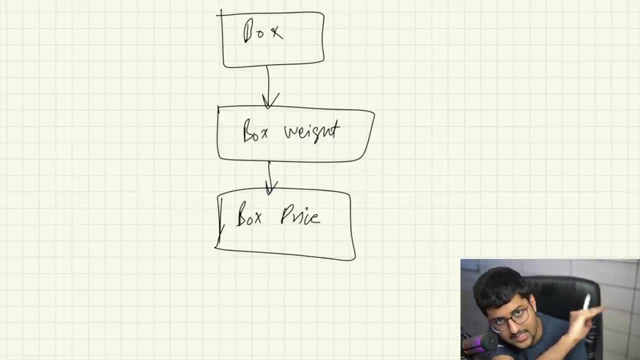 object programming recur in recursion. i taught you right how to understand recursion. this is the how to understand object from a problem experiment. why always ask the question why? why is this happening whenever you do something and everything is common sense, all the basics and everything. i'm covering, even stuff apart from basics, doubts that you will get debugging and everything. 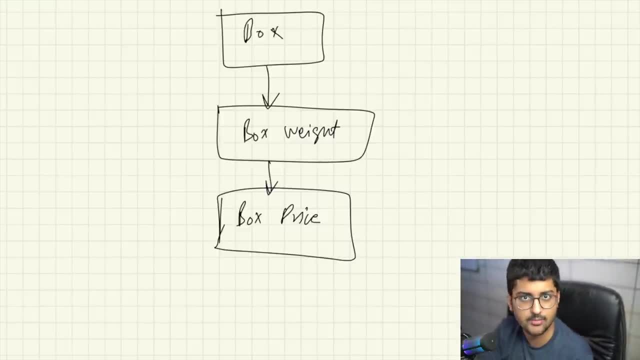 everything i'm doing. still, if you find something that you are not able to like, something that is new- which i'm pretty sure, like you, you might, because there's a lot of things, but i am pretty sure it will not be something different than we are already covering in this video, okay, let's try to see answer all these questions like box box weight. 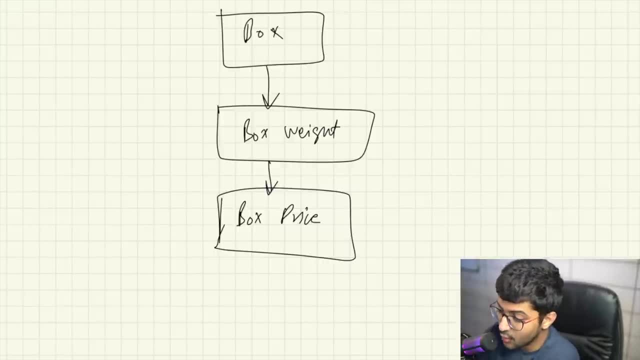 what will it access? how will it access, how will it move and all these other things, how the objects will be created. so common sense that we've already discussed is above class has no idea of bottom class, but every bottom class has idea of all the above classes, basically all the above classes in 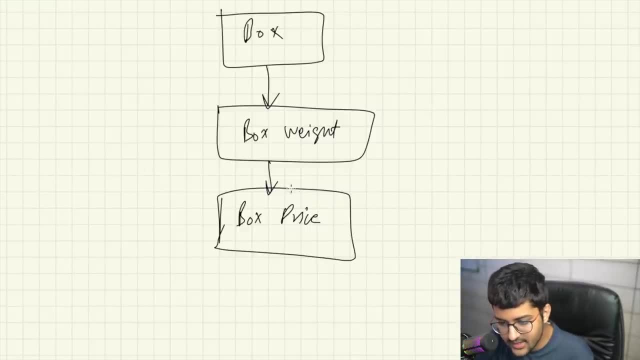 this trail. okay, if, if this, this, this box, this box, price class is connected via all the other classes using this arrow, right, so it will obviously have all the information about the above ones that it's connected with the arrow, so this is connected with this. hence, this is connected with. 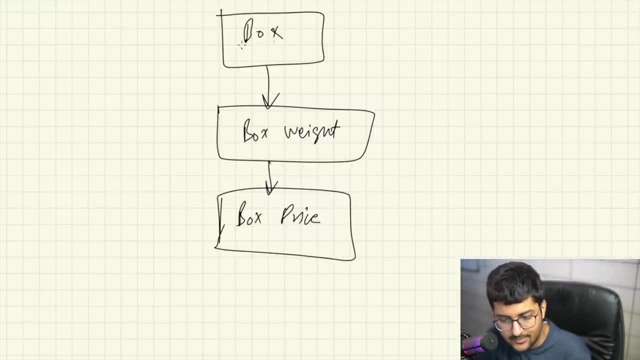 this hence box price, will definitely have access to the elements in box. if you put out something like this, this is something we'll do later on, or something like this. let's say something like this class a, now this box price. and this is not connected. connection only happens. 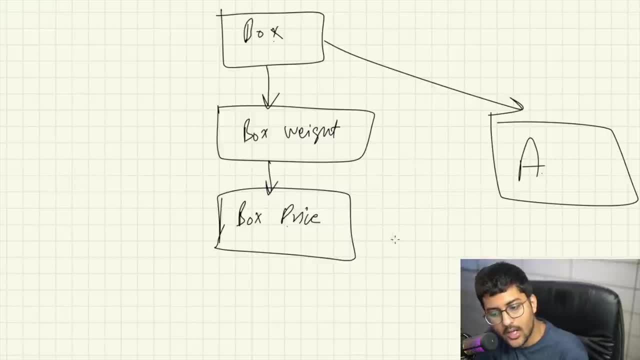 above, not like above, then below, okay, above only, so it will only have all the access to the classes above it, not like above and below. no, just go above only, okay. but uh, let's move forward. and uh, check out like this is actually very simple. i'm pretty sure i should not do it, but still, i'll show you. 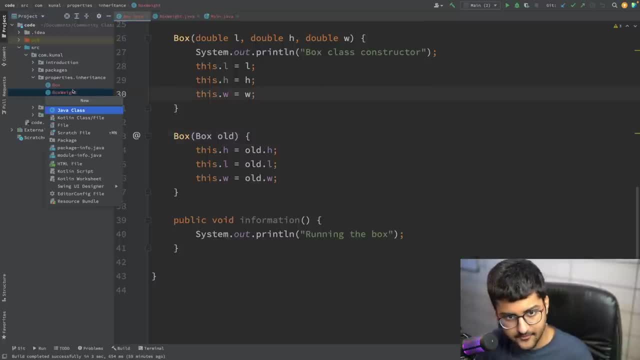 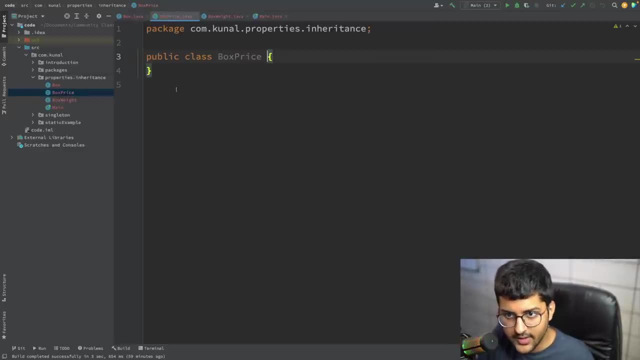 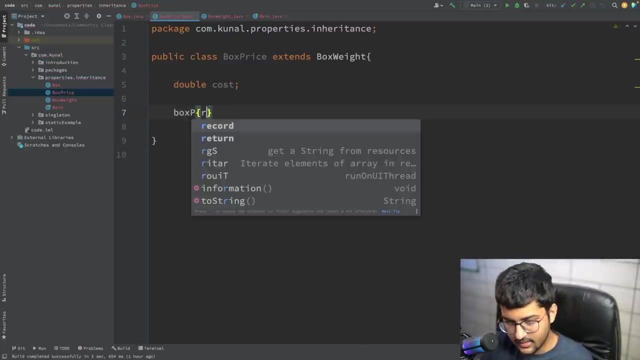 let's go okay. so let me create over here box price, no problem, it extends. what? box weight? okay, no problem. let's say it will have a price or a cost or something, so i can say: cost, okay, something like that. initially i'll just say: a simple constructor. 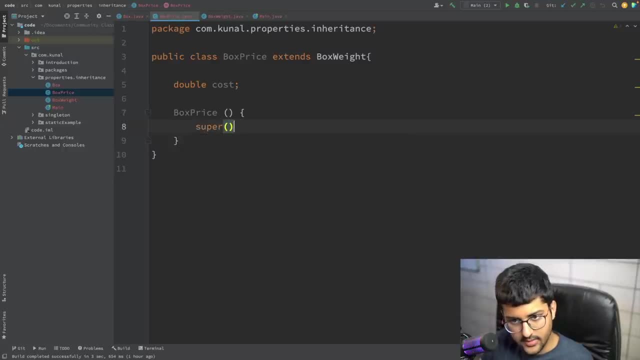 that's it just going to say: call the super keyword, okay, we'll see how this thing works internally and everything and itself it will set the cost equal to minus one, okay, similarly, you can have another box price that takes, uh, another object of type, box price or other. 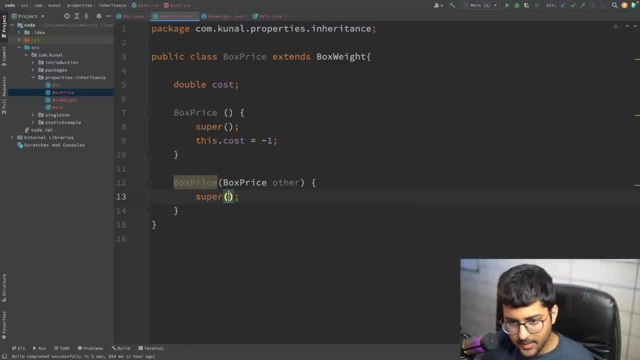 something like that. okay, so there you will say: super of other and this dot cost is equal to other dot cost, that's it. similarly, you can have another constructor of that is actually taking all the arguments, so something like this: actually one second, so that's it. like this. okay. so here it's saying: super off all these three. 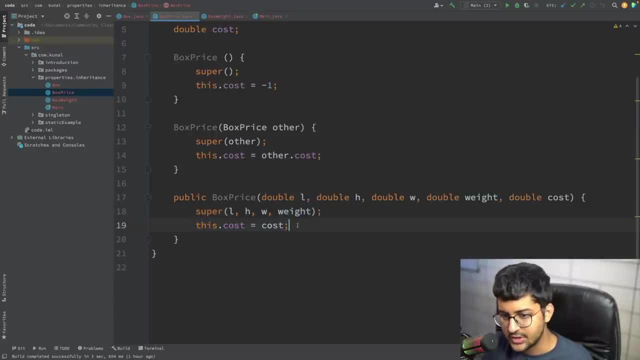 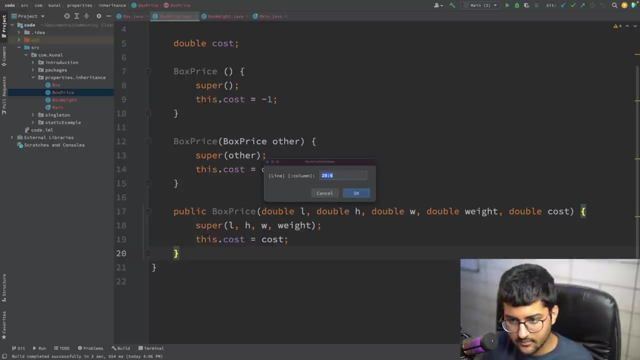 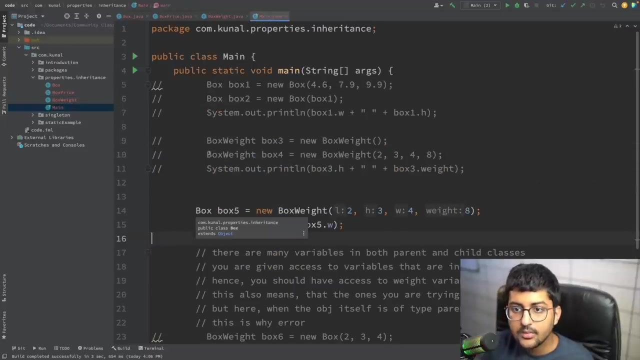 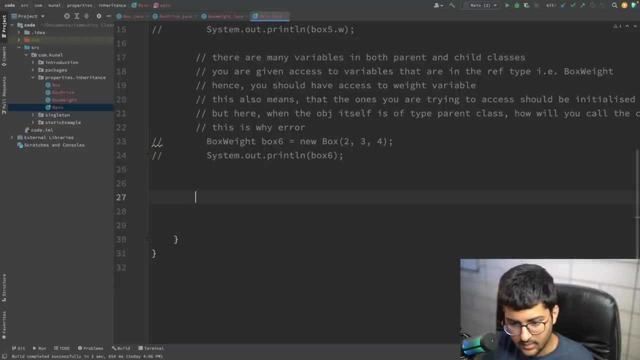 and the weight plus um cost. okay, sound good, okay, so that's it. yeah, let me create. uh, yeah, that's it. yeah, that's it. yeah. cool, let me do something in the main. let me just hide this. start a fresh. okay, no problem. so i can say: box price: box is equal to new box price. 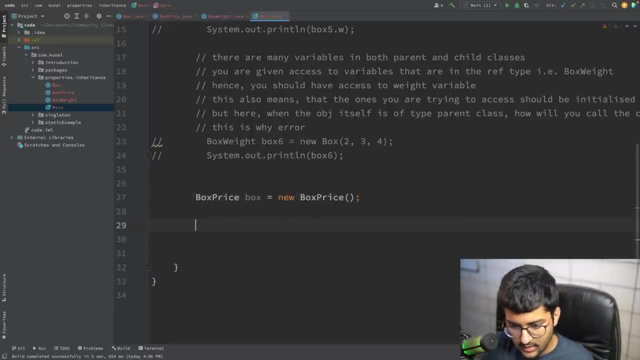 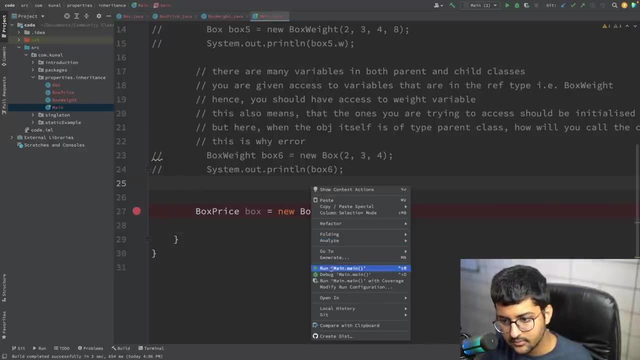 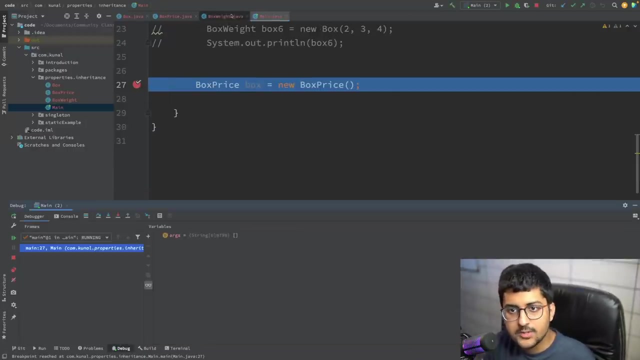 okay, initially i'm not passing anything into it. okay and uh, let's see how it works internally. till box It's gonna be like you take a lil bit, but in there of like a box so calling the box price method. so it will be like, okay, box price is being called. 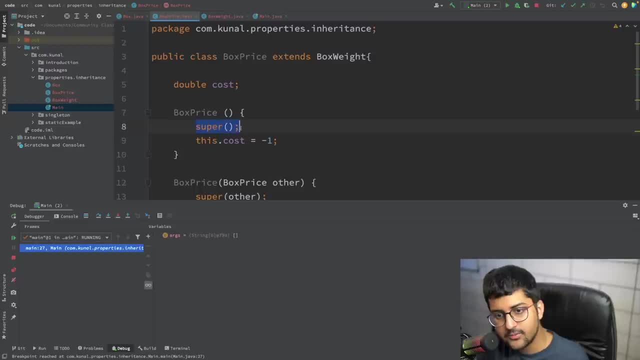 i told you what. don't ask me questions like which super keep super construct rate will call. i just gave a really big explanation about superRYP needs to start 100 years old. you just a really quick question about super calls. which one you tell me you can super calls the constructor, usually right now, either �ن. 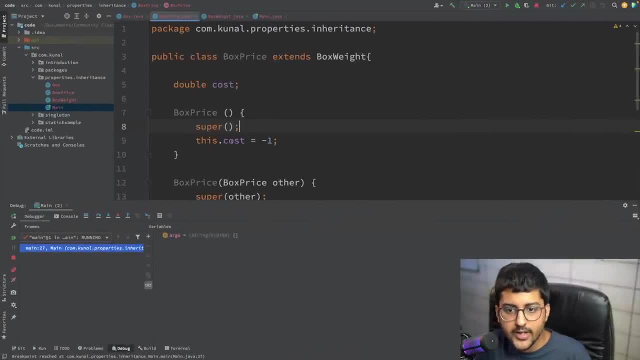 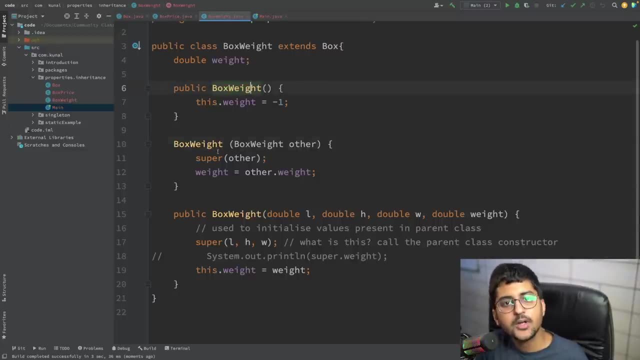 is a construction company. The world is which one is just above box. it will call box weight. there you go. don't need the debug part. we can, i can do this. okay, so it's calling the box weight. box weight will call which one? the box one. so, for example, if i put something like this: let's 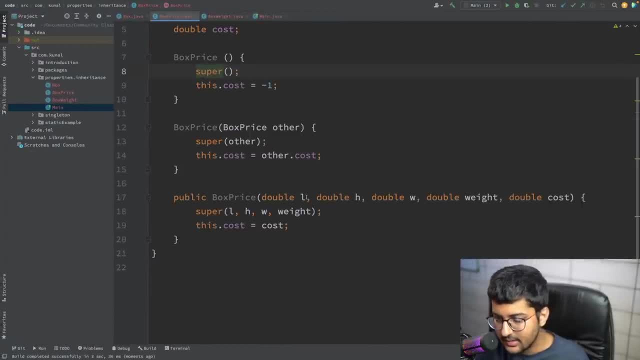 say in box price, i'm actually putting something like uh, length, width, or i can create a side as well. i can say double side. now i can just pass a side over here like this: one second. we need a side over here as well, obviously, because this is going to call the super keyword means the 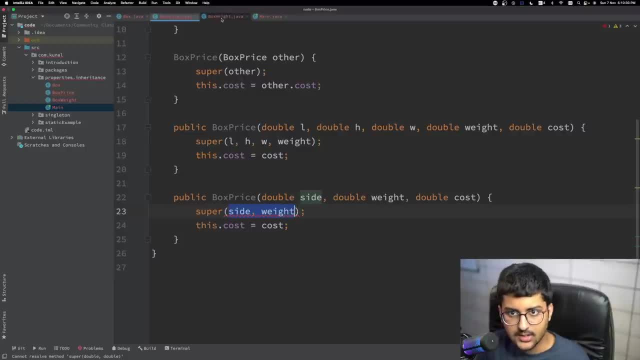 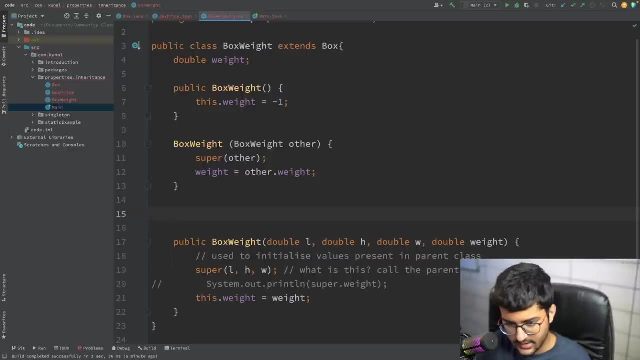 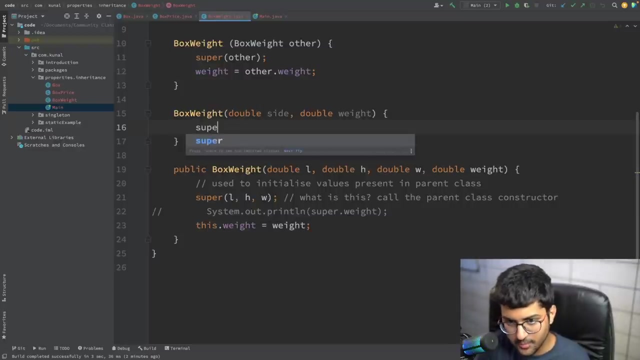 constructor of box weight- box weight. there should be a construct that it takes two things. there is not. let's make it constructor that takes two things. okay, no problem, it takes a double side and, uh, double weight. now this box weight will call the constructor super with side. 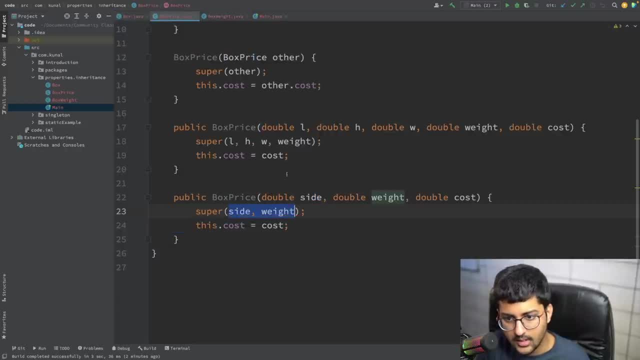 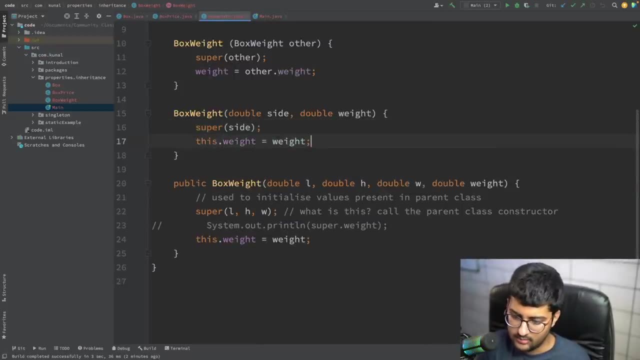 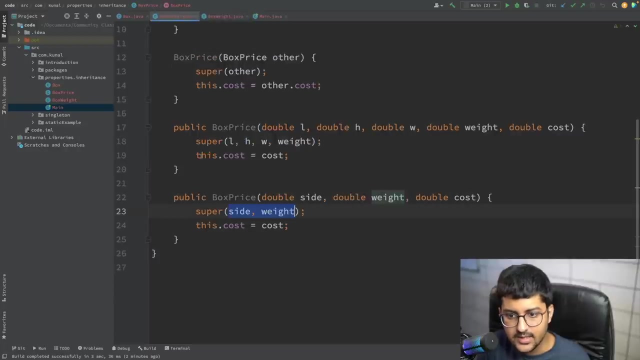 that takes one argument. there is already one available for that, no problem. and this dot, weight is equal to weight, no problem at all. okay, no problem at all. so this is calling, let's say, if i just say box, uh, box price, and i just uh, let's say, call this one which is side weight and cost, side is, let's say, five, weight is: 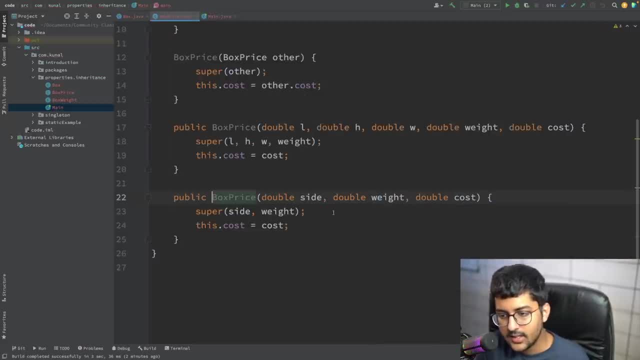 eight cost is 200 internally. it's calling which one it's going to be. like: okay, box price means box price one. okay, this will be called double side comma bit. these two are the ones that are actually above in the above function call. like: okay, pass it in the above function call. 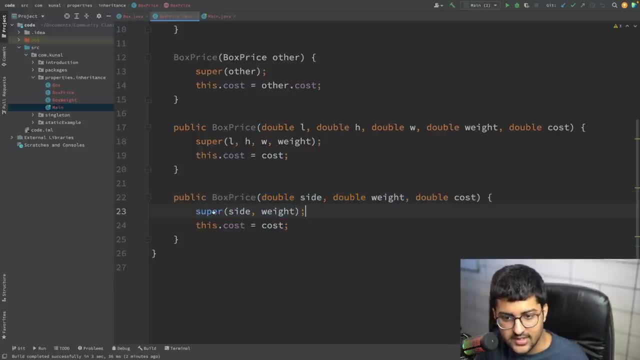 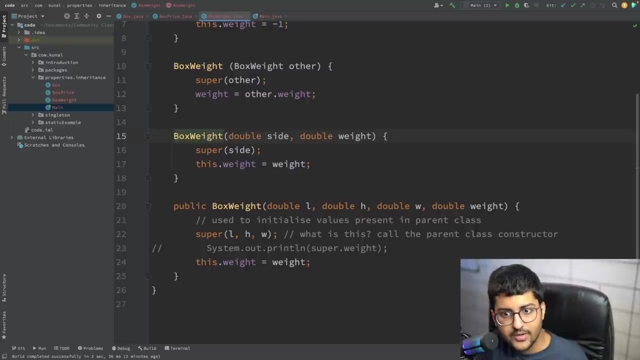 and i literally just made this right in front of you. so obviously, if it's calling the super one, it means that it will call one in box weight. hence box weight should have a constructor that takes two arguments- arguments and it itself will set the cost to itself. now it will go above box weight, so like 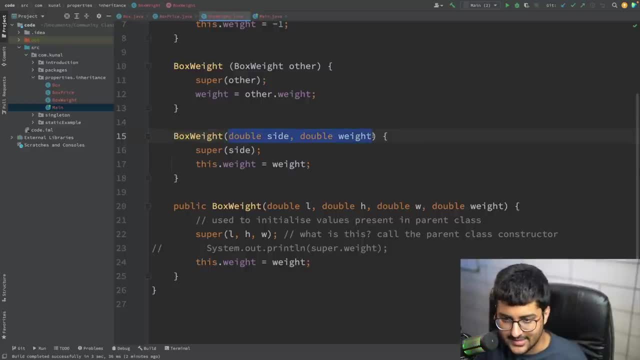 does box weight contain a constructor? that which takes two argument: yes, it does. now, this is one specific to box weight. this is for its super class. the side one is going to be like: super side means there should be a constructor in the super class. means the box class. that takes one argument. 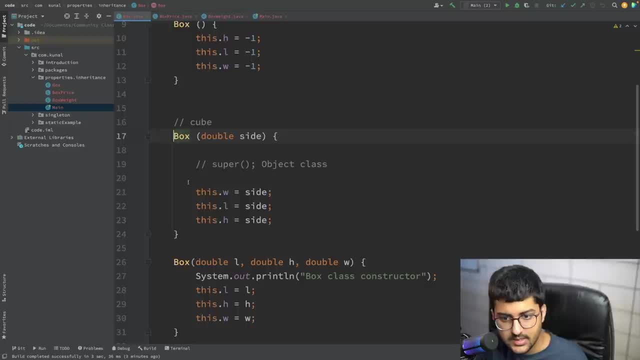 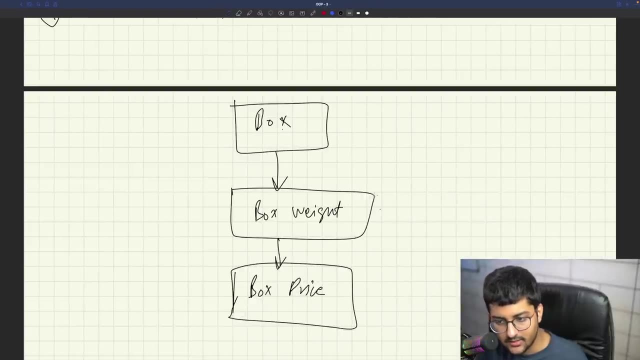 and it will set its weight over here there is, and then it will do the following simple: so this will call its constructor. it will instead. it will then call this constructor. it will then call this constructor. only doubt you may having is how many arguments in every constructor. 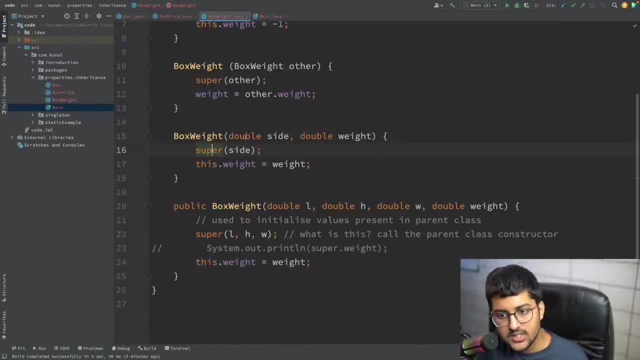 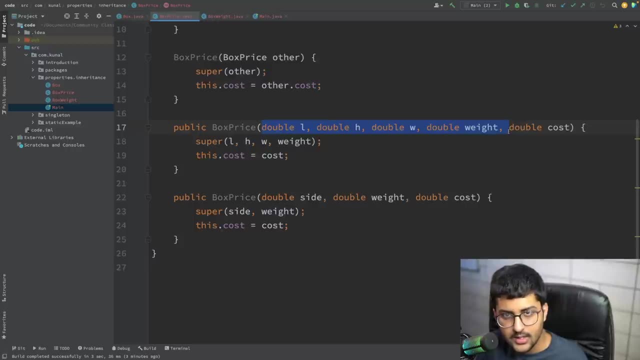 that is obviously up to you. okay, usually it's convention like to how many, how many? um, how many super class keywords you have over here, like super class variables you have over here, just put it over here like this. then the base class ones you put it over here like this: but we already covered. 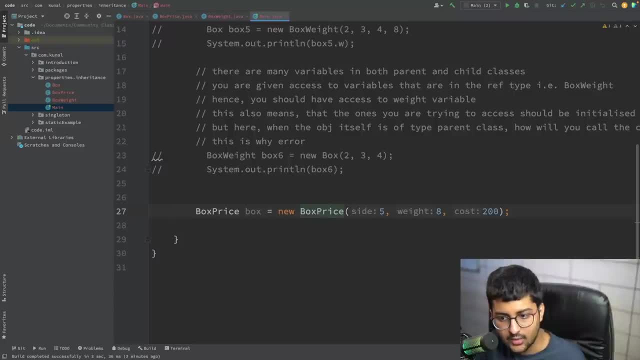 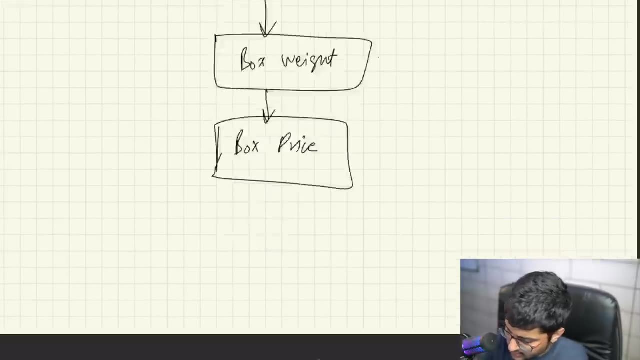 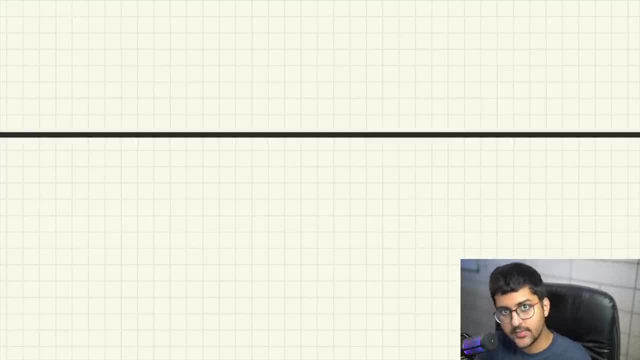 classes, how functions are resolved and everything. that is the next topic in this video. only so make sure you like, share and subscribe. okay, the third one. the third one is third one is what? multiple inheritance? multiple inheritance, okay. so multiple inheritance means when one class is extending more than one. 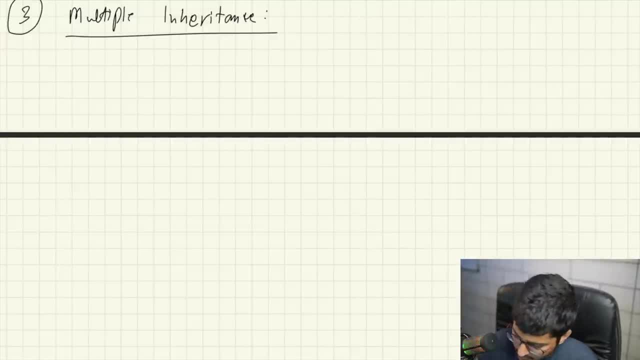 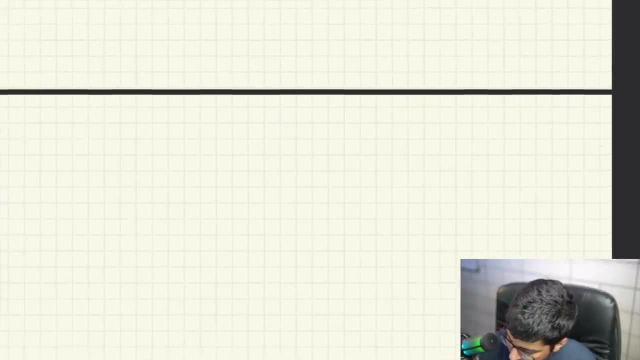 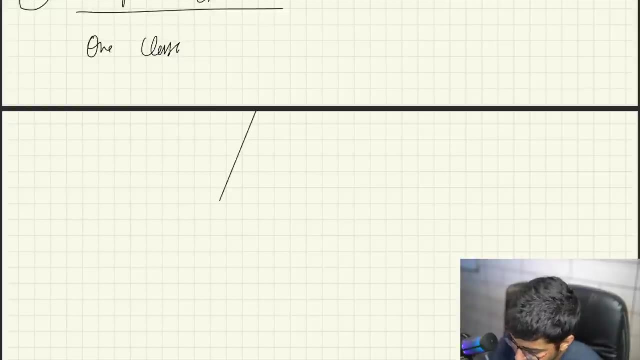 classes. okay. so when one class is extending more than one classes, for example, this is something like this: let's say you have so, for example, one class extending more than one classes, for example, class A, class B, class C. these are both parent classes, so C has access to properties of A also and B also, okay. 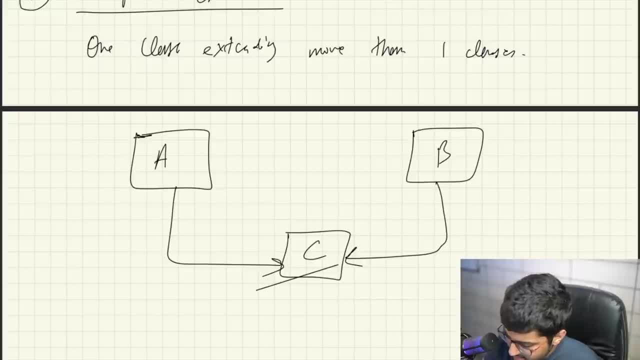 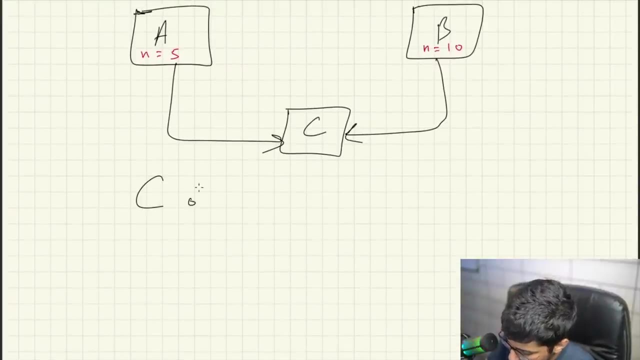 something like that. but imagine that it has a variable called n is equal to 5 and it has a variable of n is equal to 10, for example. okay, now you do something like it's a question for you. now you do something like C object is equal to new. 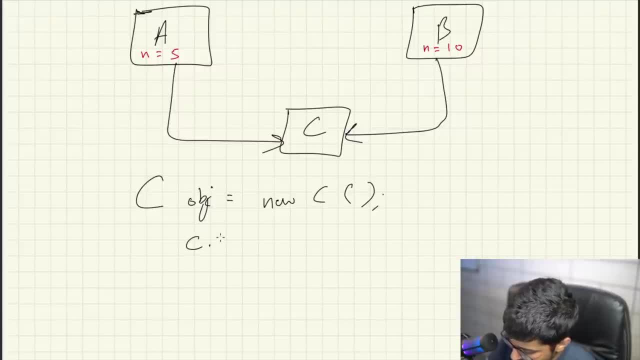 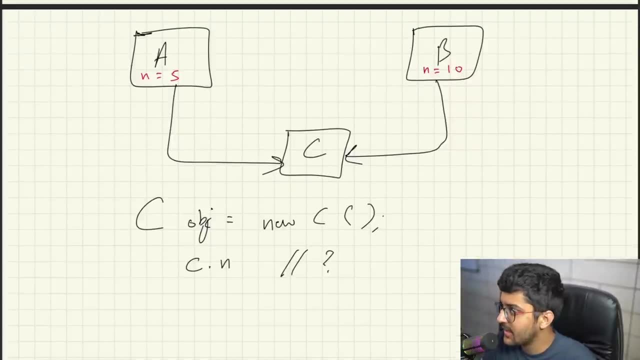 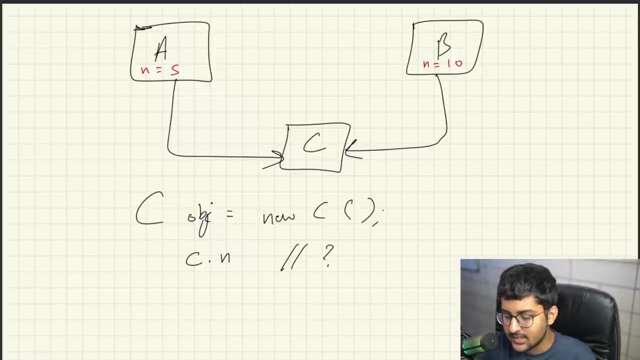 C and then you try to say access C dot n. what will be? the output is only n does not exist over here. okay, then usually it looks for the parent one. is it going to print 5 or is it going to print n? that is the question. that is the question. what is it going to print? so? 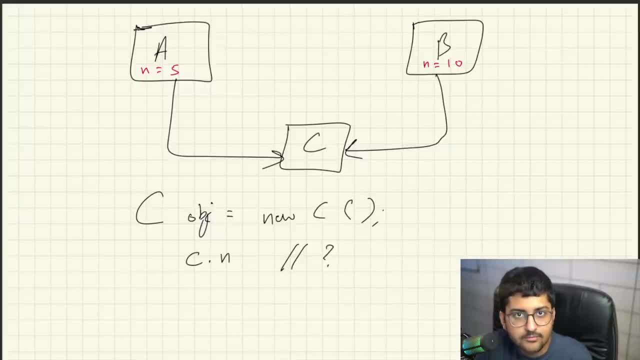 now, here you have a problem, an ambiguity, whatever. it's not able to decide which one to pick. this is why that is. this is why Java does not support this. multiple inherent inheritance is not supported in Java. why? because of this reason, if two or more parent classes have the same variable or something, property, then child class will get confused. 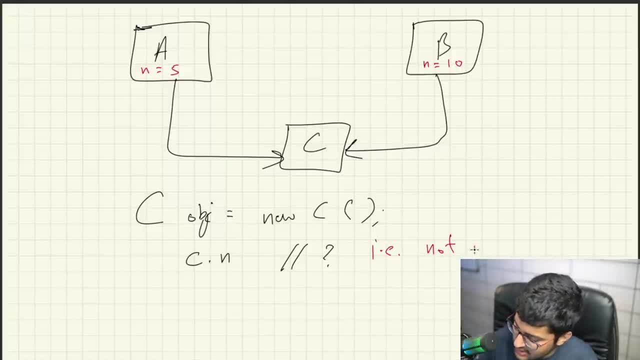 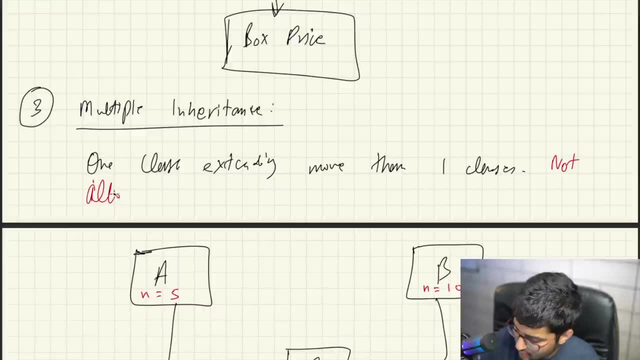 which one to pick. hence, not in Java, okay, not allowed in Java. then you will be like man fine, multiple inheritance is not allowed in Java, no problem. then how will you implement this thing? like there might be some use cases where you might want to access the properties. 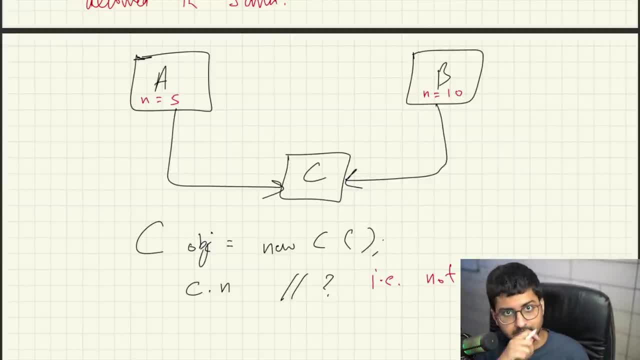 of one or more classes as parent classes might be a possibility for that and you are correctly, you're you're correct. there might be a possibility where you need to create a child class that has one or more than one parent. then how will you do it if multiple inheritance is not supported? 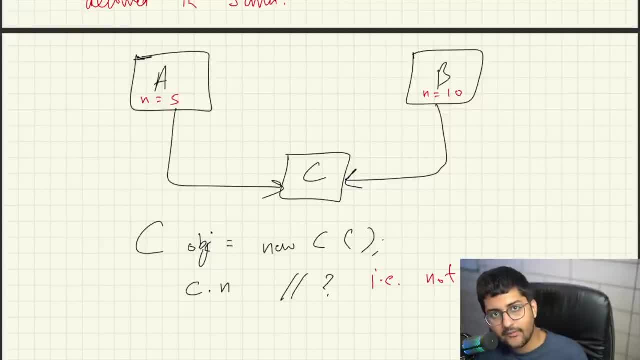 in Java by using something called interfaces. interfaces defines what a class does, not how it like, not how it's actually like, not the values of it, but just like the template for it. values will differ on like. we'll cover it in a separate nice video called abstract. 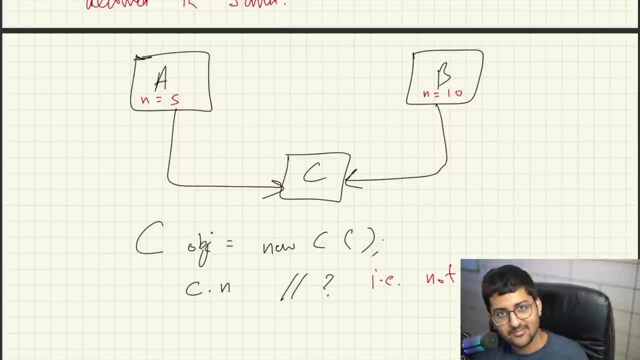 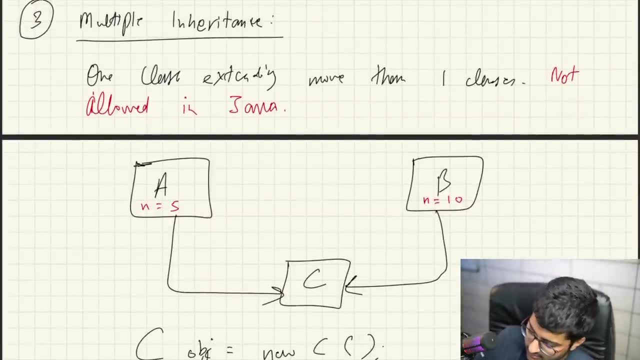 classes and interfaces. okay, that will come later. okay, make sure, like, share and subscribe and follow the object to environment playlist. for now, we will, we can. we will see you in the next video and we will do this in interfaces later on. okay, so that's multiple inheritance. 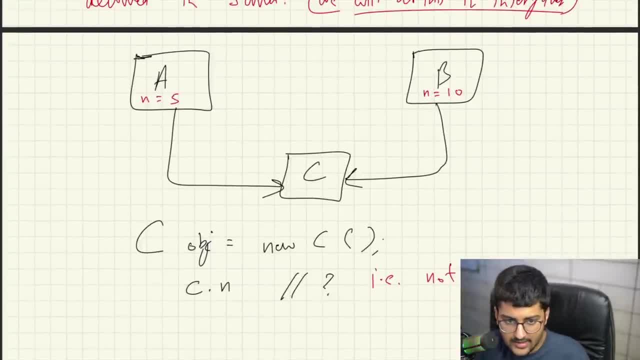 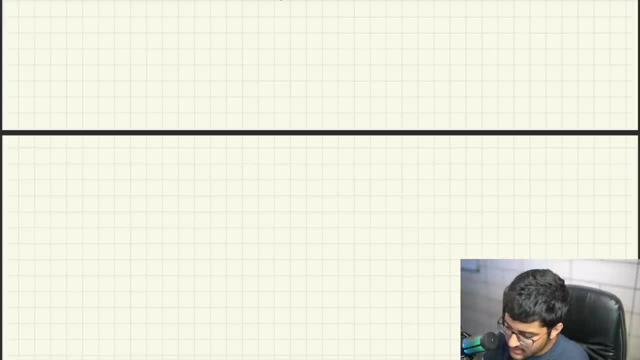 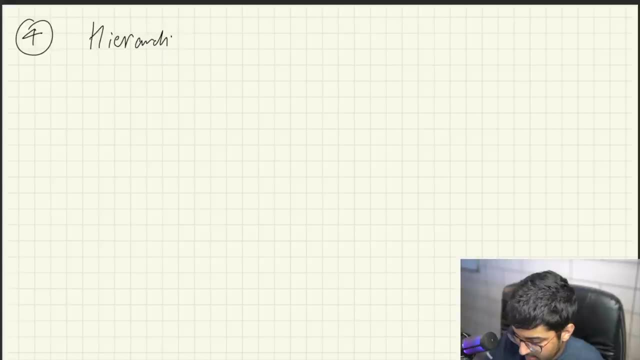 in Java. okay. so multiple inheritance is not really allowed. similarly, there's one more called hierarchical inheritance. this is pretty simple, something like hierarchical inheritance, hierarchical inheritance- this is actually pretty simple, it's exactly the same. all the concepts we apply in the previous one, right same, will apply over here, because nothing. 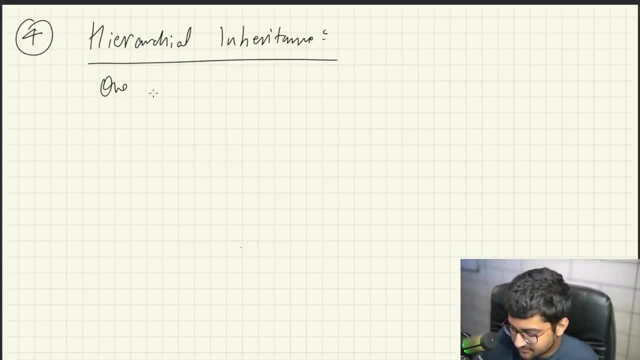 is different. okay, so basically one class is inherited by many classes, so it's exactly the same we did before. no problem: a class over here, b class over here, b, c and d. now you'll be asking Kunal, how is this similar in theory and everything as previous ones. 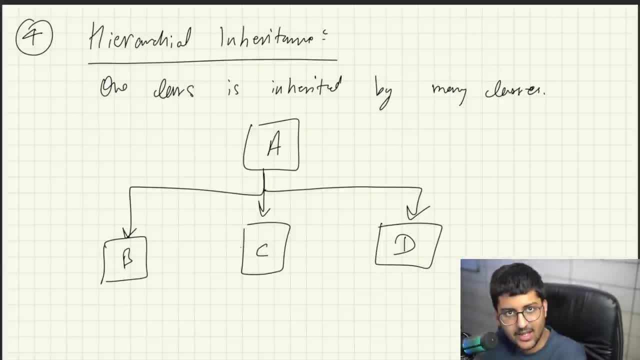 well, all the rules we applied for single level inheritance same apply over here. i told you this: b will have access to all the things above it. so all the things that you are getting above it a, it will have access to those. will it have access to the a stuff in c? no, because 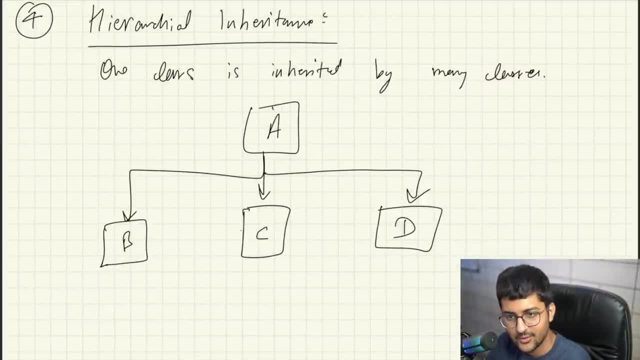 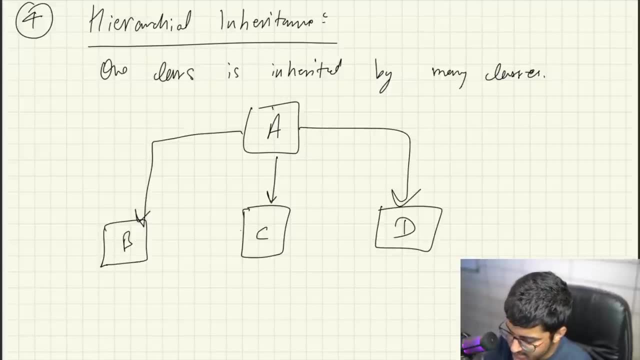 you cannot go up then down right now. what you have to do now is to go to level centre down. okay, so it's not actually like this is actually like this. you can't really say go up then down, no, it only be accessing from above it and from below. 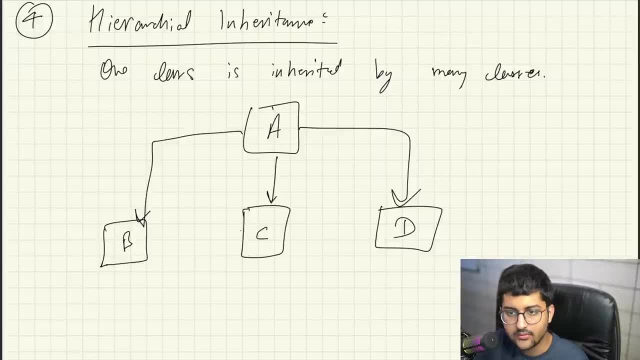 it will have no access. okay, very simple, you can definitely do it, just do, just make multiple classes, just do, you know, make multiple classes and just do extends to it, that's it no problem in this. create another class: class a extends box. class B extends box plus C extends box, box color, whatever you can. 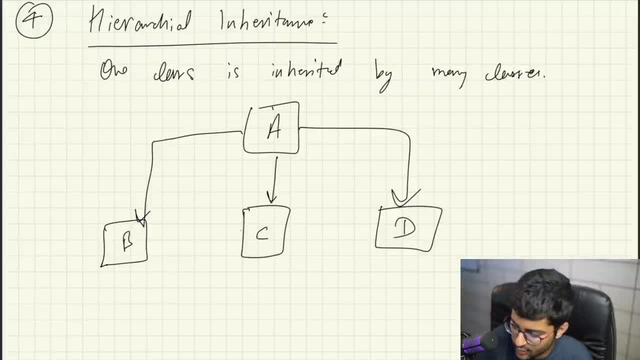 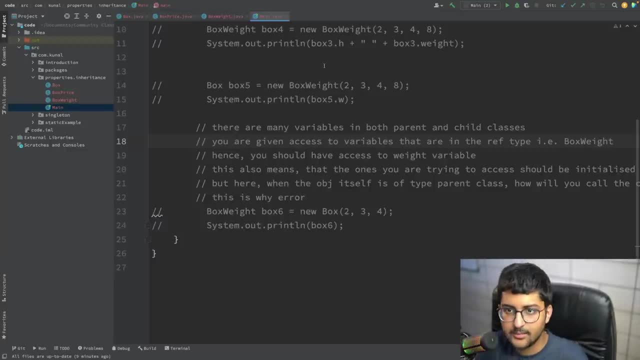 make no worries in that I can show you, if you want, okay, an example of this thing. it's actually very simple. an example for this can be something like this: box is being inherited by box price. a box with box price or box price is being inherited by box weight. 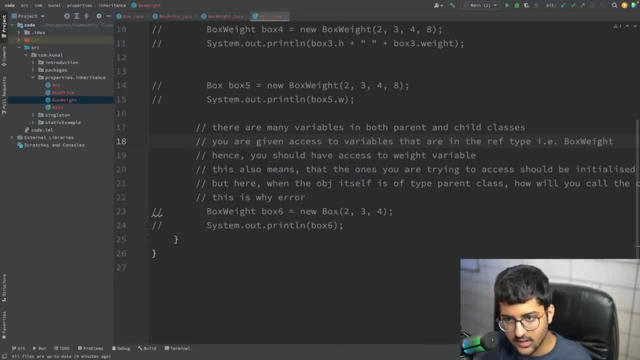 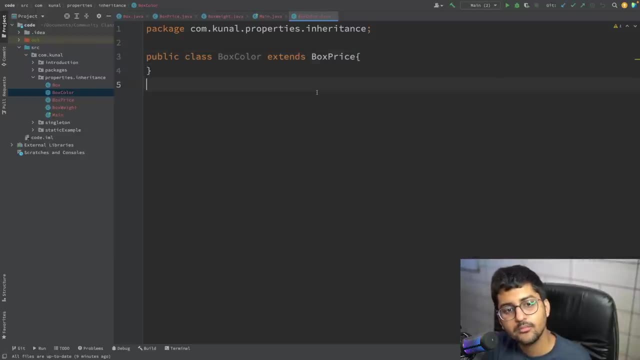 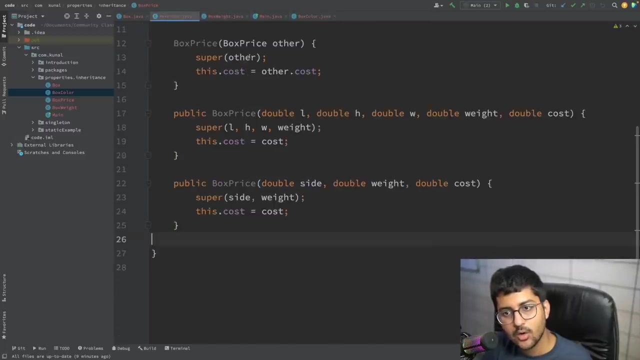 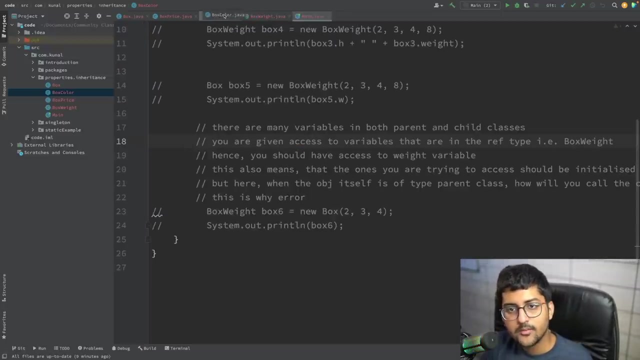 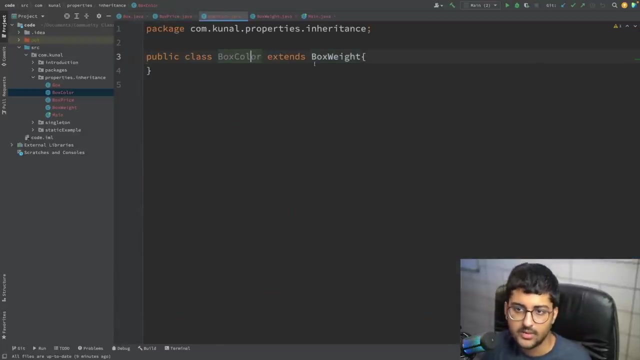 I can make one more: box color extends box price, no problem, okay, so box weight also extends- sorry box, not box price, box weight. okay, so box price also extends box weight. box color also extends box weight. all the theme is going to be applied and simple stuff will be available over here as well. 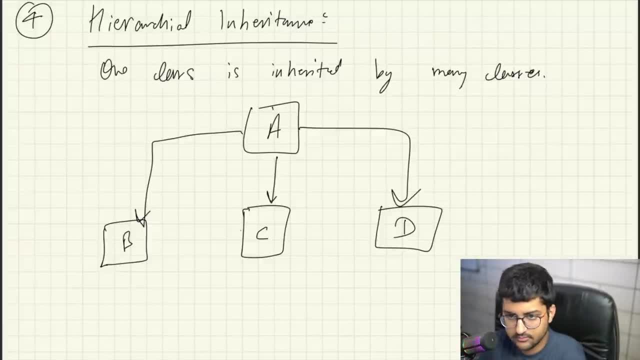 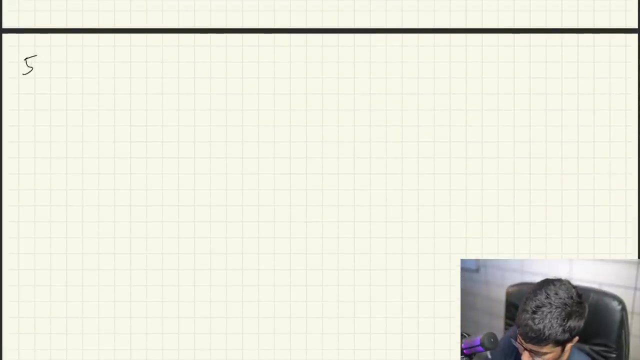 okay, that is it. okay. extending box weight. this is also extending box weight, no problem in this. okay, let's move forward. there is one more, which is known as fifth one: hybrid inheritance. what does it mean by hybrid inheritance? so, hybrid basically means that a combination. it is a combination of single and multiple inheritance. single and multiple. 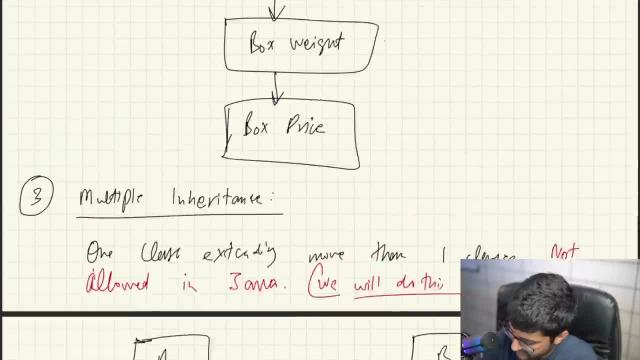 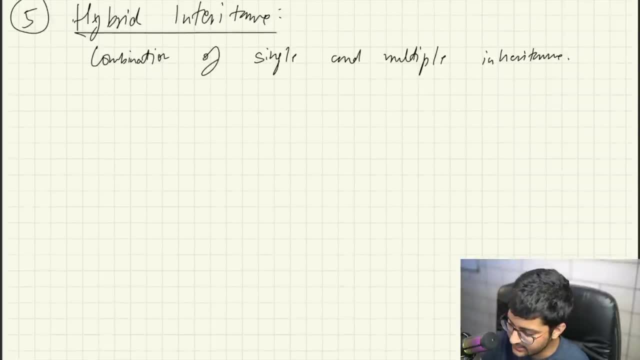 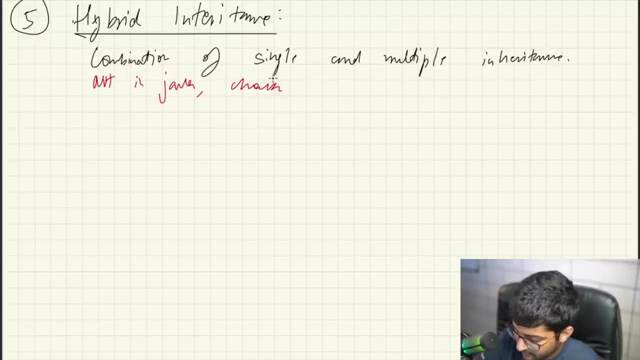 inheritance and in, since in java we don't have a multiple inheritance. similarly, we don't have hybrid inheritance either, because it consists of multiple inheritance. right, so not in java. check interfaces, lecture: okay, in interface, we'll try to do all these things. so yeah, single level stuff like this- a, b, c, it's just like some single single level or like. 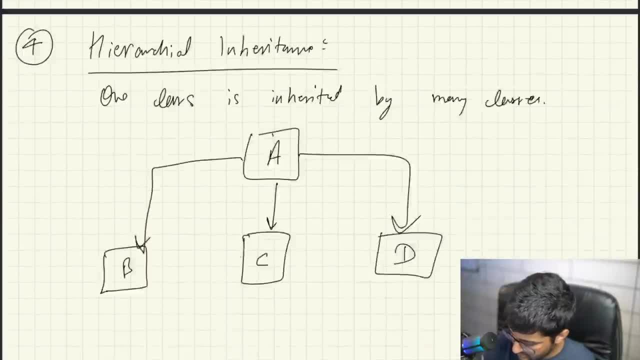 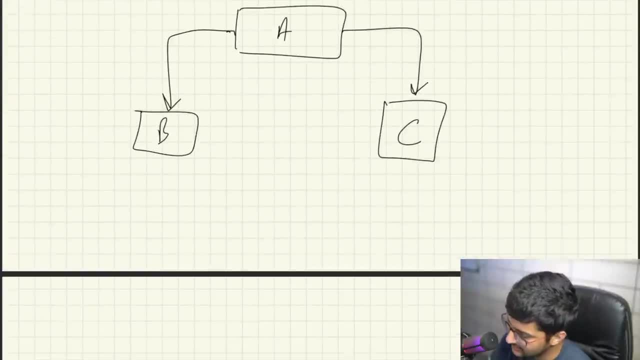 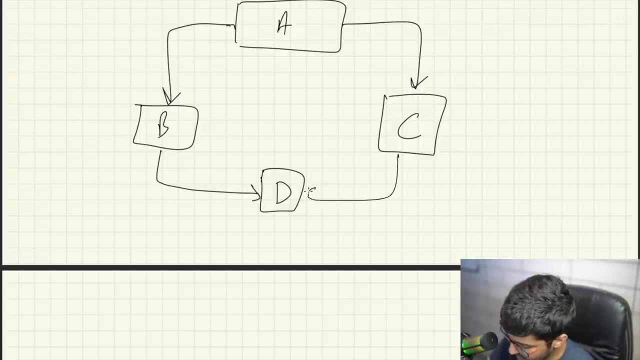 your, uh, you know, your, your, this one, like the hierarchical one or single one. the rules for both are same and uh, so this is one single level, this is another single level and multi level means these two are doing for d, multiple, multiple inheritance. this combination of these two is called hybrid inheritance, so the combination is known as higher hybrid. 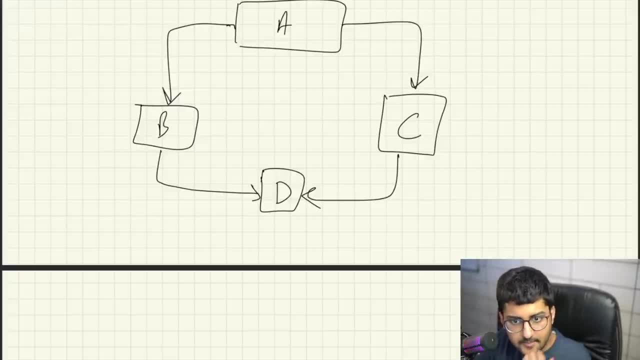 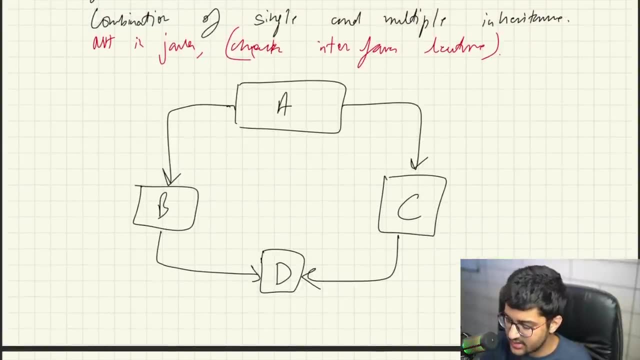 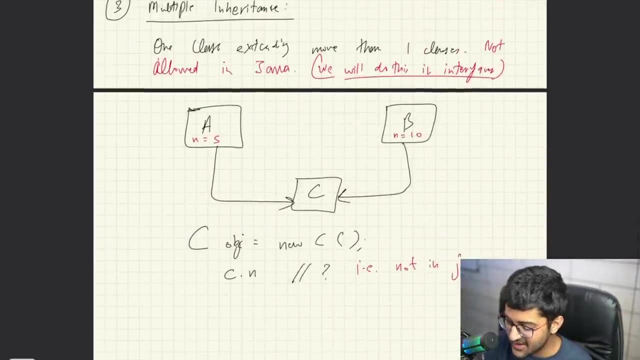 hybrid inheritance. okay, so java does not support this. okay, but we can use these things using uh, interfaces. we can use these properties and stuff in interfaces, like we can achieve this sort of a functionality using interfaces. that we'll do in the interfaces lecture later on. okay, that was the first property of object related programming inheritance. pretty cool. the video of inheritance handle is the last one. it's already done, but i will share the links as well, so you can do the same. this is the first step of the project word. imagine this to get all the possible properties of object related programming, ie for every object. 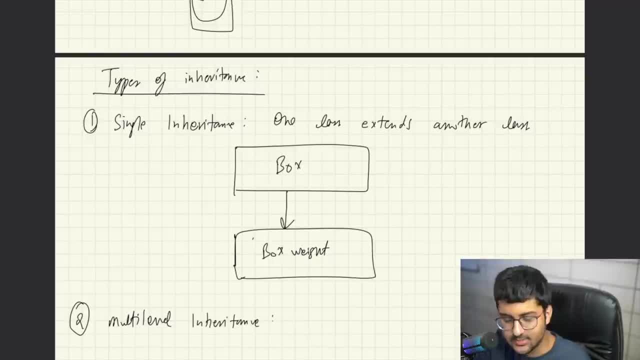 so this is an example of first time property, of object related programming in heritage. okay, so the first inheritance not over. i will cover it after the next property as well. about some two properties like combining each other, we'll cover those concepts as well. everything will be done in. 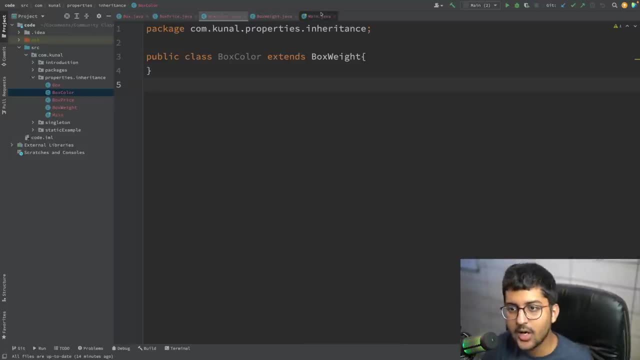 this video only okay, so make sure you like, share and subscribe. okay, but you can't do something like this. um, you, you can't inherit from inherit like what? what is this, you know? uh, you can't like. this is cyclic inheritance, right? so you basically box car is inheriting itself. that is it, like that? 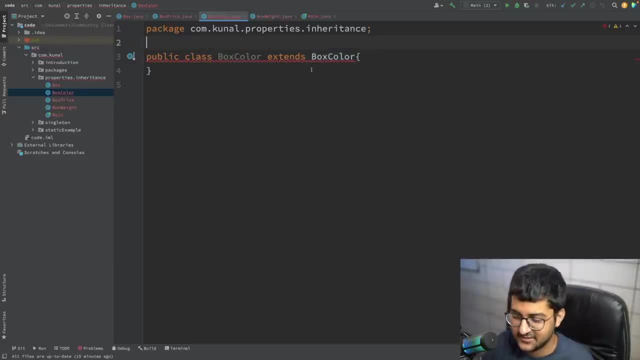 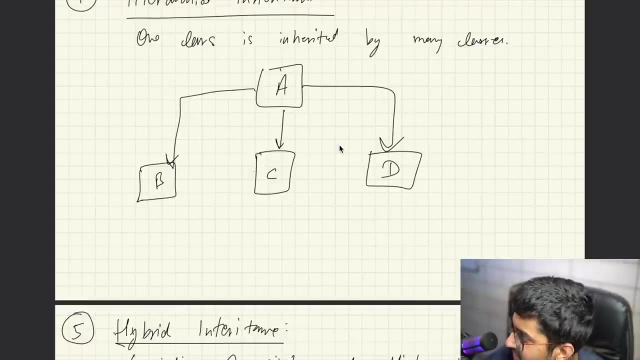 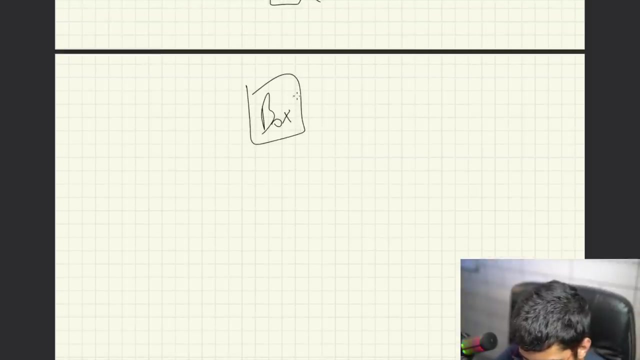 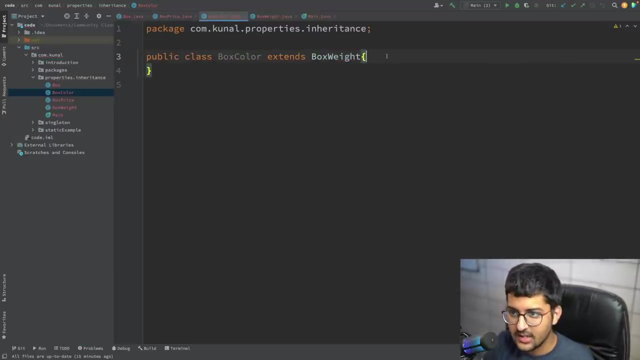 then this is inheriting itself. inheriting itself, okay. so something. uh, you're doing something like this, so you're doing something like this, like this: not allowed, okay, can't inherit. a class cannot be its own super class is basically what i'm saying: okay, so don't do that. so that was about inheritance, but we'll cover, obviously, a little bit more. 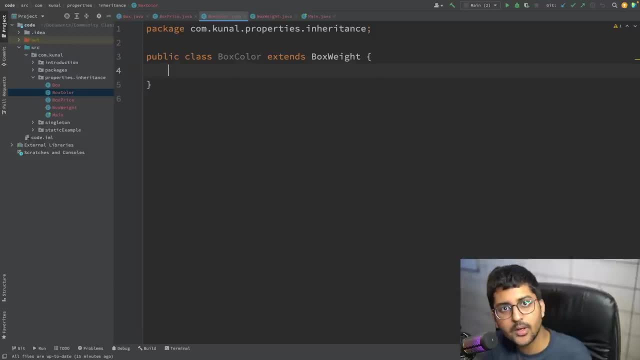 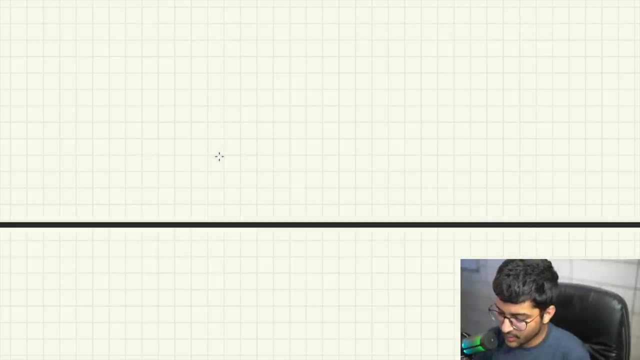 advanced stuff in this video only. but um, let's move forward to very important topic. second property of objective programming: polymorphism. some important points over here. so polymorphism, first of all, what it is. so second property of objective programming is polymorphism. okay, what is it? what does this word mean first of all? so when we talk about polymorphism, 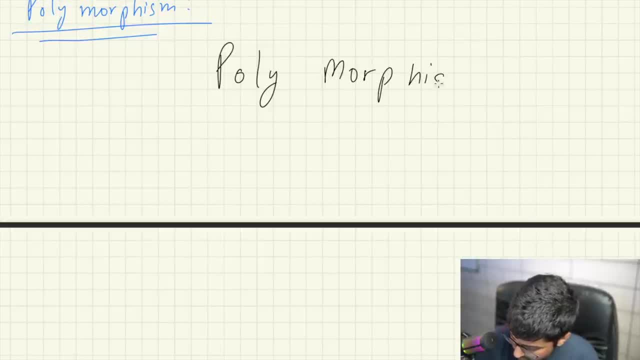 poly means many and morphism means ways to represent- represent. so polymorphism means many ways to represent a single entity or item. so polymorphism means many ways to represent a single entity or item. so polymorphism means many ways to represent a single entity or item. that is as simple as it can be. 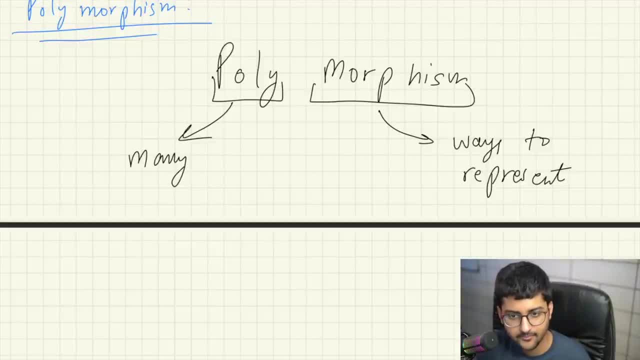 okay, all right, cool. okay. that's polymorphism in simple terms, but in terms of like java and stuff. i'll definitely tell you more about it. so this is like. these are greek words, by the way. okay, so it's very, very important um to understand, like, what it means. so sometimes it maybe happened. 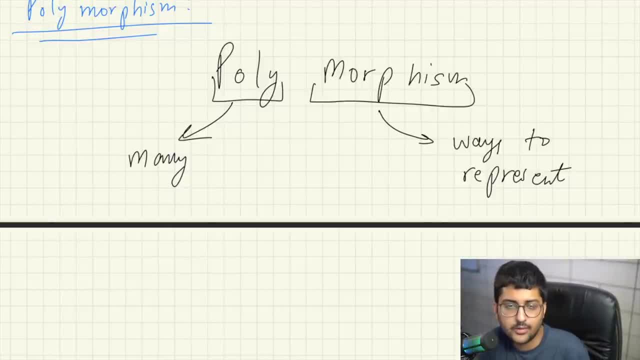 that you know a task is uh performed. you know like uh as a single action, but but in different ways. for example: okay, so any language that does not support polymorphism. we cannot refer to that as like: okay, this is an object-oriented language or whatever. okay, but they are instead known as object. 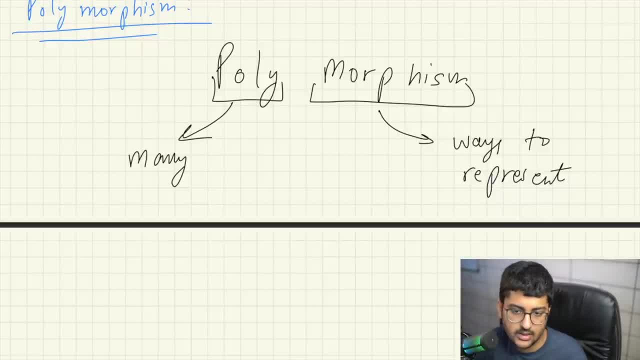 basis languages. ada, for example, is- uh, you know, for example, but java supports polymorphism, so we can say it's object-oriented language. so we can say it's object-oriented language, okay, when does it occur? it occurs during inheritance. okay, because there are many classes that are relating to each other. so let's talk a bit more. 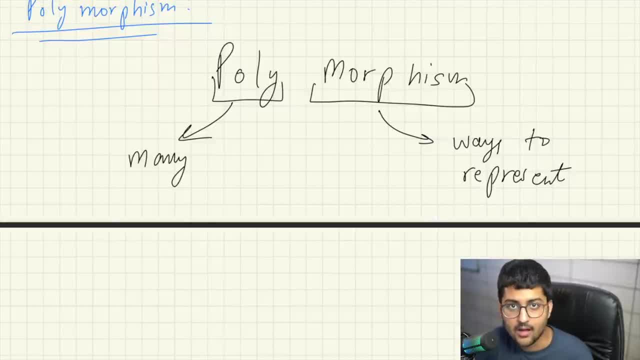 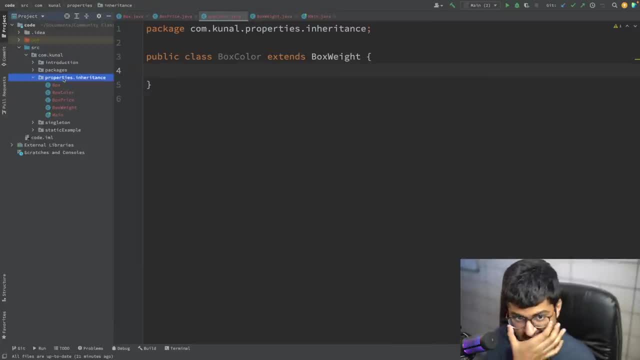 about it like how it actually occurs. okay, let's give an example, real world example. so another real world example. let's take, let me um, let me create another package for you, known as polymorphism. let me close. all start afresh. let's say i create a class called shapes. 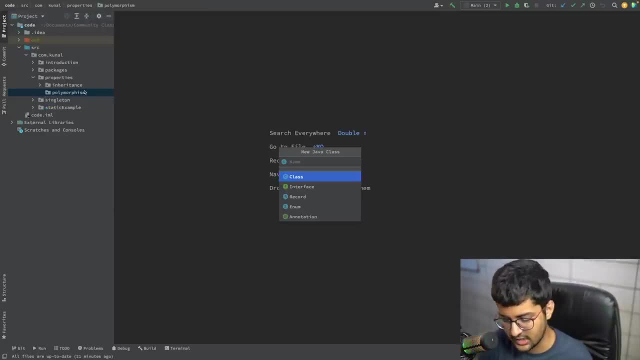 okay, shapes class, something like that. okay. and let's say we create, uh, so many other classes of subclasses of shapes. so, example: we can create a circle. okay, extends shape, no problem. okay, the attention is that this one is my, is my subject, so let's say that this one looks like that, okay, 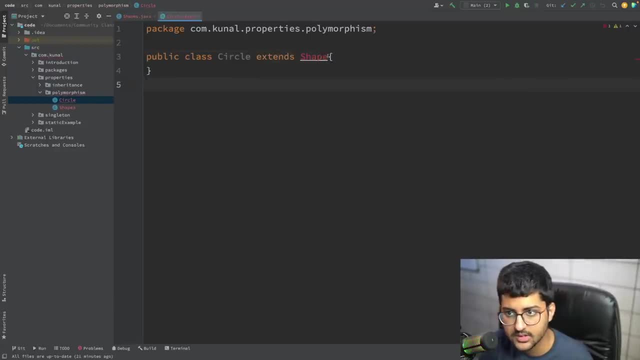 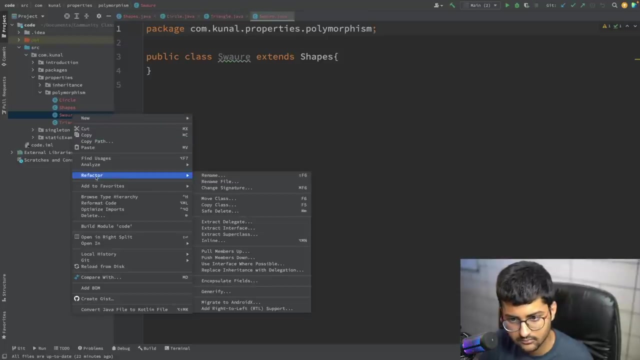 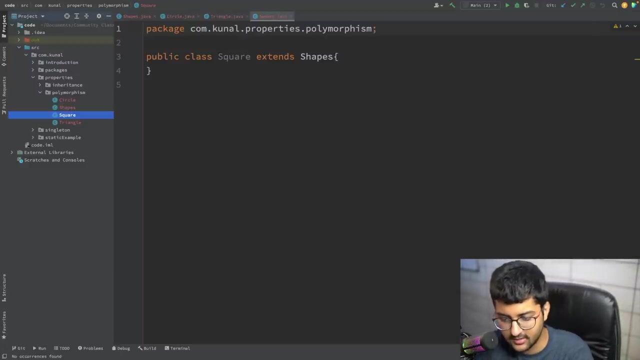 okay, circle, extend shapes. we can create one more called, let's say, triangle. okay, we can create square, okay. so this is like shape is being inherited by many, so this is hierarchical, right. so there's another nice example for hierarchical inheritance. you can create one more. we think square is fine, okay, no problem. so shapes, that's cool. I. 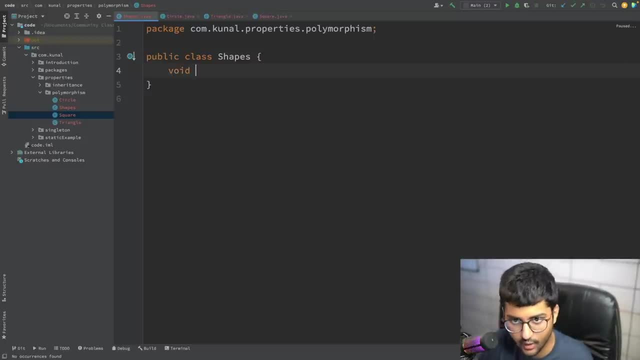 can create a, I can create a function over here. I can say void area or something like that. I am in shapes, okay, something like that. for circle. it will also have, let's say, an area, something like this, something this will also have and this will also have it. so it will be like area is. 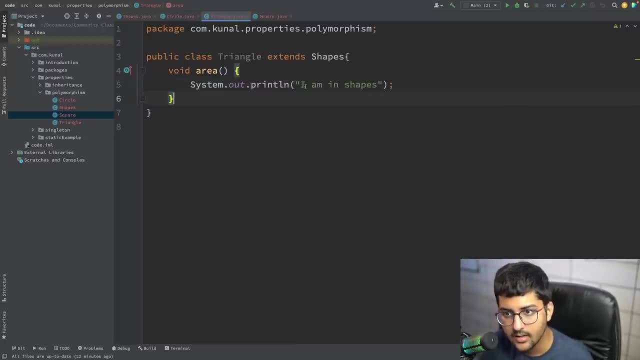 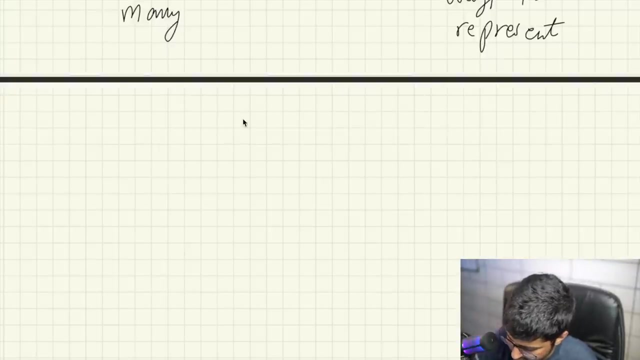 square of side here will be like: area is 0.5 into height, into base, or something like that. circle area is pi into R, into R or something like that. okay, so if I draw it like over here, this is a shapes class, this has some area area method like this, okay. and here we have, let's say, triangle. 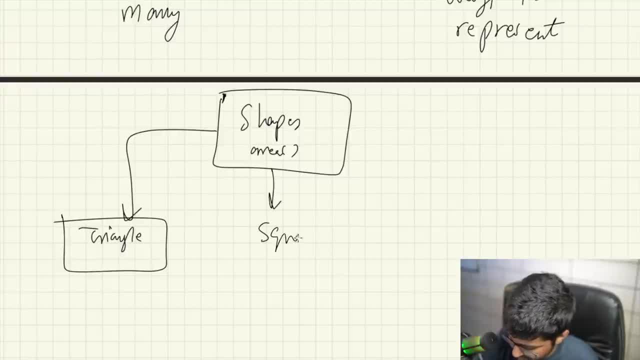 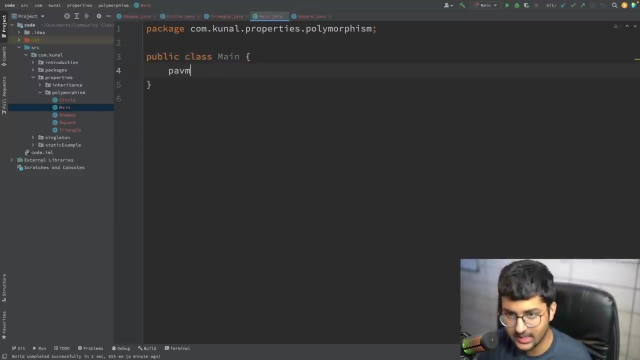 this also has its own square circle. okay, they all have its. have their own, let's say, representation of area. obviously, so let's see how it works. like you know, when I actually try to call it so, I'll create a main function, a main class. I'll say public, static void main. 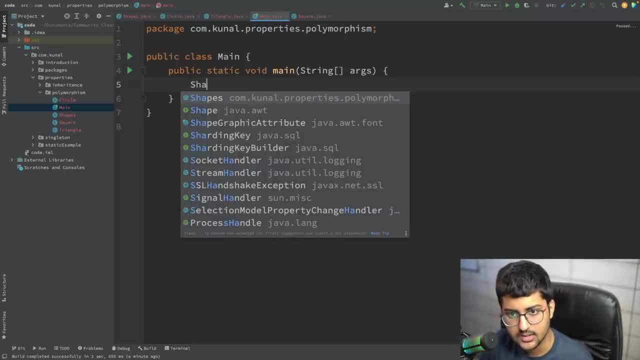 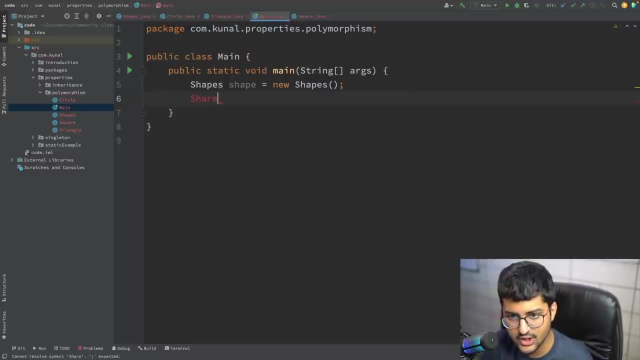 and I create an object of, let's say, type shapes. so let's say shape, shape is equal to new shapes. then I say shape not, not shape. I say circle, circle is equal to new circle. then I say square, square is equal to new square, square is equal to new square. let's just ignore triangle for now, because we already have. 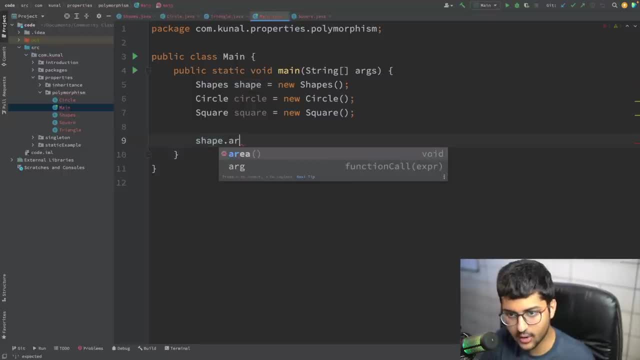 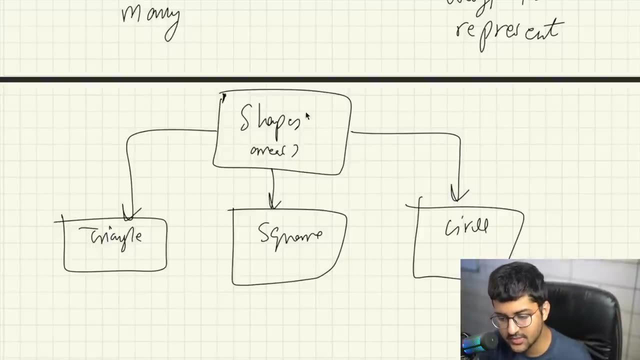 quite a few. what will happen if I say shape dot area? it will be like, hey, does area exist in the shapes one? it's gonna be like: yeah, it does, because I told you before what variables it has access to depends on the type of the reference variable type here is shapes. it will like the shapes have. 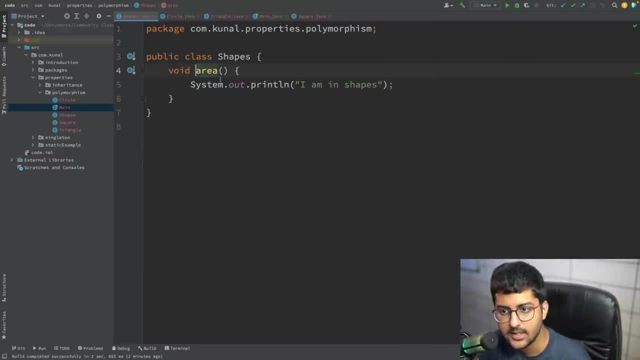 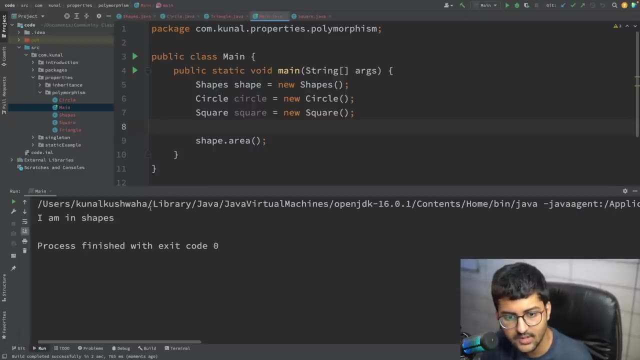 area. yes, it does no problem, it does. it will hence called I am in shapes, let's try to see. let's try to see that I am in shapes. similarly, if I called circle dot area, it's gonna be like: this area exist in circles. it's gonna be like: 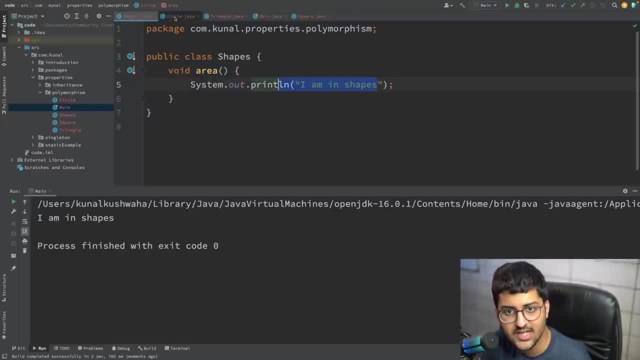 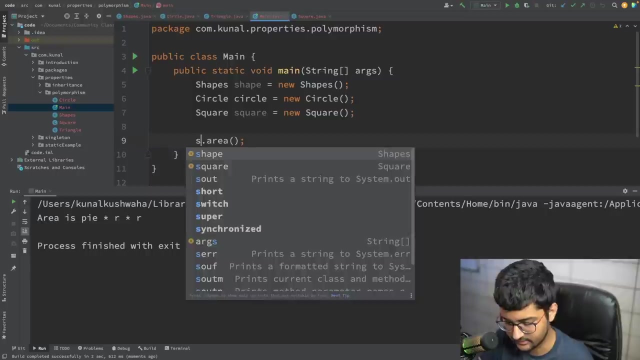 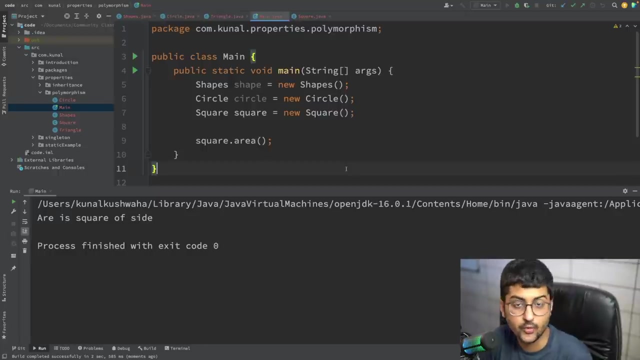 yeah, it does. you can see exactly the definition of function is same in everything: void area, void area, void area. so the definition is same. let me just print it again. there you go. area is pi r squared squares area. i'll go into the technical deep dive of this as well, don't worry. please don't miss this video. 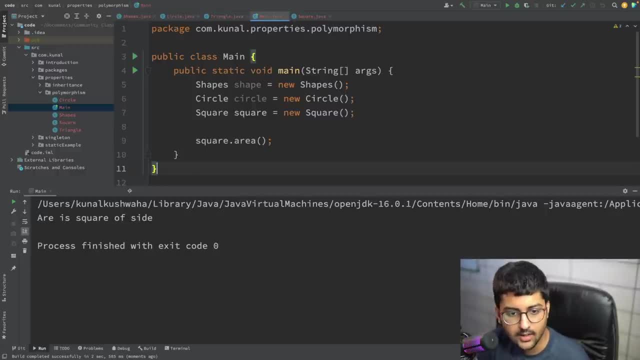 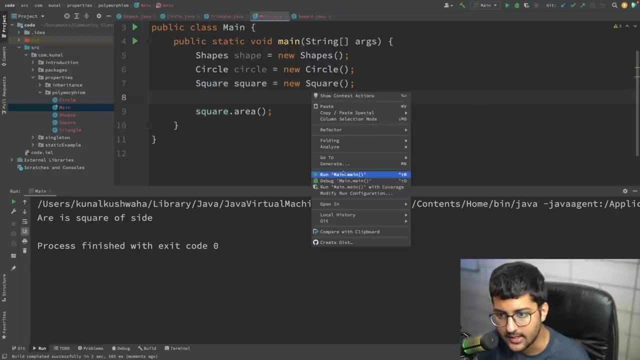 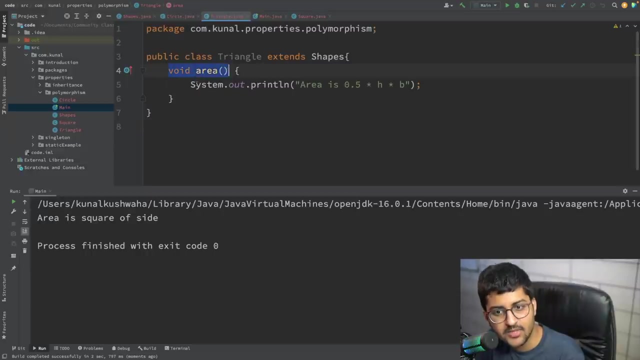 the very. i will go into very technical details. okay. so area or r, it says r. i can just say area in the square. i can say area is equal to, or whatever. okay, you get the idea. area is side square of the polymorphism act of representing the same thing in multiple ways, multiple ways. 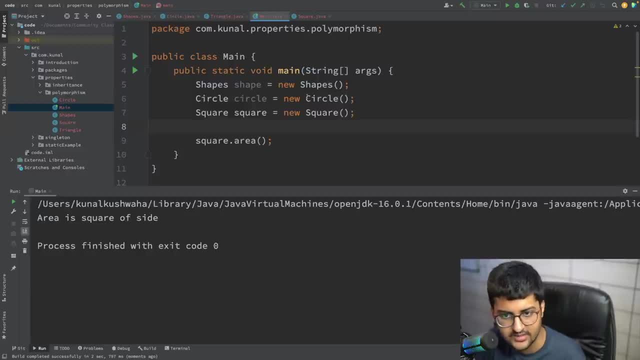 polymorphism, how it works internally, how it's calling specific ones. i will tell you later on. for example, i have the. this has shapes, okay, and the object is of type square, but the reference variable is type of the parent class. obviously, what? what will it have? what will it have it have access to? 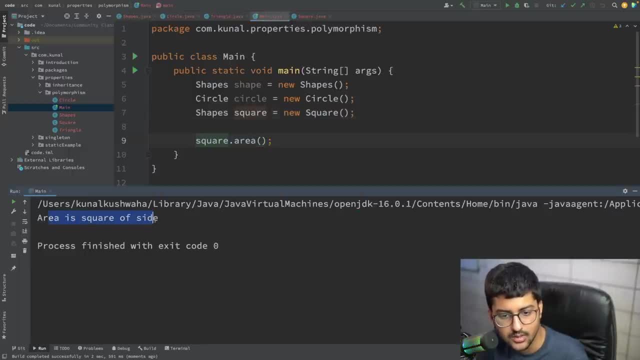 now over here you can see it has access to this particular one, the one in the object. cool, but how? how is this thingy working internally? you're gonna like kunal. this is shapes, so you should have like a shape for you know, like this one type. right, but why is it still calling the square one? 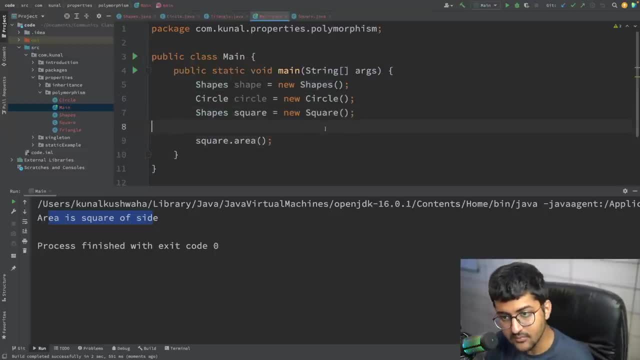 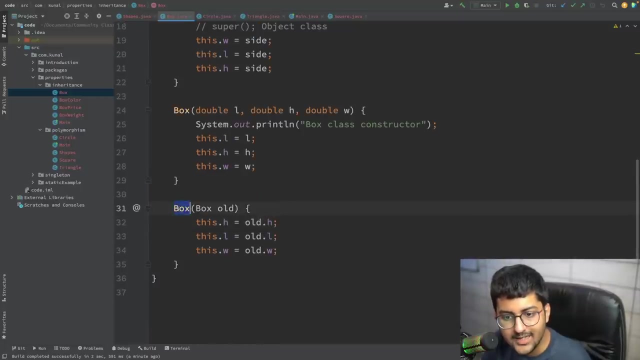 how is that working? let's see. so let's now look into the technical details of this so you are able to understand how it's working internally, okay, what it actually means and what. what are these things okay? one more thing i want to share with you is um over here, i created multiple 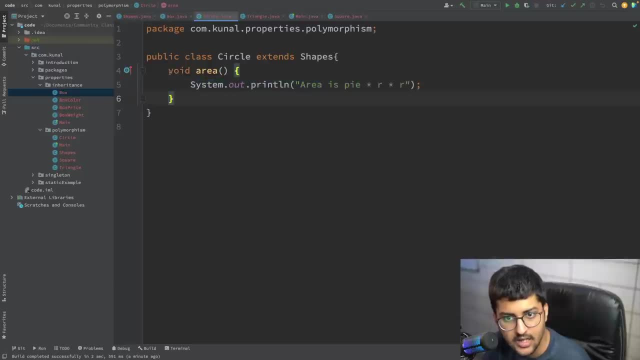 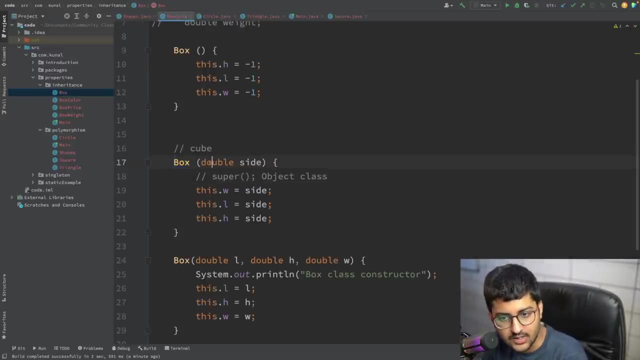 this is also a second type of polymorphism. this is first type of polymorphism, where the exact like the definition is same and here the definition is different. so, example: i can create a constructor that takes a double side. i can create a constructor that takes three things. i can create a constructor that takes 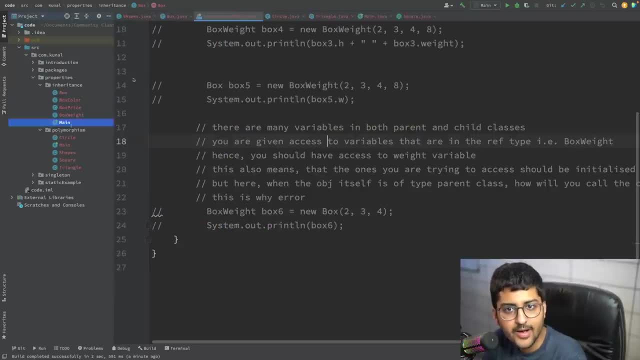 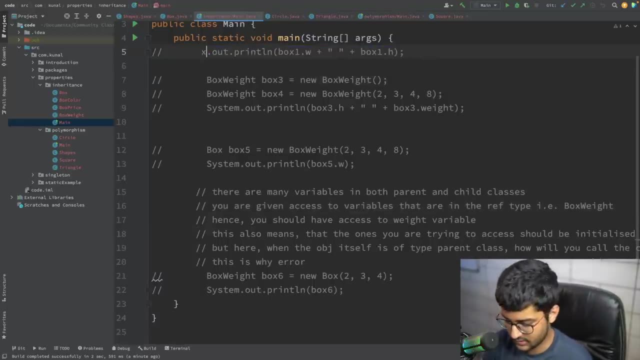 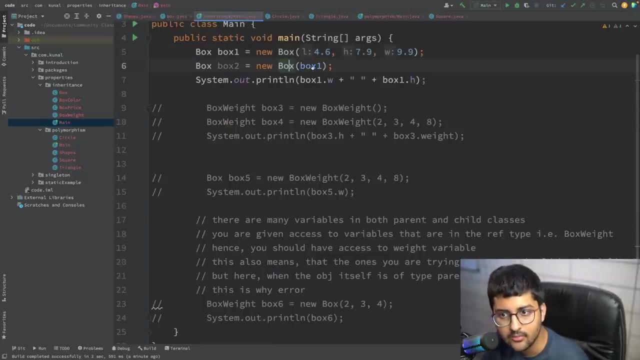 one object and automatically when i call the main function, automatically it will determine that, okay, i have to call the three part one whenever i run this, automatically it will know that i have to call this one here if i am calling the with the another object, automatically it will. 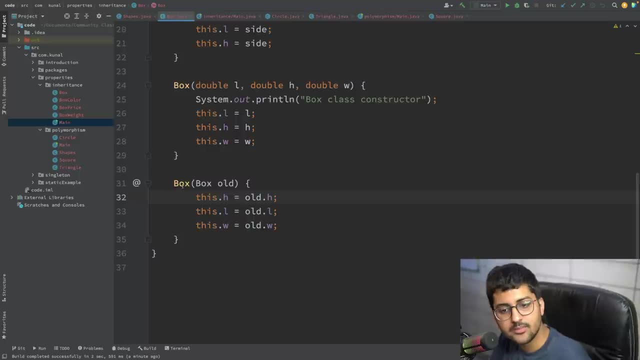 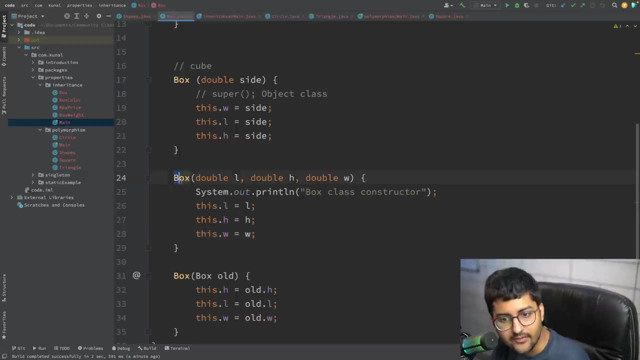 know i have to call this constructor. so this is also polymorphism: act of representing the same thing in multiple ways. here just the body was different, here the actual definition is different. now it's time to look into the technical details of what these things are and all the terms and 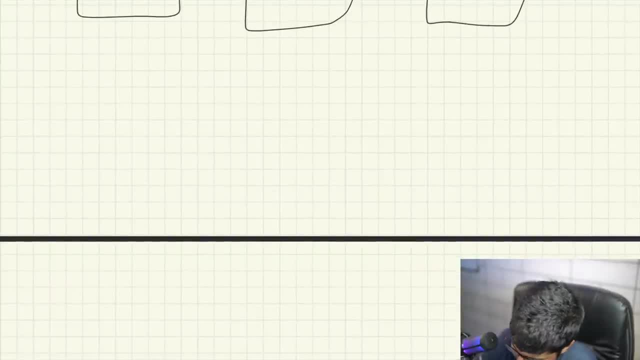 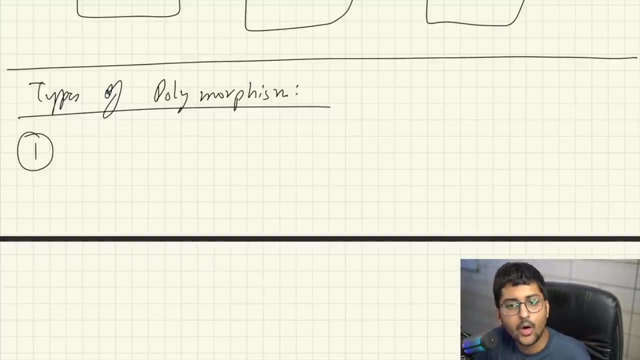 everything collectively. so types of polymorphism: we we informally we took took a look at two types right now, but let's look at it formally. types of polymorphism. types of polymorphism: type number one. type number one is known as what type? number one is known as compile time. 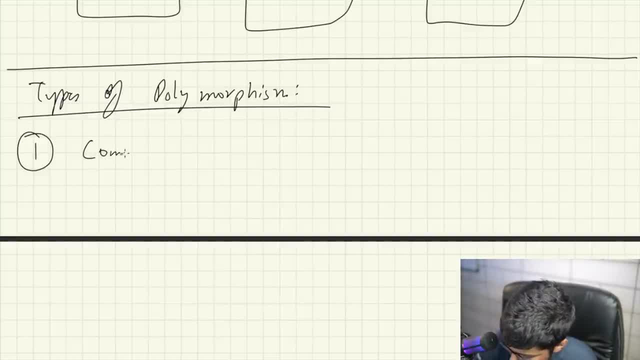 polymorphism. polymorphism, it's known as compile time or static polymorphism. okay, this is achieved via method overloading. okay, it can also be achieved by operator overloading. but uh, in java they don't provide us operator overloading. okay, what is method overloading? method overloading is when a 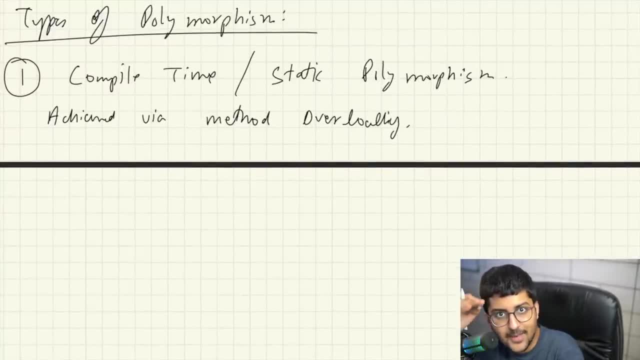 has multiple methods with the same name, but the number and the type and the order of, like the parameters and the return type can be different. okay, method overloading is what method overloading is? mimic maverick, the classic method overloading loading is something like this: method overloading means same name of method, same name but types. 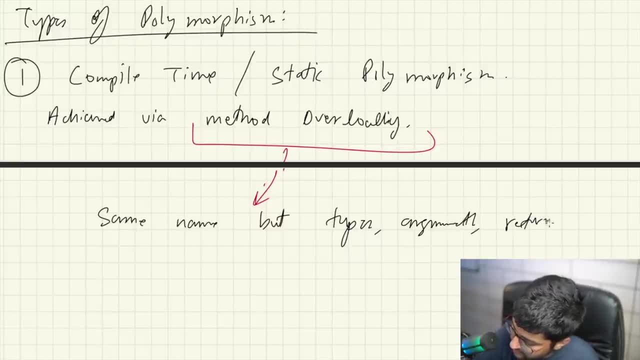 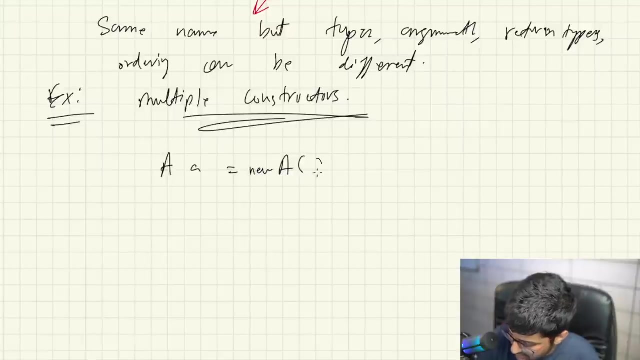 arguments like return types and etc. not etc. i can just put like the one other one as well, like ordering can be different. example: multiple constructors, multiple constructors. when you say something like a- a is equal to new a, then you say something like a a 2 is equal to new a, 3 comma 4, something like this: 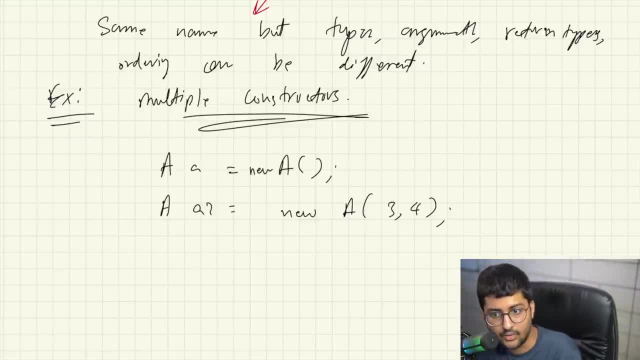 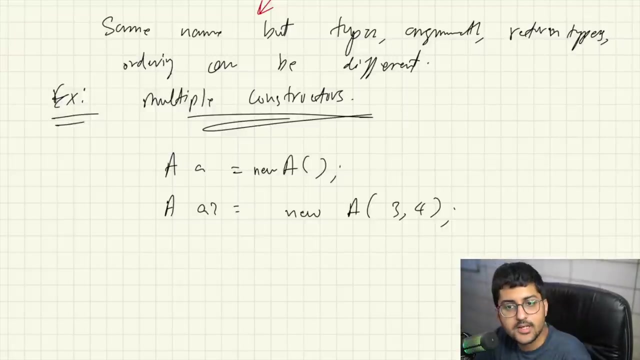 this is known as compile time polymorphism- method overloading- okay, so why is it known as compile time or static algorithm, static polymorphism? what might be the reason for that? the reason is that. what is the reason? the reason is that it java determines which constructor or method will be called at compile time in compile time polymorphism. okay, so we. 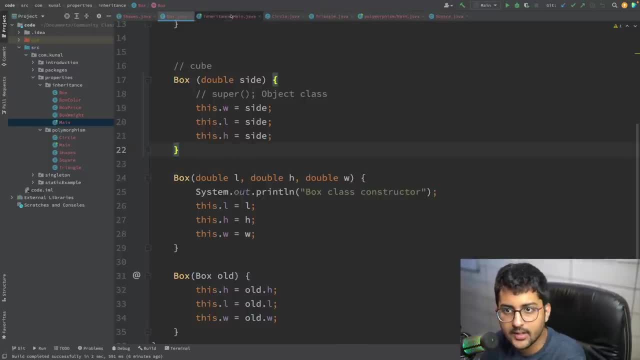 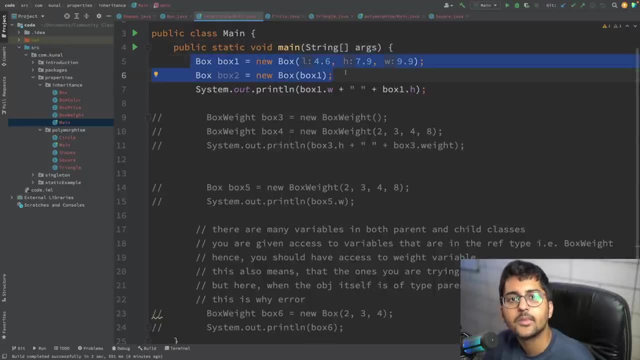 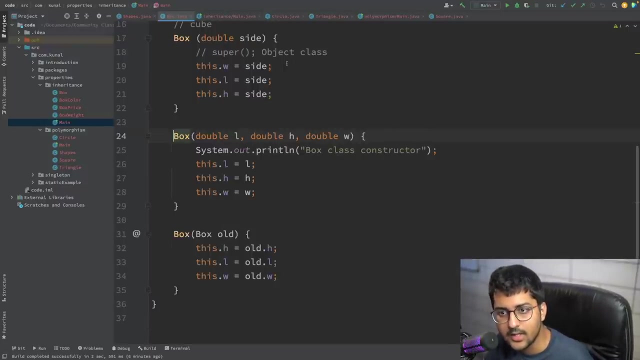 actually did an example of this as well. so over here in the box main this: this is compile time polymorphism, this thing at compile time. when it's compiling, it will be like: okay, uh, which one do i need to call? it will be like, hey, you need to actually call this one at compile time. it will look like: look for that. 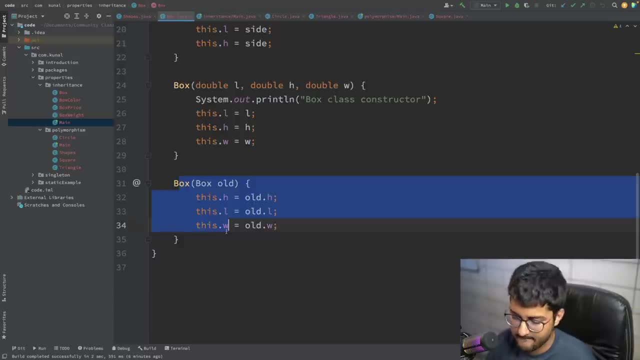 which constructor do i need to call this one? do you need to call this one at compile time? it will look like this: so here you use compile time and this will look like a compile time. uh, i'm just gonna tell you this here. do you have any idea what this FREEDOM is? 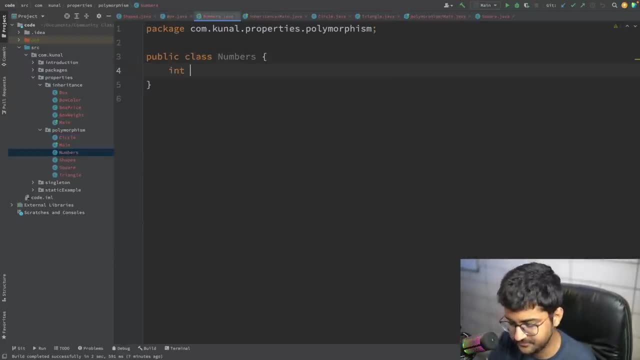 i'm gonna tell you that this is a function that is used in the, our libfile. so make sure we're looking in the libfile. so we are going to search for a file in the libfile, let's say, let's say, let's say step 2. 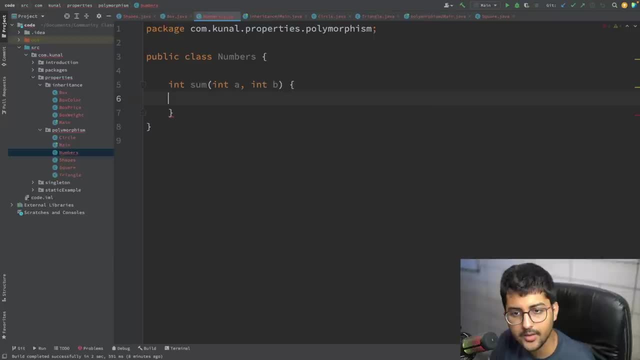 let's say, let's say some kind of a file, i can add some kind of a file, i can add a file, so that is step 2, so i can add that 2, because step 2 is whenever you want to. or you can add some kind of a file. 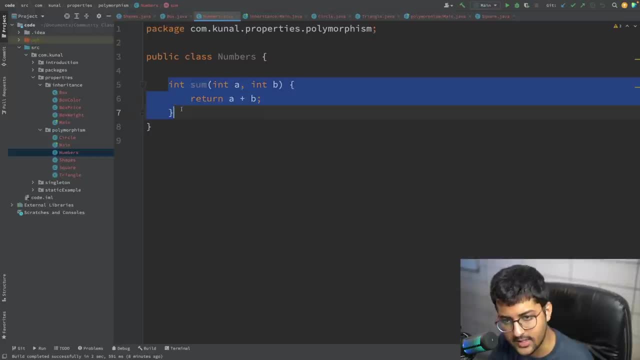 a plus b, i can do. method overloading means i can do method overloading like this. now the error is gone. if the name is same, then the number of arguments, or like the return type or the order, should be different. now don't say like something like this: kunal, can this work? 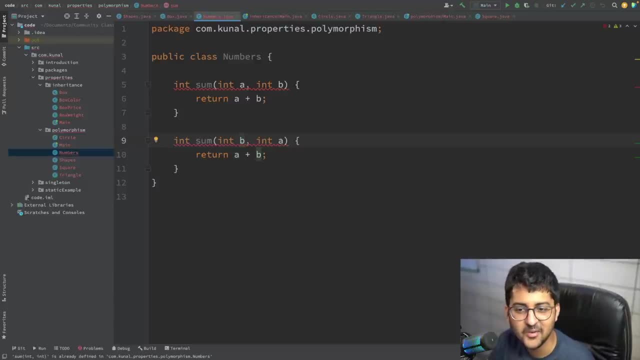 no order by order. i mean, if this is something like string b, this is something like string, this is like void, this is sorry, this is like something like let's say nothing. void, this works. order should. order of the type should be different. okay, order of the type. 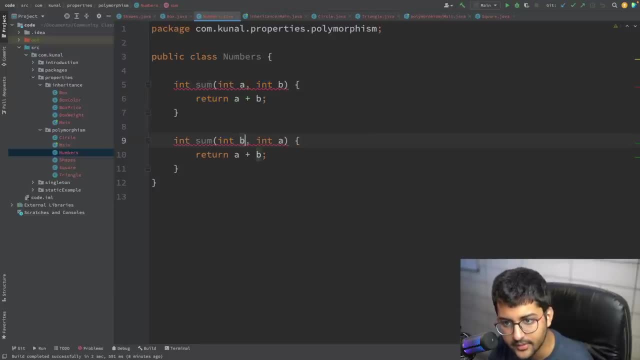 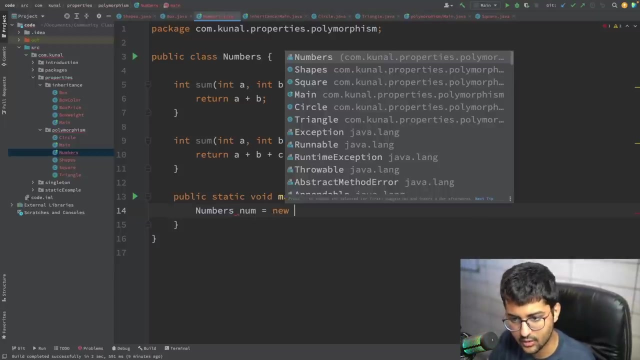 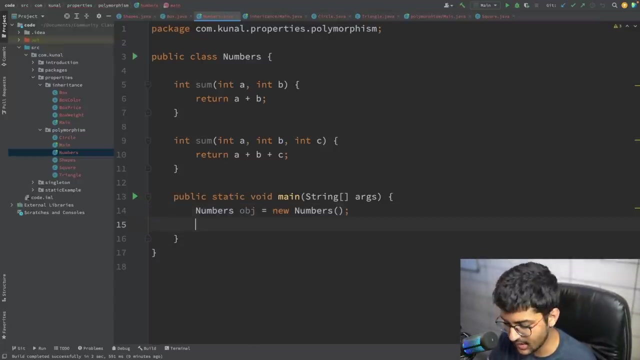 okay, moving forward. int a plus b plus c, no problem, i'm just going to say over here, public, over here also i can see public, static void mean i'm going to say numbers, number is equal to new numbers. or i can just say object. okay, now, now you will understand. object dot sum. i'm just going to say 2,3. 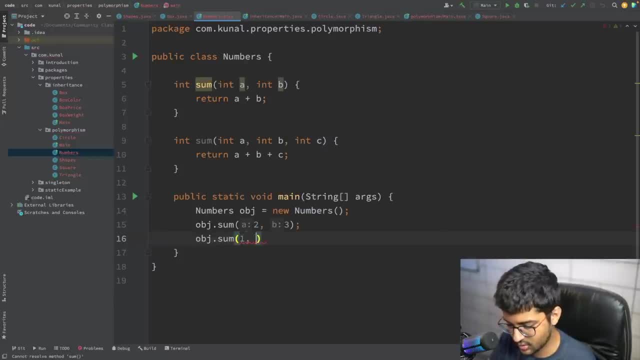 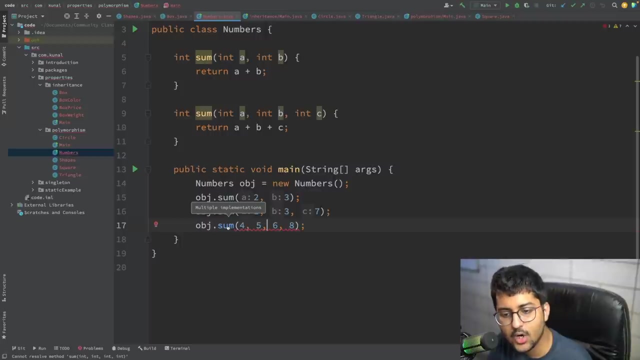 and object dot sum 1,3,7 and object dot sum sum 4,, 5,, 6,, 8. this is giving me an error because there is not a function sum in object in the numbers class. that takes 4 arguments. ok, so at. 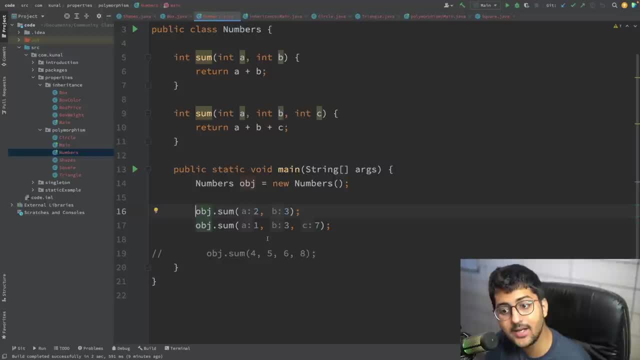 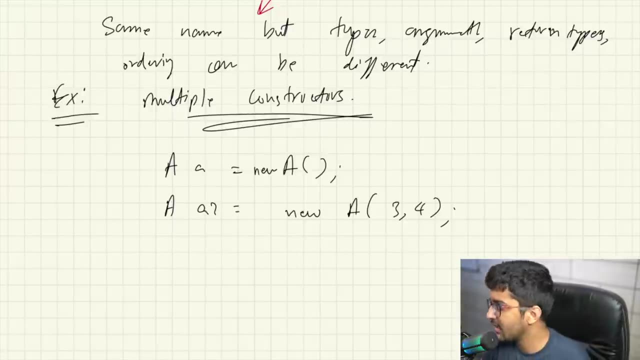 run time. it's gonna be like: hey, you are trying to. you know when I'm talking about, like the compile time, polymorphism. so over here you can see that the constructor and everything that is memory being created. this is actually happening at run time, but at compile time only. it will give you an 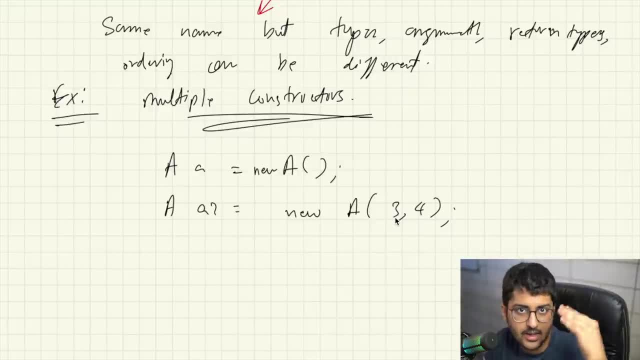 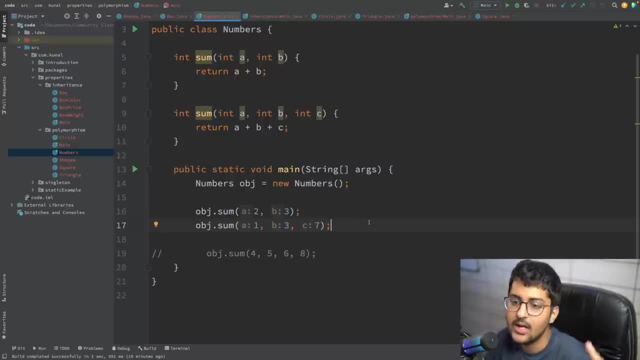 error if you are. you know, like when it's doing the type checking and all these other things. on this case also, like this will also happen, like on compile time. obviously actual memory allocation happens on run time, but the checking and everything and which method to actually run, ok, determination. 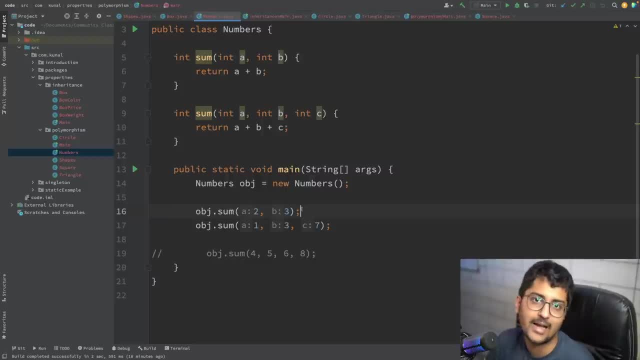 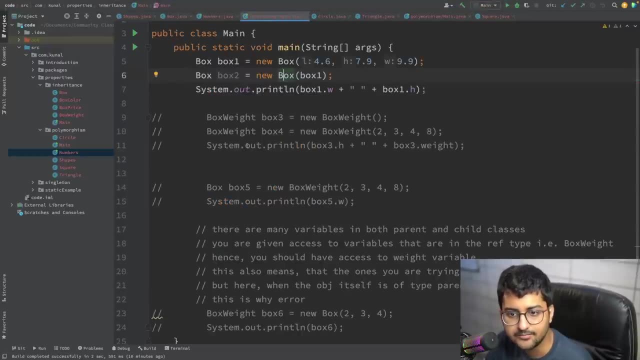 for that happens at compile time. that's why it's known as, like, compile time polymorphism. so here at compile time, it will know that it has to run this because you have passed two things. here at compile time it will know that it has to run this one because you have passed these. 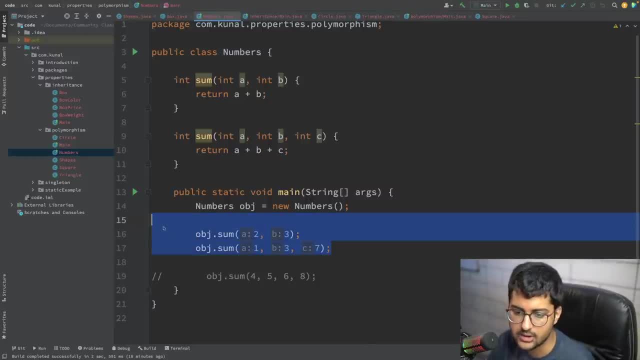 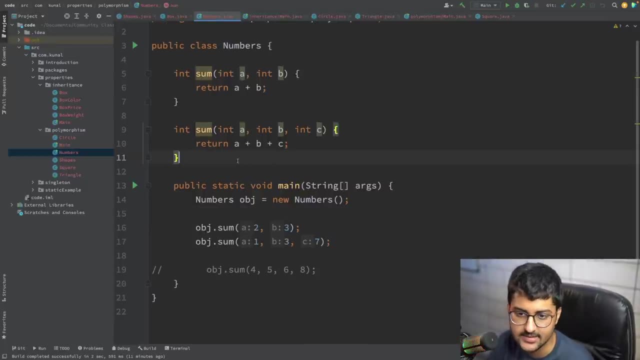 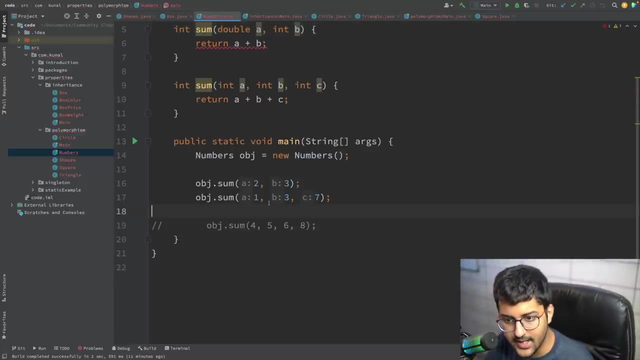 three things: compile time polymorphism, also known as static static polymorphism. now one more thing can happen is: let's say you are doing something like this, let's say you are taking this as a double. ok, you are taking this as a double, but here you are passing. 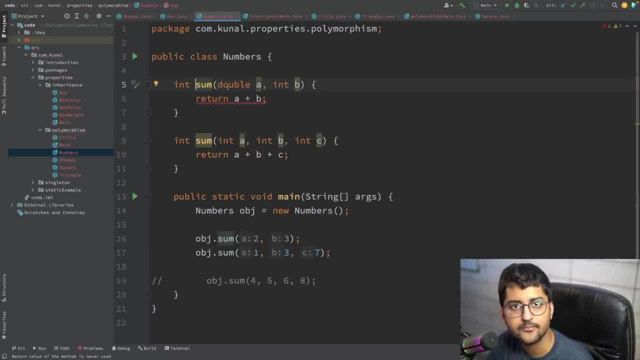 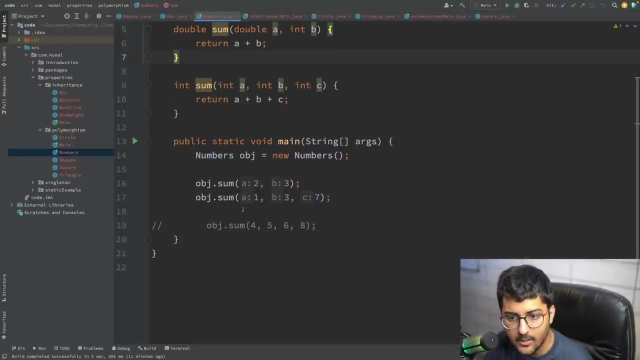 an integer. still this one is called. still this one. obviously I would have to cast this in because I am returning an integer, or I can just return a double as well, no problem. but you can see, here you are passing an integer, still a double is being called. 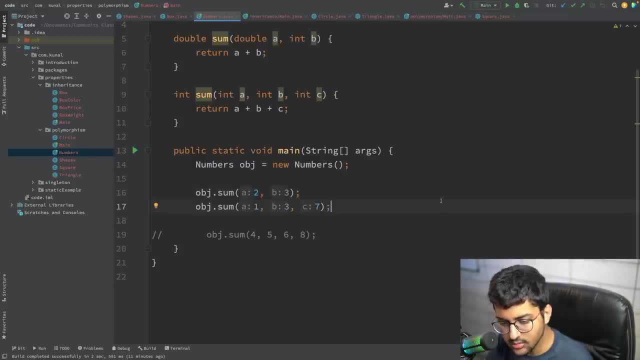 what is happening over here. so in this case you can see that when we are adding an integer argument inside this sum, so no matching is, let's say, found, but java automatically converts that integer into a double. ok, and this will be resolved. this will be used to resolve the call. 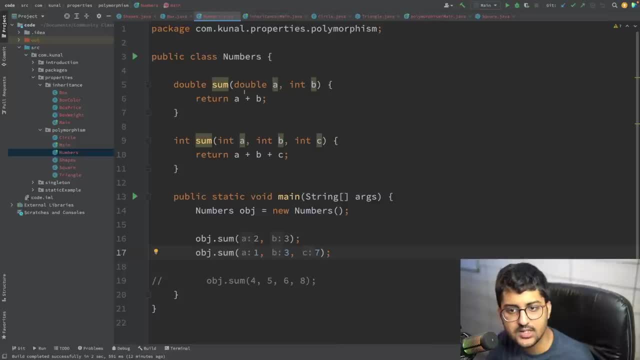 ok. so since an integer for this is not found, a version where this is an integer, this is also an integer, so it just converts it into like double ok, but what if you pass an integer like something like this over here here? it will give an error. so for this, watch the. 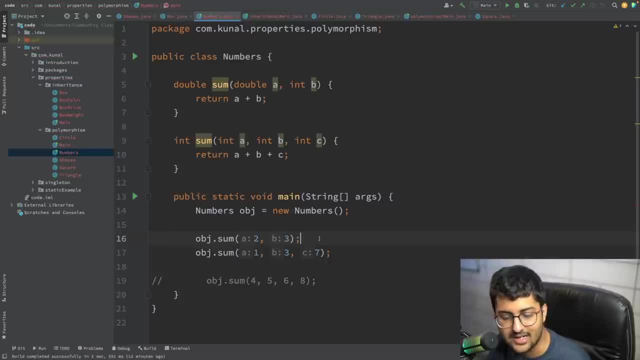 video where I was teaching you casting, how automatic casting happens. basically, in that video I taught you automatic casting. same rules will apply over here. I am pretty sure I will not explain it in the this lecture because I have already made a hours and hours long video on that casting. 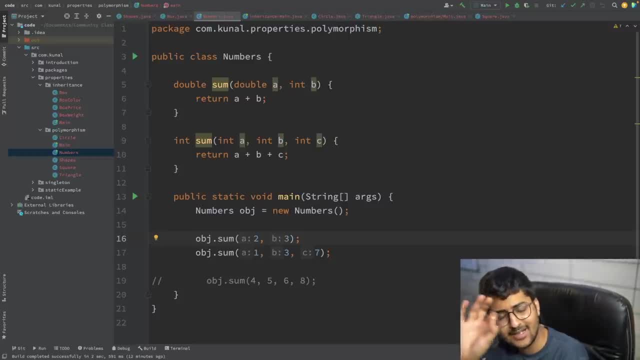 how casting works in java- entire video on that. exactly copy paste those rules over here. exactly copy paste. ok, I have explained how. so basically how automatic casting works is. you can take it over here as well. ok, but for example, if an integer was defined over here, then it would use this: 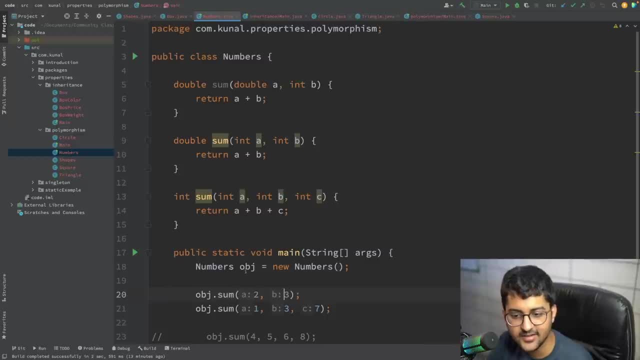 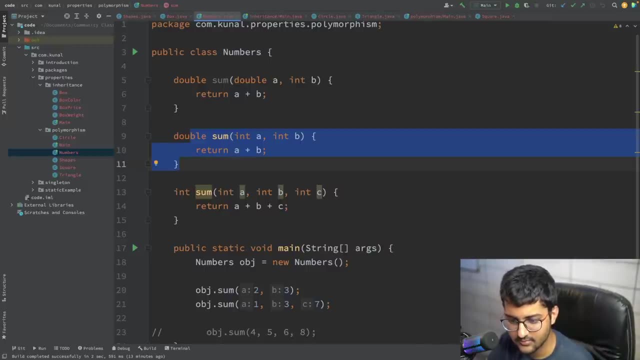 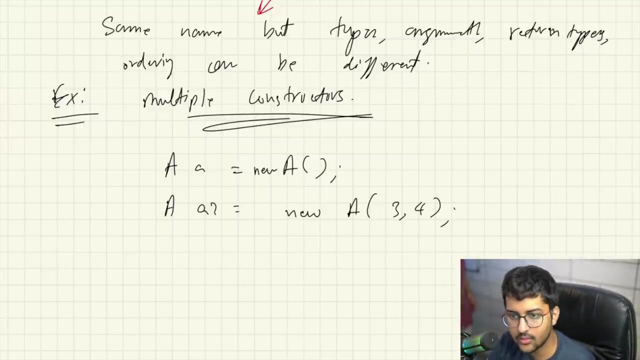 ok, integer, integer. in that case, it would use this. ok, cool, so that was pretty good. ok, so this is known as constructor over loading. now, that was it. yeah, that was it for polymorphism part number one. now there is a second type of polymorphism, something that we have. 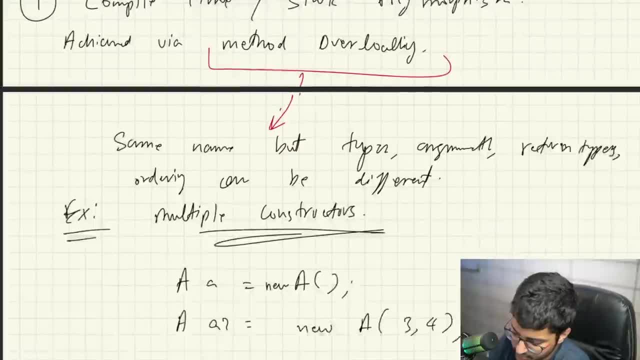 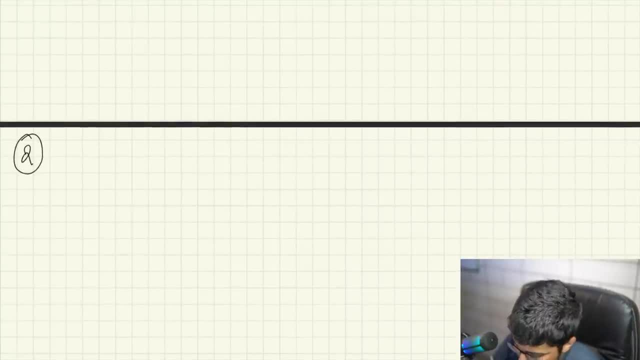 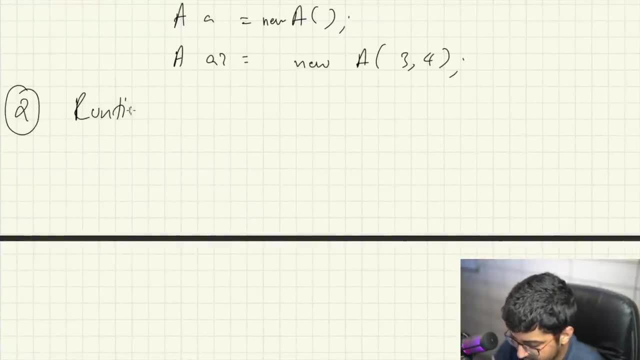 already covered, but now it's time to define it. now it's time to define it. second type of polymorphism- what is it called? second type of polymorphism is called- I am just going to write it above, no problem- runtime, polymorphism, runtime or what dynamic. I will also. 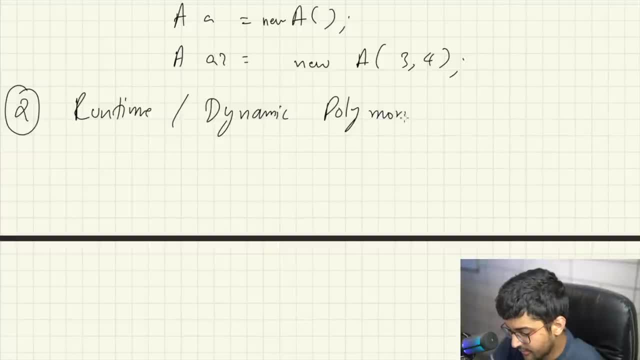 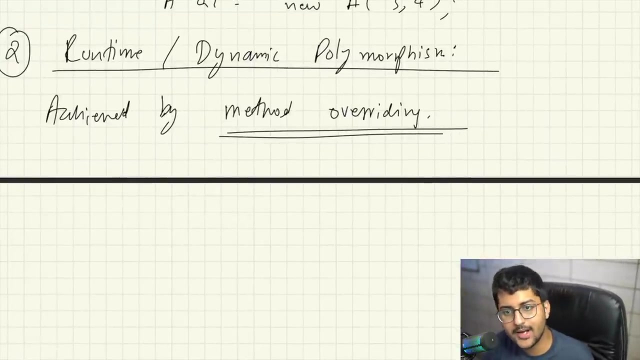 tell you why it is called dynamic dynamic polymorphism, runtime or dynamic polymorphism achieved by method overriding- very important, achieved by method overriding. what is overriding? overriding is simple, overriding is something we have done already. so when a child class, you know, has a method name same as 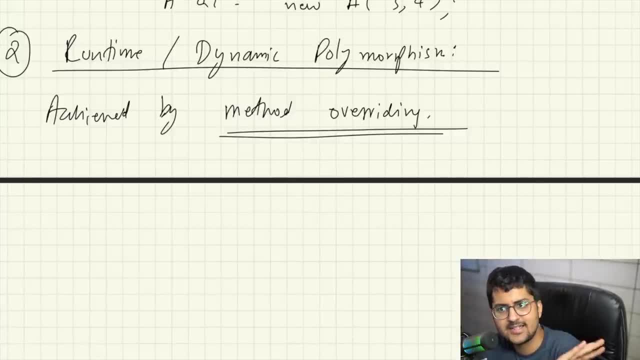 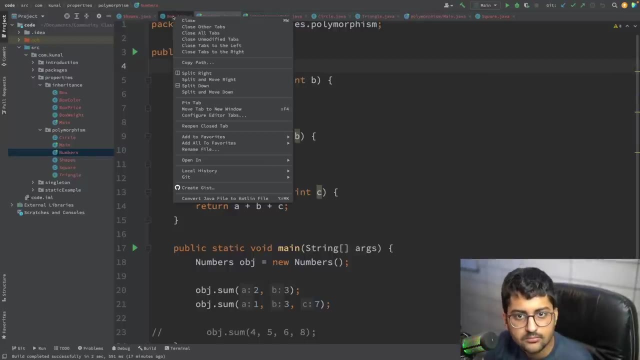 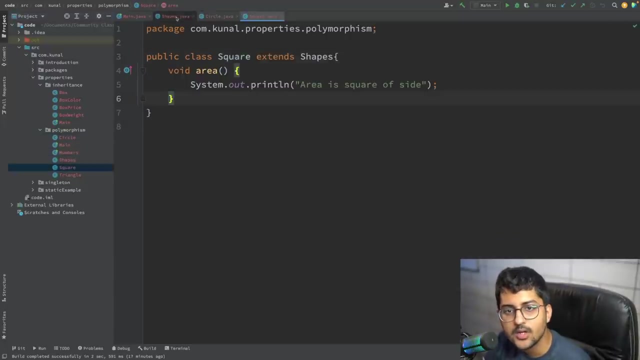 the super class, the parent class, exactly everything is same. ok, parent class has a method, child class has a method parameter and all the return type and everything is same, just the body is different. so for example, over here, close all main shapes, circle, square. ok, shape is the main one, circle. 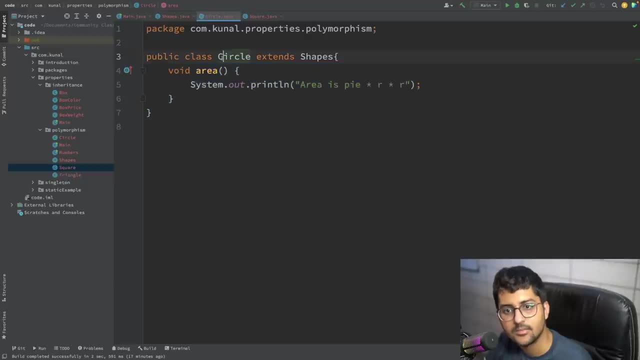 is the child one. this is the child class. ok, this is the circle child class. extending shape: it has a function called area. shape also has a function called area. ok, so this is what is known as overriding. this is known as overriding. you write it some word like this: 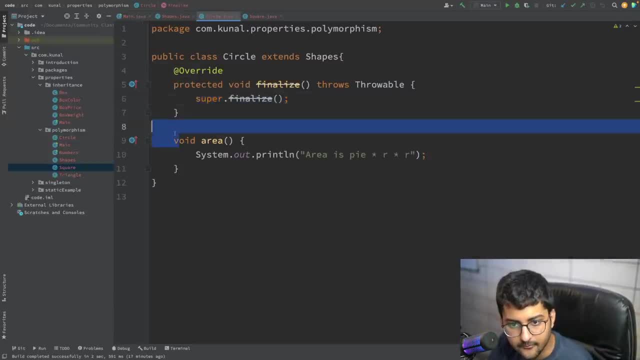 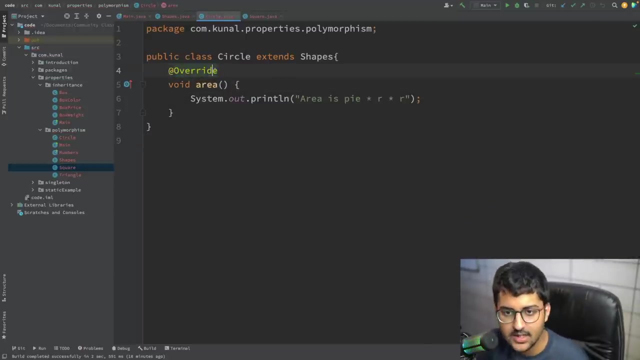 overriding, overriding, overriding, overriding, something like this, then it is giving an error. I will tell you what this is basically. don't worry, ok, I will tell you this right now what this is. so this is basically known as overriding. basically, if you want to check whether a method 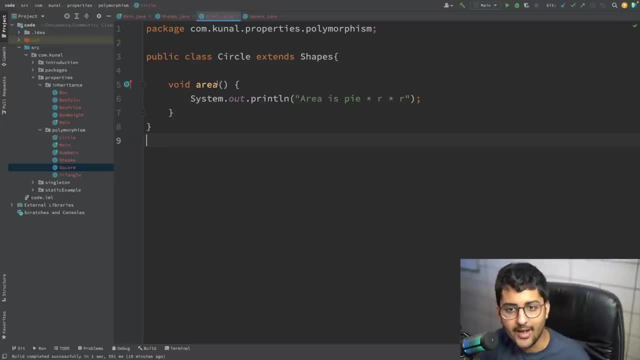 is actually being overridden or not. ok, by common sense I know this is overriding because shapes has void area and circle, which is a child class, also has void area. that is overriding same function in parent class, also child class, also child class is overriding the main one. this will 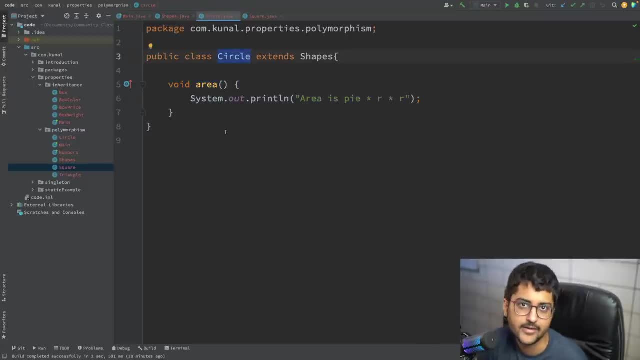 be given priority whenever the object of child class is created. ok, this will run when object of circle is created. hence it is overriding the parent method. ok, what is this thing at the rate override? this is called annotation, basically, if you want to check whether a method is being. 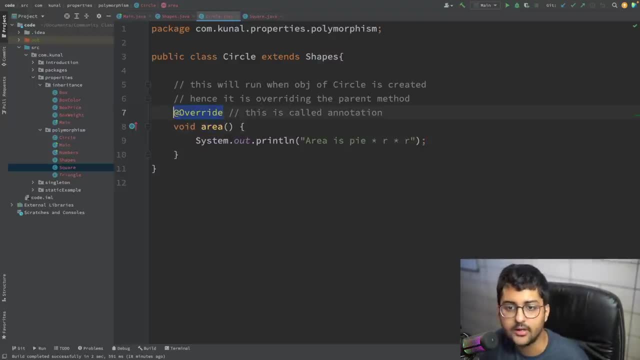 overridden or not, just put at override above it how to create it on its own. these can be created using interfaces, which will look into interface lecture. ok, but for now, if you want to check whether a method is being overridden or not, just write at override over it. 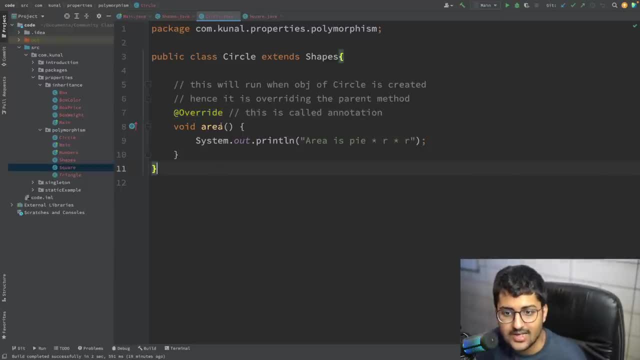 how it works internally. obviously, we will learn in interfaces. so, for example, lets create another function called area: is area being overridden? or if I say area2, is area2 being overridden? no, its not. hence this annotation is giving me a, giving me an error. is area being overridden? yes, it is, hence its. 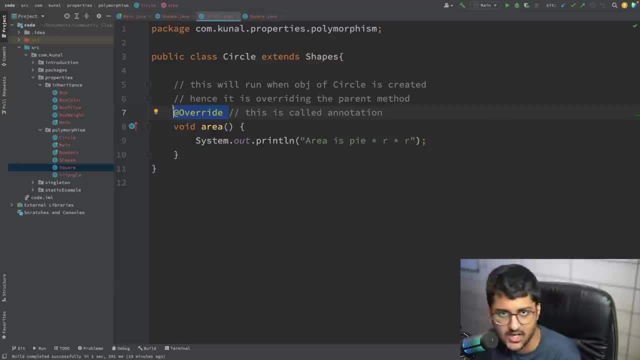 not giving an error, its just a simple check only. ok, check use for check purposes. so that is why in the main function, when you say square dot area or circle dot area or whatever, since the type is of circle, it will call circle only. object type is circle, nothing can change it. 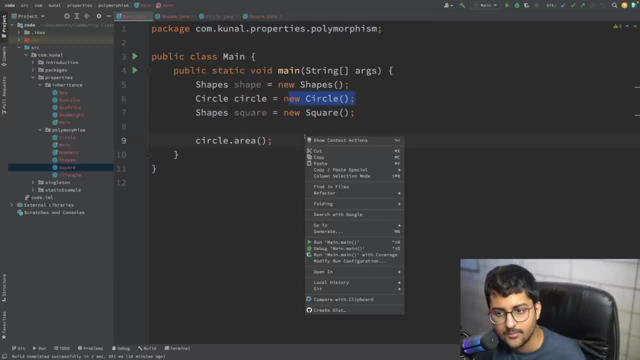 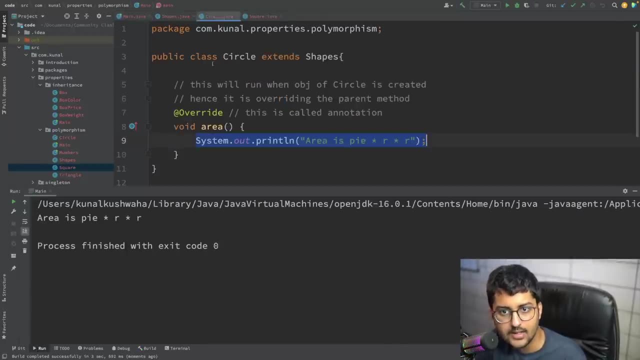 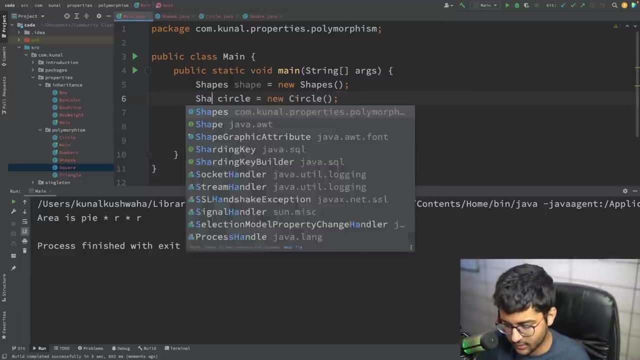 will only call this area is pi r square. ok, it will not call the parent class 1. so, as you can see, in overriding, this thing should be exactly the same. only the body can be different. just everything should be the same. only body will be different, as here if you put shapes. 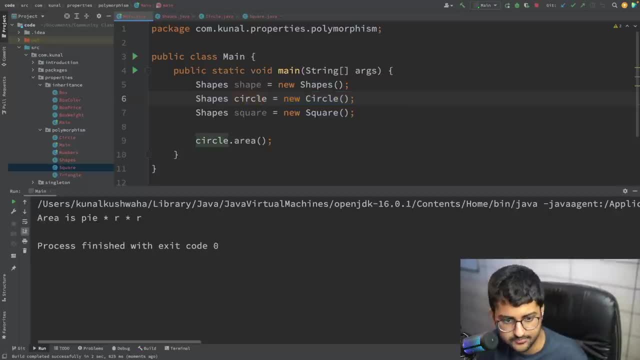 whatever the type of object is, that is the only type that will be used. but you are saying, kunal this, what method, what variable it is able to access? that depends on the left hand side, and you are correct, it depends on this thing. but how is it actually checking which one to? 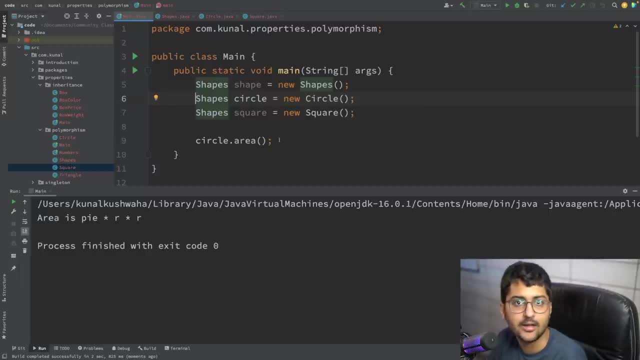 run. how is it actually checking that? lets look into that. you will be able to understand why this is always calling the type of the circle. if you put shapes over here then obviously it will call the shapes one. so here type of method in overriding that is called depends. 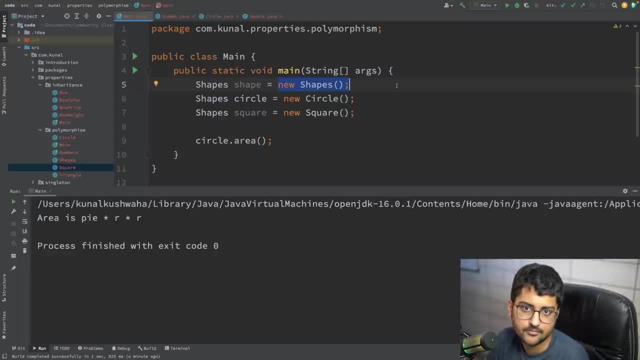 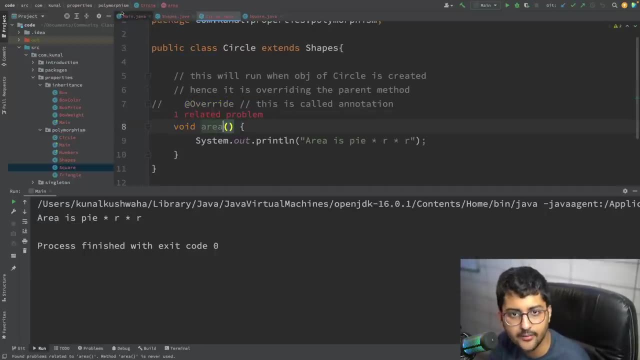 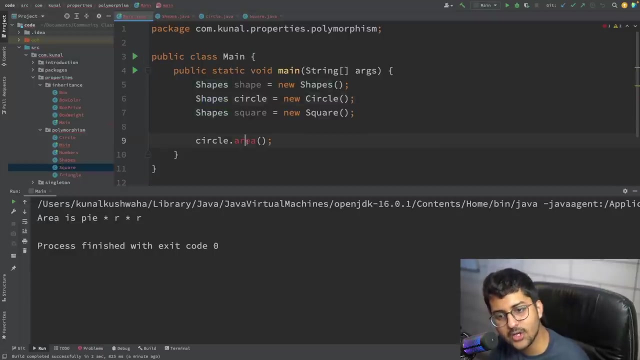 on what the type of the object is. ok. if you remove area from here, ok, hide this over here. now it is giving me an error. so to access area should be obviously there. i am not defying my statement. my statement previously was that all the elements that are accessible to. 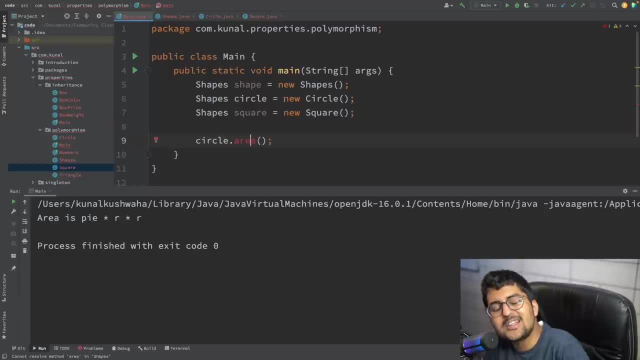 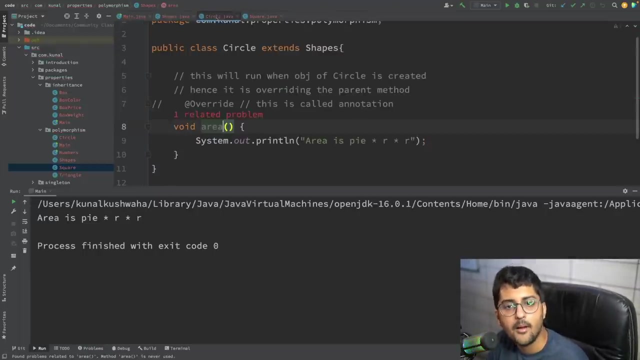 shapes will be available, because what is being accessed does not depend- ok, does not depend- on the object type, it depends on the reference type. so reference type should have an area. it does not have an area. that is why it is giving an error. it should have an area, but 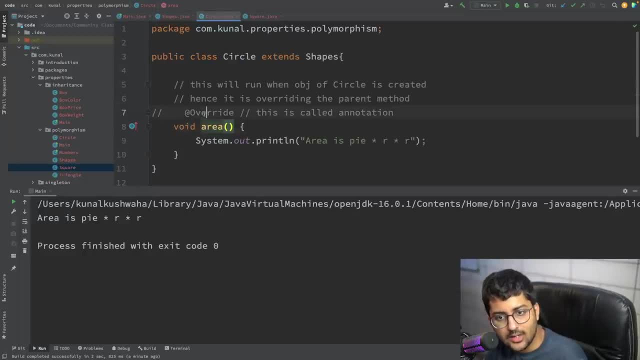 its actually not going to call this. its going to call this one if the object type is of the base class. why? because the objects base class one is actually overriding the above one. why so? actually, what its able to access is defined by the type of the reference. 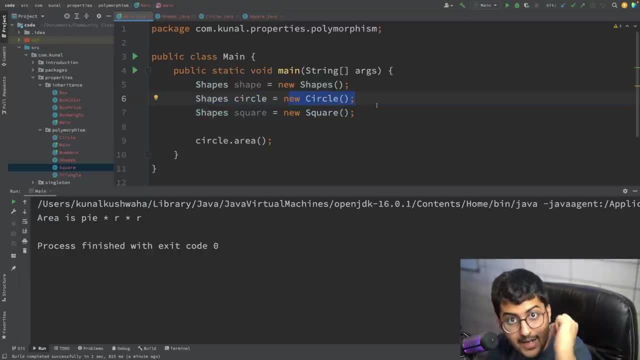 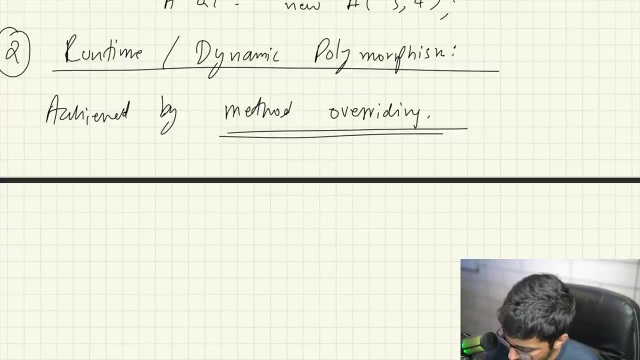 which one its able to access is defined by the type of the object and how. lets look into that. ok, so let me tell you about this thing. then now lets see. so let me bring on my like code sample once again, because i wanna show you, like, show you something. 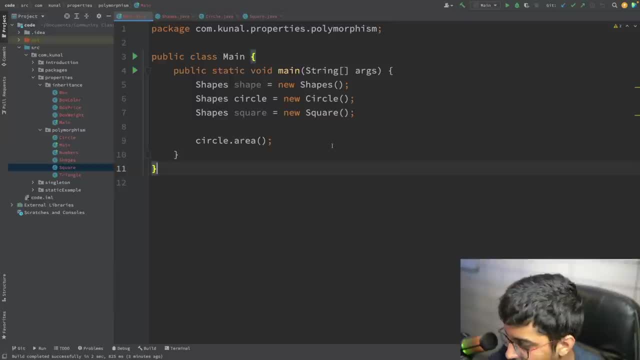 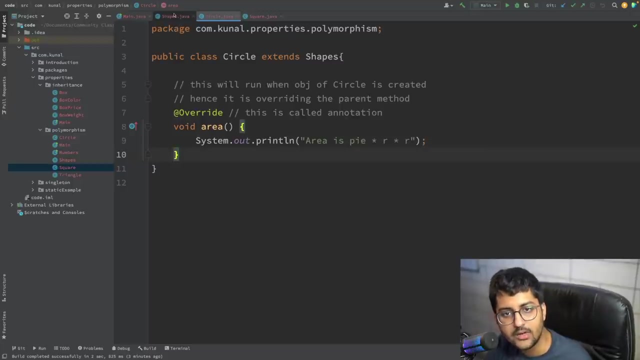 so over here in the code sample here you can see: if i directly just create this as circle, right, if i directly just create it as circle, it will obviously call the one inside this circle. that is obviously no issues. you are like kunal, what if? like, even if you. 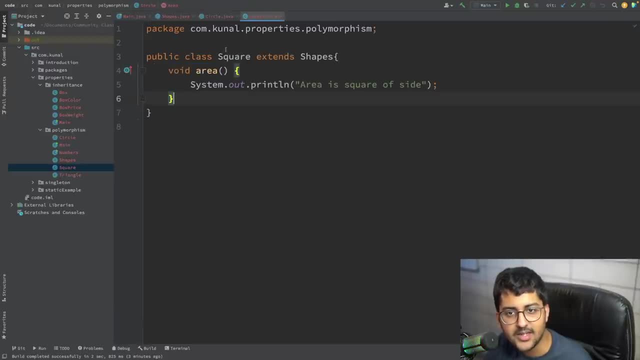 weren't having main in the main, main shapes one, if you were not having area. in that case also kunal, it was calling the area of a method. then what do you mean? what does it mean then? how is it like overriding? overriding basically means if the type is the reference variable. 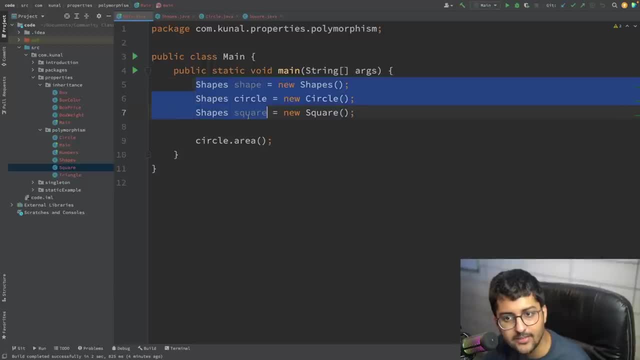 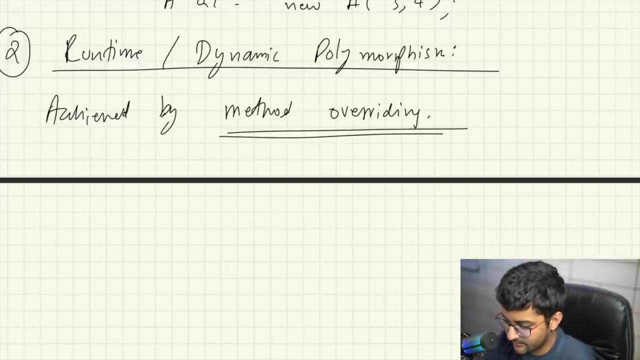 ok, if you have the type of the reference variable as the parent class. the type of the reference variable is parent class, but the object is of type, the subclass. ok, in that case what happens? lets see, because otherwise it was doing the simple stuff. ok, but if the type 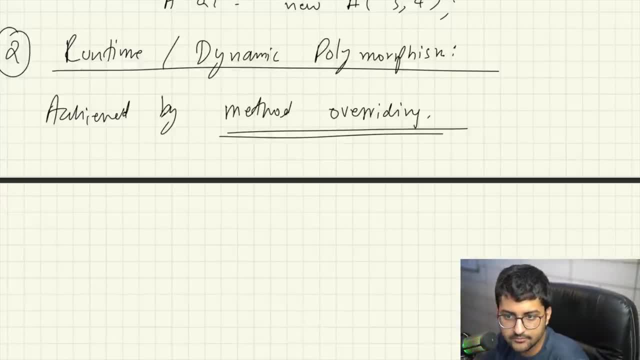 is parent class and the object is of you know the overriding. how it actually this thing works, because child class reference child class. parent obviously is calling its own one. ok, but overriding is done when the reference variable you are using is of, like the super class and which particular method will be called. 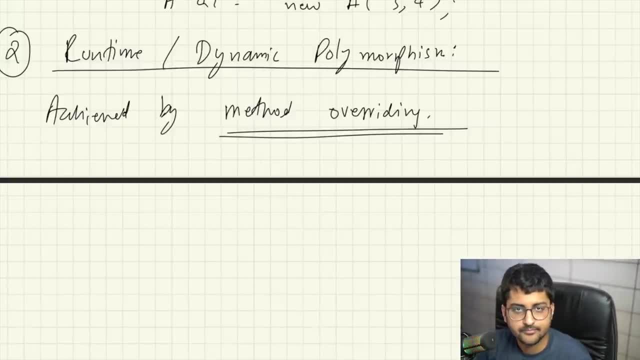 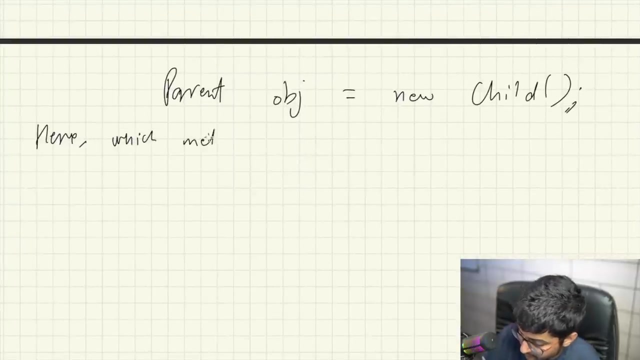 that depends on object that the reference variable is referring to. so, parent, parent, object: new child, child here here, which method, which method will be called, will be called, depends on this: the type of child this is known as. this is known as. this is known as up casting. 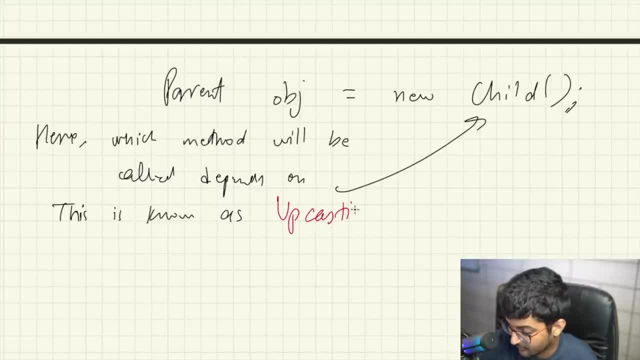 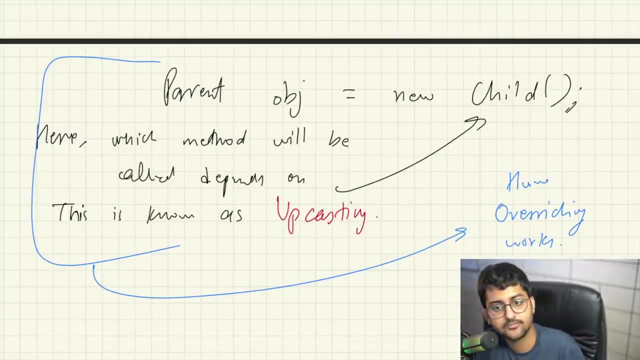 this is known as. this is known as up casting, and this entire thing is known as this: overriding- how overriding happens. how overriding happens, how overriding works. ok, thats basically it. this is how overriding works. thats it. okay, no problems, that's it. also gave you an example, but one more thing i forgot was, uh, how it actually 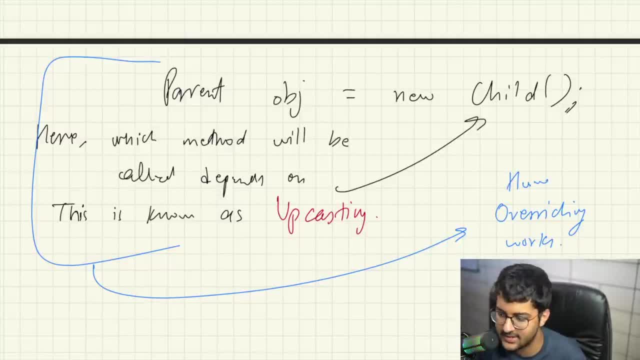 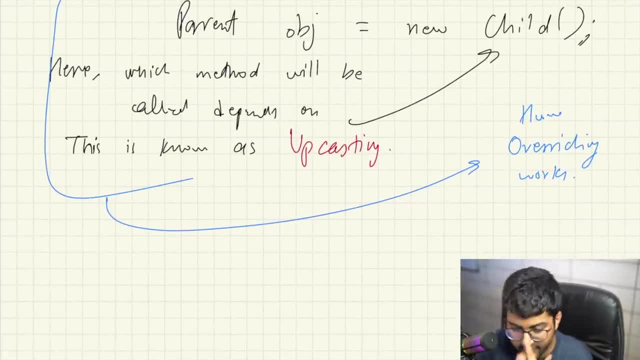 works internally- the memory management, uh part and stuff. let's talk about that as well. okay, so this actually happens, like: how does it know, how does java know, which particular function to run? there is a function with the same name in the parent class. there is a function in: 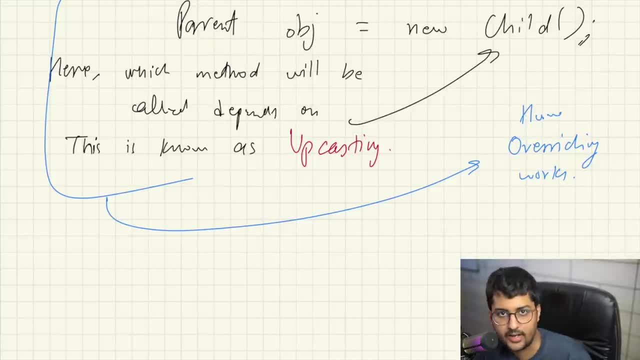 the same name with the child class. we know that child class one will run. we know that because which one to run actually child object, that the object type defines which one to run, okay, and the, the reference type, defines which one to access, which one it can access, okay. so here, see here. 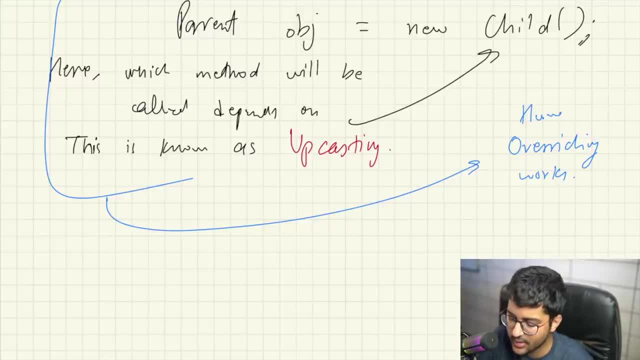 basically, um, uh, parent one says that, okay, you can have, you can access a function with, with the name that has the name as what. it has the name as: uh, print or what, what, what are you printing? we are printing, uh, the sum or whatever, or shape or area, area, area, okay, but 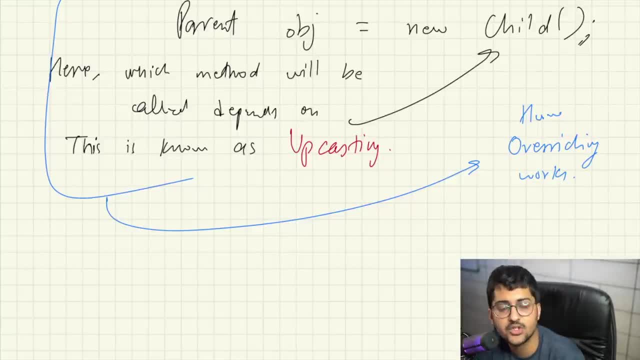 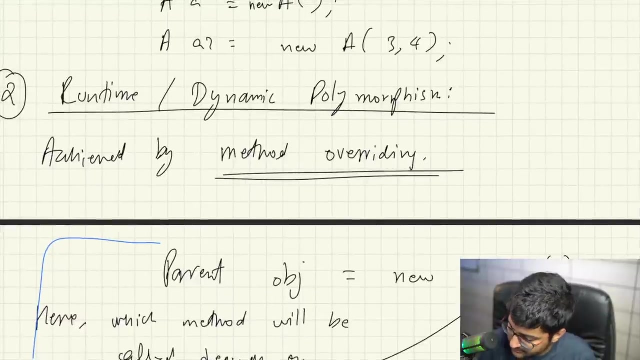 which particular version of the area, which to call that, is defined by the object. that is determined by the object. but another question is how, how it happens, how java determines this? how, how java determines this? how java determines this? the java determines this with something known as dynamic method dispatch- very important. this is why it's known as dynamic. uh, dynamic. 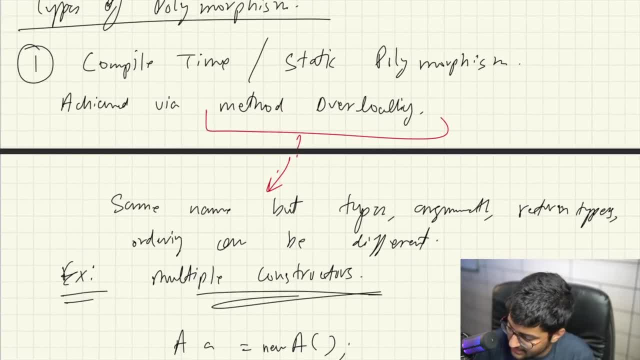 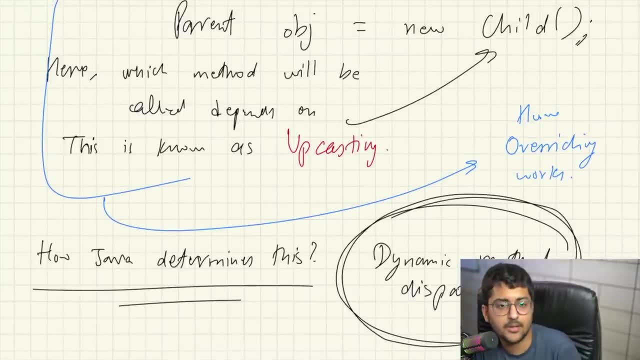 polymorphism. so this one was compiled. time. static polynomial morphism by overloading: this is runtime. dynamic polymorphism by uh: method overriding- okay. so what is dynamic method dispatch? it is just a mechanism by which a call to an overridden method is resolved at runtime rather than compile time. all the compilation. everything is done when the method, when the, when the program. 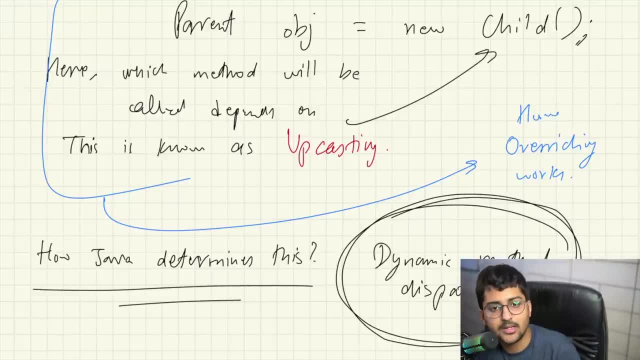 is running. during that time, java will determine which particular method to run. it's important because this is how this is. this is why this is how we are doing runtime polymorphism. that's where time comes in. okay, so we know that a super class reference variable can refer to a subclass. 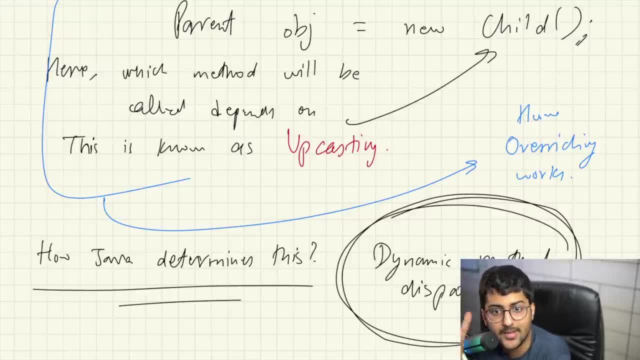 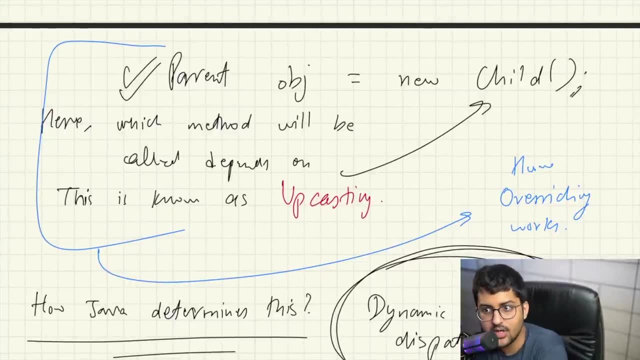 object- we have just covered this- and when an overridden method is called through a super class reference variable, for example- in this case, java determines which version of that method to call based on the type of the object at the time this call happens. hence, this determination will be made at runtime, when it's actually calling it. when is it actually calling it at runtime? 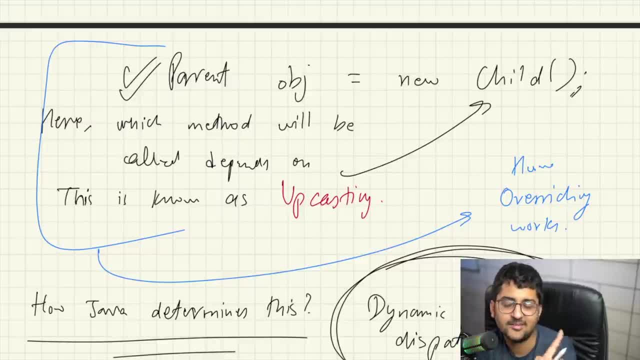 don't ask me what is runtime and compile time. okay, please watch the uh lecture number one. okay, now that's it. yeah, in other words, you can say that it's the type of the object being referred to, not the type of the reference variable, that determines which version of the 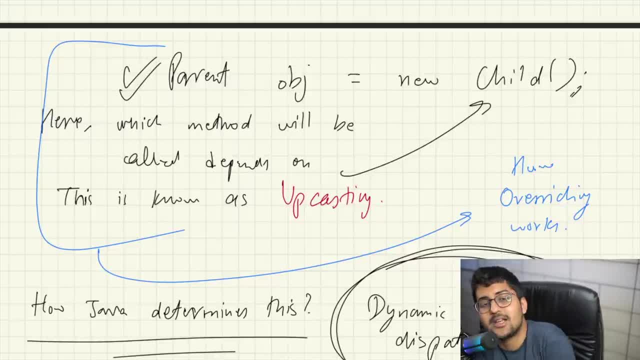 overridden method will be executed. but i also stand by my statement that the reference variable type actually tells us which all things you can access. that is why, once, even though the one in the subclass is being called, and you're like, hey, if the one in the subclass is being called, 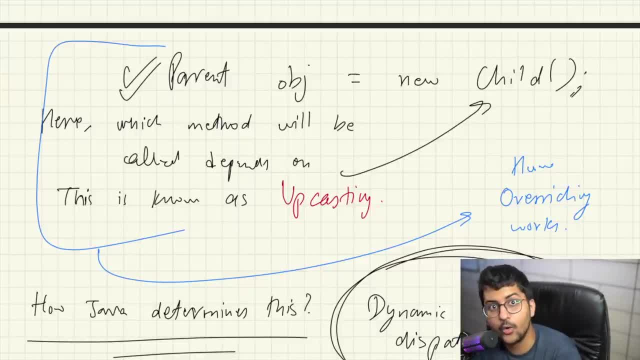 why do you actually need to put it in the parent class also? then you can be like: no, if it's not in the parent class, then it will be like: okay, uh, in the parent class it will only be accessing the one that is like the: the parents one. hence you don't have it in the parent class, so you can't access it. 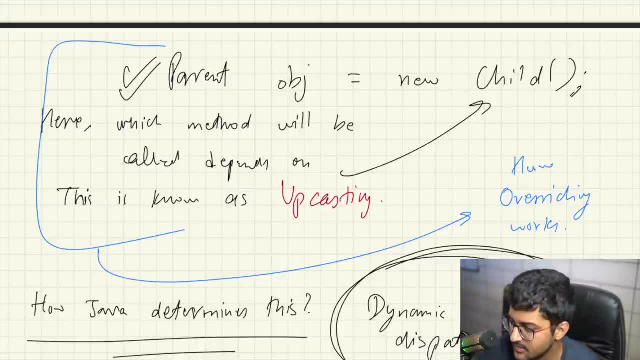 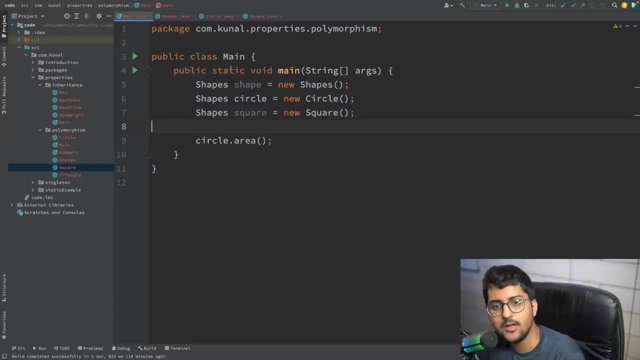 okay, sound good. so same example over here. so you can say: in shapes, if i remove this particular thing because you are saying kunal in this line, it's actually calling this one, can't you just remove shapes. then you can be like, no, it can't, because if the type is shapes, 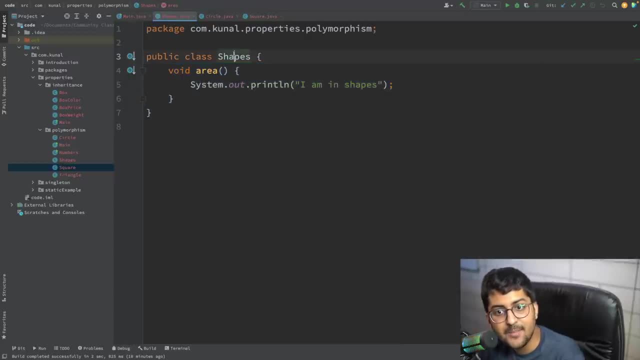 then it will only access whatever is accessible in shapes. shapes have no idea what is in behind, what is below it. okay, it has no idea what is below it, so that's why we need this for accessing, like. okay, we know that it can access a method called area because it is available over here. 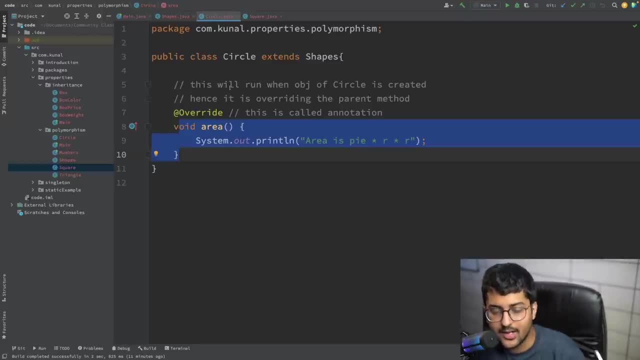 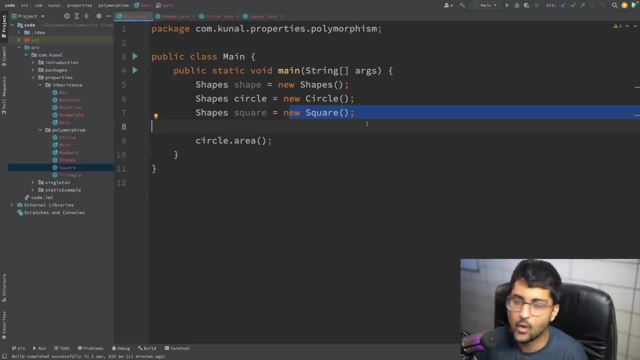 but which one to access. that will be determined by java during runtime using dynamic method dispatch, and it will all obviously be dependent on the type of the object that is being created. cool, that was it. let's move forward. okay, and this is the same thing we were doing previously also. 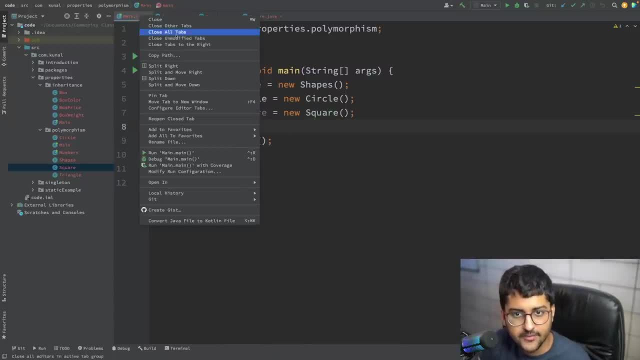 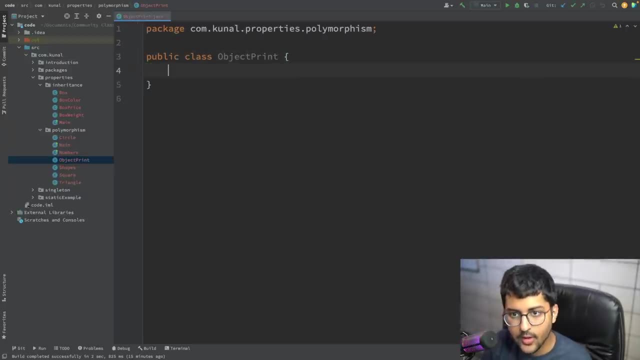 internally it uses, let's say, the two string method. right, let me just close everything. and object print, for example: okay, i create a public static void main. this object print has a something like, let's say, int number constructor using a number or whatever. okay, i create an object from it. i can say object. 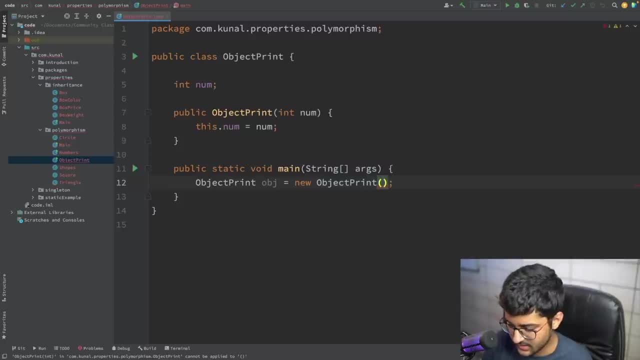 is equal to new object. it passes a number, let's say 54.. if i try to print this object, java, i haven't told java that whenever you print this object, i just want you to print, let's say, the number, the value of the number or whatever. okay, i i have not told java, so java will do something internally. 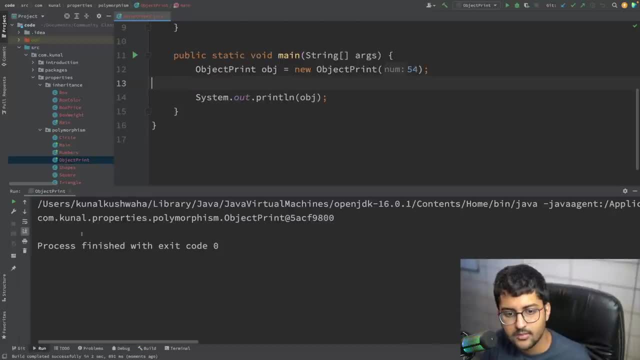 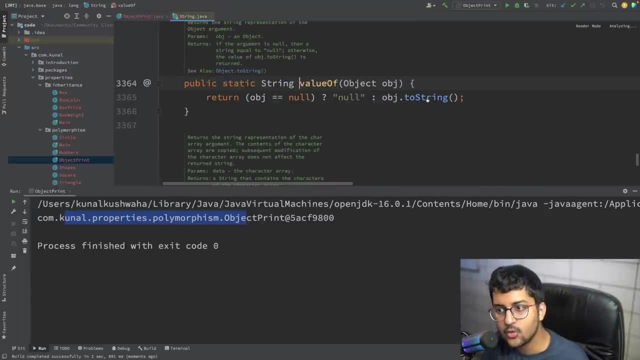 on its own, just printing this. so print l and taking an object inside it, it will call the value of function and that will call the two string function: object dot two string. object dot two string. so it's like our. object object dot two string. object dot two string. so it's like our. 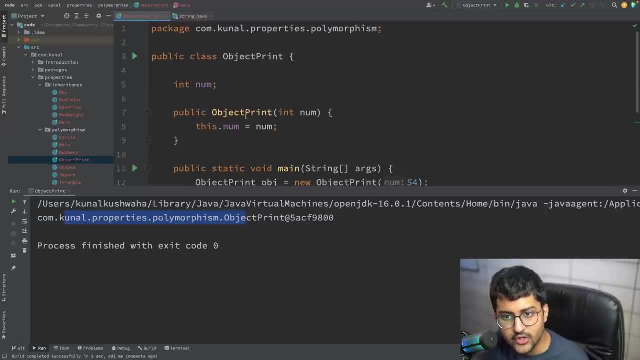 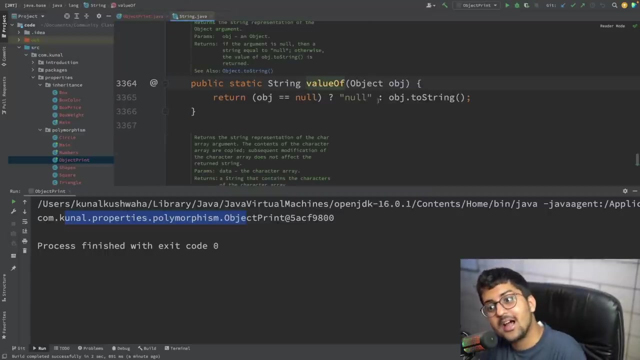 object object that we have passed. does it have a two string method? no, it does not, so it will use the default one. and which is the default one. every class is inherited from which class- object class or not, so it will use the object classes two string method. 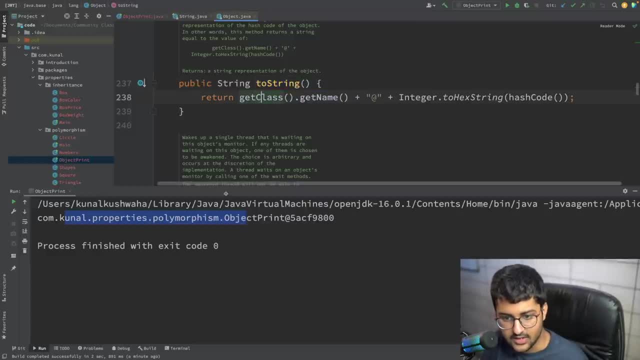 object class as a two string method. just get the name of the function in class and, uh, do an add the rate. yeah, it's putting an add the rate. okay, the hash code. hash code is just a random value, random number. i'll cover it more in detail. 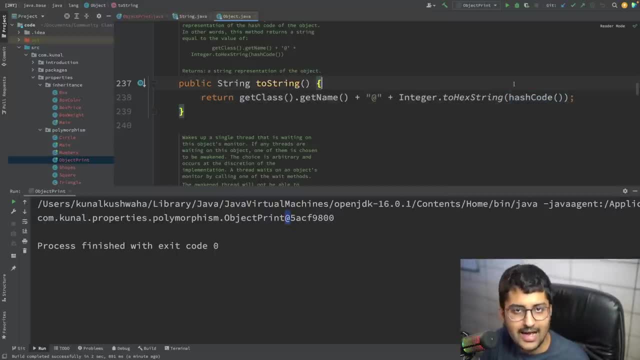 in the um, in the uh hash map tutorial. but it's for now. let's say it's just a random number, not let's just say it is literally a random number. okay, based on the value of the object, some internal implementation will actually write our own hash code method. i'm getting too excited. 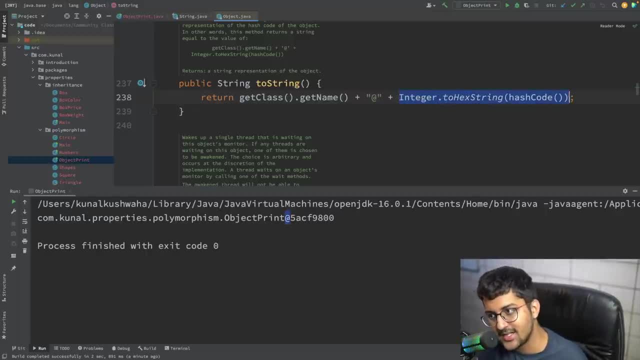 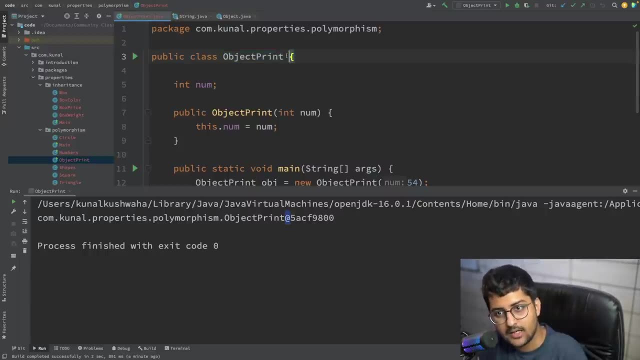 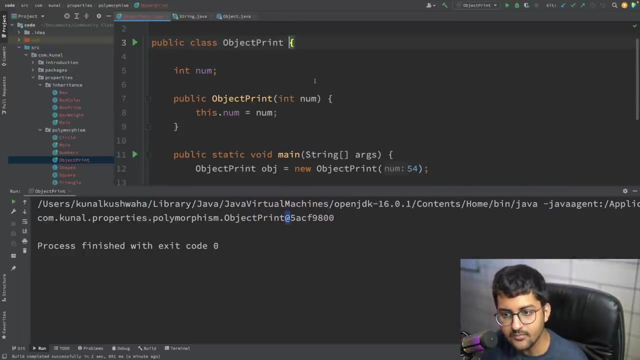 so please wait for hash hashing method, but for now let's say it's a random number, so it's actually using the one with object class, because i know every class, even the classes, are right. they are extending object class extends object class. okay, so that is what is happening over here. 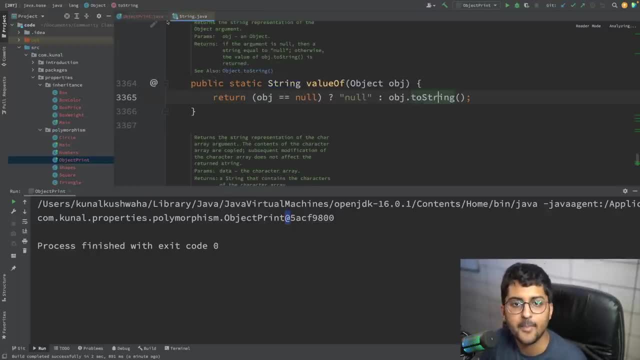 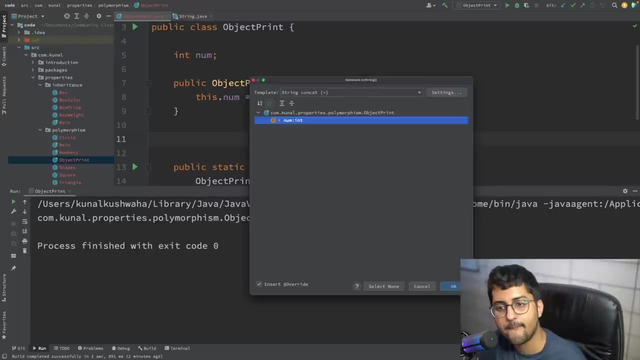 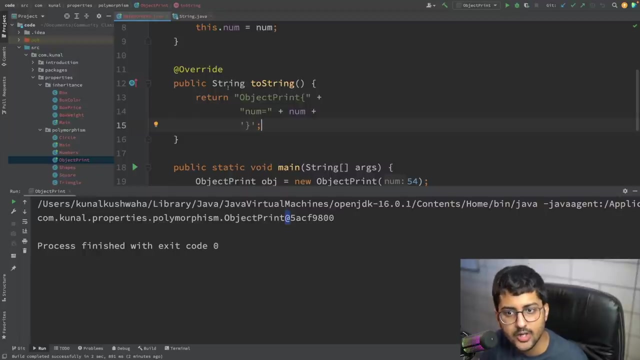 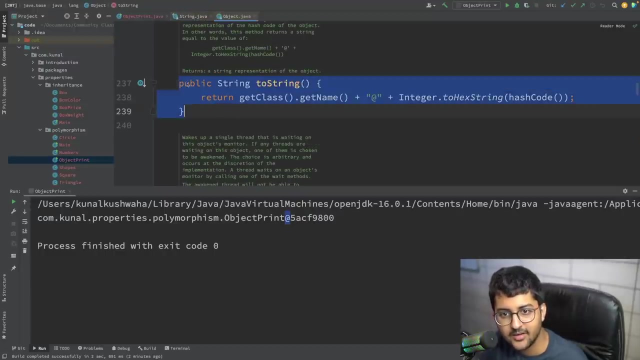 it's using the object classes to string method. but what if i provided a to string method? what if i provided a to string method? something like this pretty, something like this two string method requires. you can see, this two string method and this two string method are same in terms of the definition and everything, just the body is different. 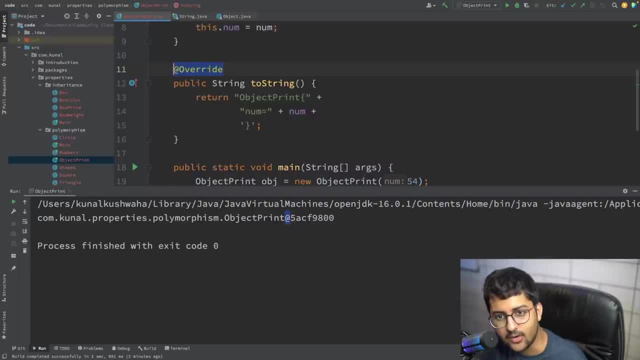 isn't that true? that's why i'm adding an override check over here. does it actually? is it actually overriding the actual two string method? yes, it is, because this is not giving me any error. you. you don't ask me a question like kunal. this is not extending anything. how is it overriding? 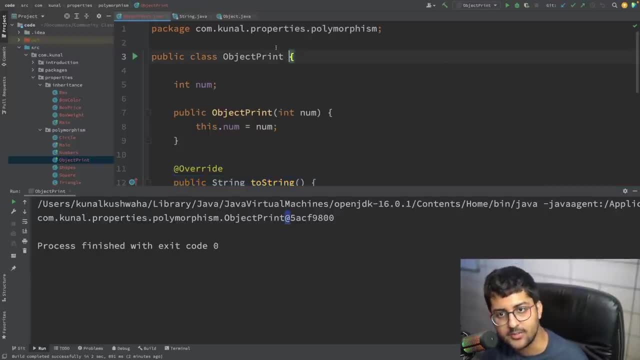 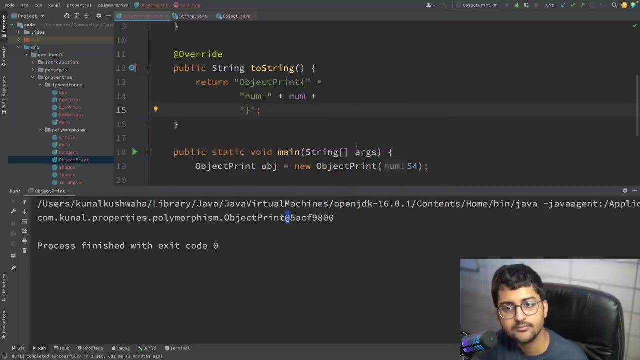 it, then it is extending. by default in java, every class extends the object class. now when i do this thing, so at run time it will define. at runtime it will determine that this one should be run at. may be joking, run, run time. now it's printing it. 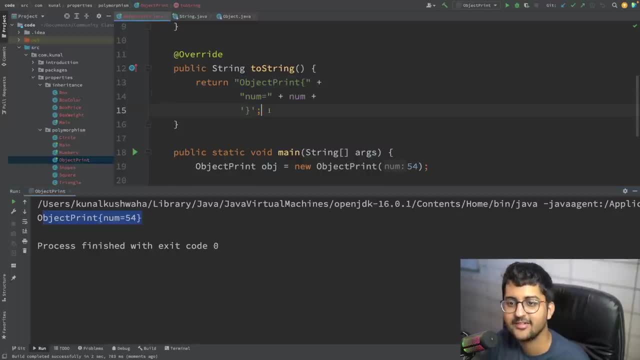 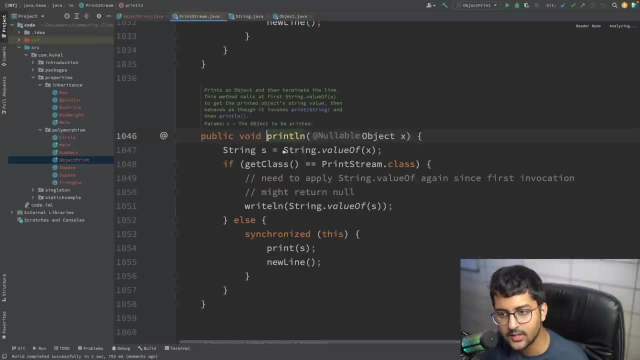 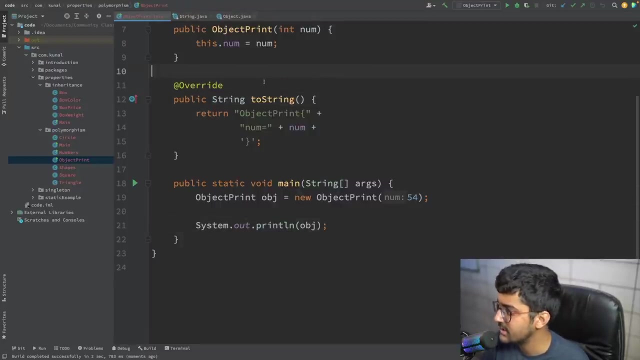 now its printing it like this, isn't it cool? so at runtime it's deciding it. that's why, even if i do control, click, control, click, it's actually not giving me like this particular object, because at runtime there is no result, so the person runtime is deciding it. okay, let's move forward. now let's talk about two more important things. 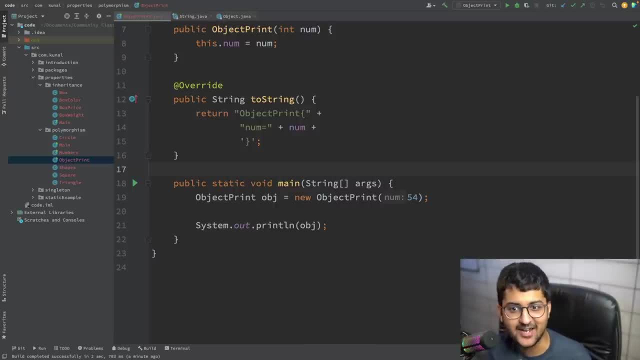 which is using the keyword final and the keyword static. in this, let's put some, let's get some like, uh, do some random things and put static here and there and see how it works. okay, so let's first put final, final. we know it's used to create constants, right, but you can also use final. 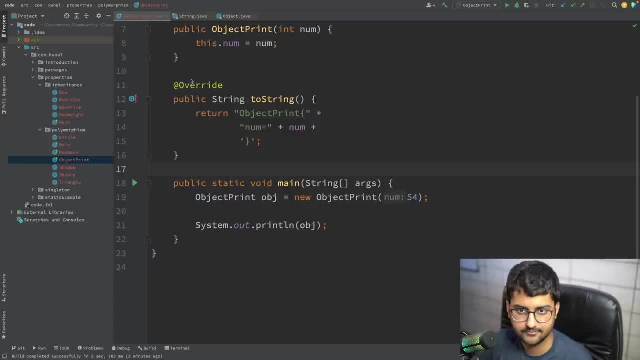 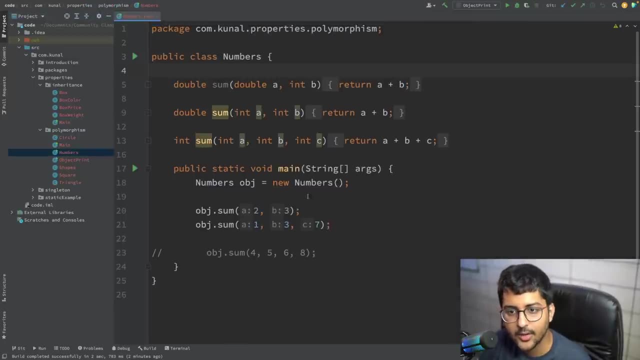 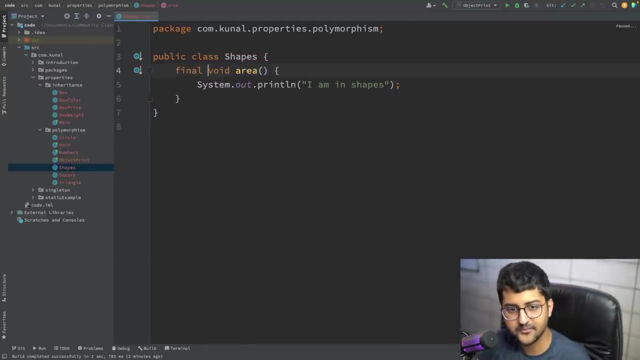 keyword to prevent overriding. okay, remove this, all this thing. numbers, okay, something like not numbers um shapes. if i put this at final, then this is giving me an error. you cannot override a method that is final. okay, if you put final over here, you will not be able to override that method. 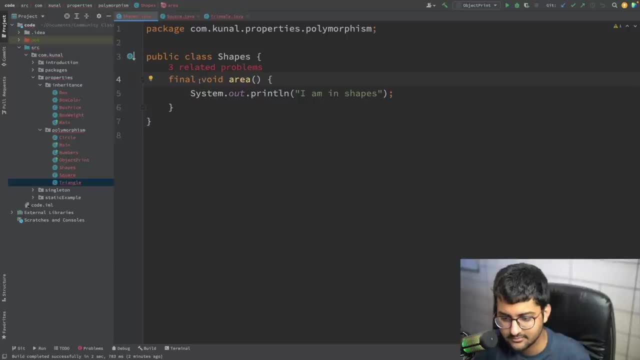 as simple as that. okay, why? because methods like this that are declared as final can somehow provide a performance enhancement. okay, because the compiler is free to inline the calls to them, because the compiler will know that these methods will not be overwritten. and i know overriding and all these. 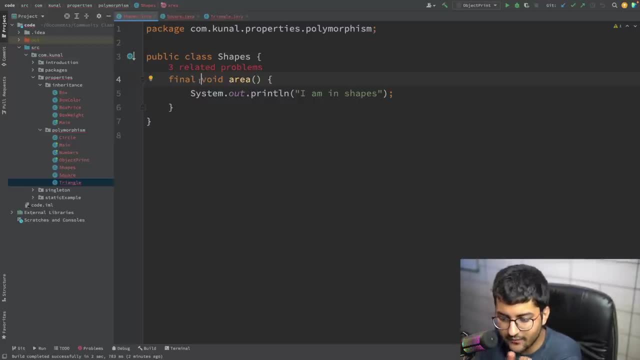 things happens at runtime. okay. so when a small final method is, you know, when a method is called java, compiler can copy the byte code. okay, from the subroutine or whatever like, the internal implementation is directly with the compile code of the calling method, hence eliminating the overhead associated. 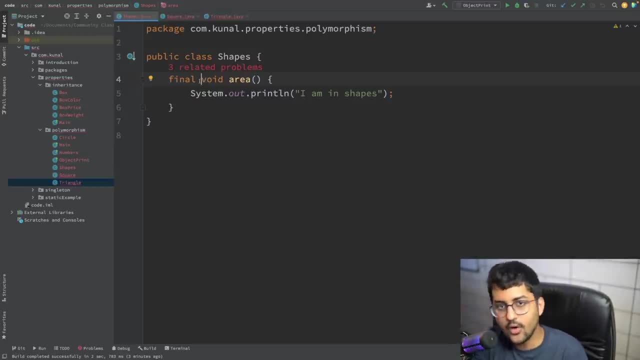 with this method called like which one to actually resolve it. no, this will be only one result, because it cannot be overridden. what is remaining, then this will be resolved, so that extra step is gone, okay, cool. so one more thing i would like to share is the dynamic method resolution, because it is happening. 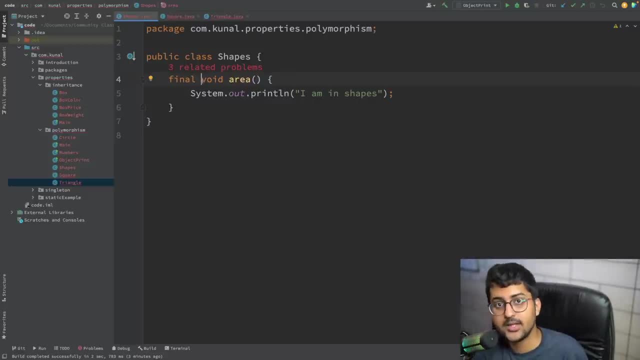 at runtime, after the compilation and bytecode stuff, and everything is done when the program is running. that is when overriding actually determines which one to run. hence it's also known as late binding. it's also known as late binding. however, since the final method cannot be overridden, a call 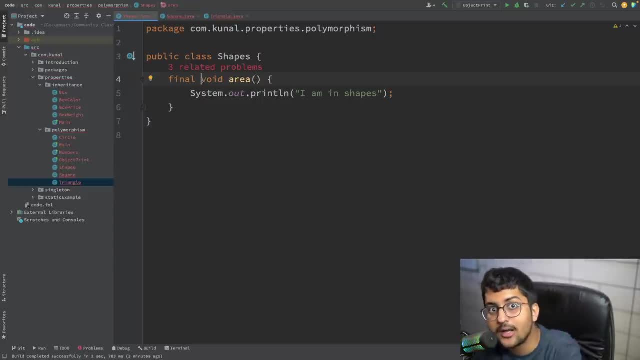 to one can be resolved at compile time only. this is called early binding. okay, early binding and late binding. okay, early binding and late binding. very important concept. just gonna write it over here, but i will put it in my notes also: early binding, check notes. okay, cool, so you can use it to prevent overriding. you can also use it to prevent inheritance. 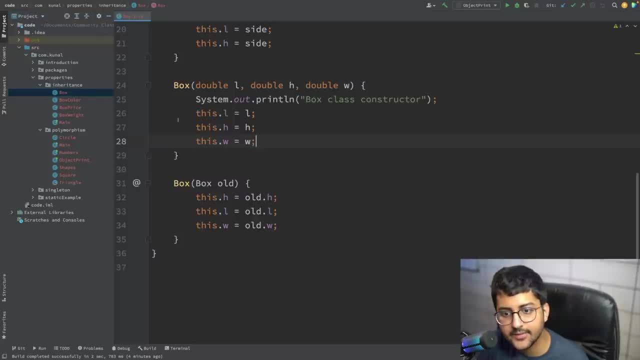 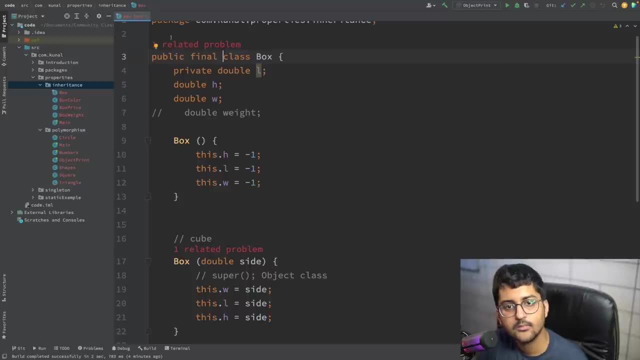 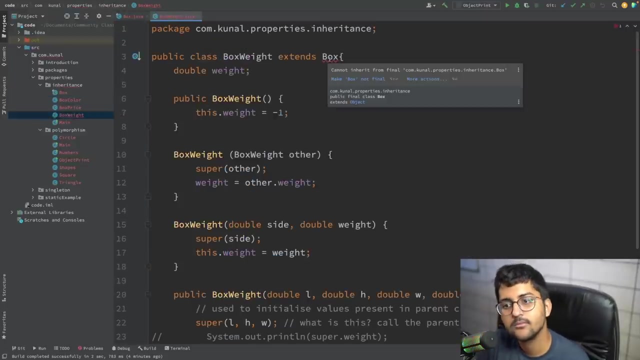 okay, close all tabs. inheritance- okay, so you can use it. and here you go, at the end of the session so you can just go on to the next step to solve it. and so now let's see how we can apply it. i separate the class from the old class. 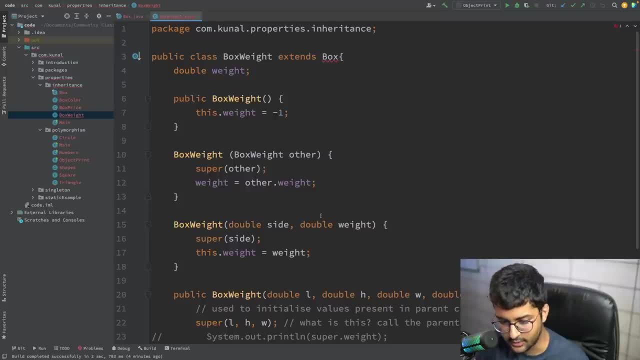 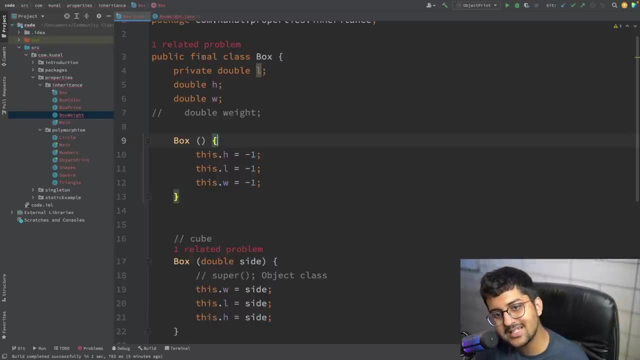 and get rid of the error, and that's it. start our loop over here and we'll see the result. you can see that it has. it's an error, error, error. so sometimes you would want to prevent a class from being inherited, or that you can just put it as final one thing i would like to point out over. 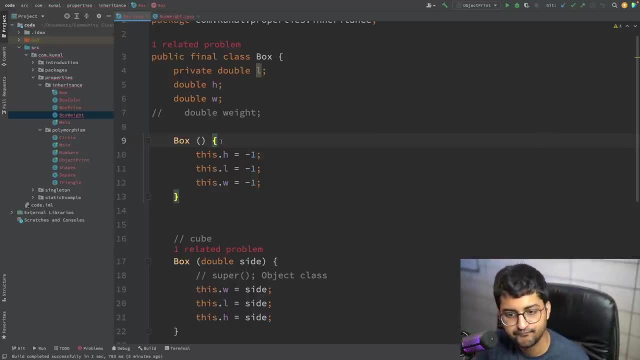 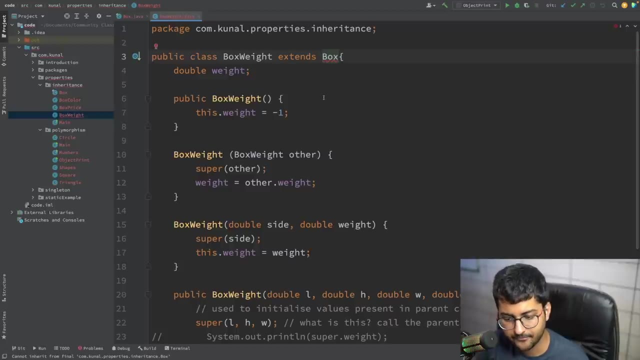 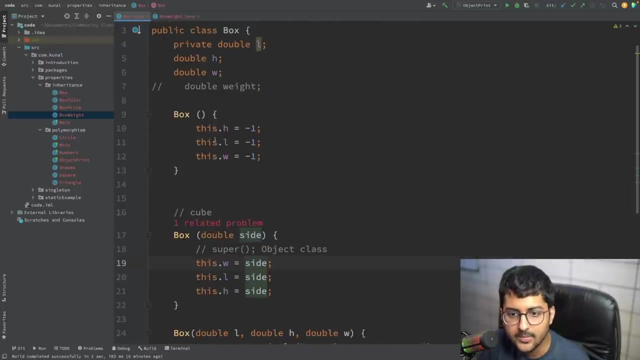 here is: whenever you put a class as final, okay, implicitly it declares all of its methods final two, the methods will be final as well. okay, cool, okay, let's move forward then. right, cool, now let's experiment something. let's create a static method. let me create a static method over here. let me create a static method. 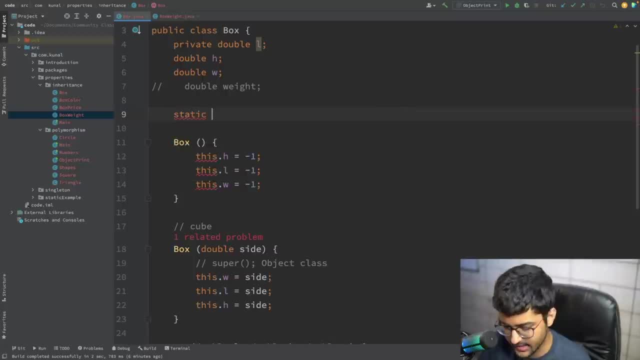 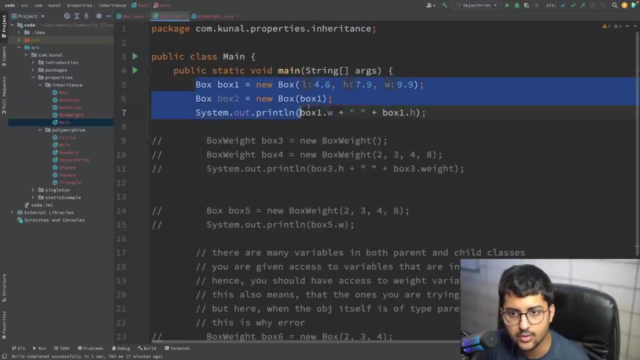 i'll just create a static method like static void greeting. hey, i am in box, i am in box greetings or something like that. i am in box class. okay, static method, no problem, let me call my main. let me just do something like: no problem, i can hide this, i can just say box one. 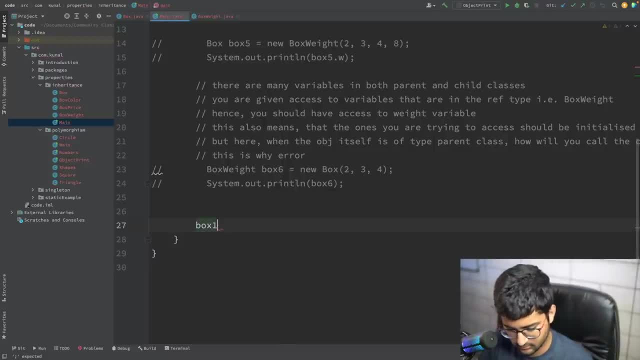 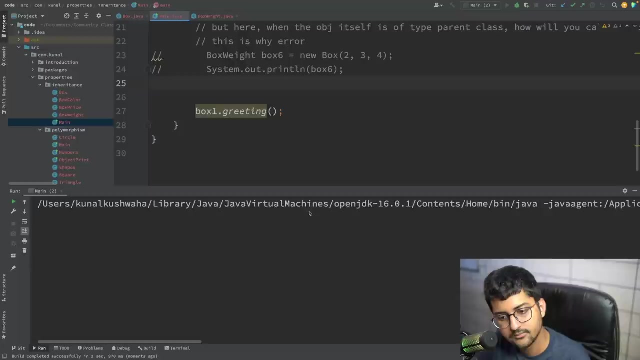 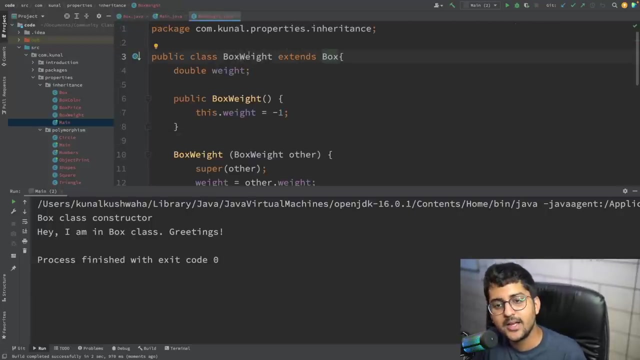 box one dot greeting. let's see what happens. print. hey, i am in box class greetings. one thing i told you previously: static methods are what it means: that it is not dependent on the object of this class, object of box. hence, to access static stuff, to edit static stuff or whatever you want to do, even though you can do it via the reference. 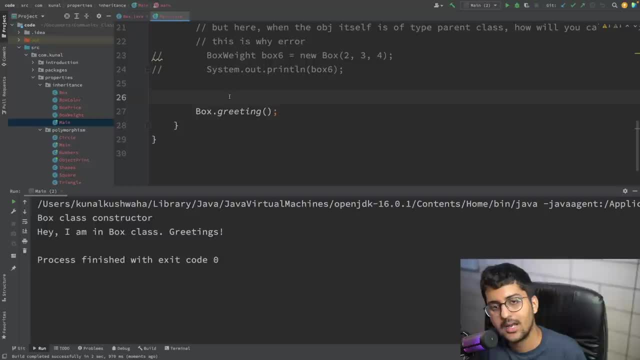 variable, you, you. the convention is to do it via the class name. why? already made a really long video on static. i explained it in the previous video, so you can do it via the reference variable. i explained static in such a great way in that video. it's a previous video, please watch. 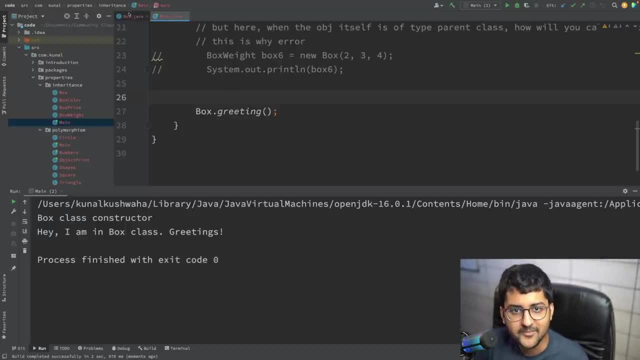 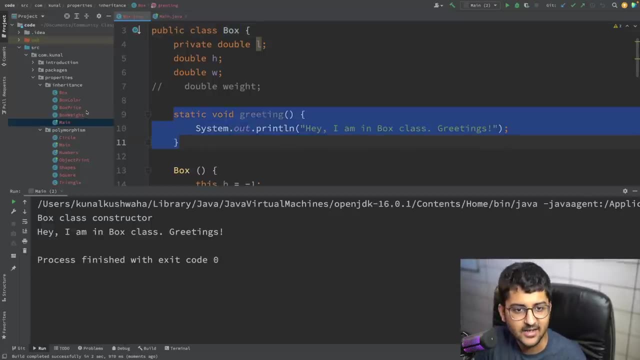 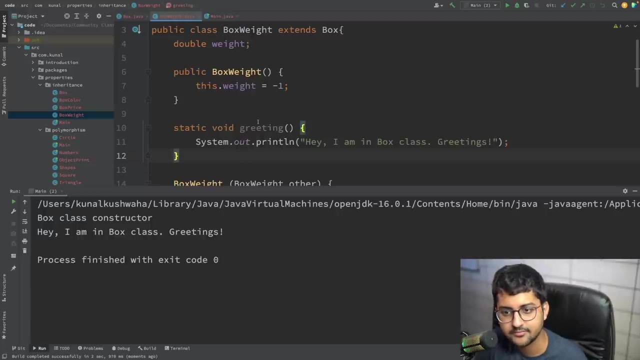 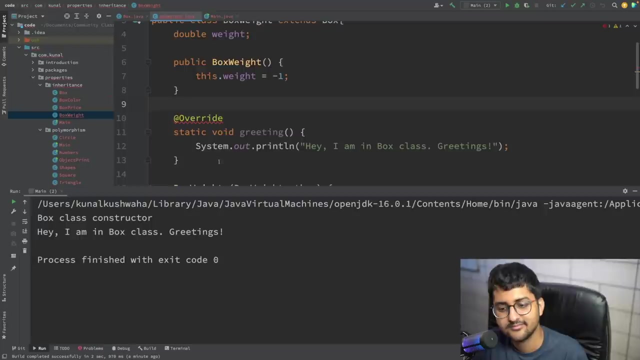 that okay. so this is cool. but the real question is: can we override static methods? what if i have another static method or something like this and let's say box: wait, okay, let's put a override over here. it's actually not overriding it. it's actually not overriding it, not overriding it, it's not. 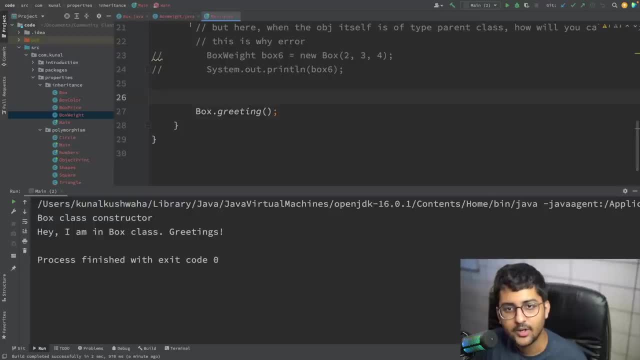 overriding it. so if i put it like: if i just put this check on hold, this is just for checking purpose, but it's not overriding it, okay. so here i can say so, here i can say: okay, box, box, box is equal to new box. wait, we just covered this type. is this whatever, whatever. okay if 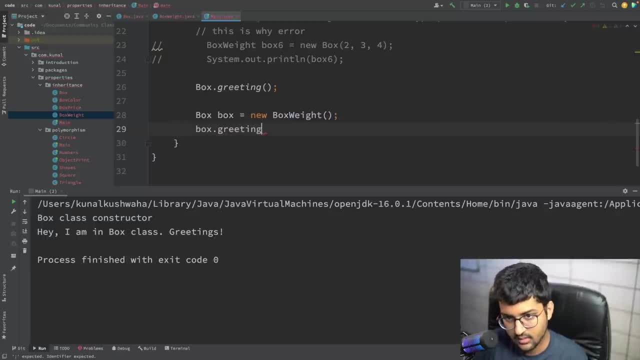 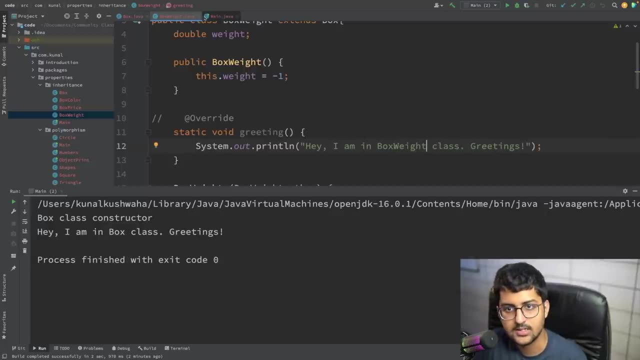 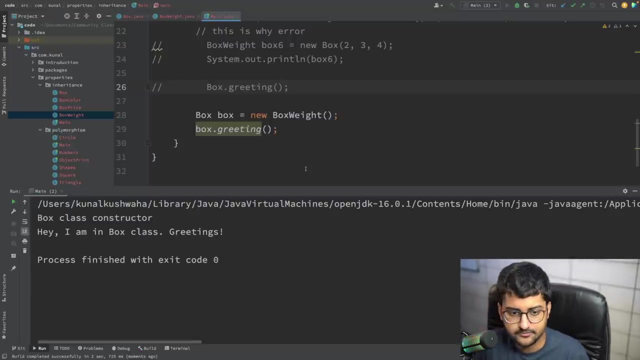 i say box dot greeting. this should be a: hey, i'm in box, wait class. let's run this thing, let's see what we will get. let's see what we will get. it's saying i'm in the box class. it's saying I'm in the box class. 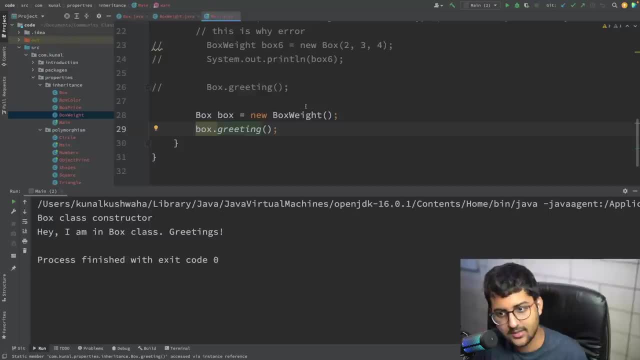 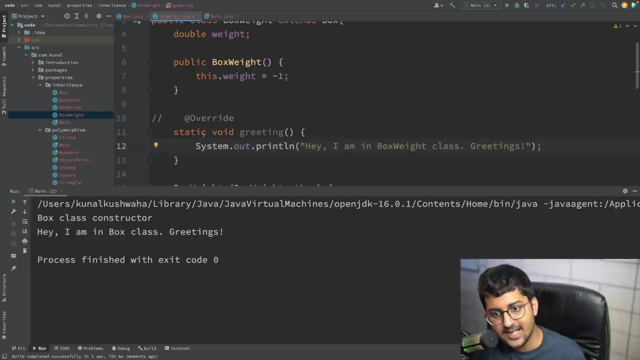 so did it actually get over it? and if it was getting over it and that all the previous things we mentioned, what two access will define this? what which particular, which elements that can access can define this? which one will actually get accessed defines this? but here it's saying the base class one is the child, class one is not getting called. it's. 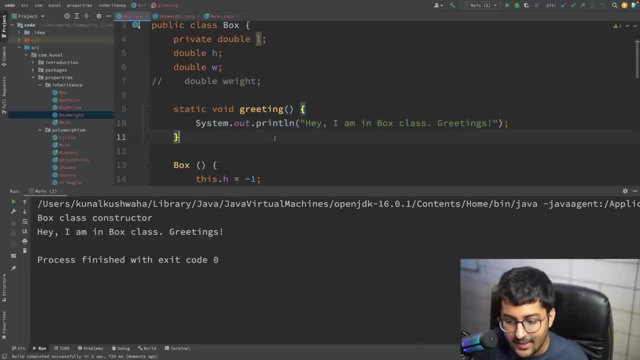 calling this one. only still, what is happening over here? think about it. all those static, static methods are being inherited. there is, let's say, imagine they are being inherited, imagine if they were getting inherited. there is no point in overriding them in the child class, because the method in the parent class will always run, no matter from which object you call it. 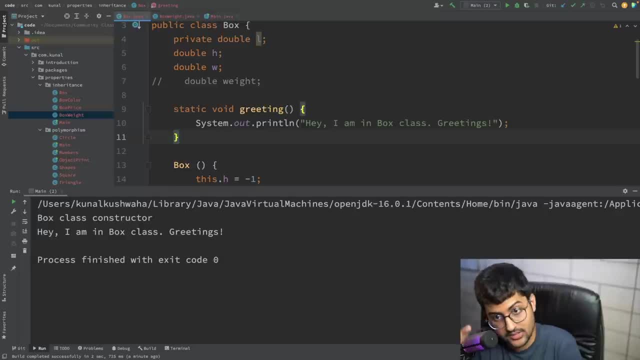 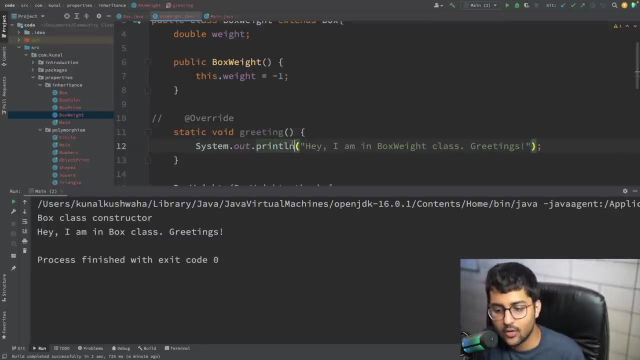 make sense because it's not dependent on object, because it's static. that is the reason that static methods like over here that we have, they are actually the, the static method over here that i have. that is the reason this one is not being called okay, because the one in the main class is actually one being called class dot greeting. 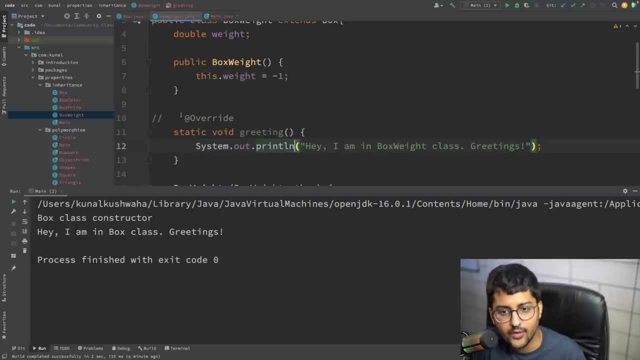 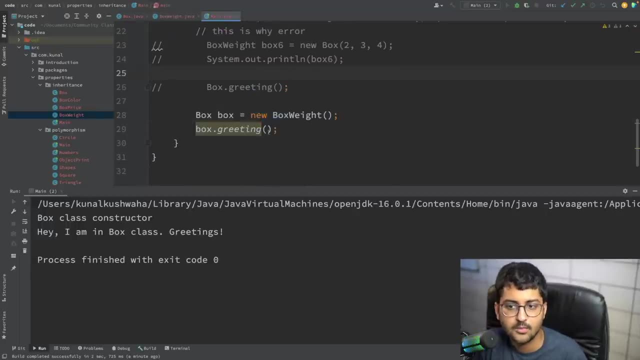 it's not actually dependent on this thing. even if you remove it from here, it will still work and it will still work. it will still show the same output. let's try to print it: box weight, it will still. now, it's nothing. it's not overriding or anything, it's just the normal stuff. 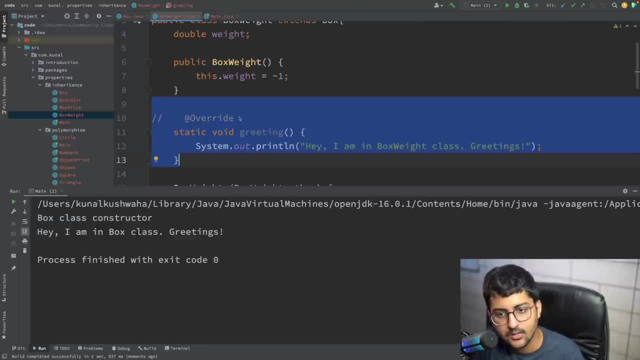 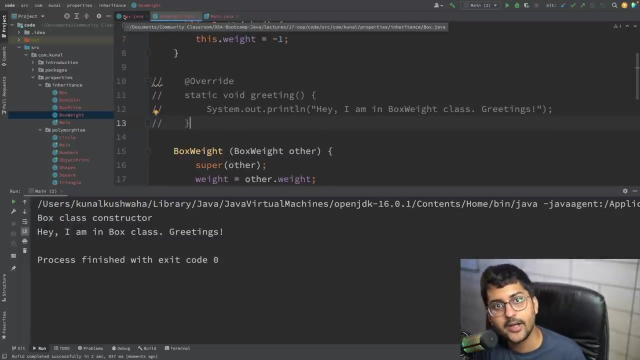 you put it over here, override over here, it's actually, you can see, it's actually not overriding. so static methods as such. you, you, you cannot override them. okay, you can't do it, even though it can be inherited. it is being inherited, right, you are able to use it via box weight. 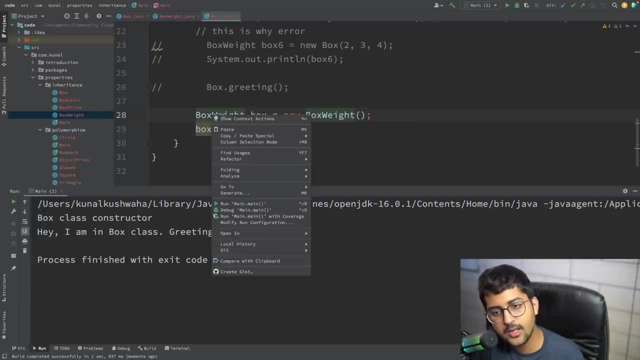 yes, this one is called theлекс wave box weight object. even you put this as box weight, you will still be able to use it. static methods can be inherited but cannot be overwritten. why? because the main class one is obviously always going to be called. it's not dependent on object. that's why it. 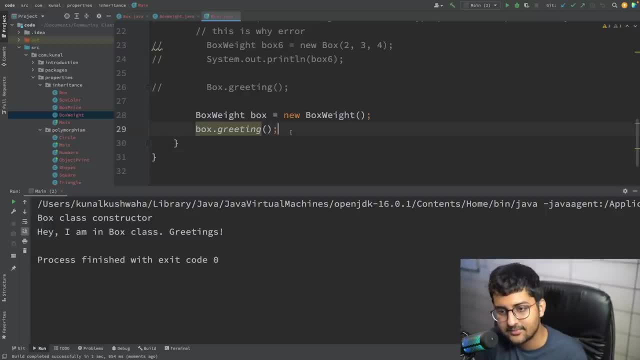 does not really matter. see, the thing is, overriding depends on objects, static does not depend on object and static methods cannot be overridden. oh, that was so quick, so that's why i people tried that to me. leave that rule in your tasks team here. dude, that's the most beautiful thing. 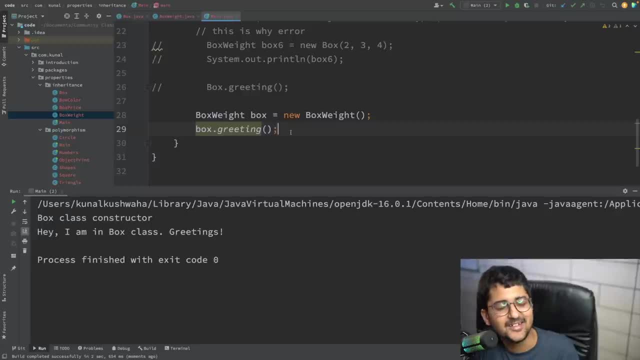 to know here, guys, all theอστ mate sãocin damageIs course you can pause for few. second is again. ärzeов was a good explanation, so very simple. oh, how i was confusing it. uh, irrespectively, no, this is a very easy explanation. overriding depends on objects. static stuff does not depend on object. 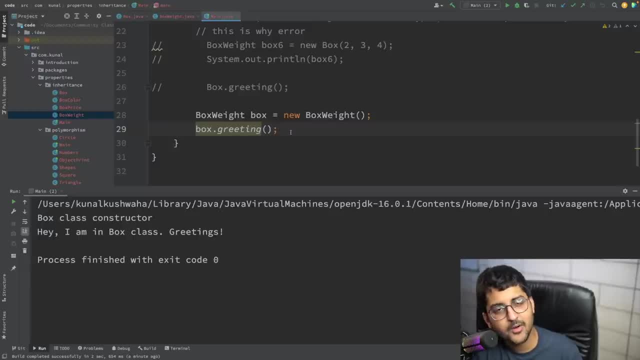 hence you can't override static methods. because in order to override something, you have to deal with objects. but static stuff eliminates all the objects, hence you can't override it. the one you have in the main class, that is the only one, will be used. why? because overriding deals with objects. 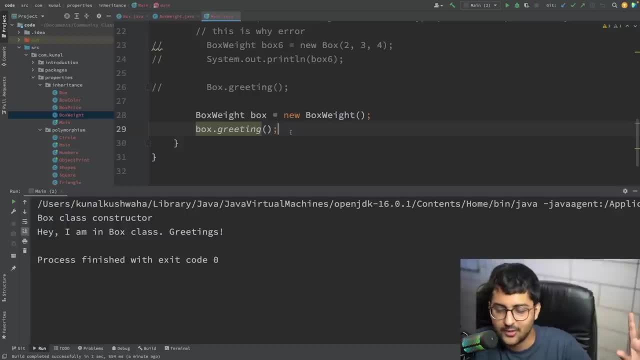 static does not deal with objects. that is like i don't really care which object you belong to, i will run irrespectively. this dynamic method dispatch will not happen if it's static. right, that's pretty much about it. cool, all right, you can also do box weight, dot, greeting, or. 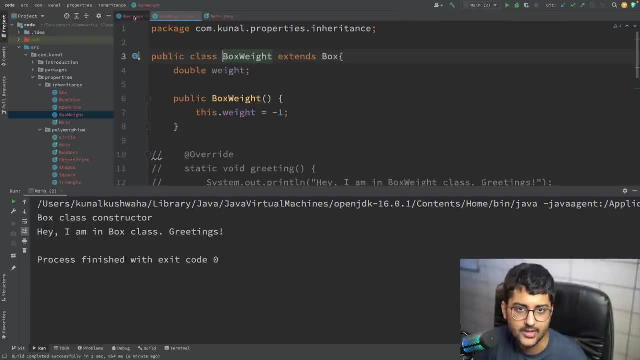 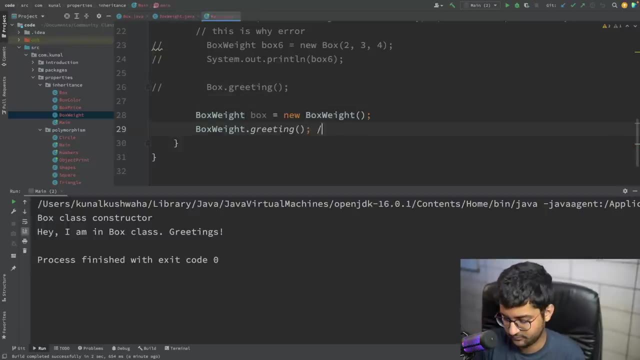 something that's also fine. it will be like: hey, does box weight contain greeting? no, it does not. this contain greeting. yes, it does inheritance: it's being inherited, but it's not being overridden. you can inherit it, but you cannot override. you can run, but you can't hide. nice, all right, you can run, but you 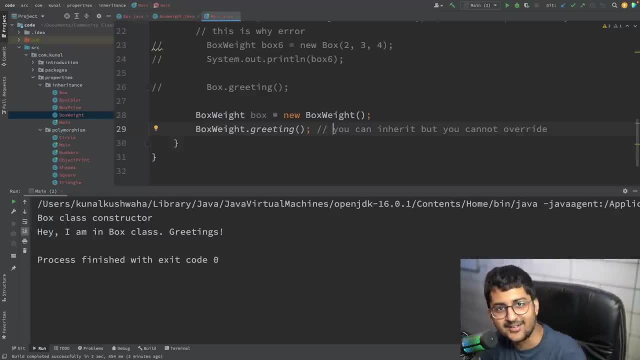 can't hide, you can inherit, but you can't override. tweet that, tweet that or something. uh, all right, cool, tweet that. share on linkedin. nice, nice little line. you can take a screenshot. cool, subscribe like share. make sure you comment it as well, all right, um, easy peasy and very easy stuff, so that's it, yeah. 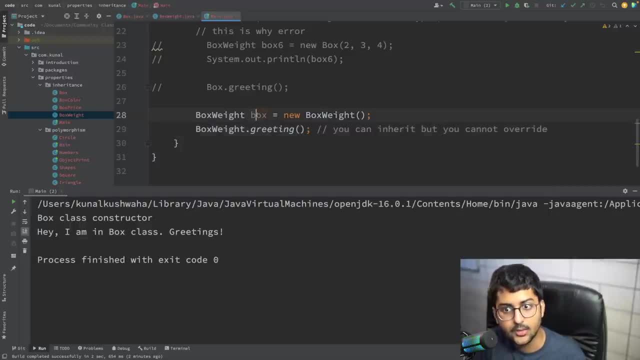 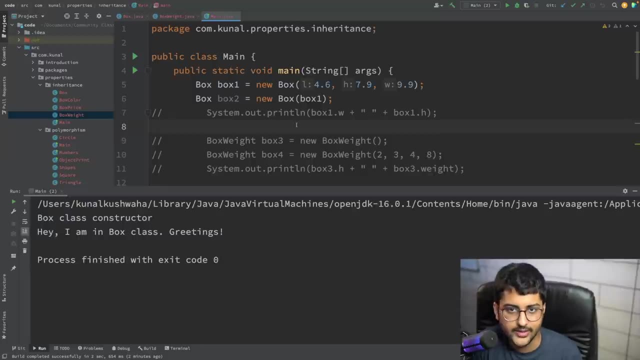 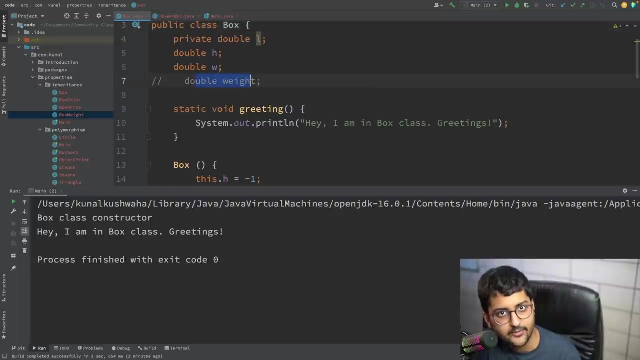 cool. uh, one more thing. this polymorphism thing that i talked about does not apply to instance variables, okay. instance where we treat it like no on its own, okay. so i gave you an example of, like adding a weight over here as well and a weight over here as well, the commented one out, you can see. 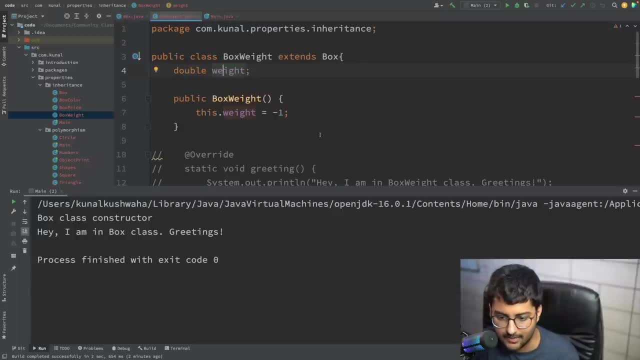 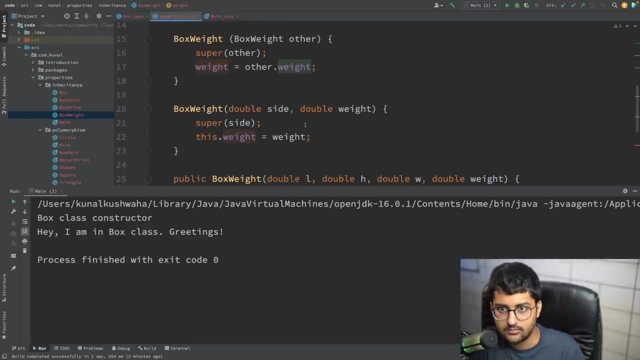 it was calling the using the super keyword or whatever. so it does not apply to instance variable. both this overloading and overriding does not apply to um. what does not apply to instance variables? okay, and obviously you cannot override the inherited static methods, because overriding in java takes place- uh, you know, by resolving the type of the object at runtime. 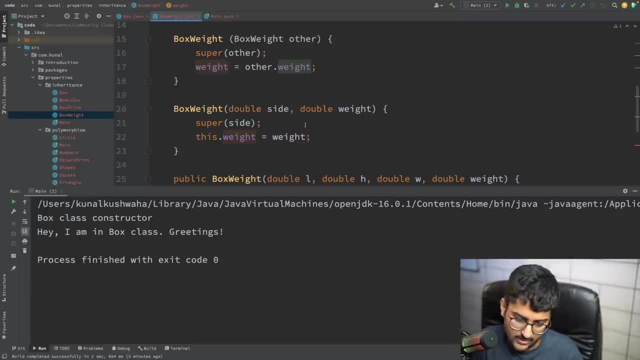 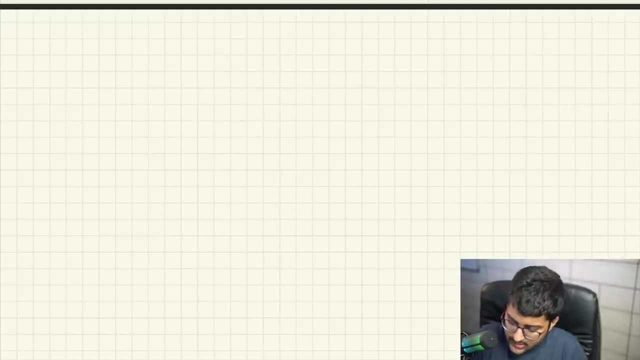 and not compile time and then calling the respective method. but that's it. yeah, cool, let's move forward. okay, now let's look into the third property of object oriented programming, which is known as encapsulation- encapsulation- what do we mean by encapsulation? so encapsulation means wrapping up the implementation of the data, members and the methods. 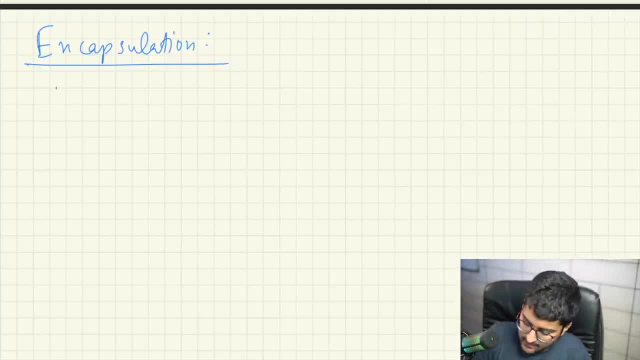 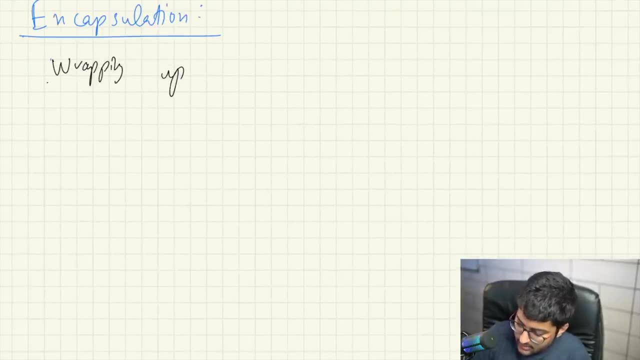 inside a class. wrap up. it means wrapping up the implementation of the what, data, members and stuff like your variables and all these other things and the methods in a class. okay, that is what we mean by encapsulation. it basically hides the code and all the data into a single entity or a unit so that that can be protected from the outside world. 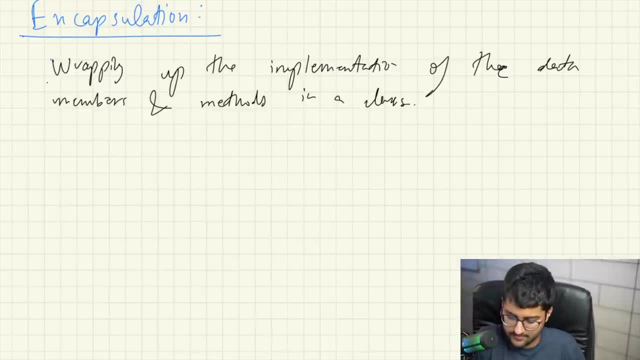 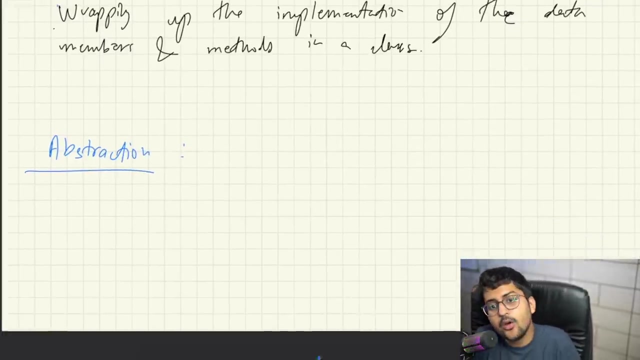 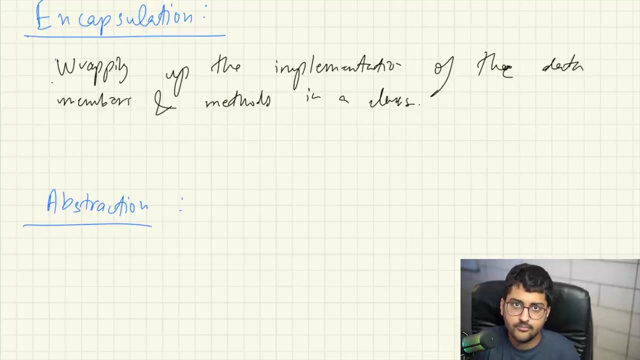 okay, that is basically what encapsulation is, and one more thing that people confuse encapsulation with is known as the fourth property: abstraction, abstraction, abstraction, abstraction, abstraction, abstraction, kunal. what is abstraction? abstraction, on the other hand, means hiding the unnecessary details, but only showing essential information. so, hiding unnecessary details and showing valuable information. 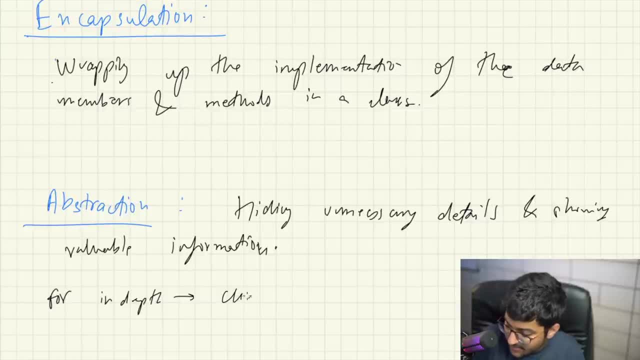 for in-depth check my video that i'm making right now. since you are already watching it, you are you already on the right track? this is just for people who will take notes, check video and notes. notes i'll upload on github. okay, but since let's now cover in details of this, in the detail of this, 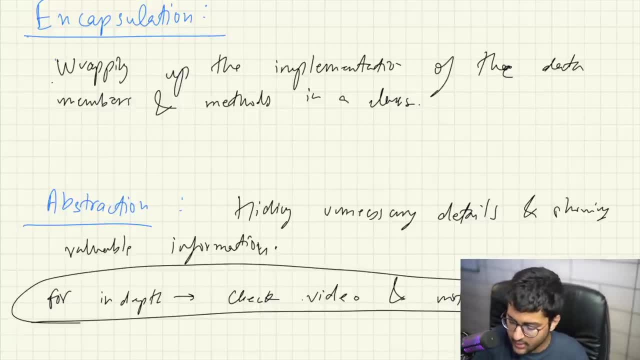 okay, because i'm not going to write everything that i already will be pushing in the note section. let's focus on understanding first. what do we mean by abstraction? so let's say you have a car, you have a car, you start your car, you put in your key and you start the car. 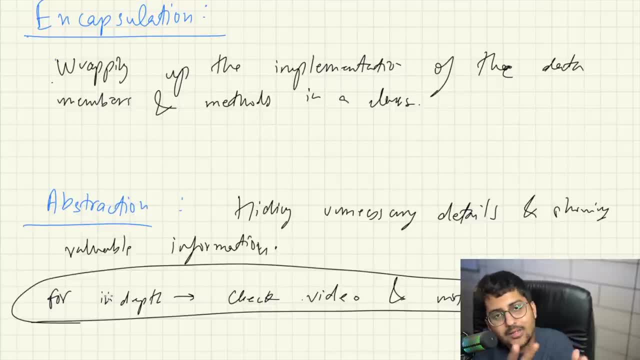 that is what you do. put in the key: start the car. how that car is being started when you put the key and run it. how the internal implementation is how the engine starts and the petrol pumps and the car gets started. car moves all the internal mechanics. do you really need to know these things? 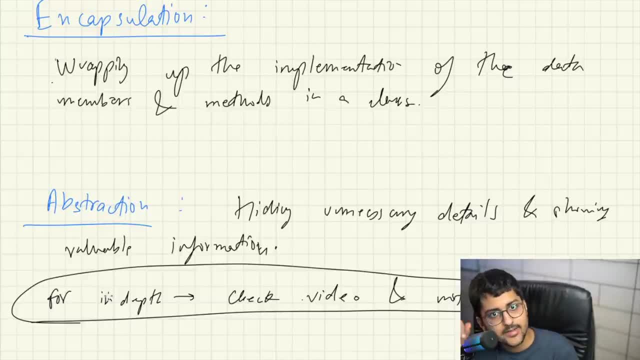 in order to start the car, or all you need is a key, all we need is a key. so this, all the necessary information that is obviously, let's say, important, but we don't really key. it's gonna take the about it. do you need to know the mechanics of the car in order to run the car? no, so all this extra. 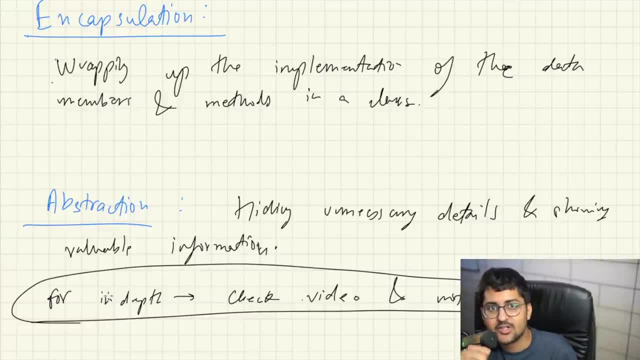 information is hidden from us. this is known as abstraction. i am 100 sure you are confused between abstraction and encapsulation. i am 100 sure you will be thinking this is the same thing. no, let me explain to you what the difference is in a really awesome way. so abstraction is more like 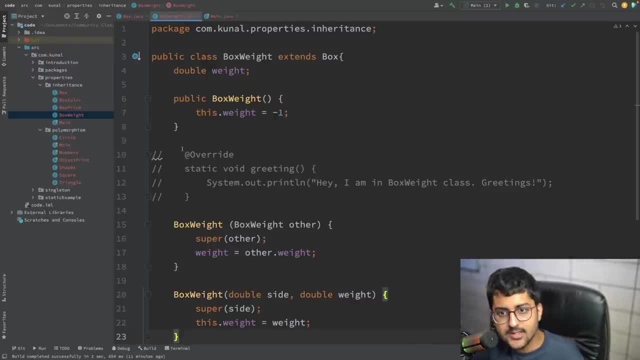 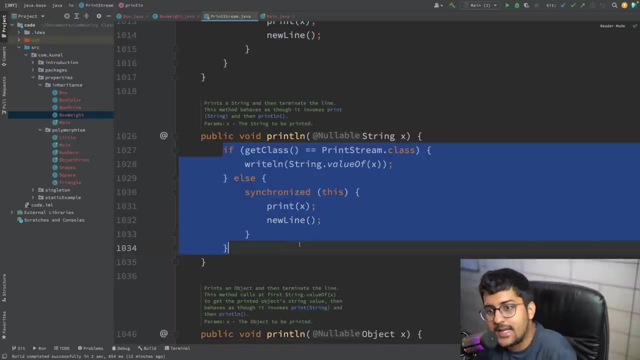 this here. you can see whenever we create an array or whatever, right, when we say uh, or when we say print ln or something like this: systemoutprintln. we just wanted to print this thing. okay, we just wanted to print this thing how it's doing it internally. i don't care how this thing is. 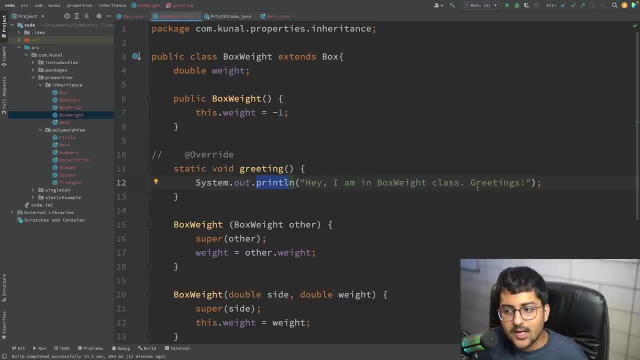 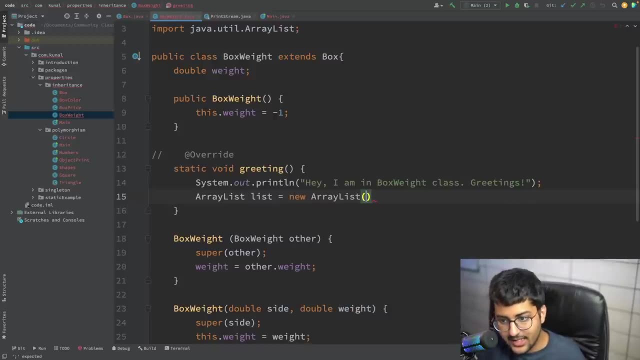 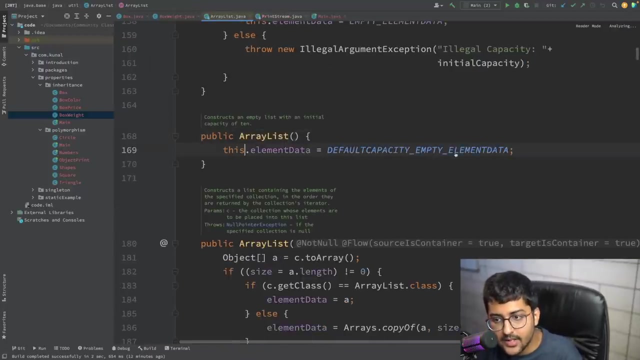 happening. i don't care, i'm just using it like this. similarly, you are given many, many classes that we have used before, like array list. list is equal to new array list. you are using this array list. okay, you are using these array lists, right. how this is defined internally, how it's made internally, all these things. 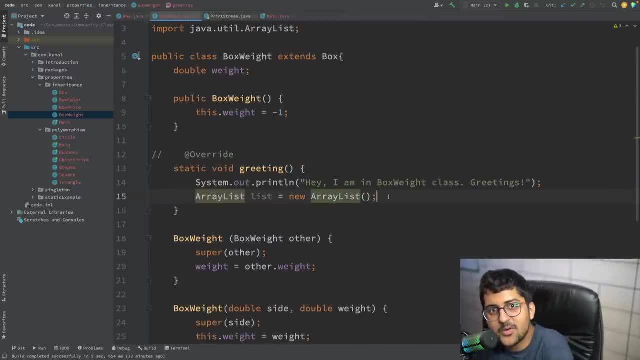 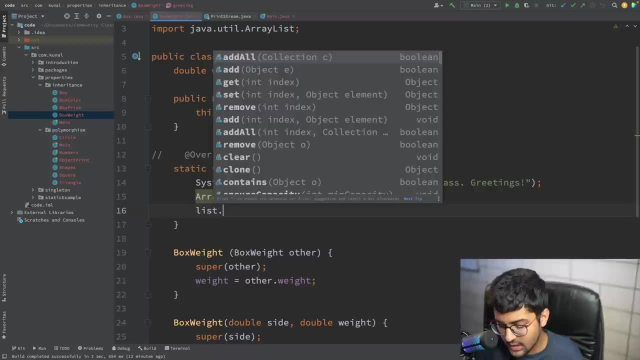 do you really care about it? no, this is why these are known as what abstract data types as well. abstract data means you are able to access and modify this using some methods like get, print or whatever, get or add or set or add all, remove or whatever, but how these are working internally, i 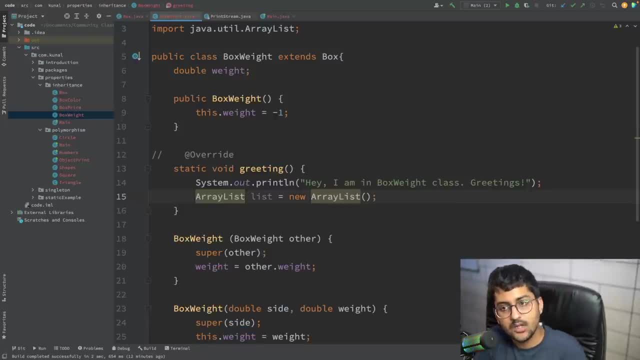 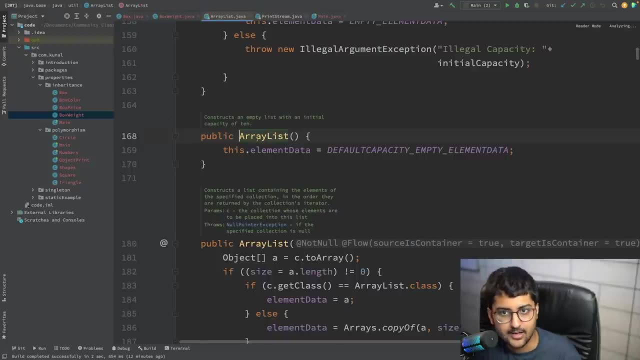 don't care about it. another confusion you may be having is kunal, but you said encapsulation also means the same thing. encapsulation means putting data inside a class and that is what you're doing over here. this is the array list class and you're putting data inside it. you are. 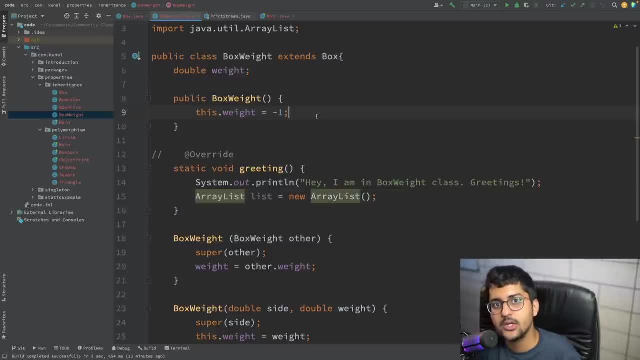 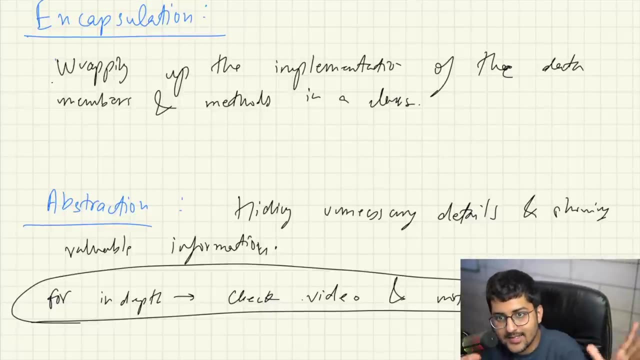 correct, then you'll be like: okay, then how is abstraction different than encapsulation? let's see. so abstraction means hiding the unnecessary detail, but only showing the essential information. start the car, get the element, print the element. okay, so this is a design issue. how it's actually being? 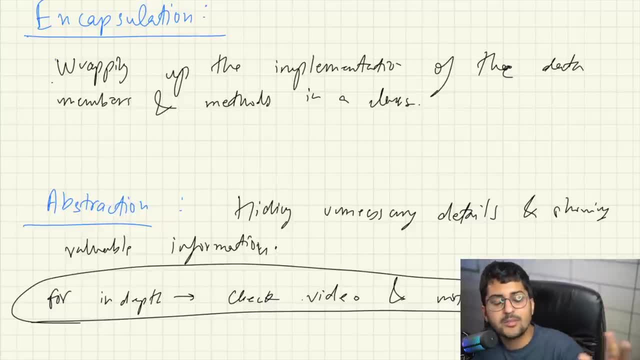 designed. the designers will tell you: hey, we need some sort of an abstraction like put: give me this method, this method, this method and whatever you put inside it. that is up to you. whatever how you do it, how you encapsulate it, how you put methods in that, how you put a class in that, 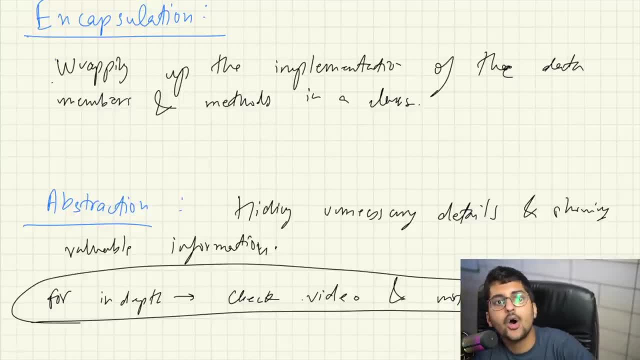 how you make it work inside internally. that is up to you. all i need is these four methods. so these are the designer people. they will tell you this thing. the people who are working on the implementation part, the engineers, for example. they will be like: okay, we are working on. 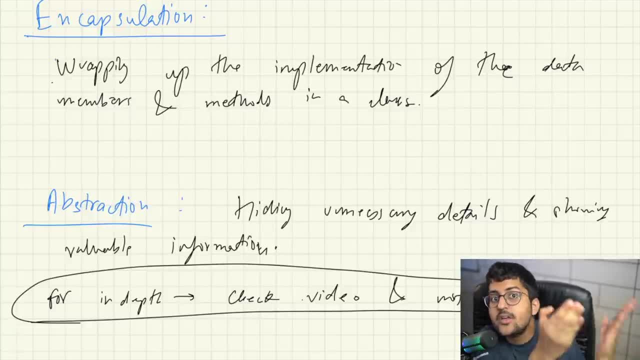 implementation. you want this sort of abstraction. we will achieve it via making this class, via making this particular method, via making this get method, this set method. this is what it will contain. so the actual writing of code, of that encapsulated thing that is providing us abstraction, that is the 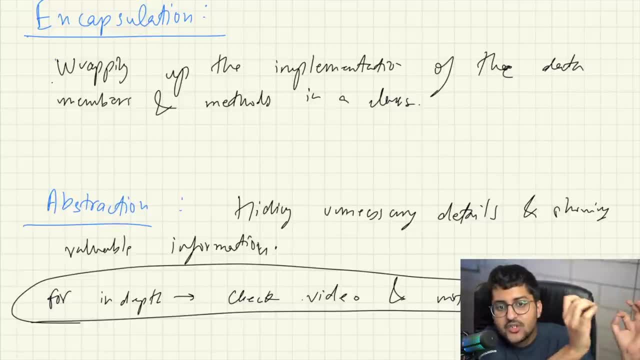 main difference. if someone asks you what is the main difference? abstraction is solving a design level issue. encapsulation is solving an implementation level issue. okay, so it hides the entire code in a single entity or whatever and protects it from the outside world. abstraction, on the other hand, is telling us that, okay, encapsulation did all these things. it's. 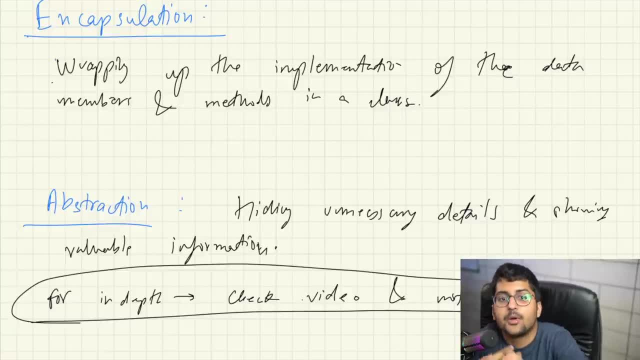 hiding something internally. I am abstraction and I am providing you some of the outside methods that you can use design way, but how this thing is working internally, that is handled by encapsulation. so encapsulation is the implementation stuff and gaps. one more simple explanation: abstraction focuses on the external stuff, encapsulation focus also on the internal working. okay. 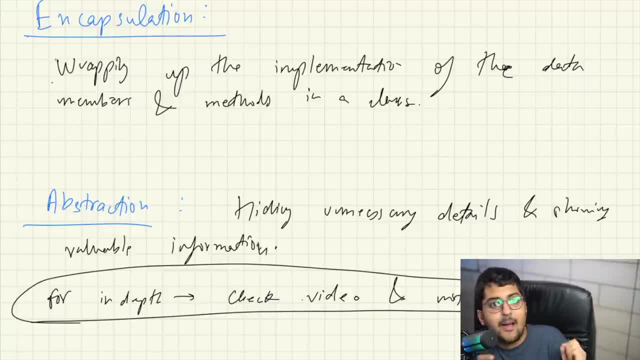 how do we achieve abstraction? you can achieve it via, like abstract classes and interfaces, which we'll talk more about in the next video later, abstract classes and abstract data types and stuff they have like only give us add method or remove method or whatever how that thing works internally. 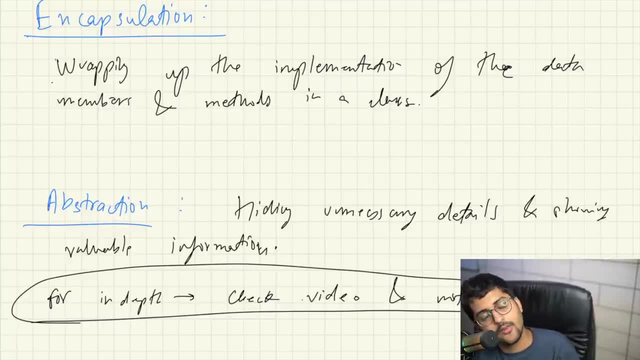 I don't care that something else like in the internal working of encapsulation when that was done in order to make that class, that was taken care in encapsulation. I am only focused on abstraction, like what are the things that are visible to me? and encapsulation means what are the bad things, not the 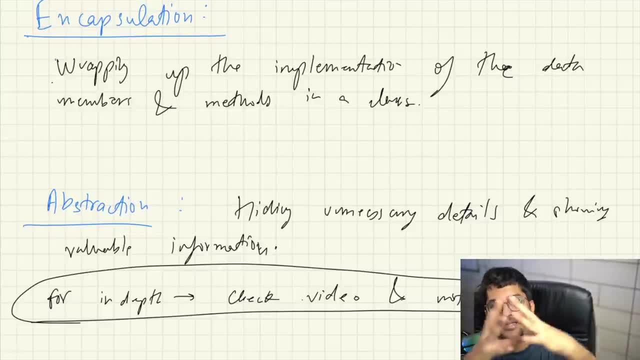 bad things, but the complex things that I need to work with. I put everything inside a class, make it public or private, or hide the data, members or whatever. that is encapsulation. okay, so abstraction is done using, like abstract classes, interfaces. encapsulation means putting things inside classes, hiding the internal details and stuff like that. 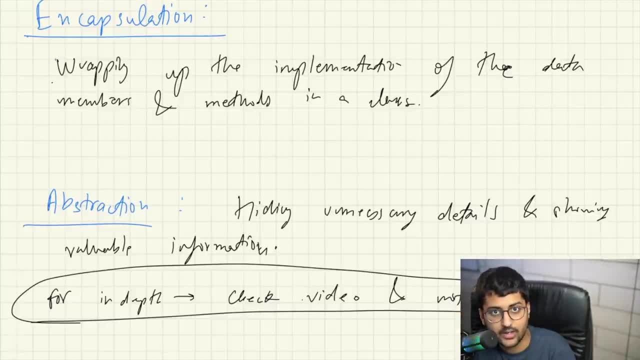 into a single entity, using, like public, private, protected methods or whatever, just like. I will give you an example of that as well. okay, one more point. abstraction is a process of gaining information. encapsulation is a process of containing the information. okay, so, in abstraction, we are using, we are going to use the interfaces and 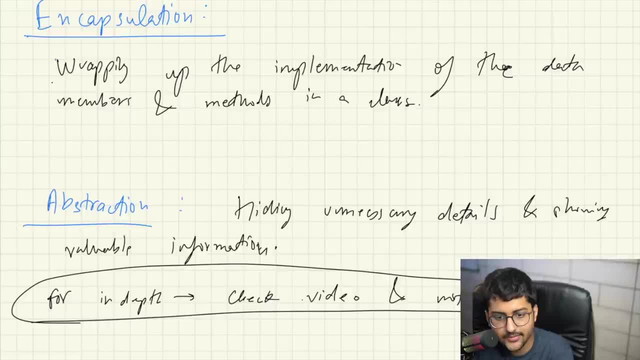 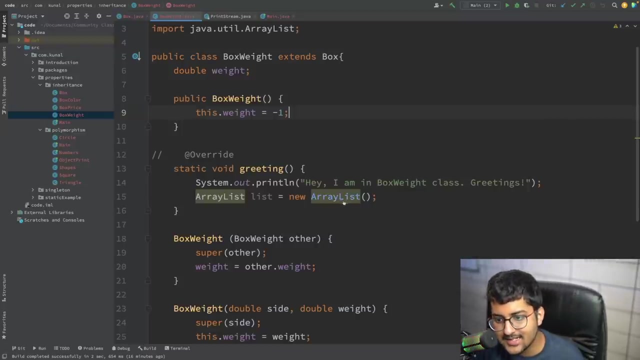 stuff that only define the structure of the program and not how it does it, and that is something we'll cover later on. okay, so the objects and stuff that we created, they were all encapsulated. okay, cool, as simple as that. right, let me show you one example, so in the array list example. one more thing I 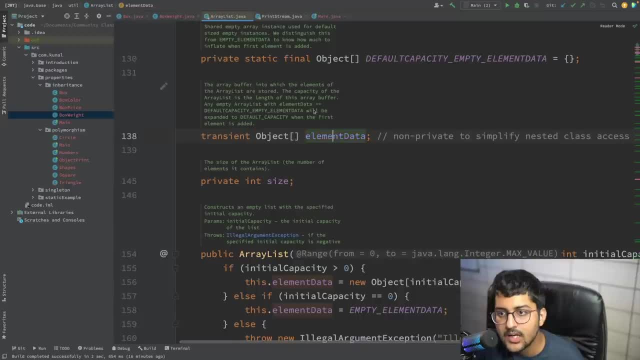 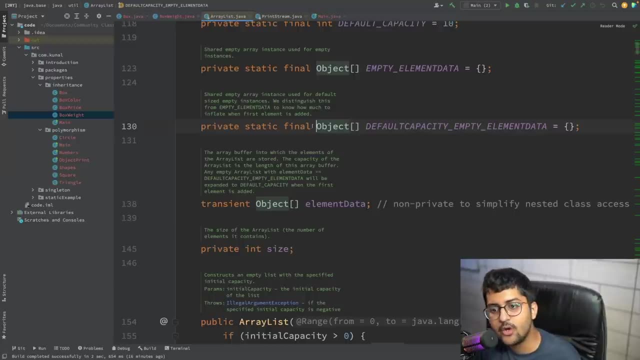 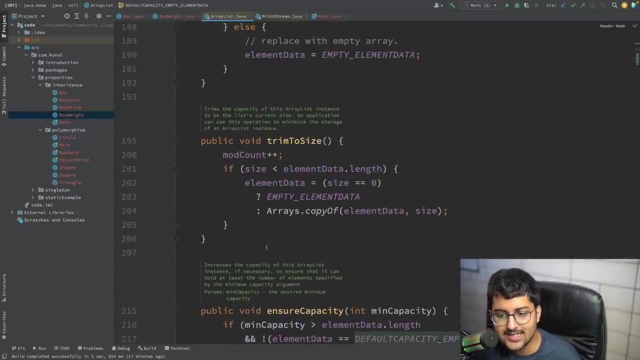 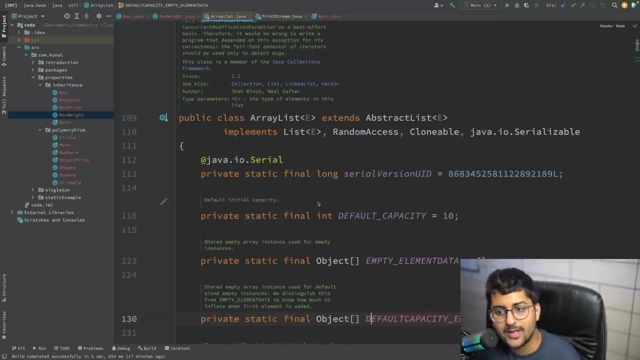 want to show you is that this thing- let's say this is your object, empty array or whatever. you are able to manipulate this or whatever let's say- let's assume this is the one- you are able to manipulate it via some getters and setters. okay, like grow size or add in it or whatever. right, you are able to manipulate it. but 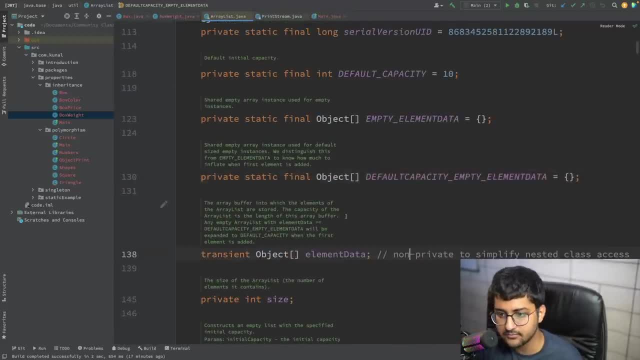 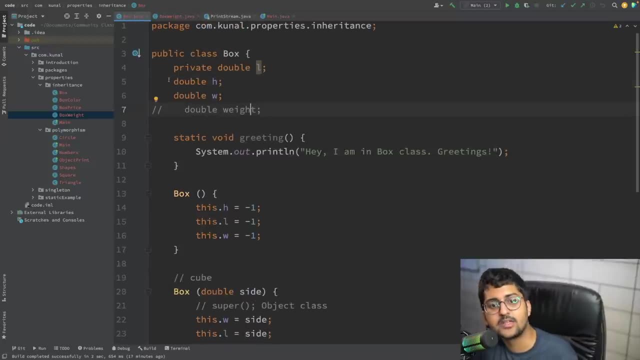 you are not able to directly manipulate it. you can't say directly: not this thing. let's say I create another one or we actually had one, for example, this one. you are able to set it via some constructor or whatever. if you want to get it, you can create a. 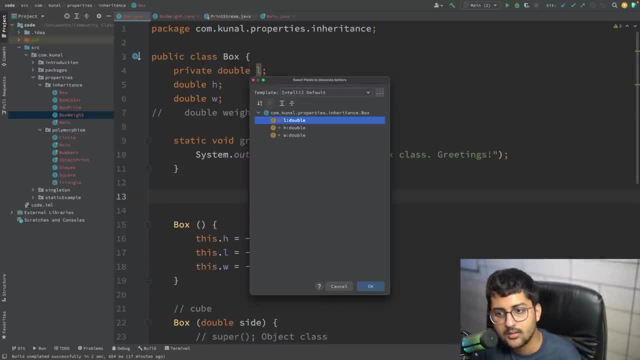 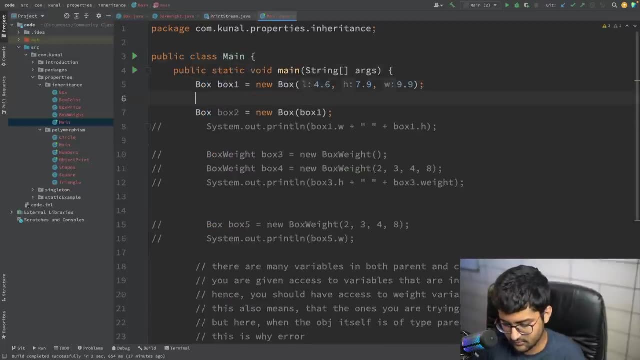 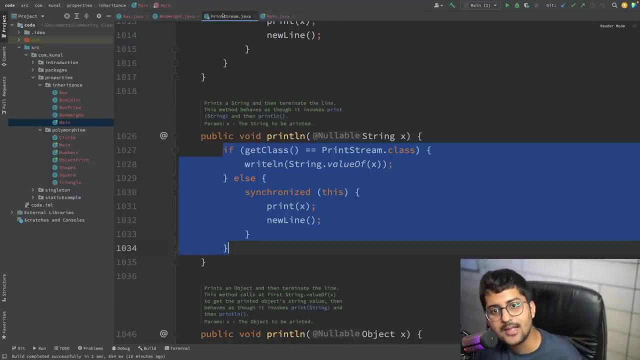 get method getter l. you want to get n. you can just say in the main, you can just say boxget l, this will print you the value of l. now you are like, hey, kunal, l is actually private. l is private that. how are you able to print it? 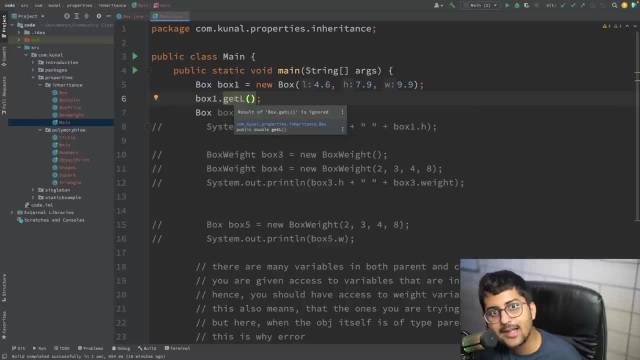 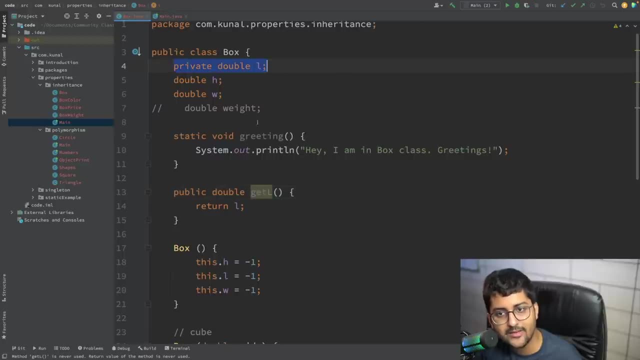 in the outside class. think about it. i am not directly accessing it, i am accessing it via a method that is used inside that class only. since this is in this class only, it can definitely access the private methods- sorry, private variables. so this particular thing of making stuff private like this, 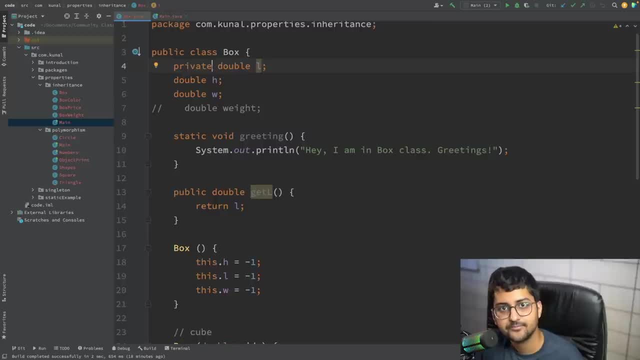 this is known as data hiding. ok, i am pretty sure you are able to understand encapsulation versus abstraction. ok, encapsulation means putting all these things, like you know, in a bundle. it is like something like this: you can use getters and setters for that. ok, so you know about encapsulation. now you know about. 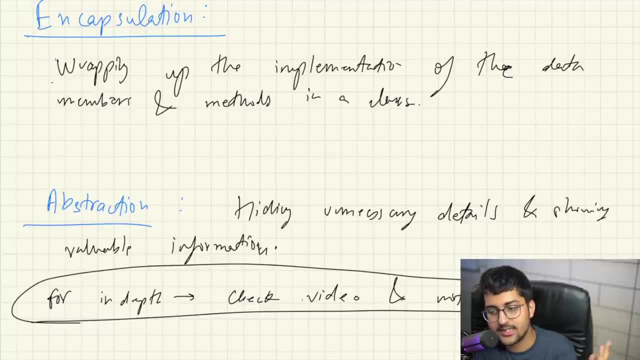 uh, data hiding and stuff. now, so you can hide the data using this getters and setters. this is known as encapsulation, the exactly same thing that i did right now. and in order for abstraction- to use abstraction, you can use, um, what you can use, abstract classes and interfaces that we will talk more about. 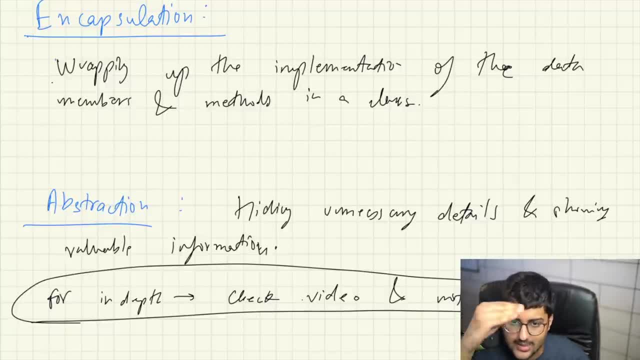 in that lecture only ok. but abstraction is what design level, external outlook, how the car is- just you need to start the car. but encapsulation is more on the internal working, the implementation, how those things are. it is the process of like containing that information, how to make it more secure and stuff. 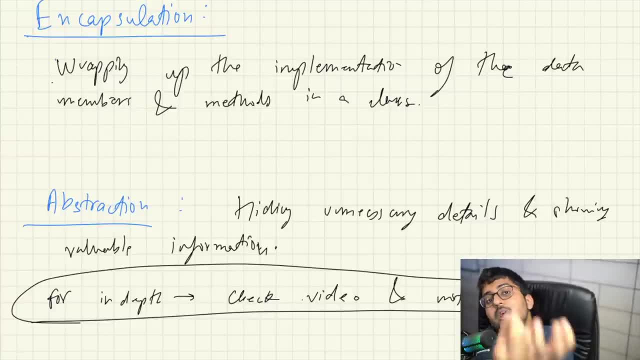 but abstraction, on the other hand, is actually gaining information, process of gaining the information. ok, so in encapsulation we use like getters and setters and classes and stuff. in abstraction we use abstract classes and interfaces. only problem you may be having now is kunal. what is the difference between data hiding? 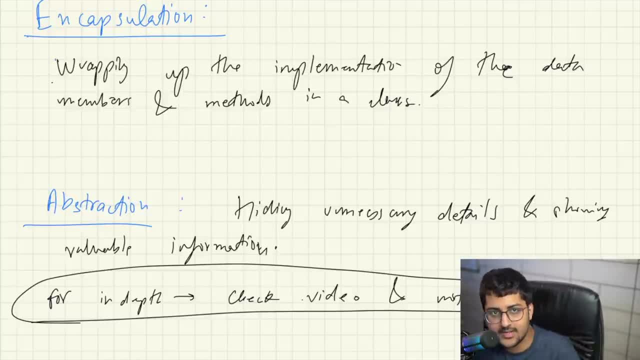 and encapsulation. kunal, you told us abstraction once again versus encapsulation. that is fine. what is the difference between data hiding and encapsulation? main difference between data hiding and encapsulation is that data hiding is focused on data security and encapsulation focuses on hiding the complexity of the system. 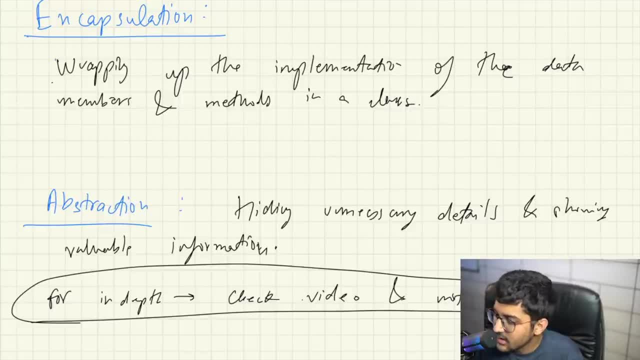 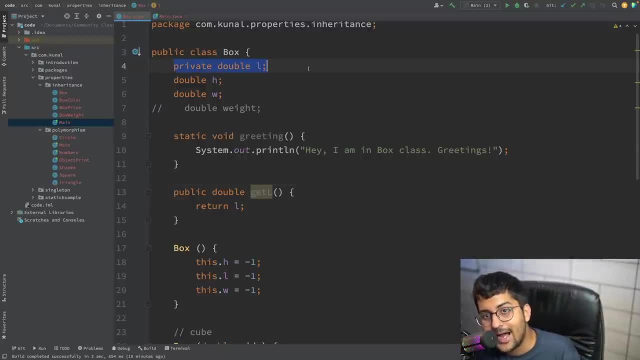 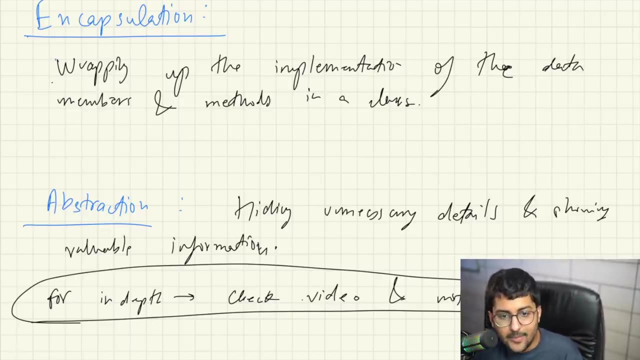 ok, for example, here you can see that you are not able to access this data member. ok, so this is actually actually data hiding. ok, this is actually data hiding. using this getter setter is actually encapsulation. so basically, data hiding. data hiding- the concern is for data security, along with hiding the complexity, but encapsulation. 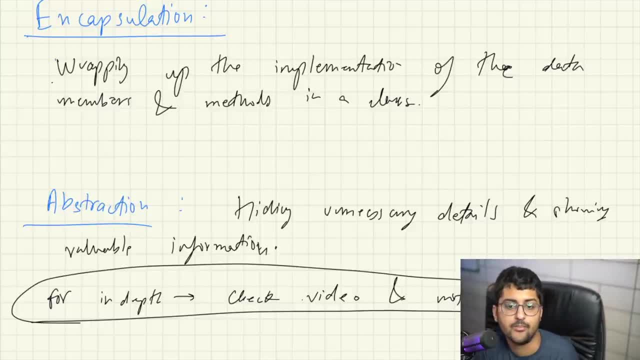 concerns only about wrapping the data to hide the complexity of the system. okay, so in data hiding, always the data that we are hiding is should be private, it should not be accessed directly. but in encapsulation data can be public or private or whatever and encapsulation I can say, you can say when our encapsulation sounds a little bit similar to data hiding. 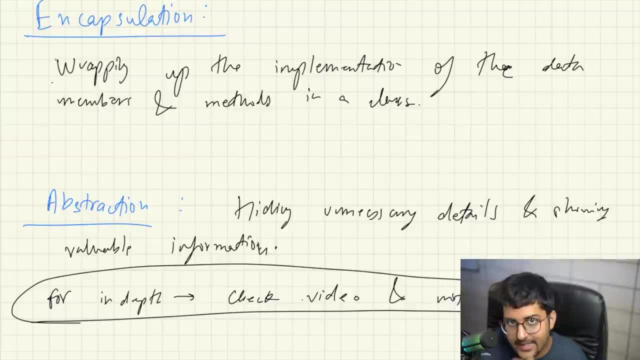 that is true. encapsulation is a sub process in data hiding. it's a process in data hiding. okay, so if you're making an array list, internally, let's say it's implemented as a normal array, or you're making a linked list and internally let's say it's implemented as a normal array. 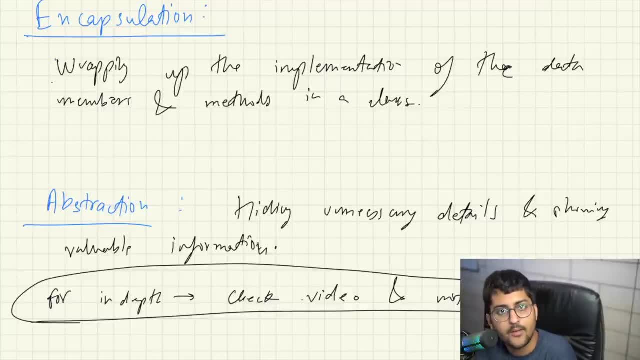 you should be able to modify that linked list. okay, via some linked list dot. get list dot update type. want to do that, right or not? okay, that's all. so I highly recommend you take list dot remove, but you should not be able to directly access that array. that array should. 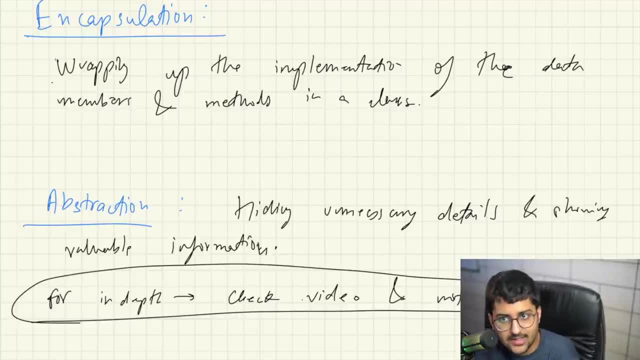 be private. that is known as data hiding. but using these methods like getters and setters, that is encapsulation. okay, so in data hiding, always put it as private. okay, so data hiding can be used to, like, reduce the you know some complexity of systems and things like that and data hiding. 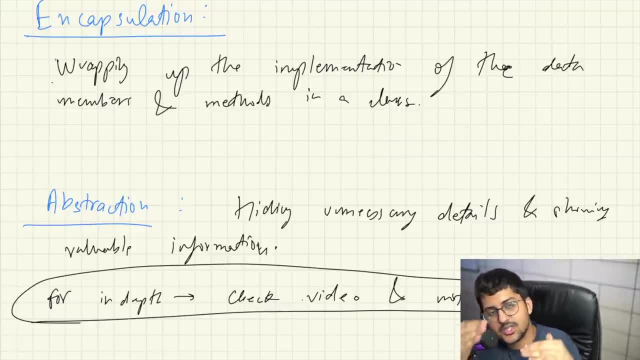 is actually achieved via encapsulation, and encapsulation is sub process of data hiding, exactly like that. that is it, yeah, cool. so i believe that gives you a bit more understanding. so that was about encapsulation and abstraction. about abstraction, uh, encapsulation we did in this video. this entire thing we did. 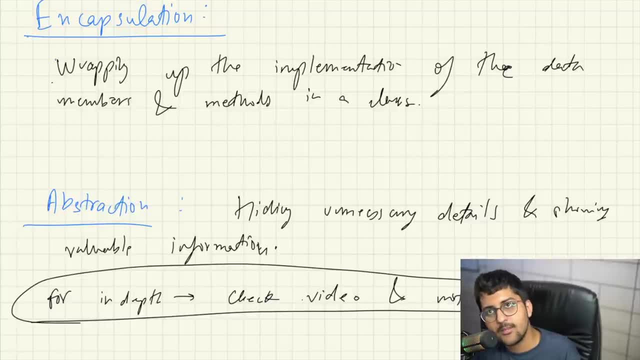 was encapsulation only, but abstraction is more on the ROBOTIC DATA HIDING, EXPERIENCY, MECHANISM, implementation level. okay, it's used by abstract classes and interfaces and stuff and i already explained what the differences are between these two. and if someone asks you what is the difference, 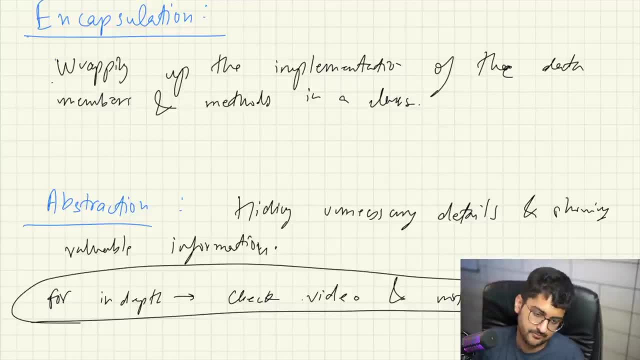 you can say: abstraction is design level, encapsulation, implementation level, things like: okay, so putting the car, starting the car- i know all i need to do is start the car is like that, but how it actually is made, the implementation of it, that is encapsulation, writing the code. you. 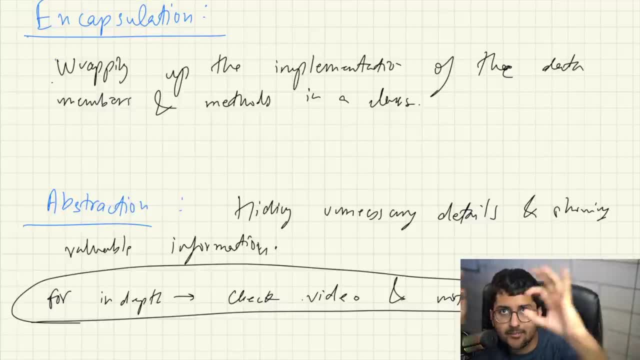 know, like putting the code inside a file, inside a class, add in some methods that's private, putting some getters, putting some setters, all of these things that i just mentioned. this is encapsulation, but getting that outside just main main methods, the abstraction, uh, of all the internal hiding. 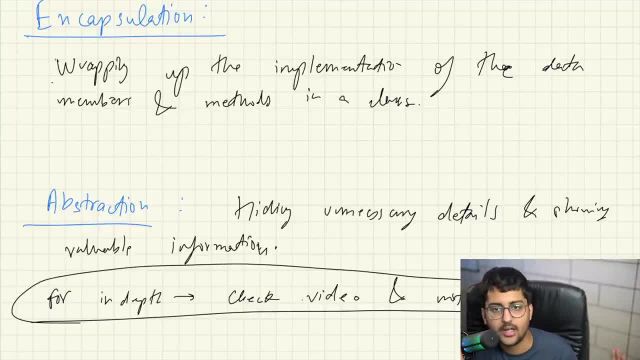 the unnecessary information, like i don't really care. i don't really care what, how it's working internally, but in encapsulation you do care how it's working internally because it's it deals with that total implementation only. okay, that was about abstraction and you encapsulation. 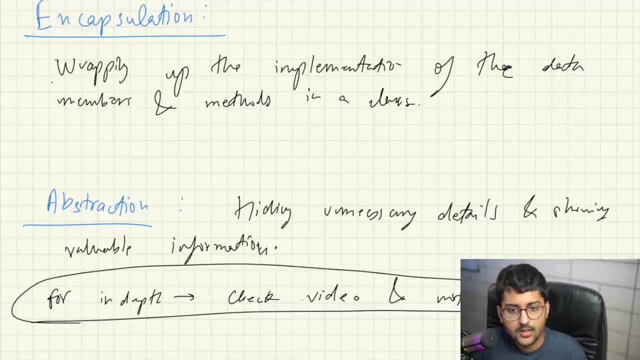 cool and that was about properties of object-driven programming. in the next video we'll look more into abstraction part, so we'll look at uh like access control and object class and stuff and object cloning and we'll look at like, uh like access control obviously is important, because i talked